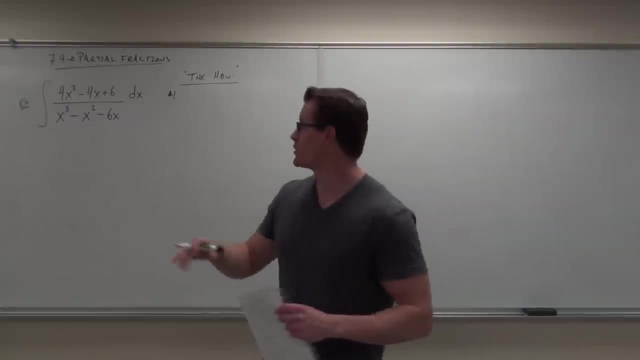 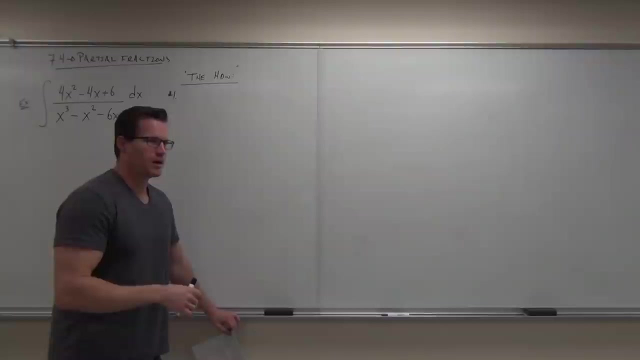 They're not like x to the negative three. They're not x to the one half. Polynomials are things like this and things like this. Those are polynomials. If you don't remember what those are, those are polynomials. Every polynomial in the world can be factored as a product of linear and or linear functions. irreducible quadratic factors that's it that's a law and we're not a law that's a a theorem approved theorem in algebra so every polynomial 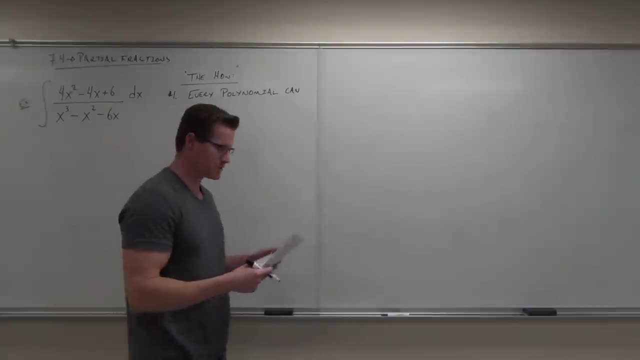 can be decomposed decomposed means broken up in different parts can be decomposed or can be factored into a product of linear 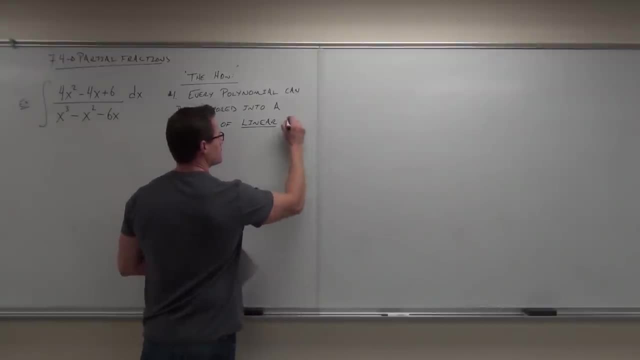 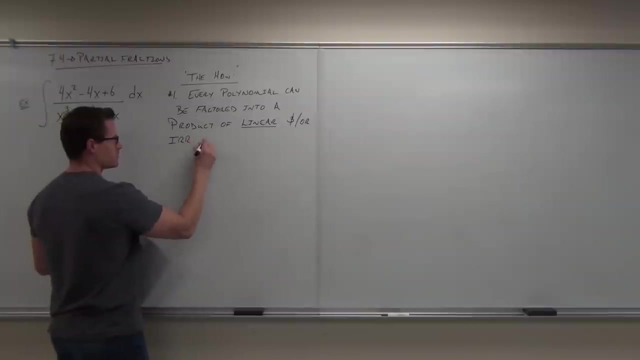 and or irreducible quadratic irreducible and quadratic 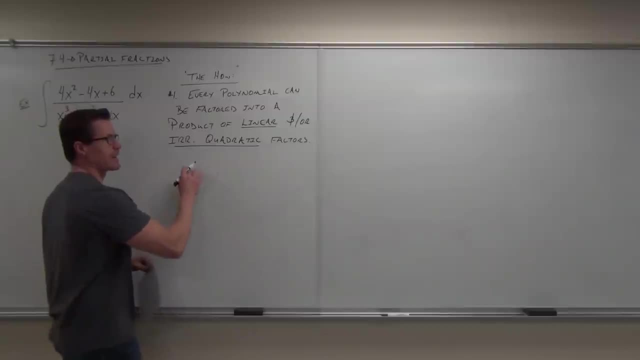 basically here's what this says if it's linear linear and irreducible quadratics it means this ax plus b 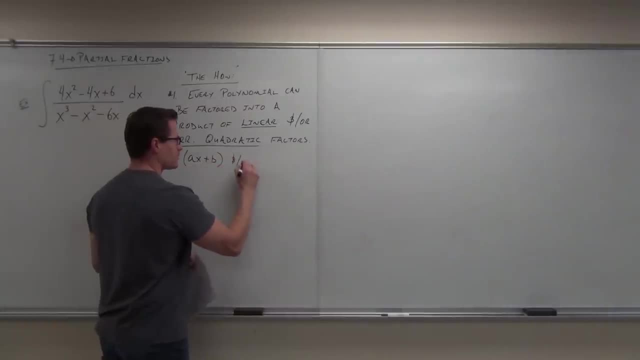 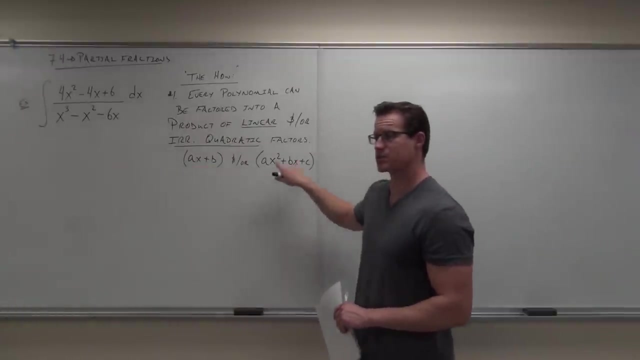 and or ax squared plus b plus BX plus C. Every polynomial in the world can be factored as stuff that looks like this and or stuff that looks like this. 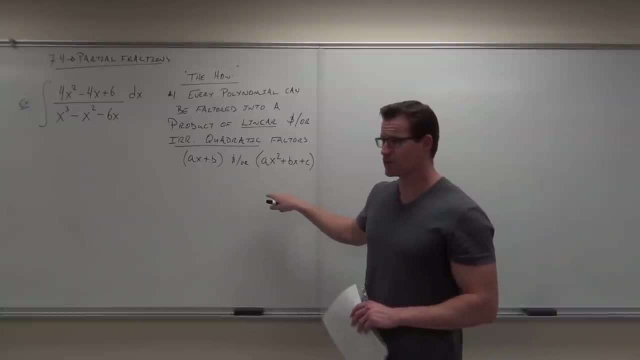 There are some quadratics that you can't factor. We know this, correct? Hopefully we know this. Some quadratics have complex factors, complex roots, which means you can't factor them with rationals or numbers. 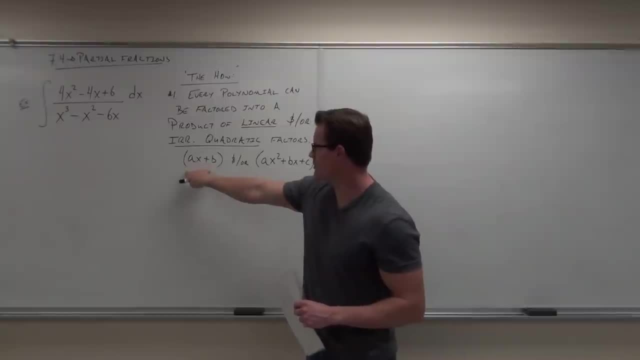 You can't do that. But we can definitely reduce them into either linear and or quadratics. This is our idea right now. Does that make sense? So when you look at this, you go, hey, look at that. I don't know if I can factor that one. Don't really care. 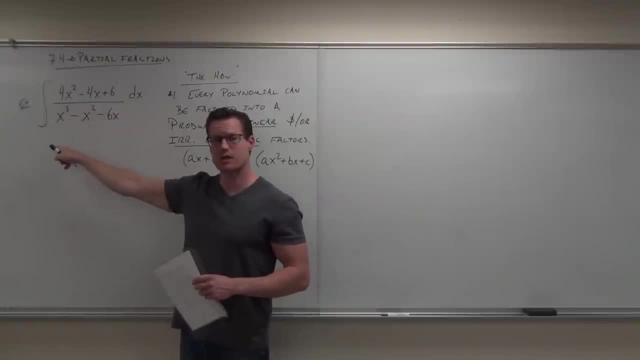 But I can definitely, definitely factor this one. It's a power 3. 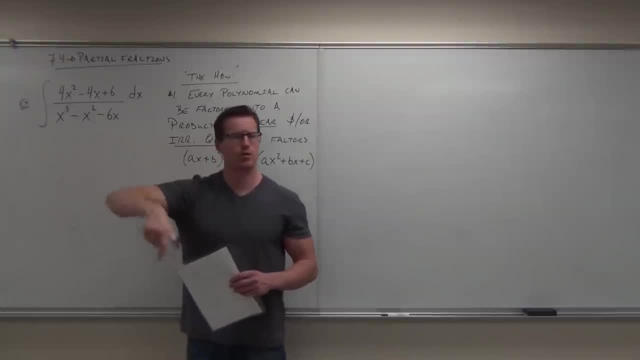 Does that make sense? I can factor that. It's going to be linear and or quadratic factors. 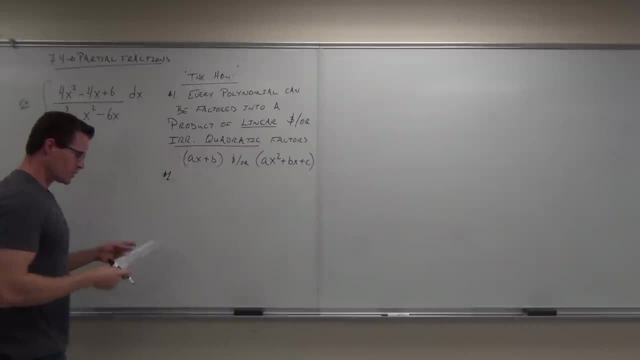 Problem number two, or sorry, rule number two. Rule number two is that every rational, every rational function. 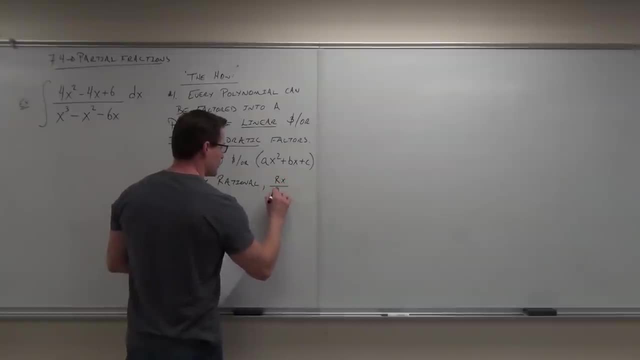 So basically where you have r of x over q of x, where r and x are both polynomials. So for every rational where the degree of r, is less than the degree of q. Can be decomposed into partial fractions. 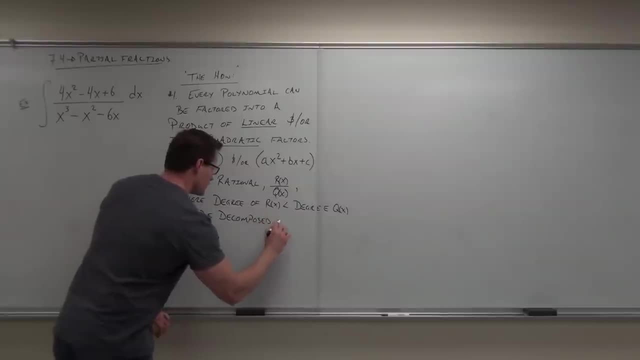 Now there's one, I know I'm giving you a lot of theory right now. And then not a lot of practice. Don't worry, we're going to get a lot of practice on this stuff. I want to give you one last little bit here. 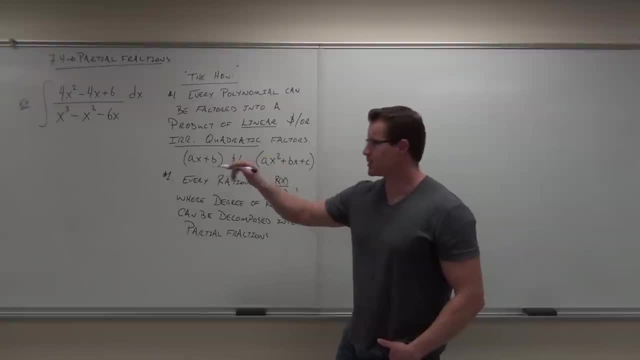 Look up here. Let's make sure that we understand a couple of these concepts. Okay. First concept. This is polynomial. This is polynomial. Hence, this is a rational. We all okay on the terminology. 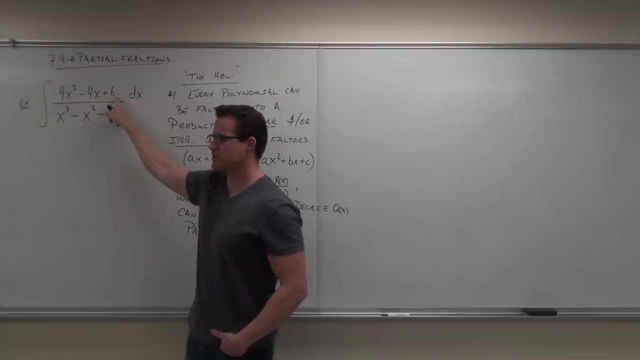 The degree of this polynomial is? Two. Two. It's the largest power. The degree of this polynomial is? 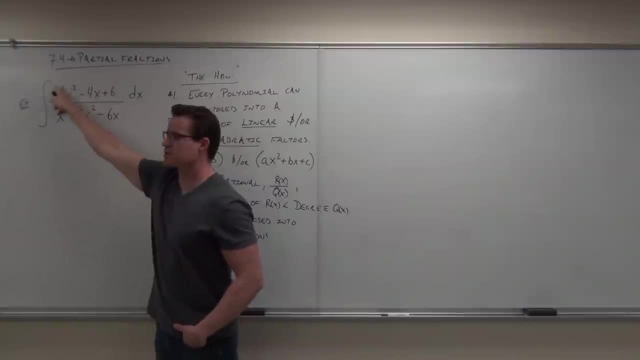 Good. If the degree of r of x, the top, the main, the numerator here. If the degree here is less than the degree here, you can decompose this into partial fractions. So far so good? 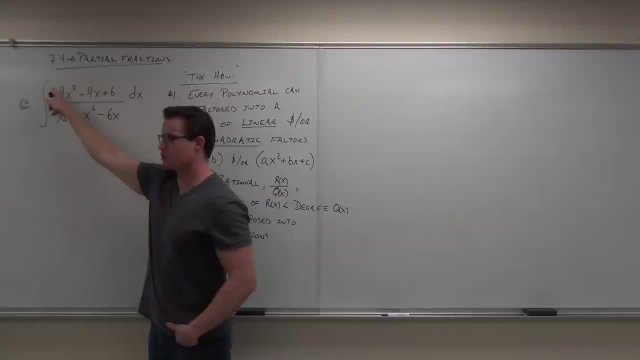 If the degree here. Is greater than or equal to the degree here. 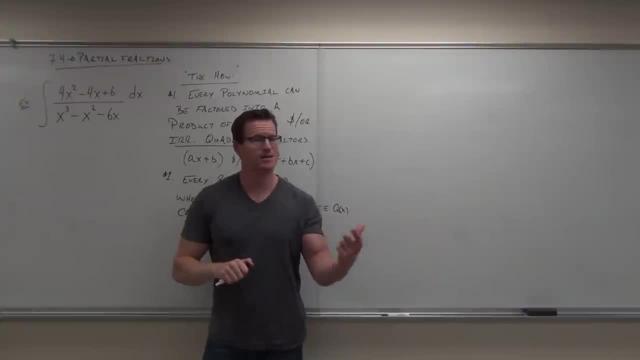 Then you do long division of polynomials first. And what that does is that reduces the degree of the numerator to something that is less than this degree. Does that make sense? 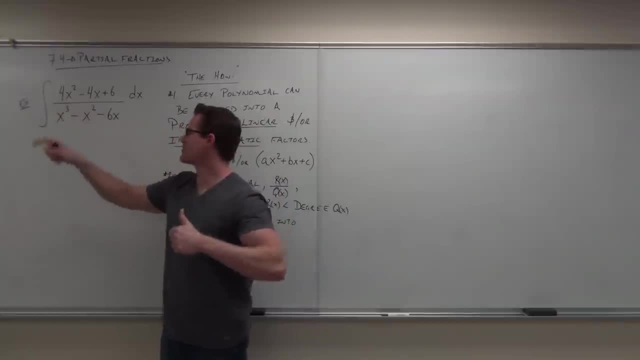 So if the degree here is less than this, you're good. If the degree here is more than or equal to this, you do long division first. 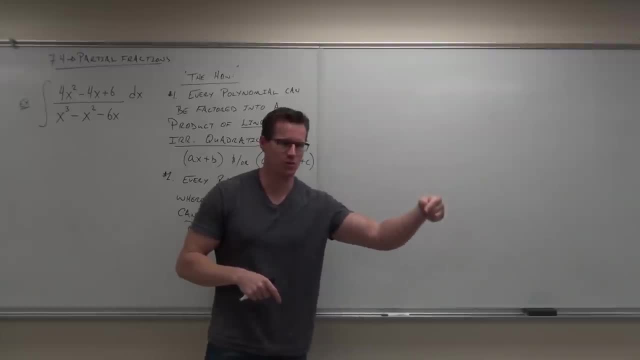 And then it reduces the degree of your numerator. And then you do partial fractions. Those problems are kind of stinky. And we'll see that in a minute. Okay. So you can see those. A little bit. So little note. No, there's not a shortcut. 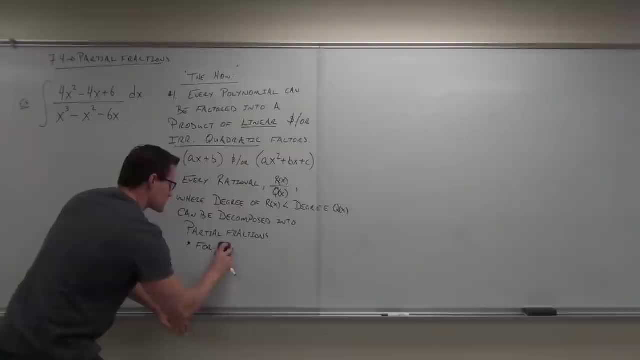 Four. Degree r of x. 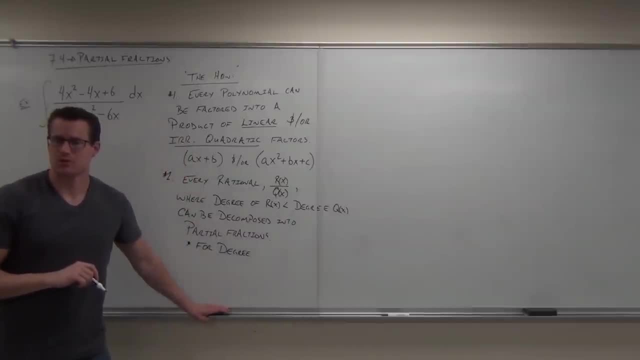 No shortcut. Not even synthetic division? Sure. If it works. If it satisfies the conditions. But that is long division. Just quicker. No. Just quicker. Okay. Thank you. 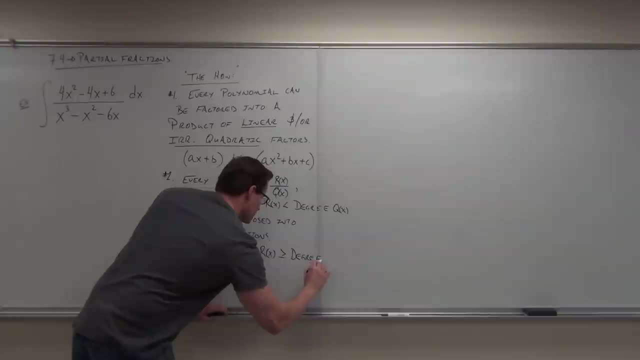 For a degree r of x greater than or equal to degree qx, do long division first. 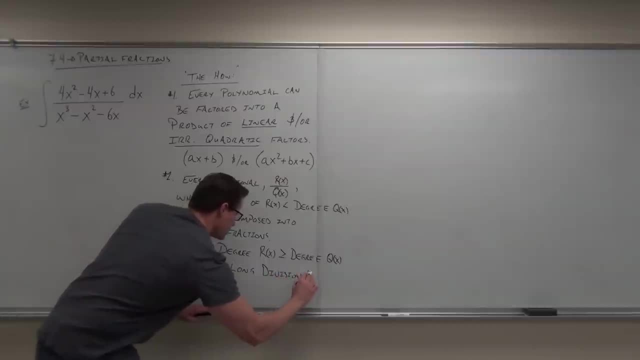 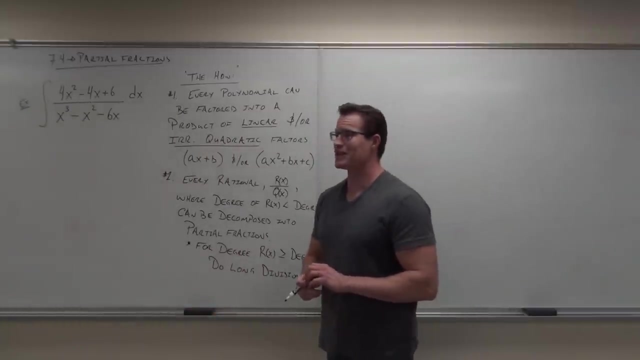 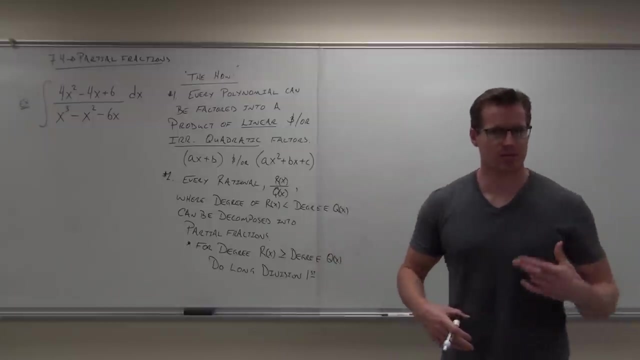 Are you ready for the next little bit? I know there's a lot of writing right now. We're going to get to this example, I promise. But are you okay with this so far? You kind of have to be. Okay. These are two theorems. They're approved in mathematics. 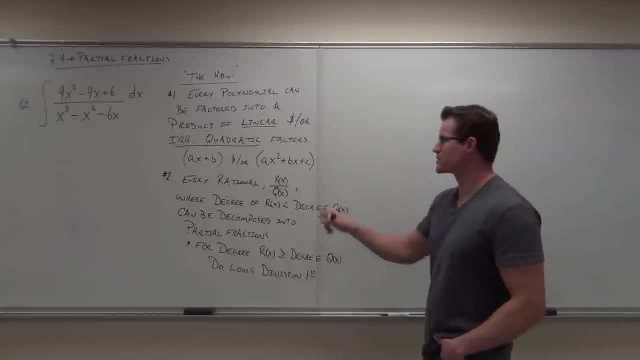 Every polynomial can be factored into a product of linear and or irreducible quadratic factors. That's these and or these. 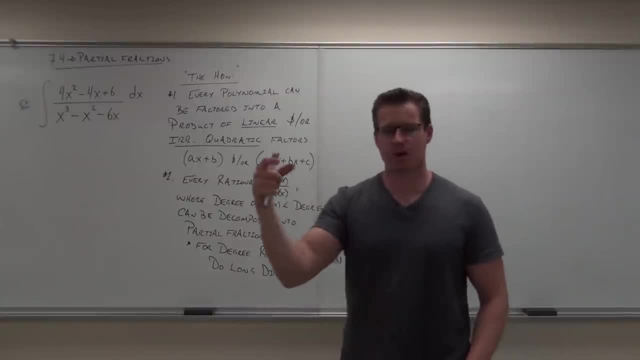 Every rational where the degree of r is less than the degree of q, the numerator is less than the degree of the denominator, you can reduce that to partial fractions. 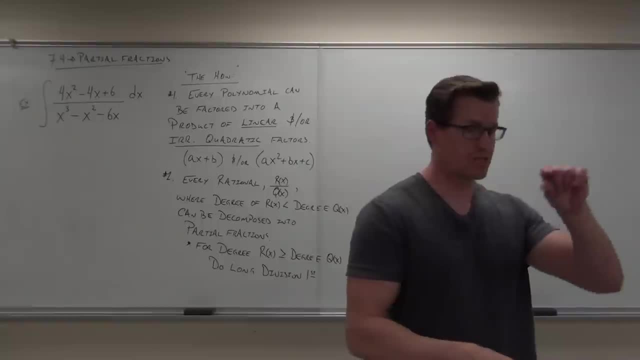 If you don't have that, you do long division, which brings your power down, your degree down. Then you do partial fractions. That's the whole deal. 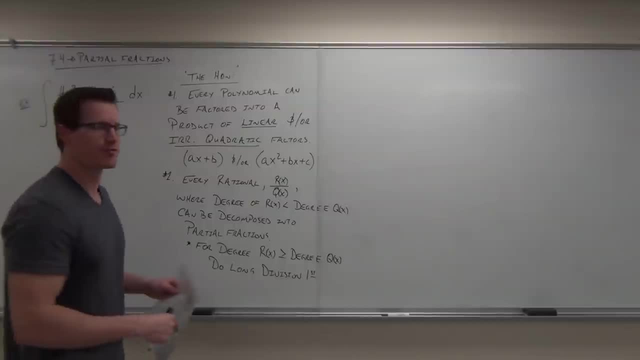 There are several cases that we're going to discover happen with these type of fractions. The first case is by far the easiest case. And we'll talk about the easiest one first. And we'll gradually make it a little bit more difficult to see what happens here. So here's case one. 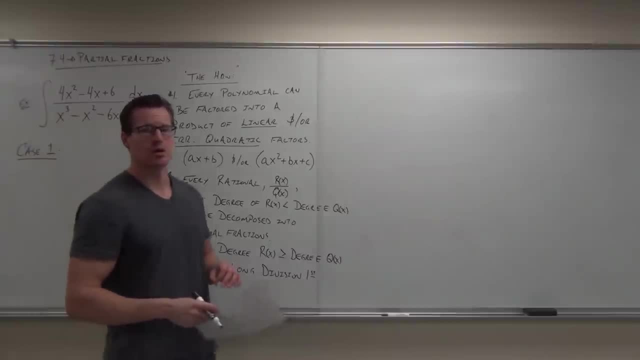 Case one. Case one is where we have distinct linear factors. 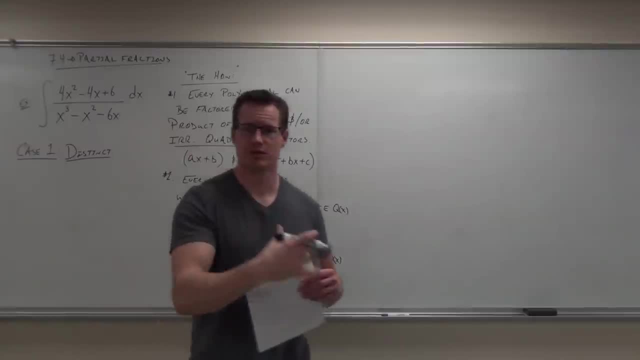 Distinct means unique. It means you don't have multiple of the same factors. Otherwise, you'd have that linear factor squared. Does that make sense? 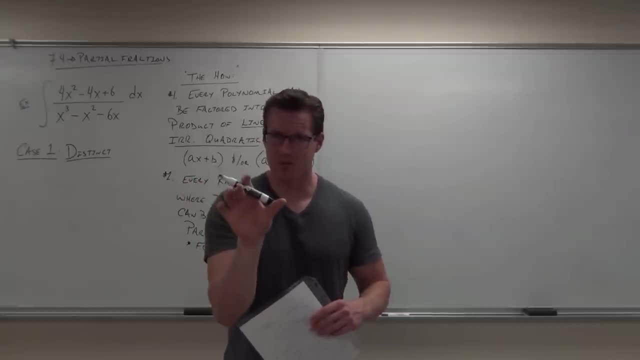 So distinct would be like you have x plus 1. X plus 1 times x minus 1 times x plus 4. What you don't get, you don't get x plus 1 times x plus 1 times x minus 4. That would be non-distinct. 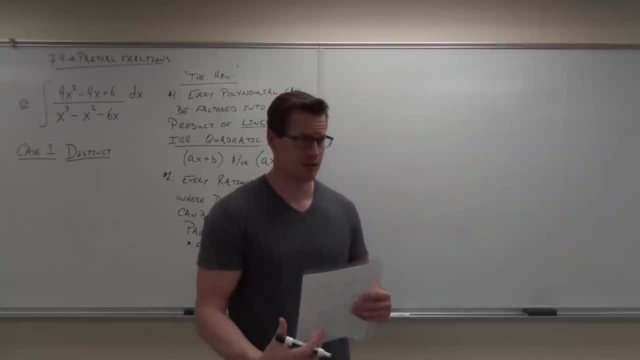 Then you'd have x plus 1 squared. We call that repeated linear factors. Are you all seeing the difference here? So distinct means it doesn't happen again. 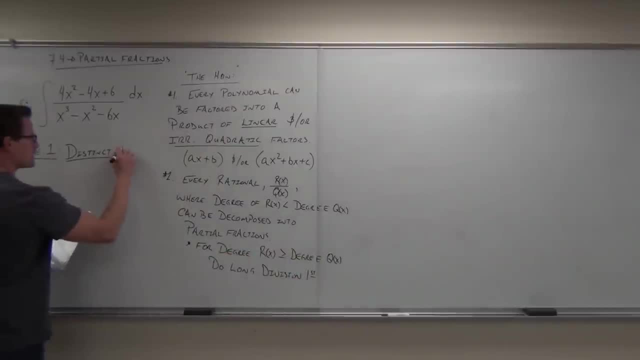 It happens one factor, and then you have a different factor. So distinct linear factors. Distinct linear factors. 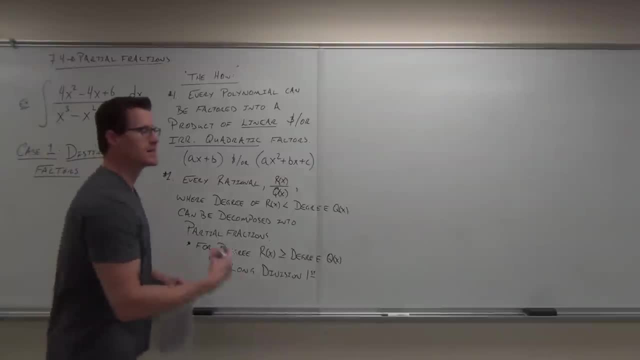 Here's what we do in that case. If we have distinct linear factors, then what we can do is we can write r of x over q of x equals, we break this up, and we write a over a x, a 1 x plus b 1. And then we have another one. B. 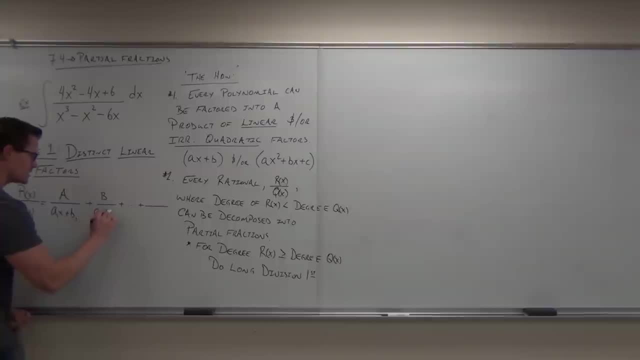 B over a 2 x plus b 2. 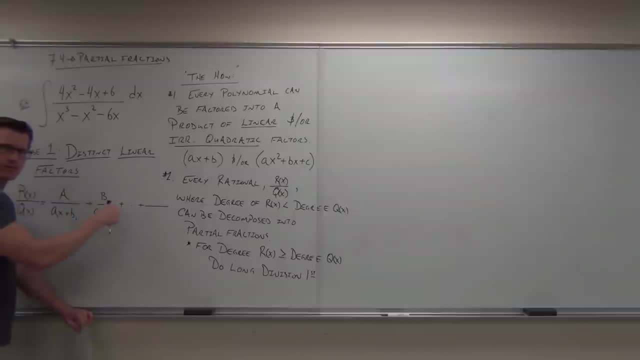 And we do this for every different linear factor that we have. Notice this is linear. Are you guys with me? It's not quadratic. It's not a power 2. This is linear. This is linear. So basically what we do is we factor our denominator. We see what factors we have. 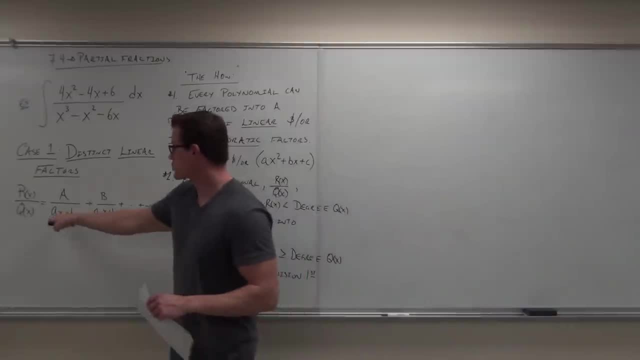 If they're all distinct linear factors, what we do is we make up a fraction for every single one of those distinct linear factors. So that's what we do. I know this might be new for you, but are you okay with the idea here? Are you sure? 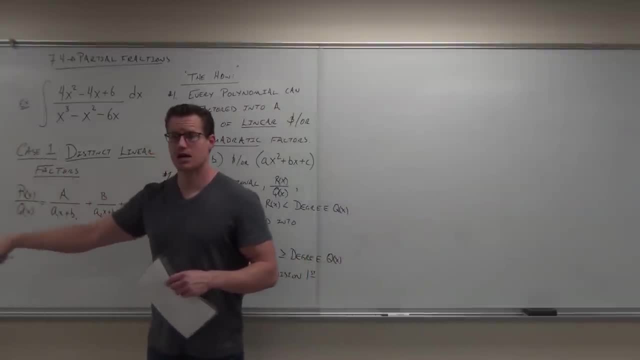 So we've got polynomial. We factor the denominator. We look at what type of factors we have. 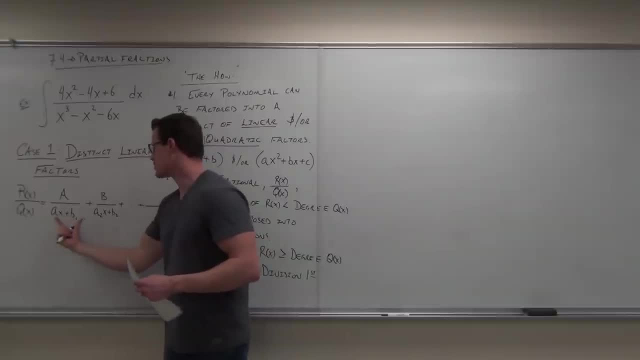 If they're all distinct linear, we write a fraction for every single one of those distinct linear factors until we get to the very last one. 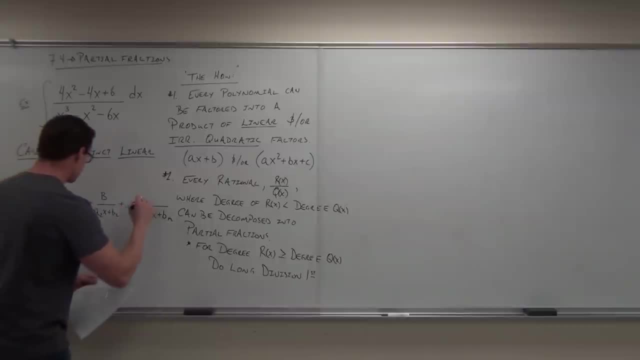 And we put whatever we have. Oh, you know what? Usually we use a and b and c and so on and so on and so on. 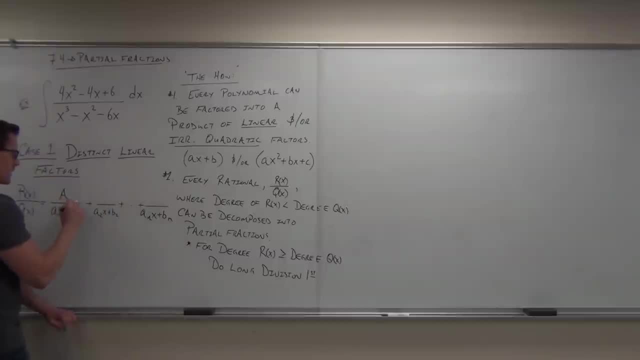 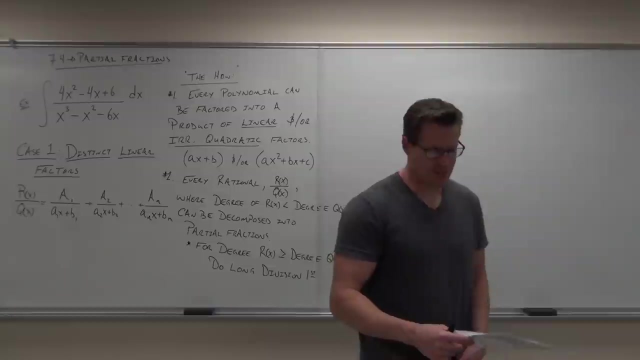 So at the very end, we sometimes, some books do this, a1 and a2 all the way to a sub n. This is just, we use a and b and c and d, but for it to make our notation a little bit nicer, we'd have the nth actual constant, where a and b and c are all constants. Do you want to see how to do it in practicality? Hopefully this will help you. Hopefully we can do this. 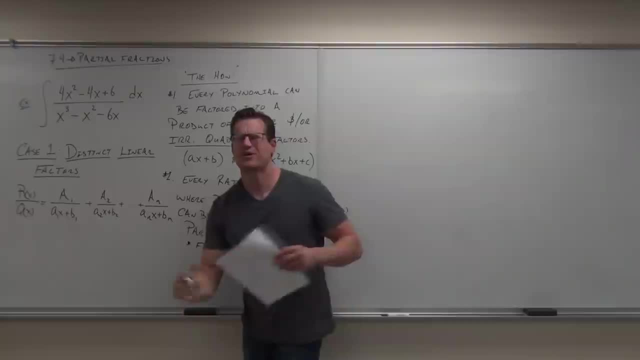 So we leave our integral alone right now. We're not even worried about it. We're not even doing any calculus right now. It's all algebra. So we're going to take the integral in here. 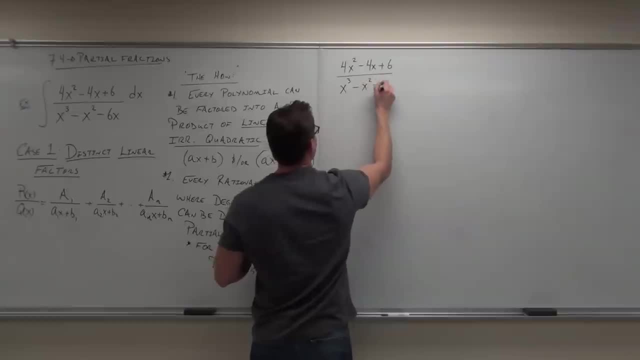 And we're going to worry about the denominator right now and see if we can factor it completely. Here's what you can and what you can't do. You can't just factor one little thing and assume you're done. 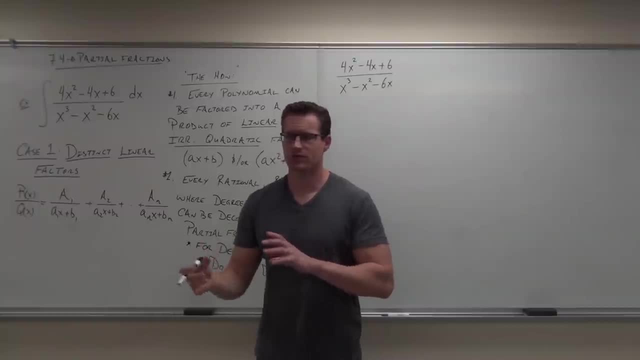 You've got to kind of show that it's completely factored. You can't just factor one little bit and go, ah, I'm pretty sure it's completely factored. You've got to know, okay? 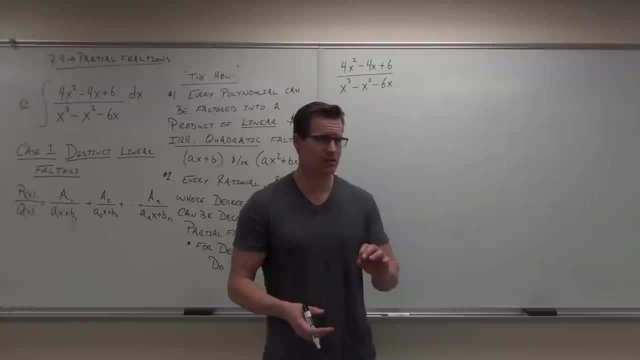 It's got to be completely factored, which means that we don't ever leave cubics, ever. We often, we sometimes leave quadratics, but you better make sure that if you have a quadratic, it's not factorable. It's irreducible. Are you still with me? Yeah. 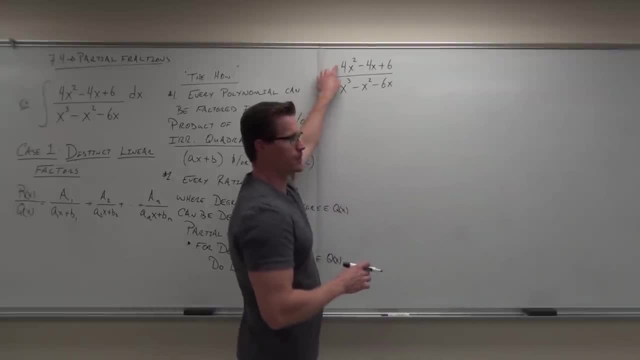 Okay, so first step, number one step, don't worry about the numerator. I don't care about that. What I care about is factoring the denominator right now. Let's factor that. How can you factor x cube minus x squared minus x? We'll take the x out. 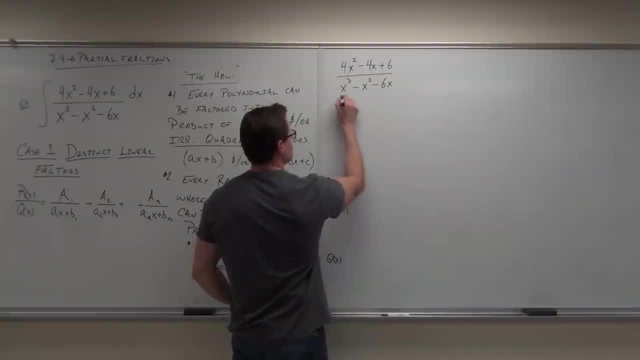 We'll take the x out. So if we do that, we're going to get x times x squared minus x minus 6. Still okay so far? Of course you are. It's basic algebra, right? 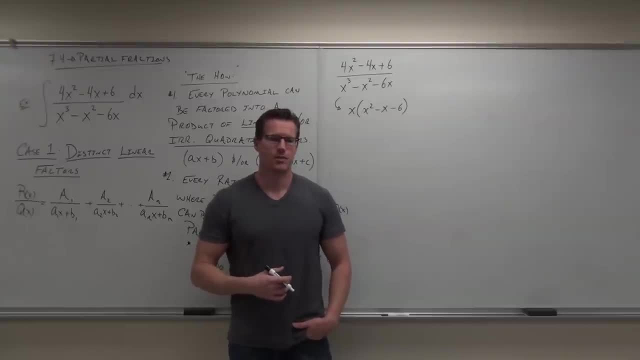 All right, now, do we stop here? You better make sure that this is not factorable if you're going to leave a quadratic. Is this factorable? Yeah. 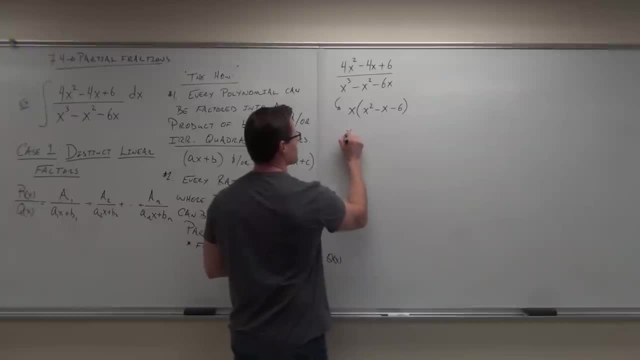 Yeah, it is. Negative 3, positive 3. Negative 2. So we have x times x, and it does not matter the order, not one bit, minus 3, x plus 2. 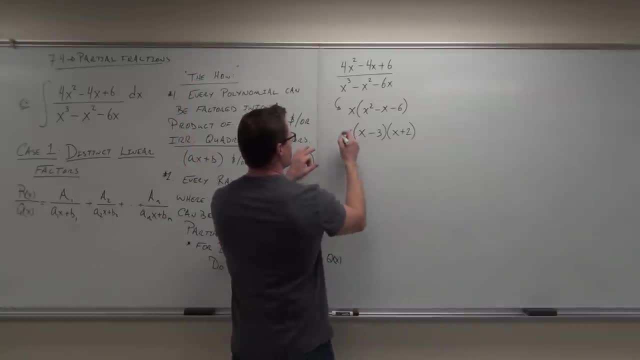 Now, here's the idea. What we know then, so bringing this down, is that we have now 4x squared minus 4x plus 6 over 4x squared minus 4x. Okay? What this is, this is the denominator. 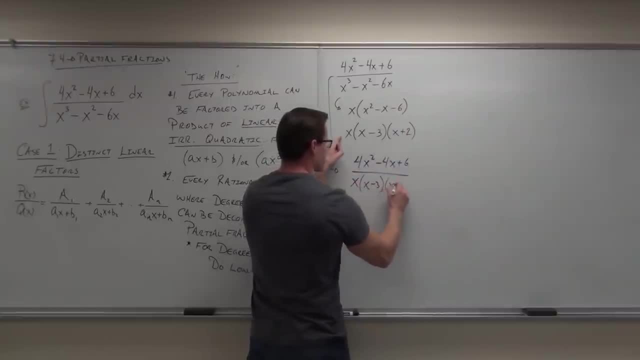 It's x times x minus 3 times x plus 2. 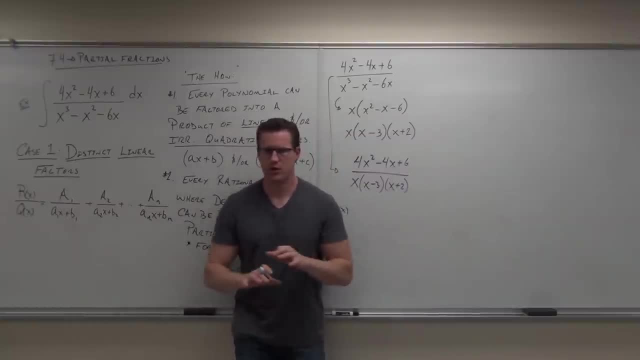 We factor the denominator completely. No saving factors until later. No just ignoring them. We factor completely. This is factored completely. Quick hit on it if you're okay with that one so far. Then you look at your factors. How many factors do we have? Three. 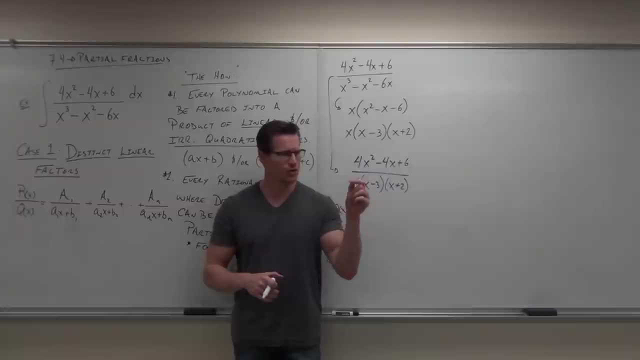 Are they all unique? Yes. If they weren't unique, you would have combined them, wouldn't you? 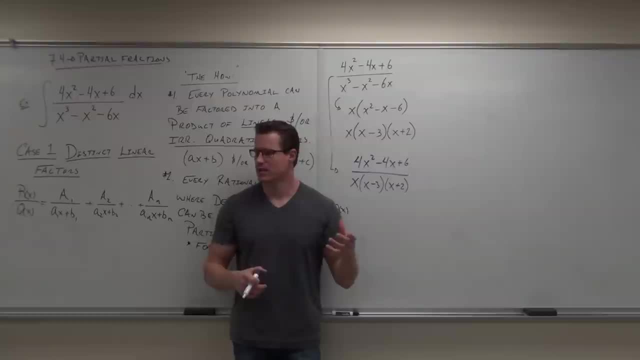 You'd have something squared or something cubed or whatever. They're all unique in this case. 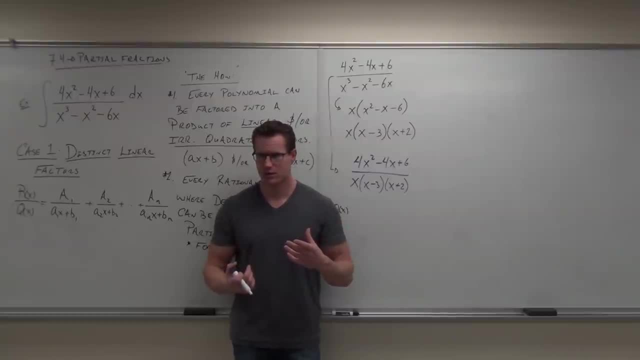 Are they all linear? Yes. Do you see any power twos there? No. So, here's what we do next. It's not a hard thing. 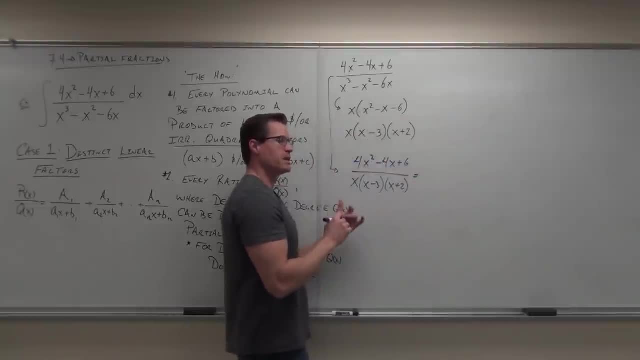 All you got to do is say what this is going to be equal to, how many factors do you have? Three. You're going to have three fractions. You're going to have x. You're going to have x minus 3. You're going to have x minus 2. We make a fraction for every. Plus 2. Sorry, plus 2. I knew something. 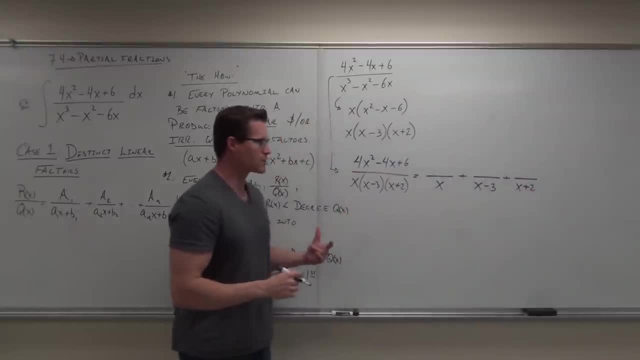 You're going to have a fraction for each distinct linear factor that you have. Show of hands if you feel okay with that so far. 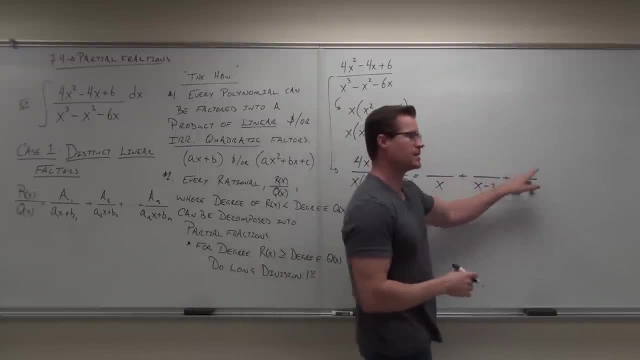 On the numerator, these are all going to be constants. This is the idea here. So, this is going to be a. We don't call this a sub 2. We just call it b to make things easy. And this is going to be c. Are we okay with that so far? Mm-hmm. 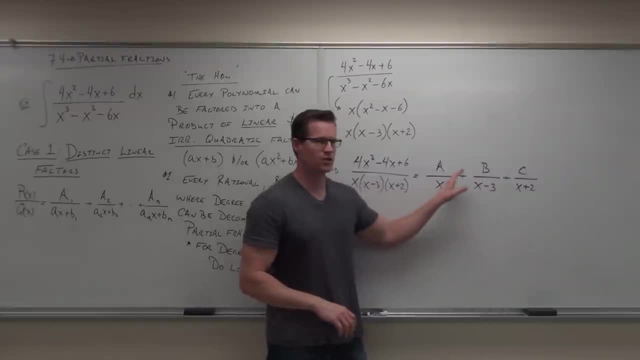 Now, the idea from here is that. If you know these things are going to be equal, if you can find a common denominator here, then our numerators would be equal. Does that make sense? If you can find a common denominator. So, that's what we work on. So, what we do is we go, okay, cool. There's an easy way to do it. 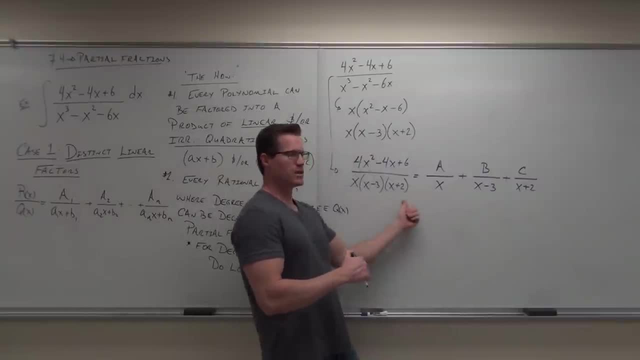 If you were to find a common denominator for this, notice that it is going to be this ultimately. That is going to be our common denominator. 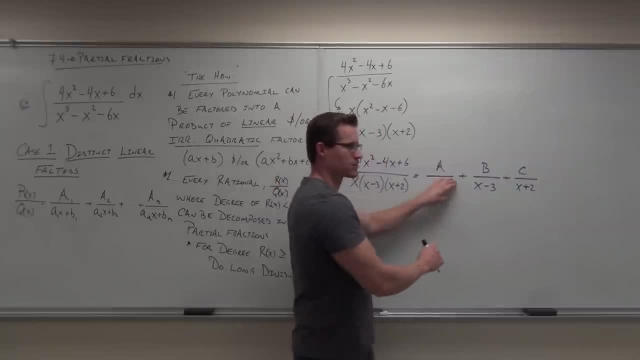 Well, this is only missing these two factors. This is only missing these two factors. This is only missing these two factors. I call this the cover-up method. It's kind of nice. All you got to do is go, okay, well, cool. Cover up the denominator. And just write the other two linear factors. 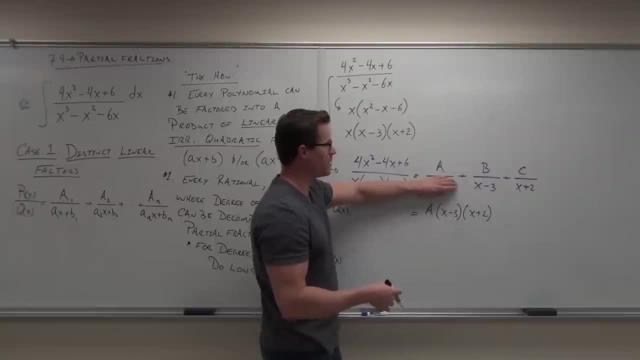 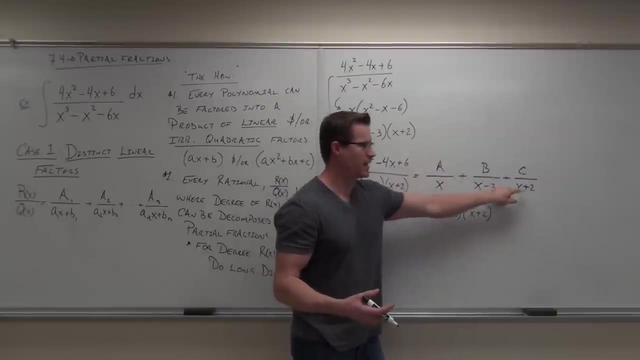 So, if I were to find that common denominator, I'm going to cover this up. Then we have to multiply. In order to find the common denominator, we'd be multiplying this fraction by x minus 3 over x minus 3 and x plus 2 over x plus 2. Does that make sense to you? We're not writing the denominator because of this. 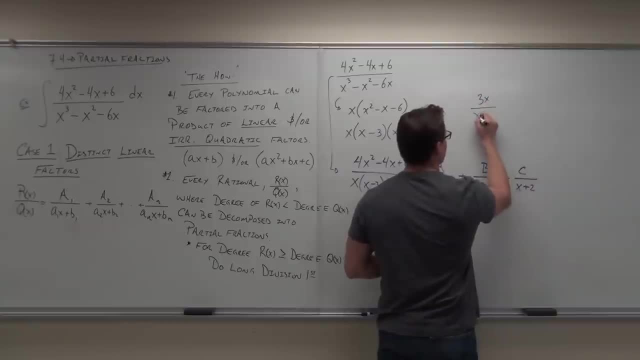 If I ever get, like, 3x over x minus 1 equals 5 plus 1, 5 plus x over x minus 1. If I ever get that, I know that these things are going to be equal if 3x equals 5 plus x. Does that make sense to you? 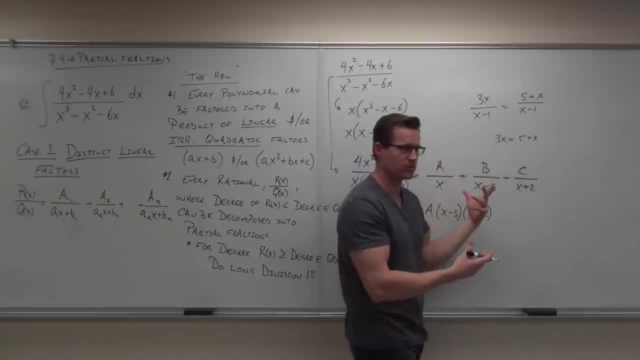 Of course, we'd have a domain issue with 1, but that's what we. We ultimately solve this problem. So, it's going to be okay with that. 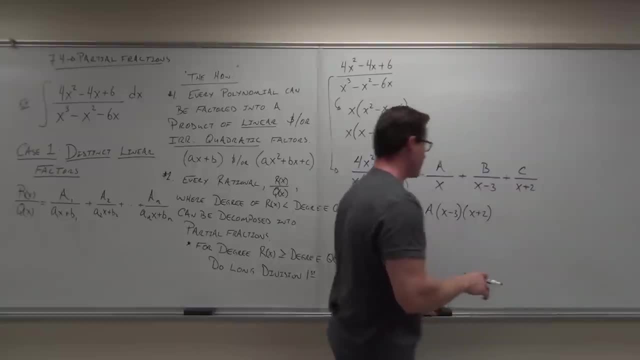 So, I'm not writing the denominators here because I know that if I get this common denominator, denominators are gone anyway. So, I've got a times x minus 3 and then x plus 2. Plus, let's see if you can do the b. 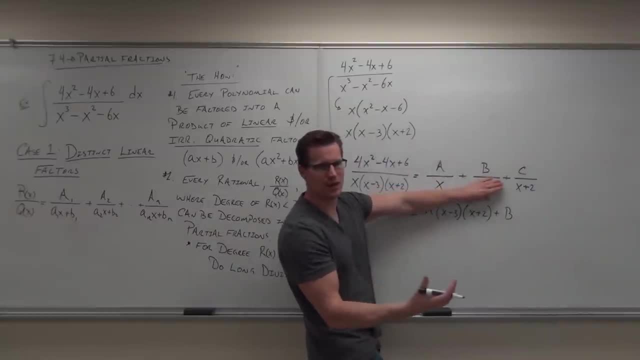 b times x. x, cool, because I'm going to cover this up. I don't need another x minus 3. I've already got that factor there for my common denominator. I am going to, however, have an x and x plus 2. Still okay? Let's do the c. 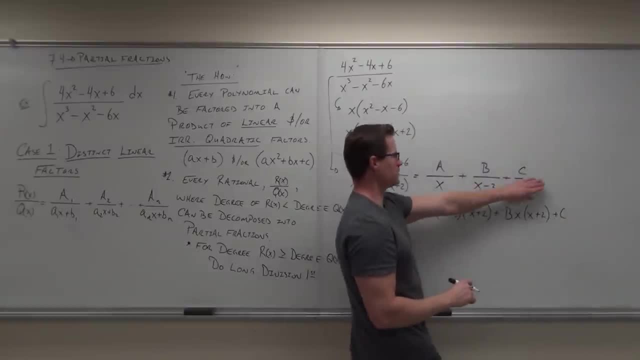 What's going to be there? What's going to be there for the c? x minus 3 plus 2. 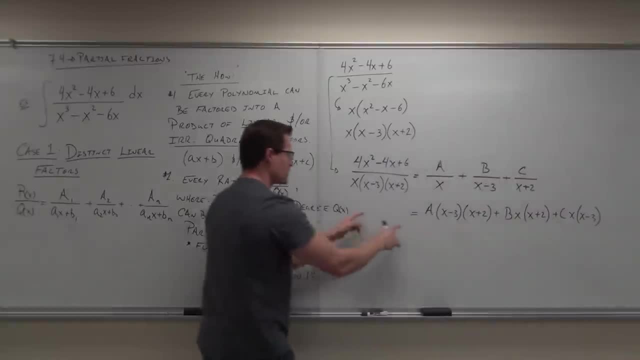 Okay, now check it out. What's this whole thing going to be equal to? x, x minus 3x plus 2. What? It's going to be equal to whatever this denominator is. 4. Why is that? 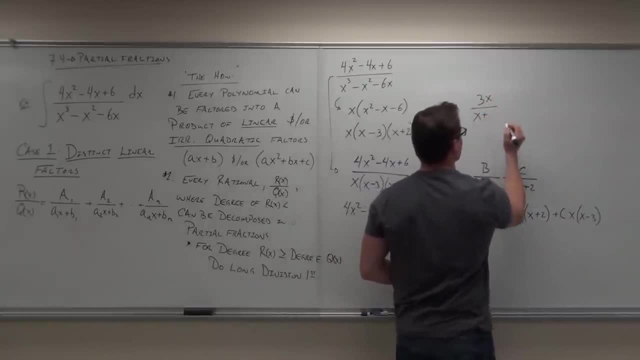 If I have 3x over x plus 1. Or x minus 1, or whatever I gave you before. It doesn't really matter. 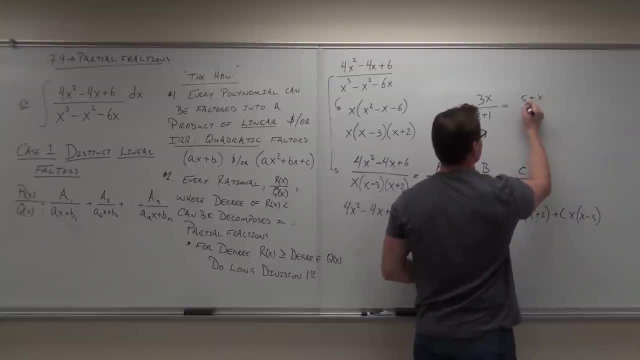 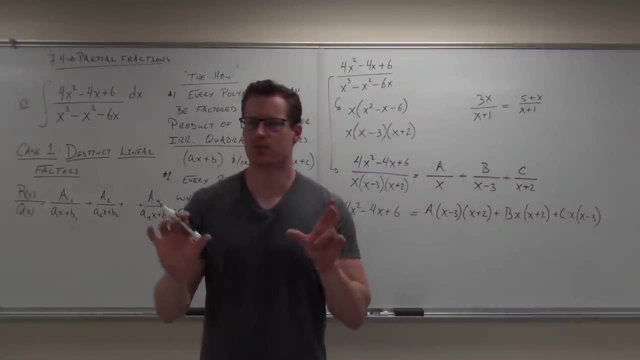 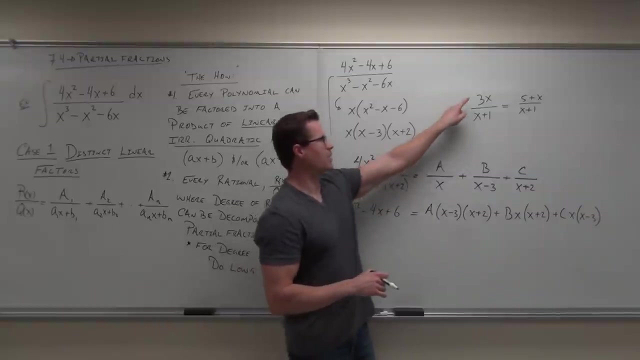 And I say that this is equal to 5 plus x over x plus 1. Whenever your denominators are the same, you can solve that problem by setting your numerators equal. You can even do that with a proportion. Cross multiply, you'll see that the x plus 1s are gone. Does that make sense to you? So, I have, I would have numerator equal to numerator if these guys are the same. The idea here is that what you're trying to get is a common denominator. You can do this the long way, you really could. But you know what you'd get? 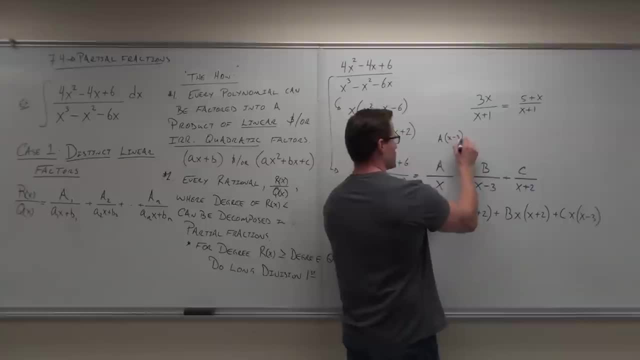 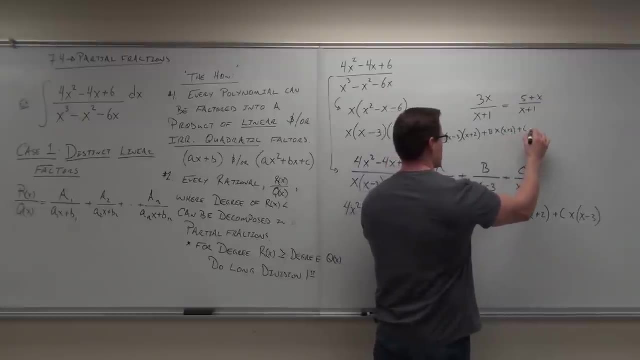 You would get a, x minus 3, x plus 2, plus b, x, x plus 2, plus c, x, x minus 3. You know what this is going to be over? It's going to be over x, x minus 3, x plus 2. 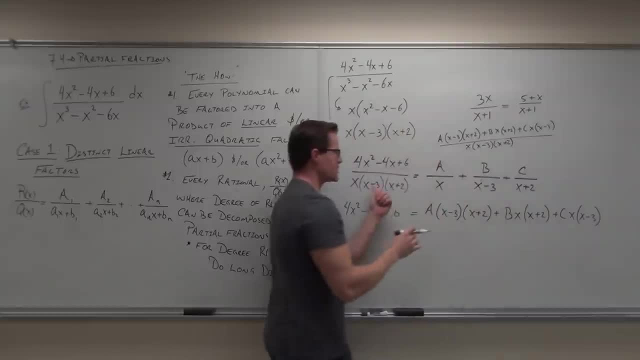 So, basically, this thing equals this thing. Do you see how the denominators are the same here? That means the numerator. The denominator gets set equal to each other. 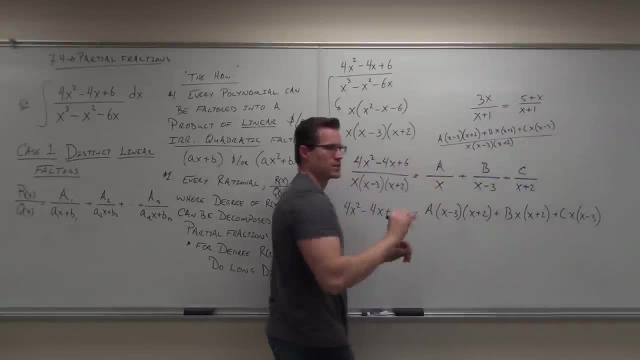 This will be equal to this because your denominators are exactly the same. Does that make sense? 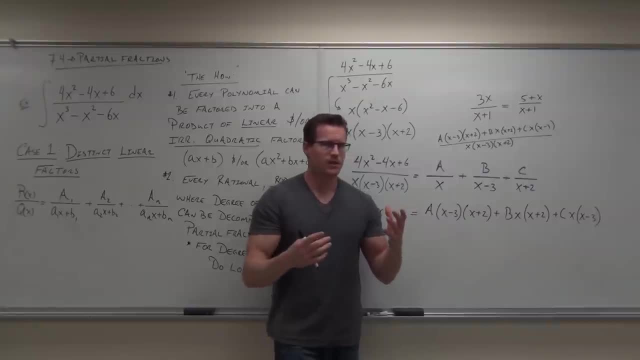 It is a, it's a cross product, that's right. It's a, it's a, it's ultimately just a proportion that you're creating. 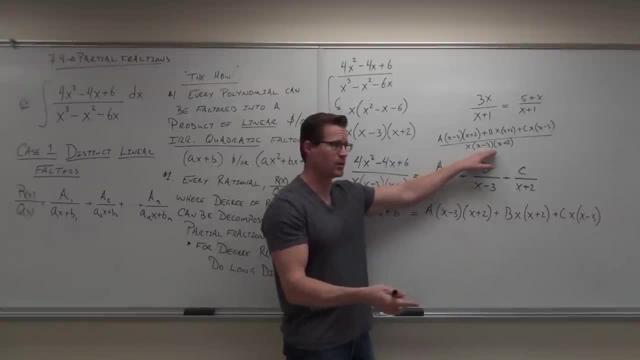 We are ignoring this step because we know it's going to happen. We know that your denominator, if you create a common denominator, your denominators are going to be the same. Look, you're keeping the exact same factors, aren't you? Therefore, your common denominator here isn't the same. And you're going to need to look at this. You're going to need to look at this. And you're going to need to look at this. You're going to need to look at this. 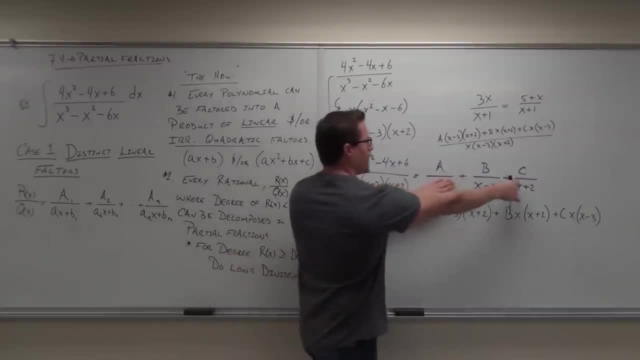 This is this thing. If we just multiply by the missing factors, we inherently create a common denominator that we can ignore because it's going to be the same on both sides. Question? 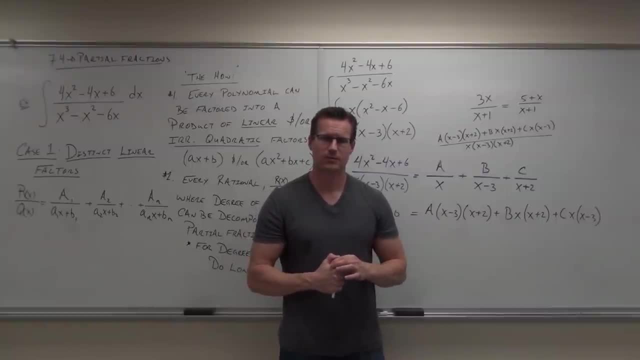 Are we going to have to worry about, for the denominator, like x nine equals zero or three or negative two later on? 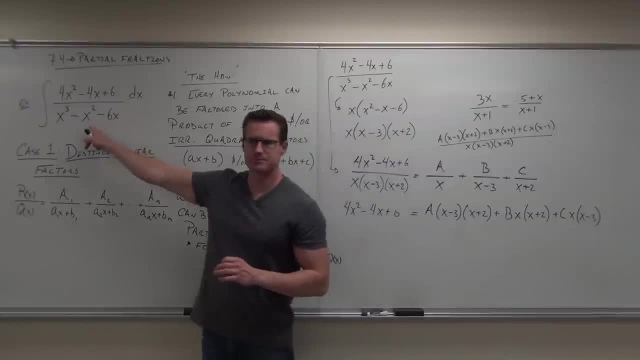 Yes. But that's the same thing that we would have worried about here, right? That, that's in your domain. So, yes. 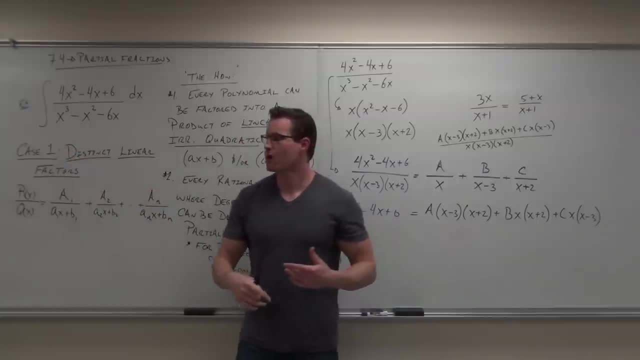 We don't create any, I'll say it this way. We don't create any additional problems with this one. Does that make sense to you? 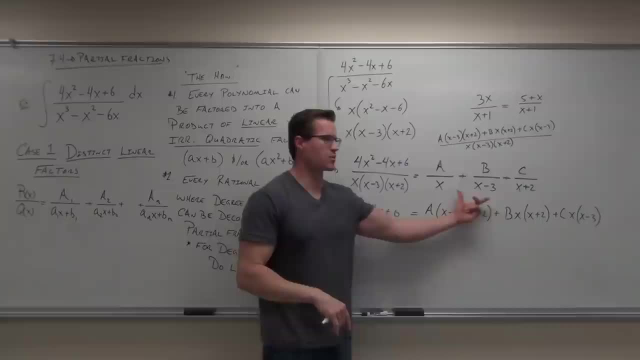 Because this already has those problems in it. And when you factor it, you just see the problems. So, yeah, we have to worry about it, for sure. 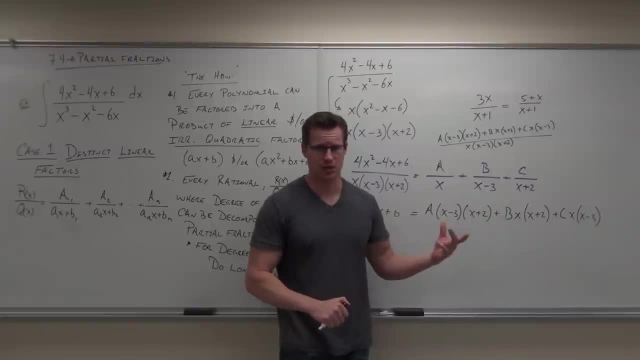 If we have those, we're going to have what's called improper integrals. That's the next section we're going to cover, okay? So we get there ultimately. 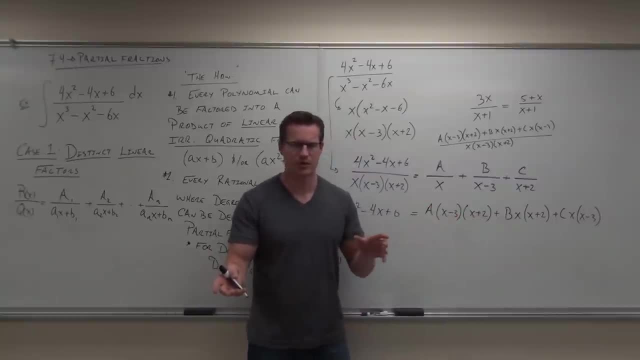 But right now, we're ignoring that a little bit. I'll be honest with you. We're ignoring it. 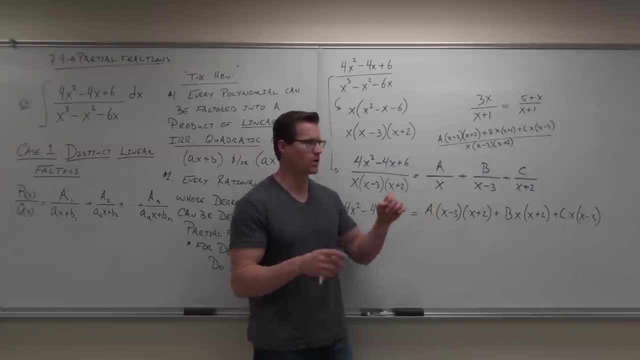 We will talk about that in the next section, improper integrals, where we go, wait a minute. What would happen if we integrate from, let's see, zero to three? 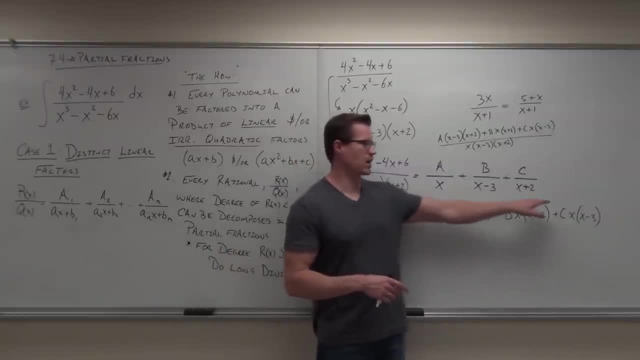 Well, we'd have a problem at zero. We'd have a problem at three. Won't care about the negative two. It's not going to show up. But we'd have a problem with those things. We will deal with that. 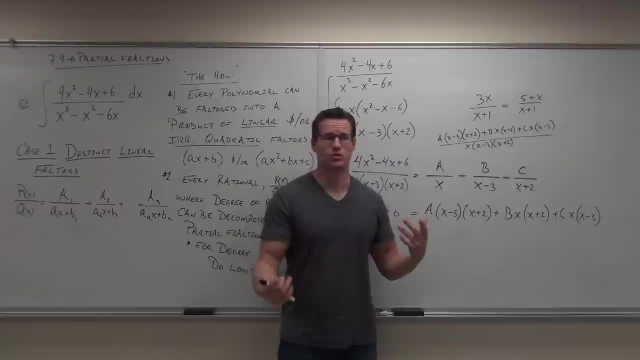 But for right now, I want you to see that we're not creating any additional issues. Do you see that? These are the same, right? Same domain issues. 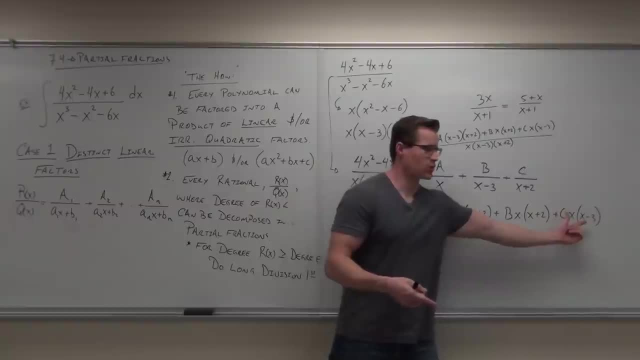 Do you understand the concept of when I do this, I create a common denominator. And when I do a common denominator, I have my numerators set equal to each other. 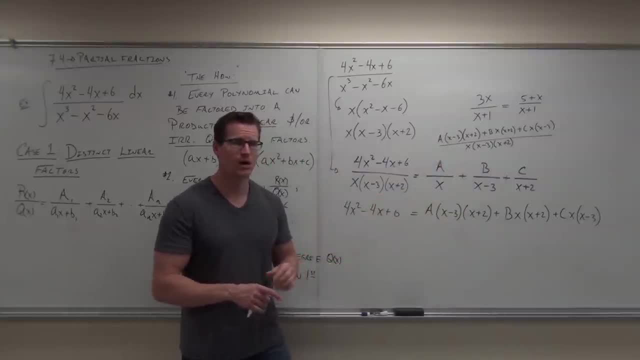 Do you get that idea? Okay. We're going to stop right there for right now. We'll continue right here next time. Well, we're going to continue. 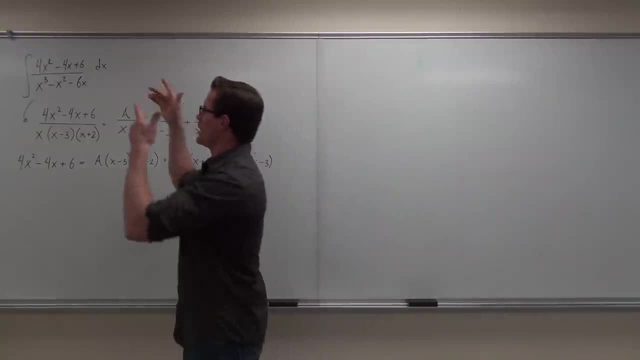 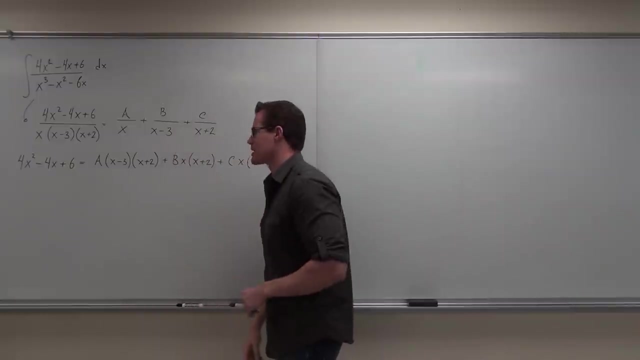 So where we left off last time was how in the world do we do an integral like that where a substitution won't work, where it is a polynomial over polynomial, hence it's rational, and where the degree of our numerator is less than, strictly less than the degree of our denominator, where it's not. I'll show you what to do in the next, probably the next couple examples here. 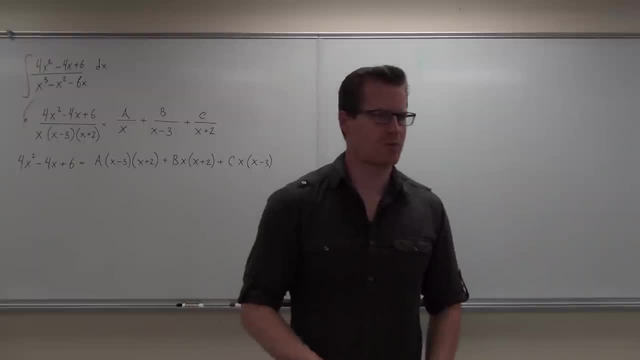 So if this is the case, what we know by some algebra theorems is that we can reduce any fraction such as this into partial fractions. 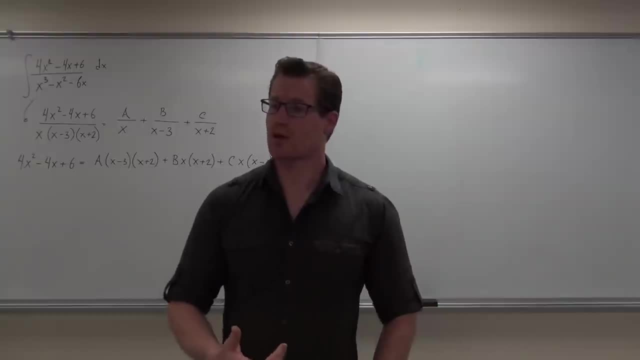 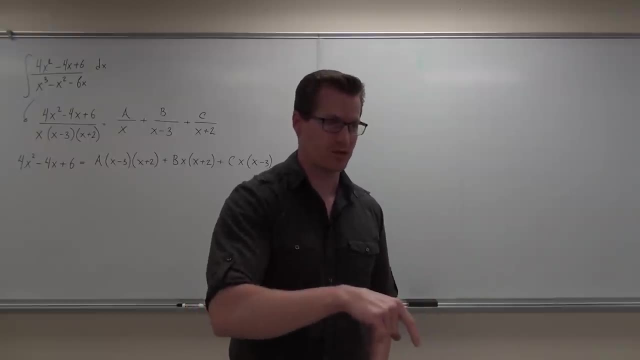 Partial fractions work in a case-by-case basis. We're either going to have all linear factors, or we're going to have linear and irreducible quadratics, or we might have repeated linear factors, or repeated quadratic factors. 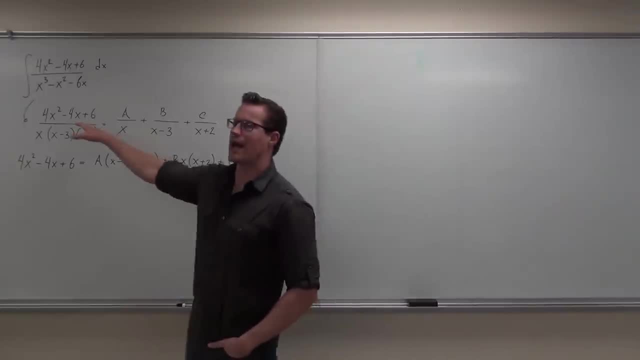 That's the idea with this. Now, in our case, when we factor, which you have to do, by the way, you've got to know that any polynomial can be a polynomial. 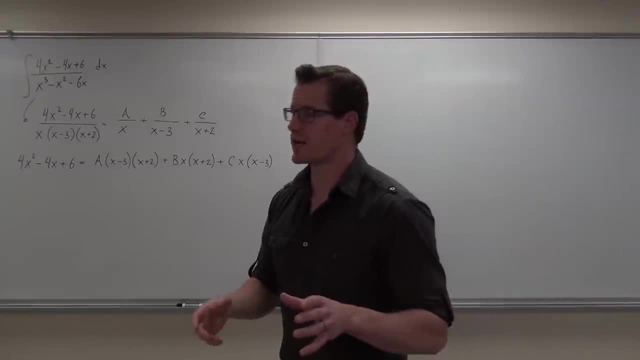 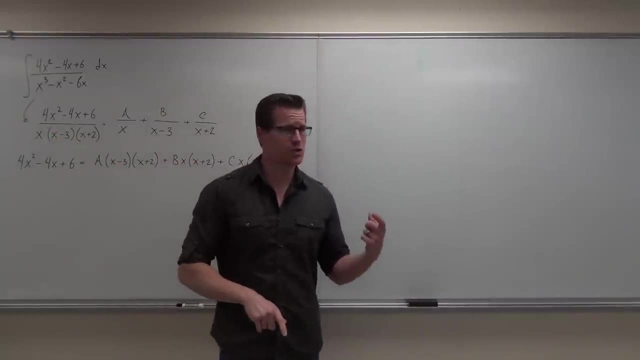 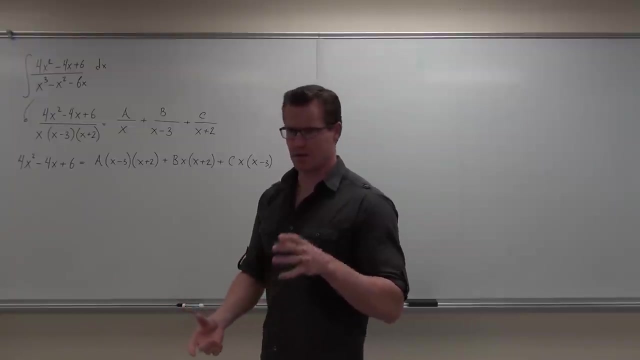 It's going to be decomposed into linear and or irreducible quadratics. So you'll never end with a power 3. It'll be either power 1, like here, here, here, or power 2s that you can't reduce, like x squared plus 4. You can't factor that, so we'd be stuck with it. That would be an irreducible quadratic. Are you guys with me? 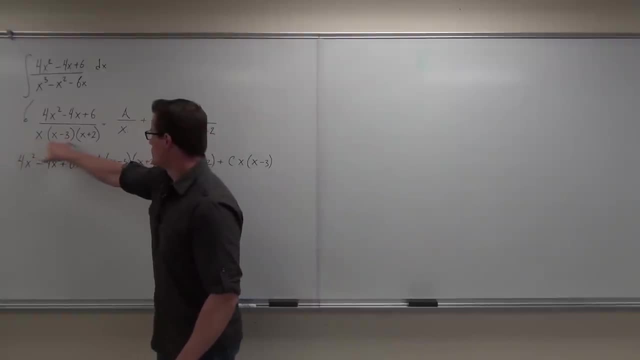 Okay, so in our case, we have 1, 2, 3 linear factors. What that means is we're going to create three fractions, one for each of our linear factors. 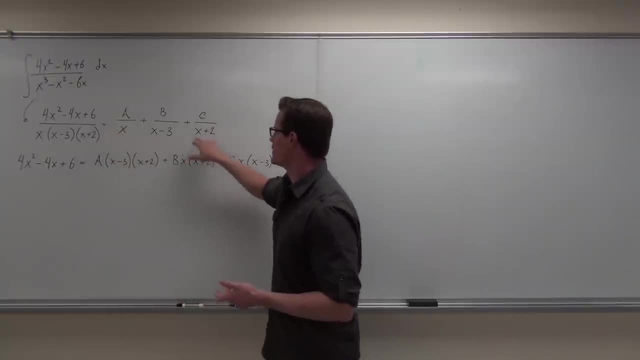 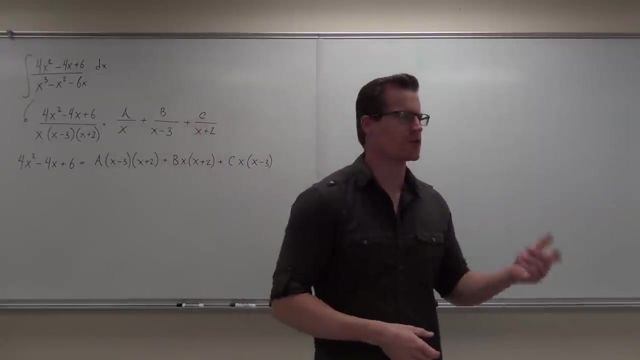 The way we do it, we just write, each of those linear factors on a denominator, and constants, a, b, c, and so on, and so on, and so on, until you exhaust all of your linear factors. So far, so good? 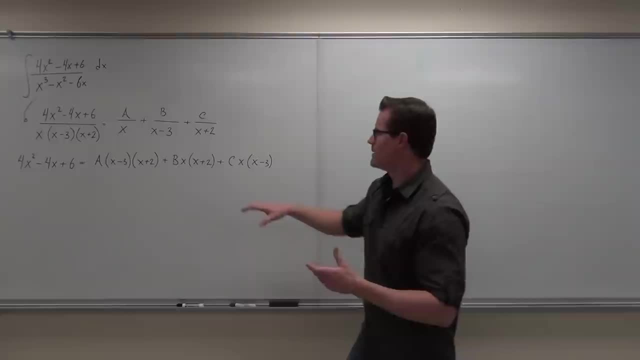 After that, we basically find a common denominator. We want to make this kind of the same denominator as this, and I explained this hopefully very well last time. 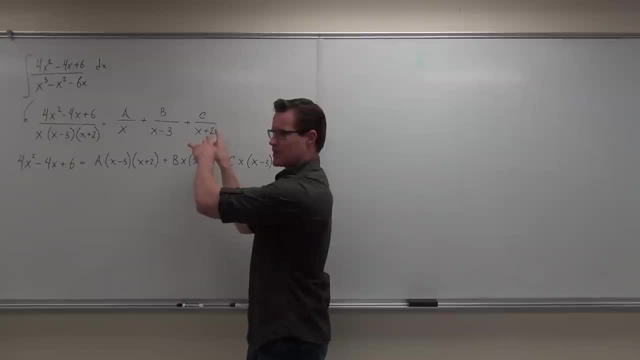 If you do that, the numerators themselves will be equal. Does that make sense? 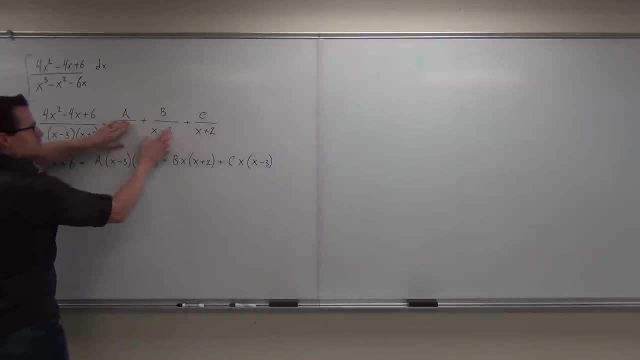 So we would multiply this fraction by these two factors, since they're missing, that's why we get a, and then x minus 3, x plus 2. 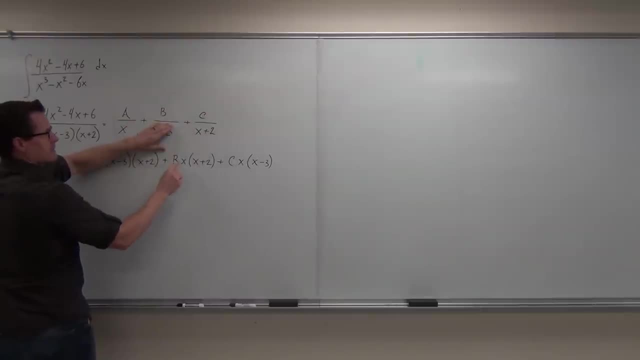 We multiply this fraction by these two factors, and so we get an x and an x plus 2. This fraction by these two factors, x, x minus 3, this is the numerator of this, this is the numerator of this, and now, because we have a common denominator, those two things are equal. Show of hands if you feel okay with this so far. 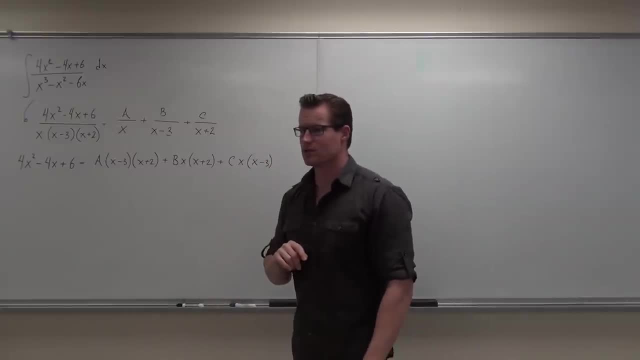 All right, now we get to continue, and what in the world are we going to do with this? Well, we're going to have to. We're going to have to destroy. 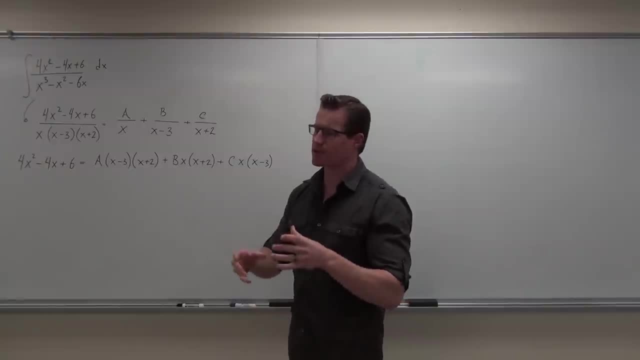 We're going to have to distribute all this stuff and organize our variables. So if we do that, I'm going to move quickly because this is, of course, well, just some distribution. So here we go. 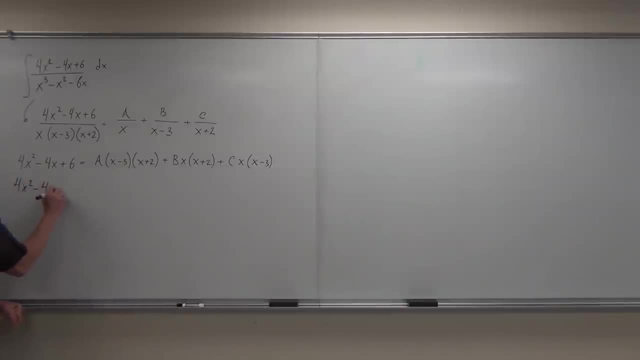 We'll have our 4x squared minus 4x plus 6. We get ax squared. We get, let's see, plus 2x minus 3x minus ax minus 6. I want to make sure that I'm right, so can you please double-check these as I'm going through, just to make sure I got this stuff right too, okay? Here we'll have plus bx squared plus 2bx plus cx squared minus 3cx. 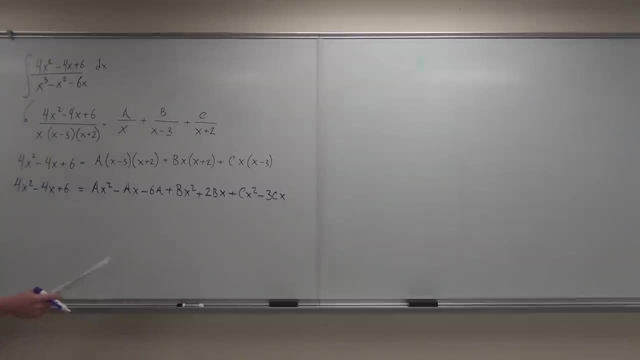 I'd like to double-check if you got that same thing. I'm going to double-check my work too. Did you get the same thing I got? 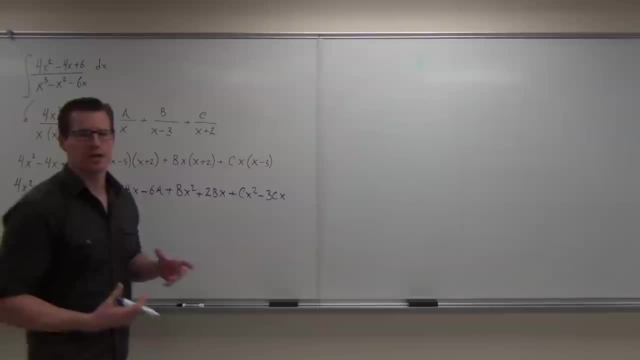 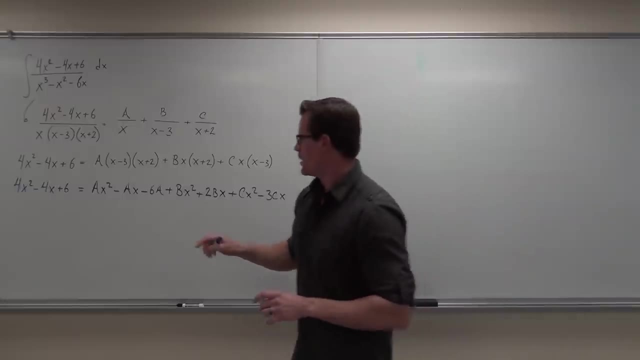 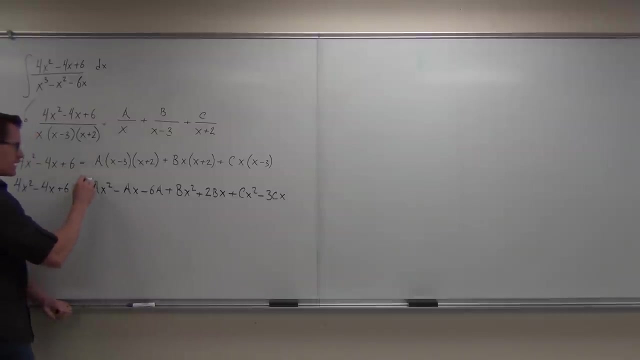 Okay, now, organize them. What we're trying to do here is we're trying to match up x squares and x's and constants. So, for instance, what I want to do is I want to look at this x squared and I want to look at these x squared, but right now it's a little bit confusing as to what's going on. So we're going to factor this out, so check it. We're going to have, do you see the like terms I'm talking about? We have a x squared. 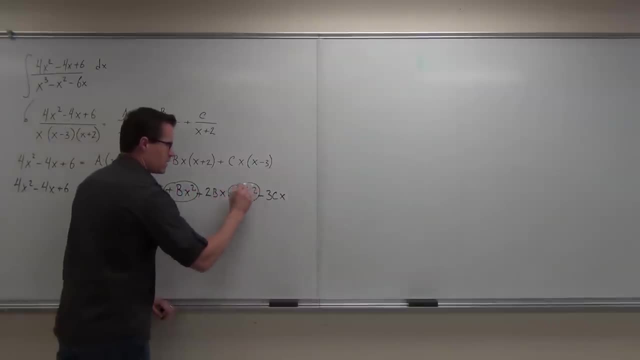 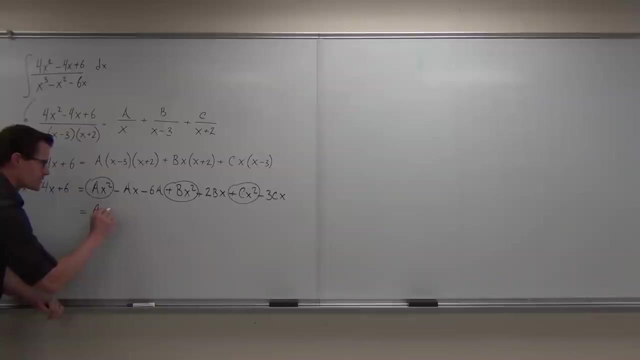 We have bx squared, bx squared, cx squared. If we factor out the x squared, then what this gives us is a plus b plus cx squared. Do you understand the idea? Hello, yes, no? Yes. 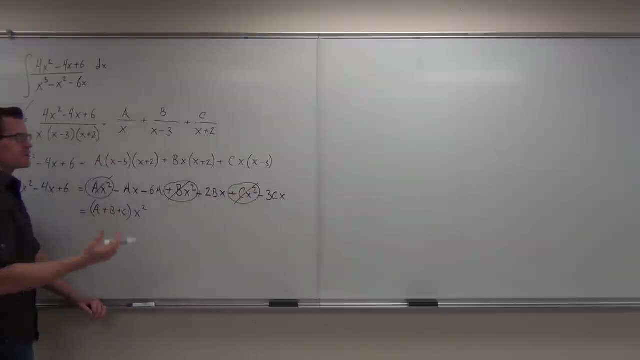 Okay, so these we've taken care of. Our x squareds are gone. Then we look for any of our x's. 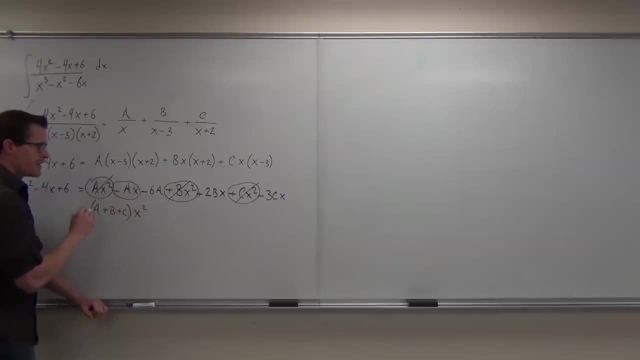 I see a negative ax, a positive 2bx. 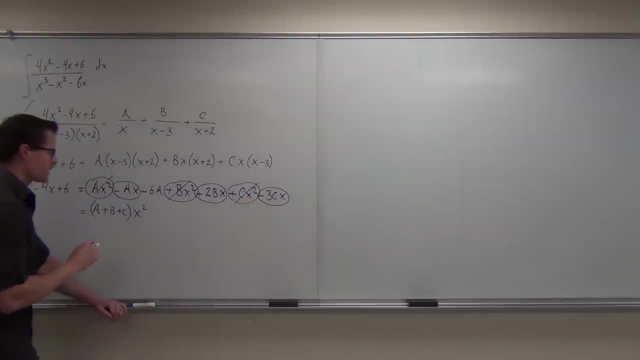 Okay? A negative 3cx. 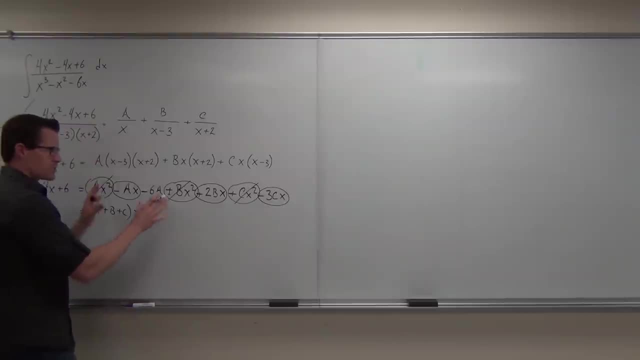 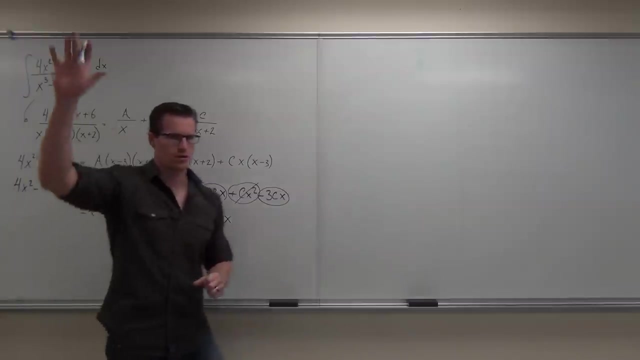 So we will have, I always do a plus here. We're just going to factor these numbers out. The coefficients are our numbers. So we'd have negative a, we'd have plus 2b, we'd have minus 3cx. So we're looking at this, we're factoring out x, x, x. Then we have a negative a plus 2b minus 3c. So if you guys feel okay with that one. Okay. Cool. 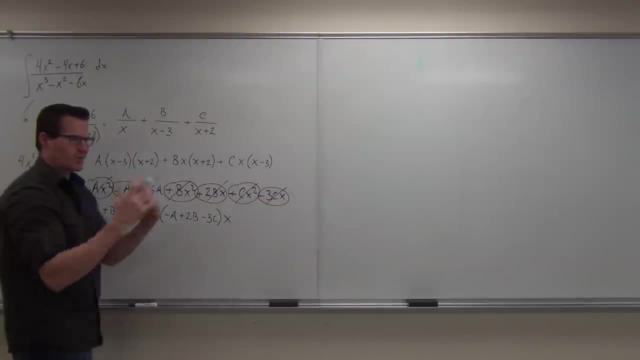 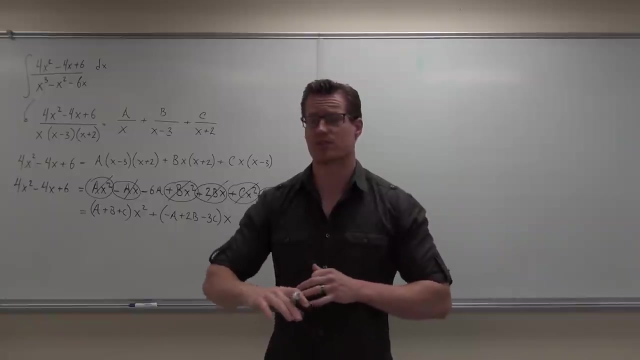 So those are now gone. I always circle them too. That way I don't get lost in what I'm doing. I definitely don't want to get lost, and you can't miss a negative here. Or you can't screw up the coefficient. If you do that, your problem is smoked. All right? You're done. So we've got to be really careful with our algebra. Lastly, well, this is it. Now this is what's kind of nice about this. Check it out. 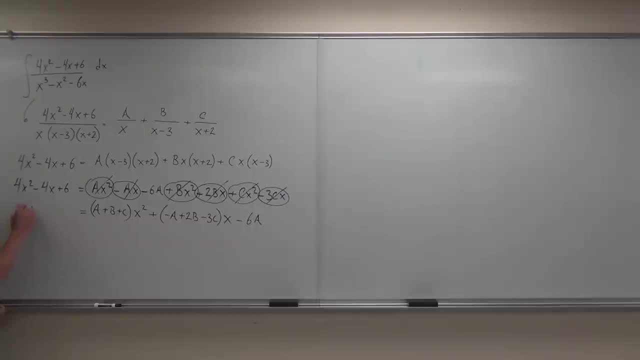 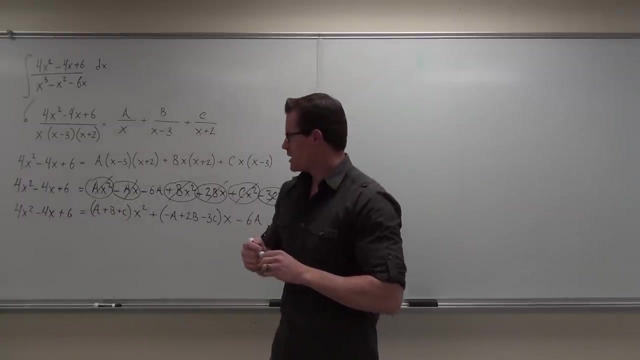 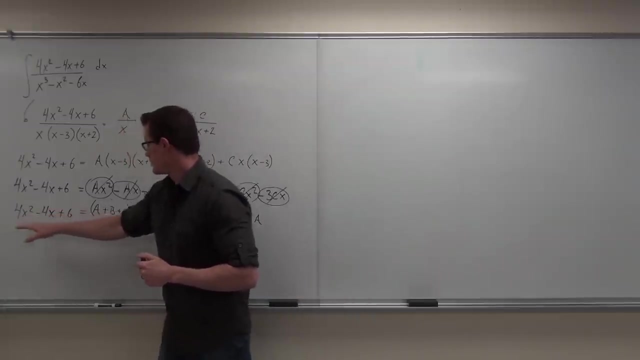 What we know is that 4x squared. Minus 4x plus 6 equals this thing, don't we? Well, look, if we know, let me have your eyes up here, this is kind of important. If we know that 4x squared, here's our x squared, right? Our x squared coefficients have to equal. 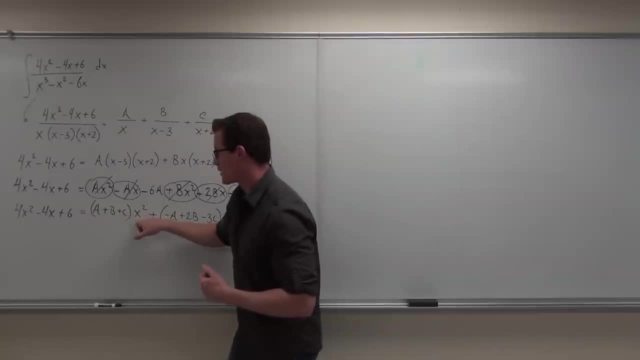 So if we have 4x squared and we have a plus b plus cx squared, then what we know is this coefficient must equal this coefficient. It has to equal that. 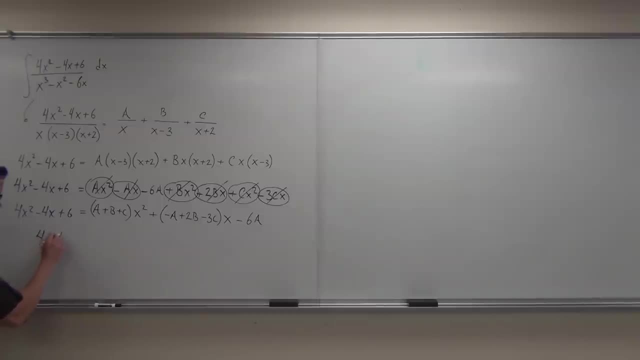 So we know that. Okay. If 4 equals a plus b plus c, that has to be the case. 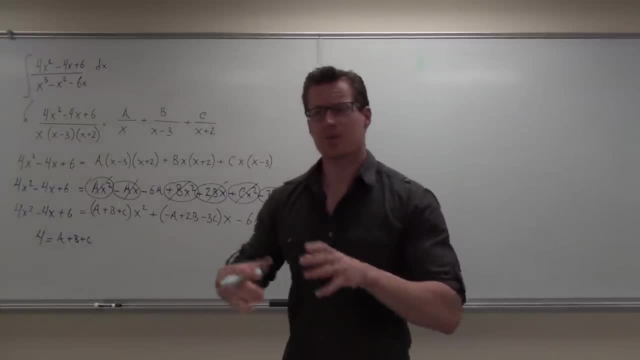 That's why we organize our x squareds and our x's and our constants so that we can make this jump. So we go, hey, here's an x squared, here's an x squared. This is 4. This has to be 4. That's the idea. 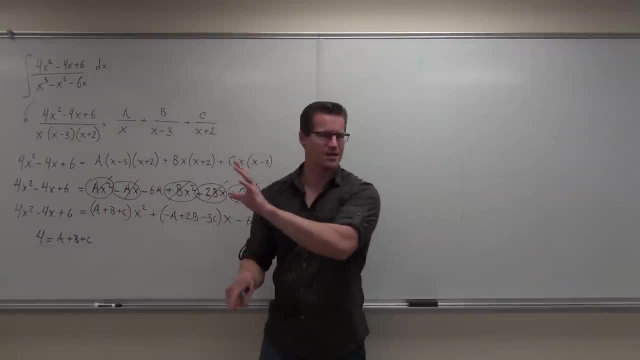 Otherwise, these things will not be equal because they have no other like terms. Quick head nod if you're okay with that one. Okay. Let's do the next one. 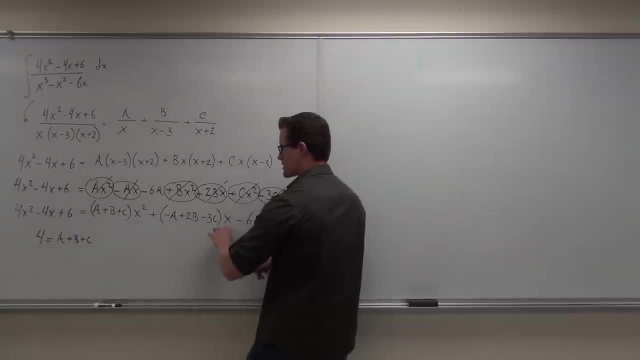 Here I have x and I have x. The coefficient of this x is what? Negative 4. 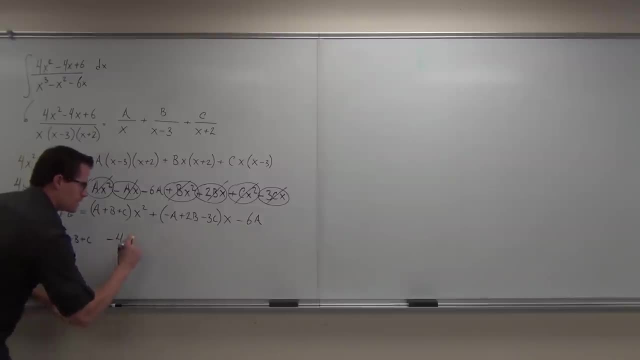 Therefore, negative 4 equals negative a plus 2b minus 3c. Just match them up. Now the last one's nice. 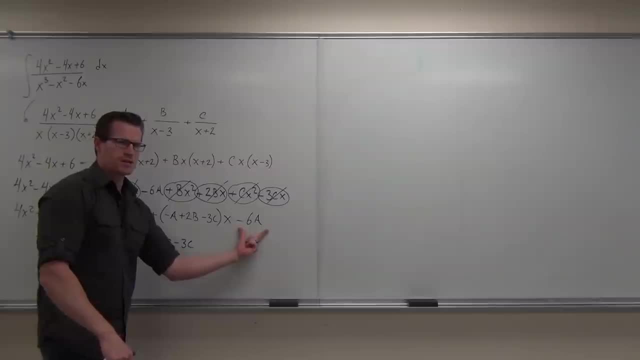 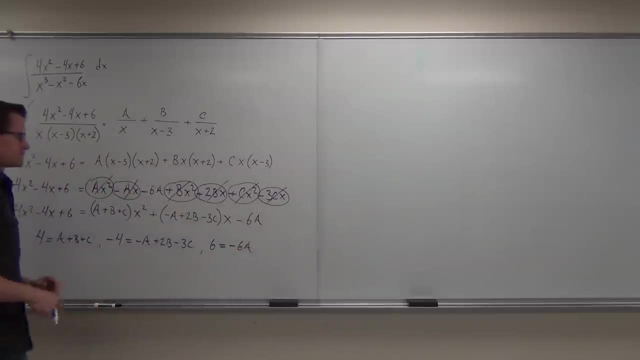 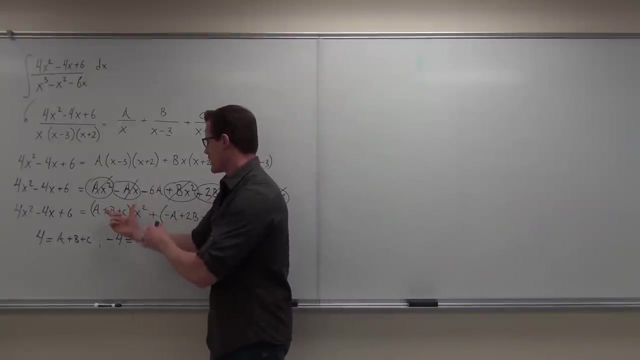 I know that my constant is 6. I know that my constant is negative 6a. Therefore, 6 has to equal negative 6a. So we've grouped all of them. We've basically factored out our like terms from our like terms. So we have. A plus b plus c, x squared, hey, 4x squared, 4 must match up with a plus b plus c. 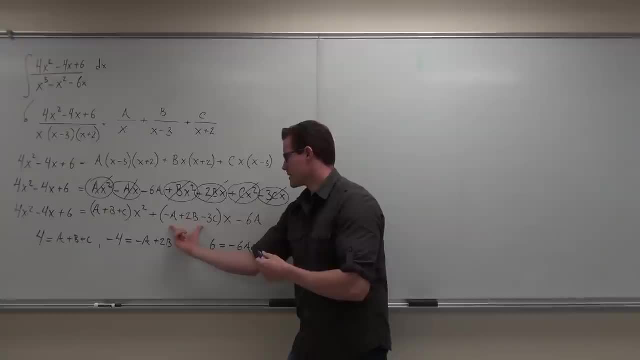 Negative 4 must match up with negative a plus 2b minus 3c. Positive 6 must match up with negative 6a. So if you're okay with the idea. 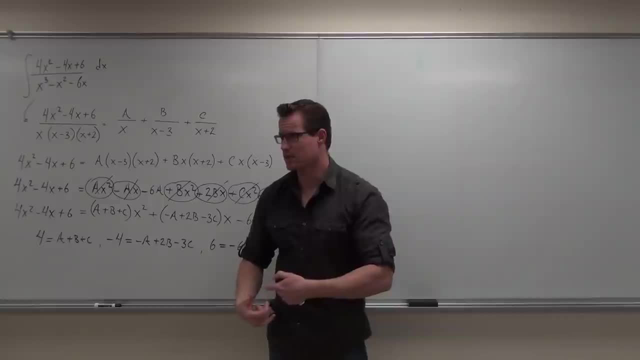 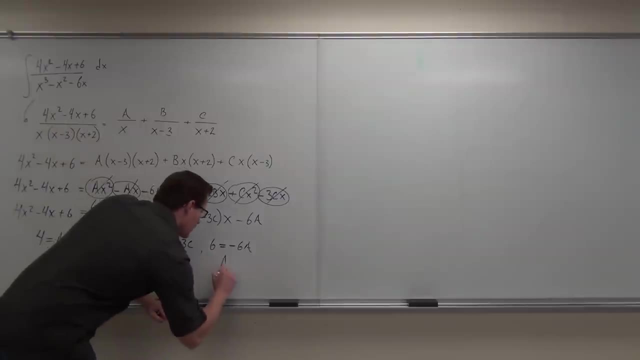 Now, use whatever algebra you know to solve these things. For instance, start easy. How much is a? Negative 1. Once you know a is negative 1, you get to use that fact over here to create a system of equations. 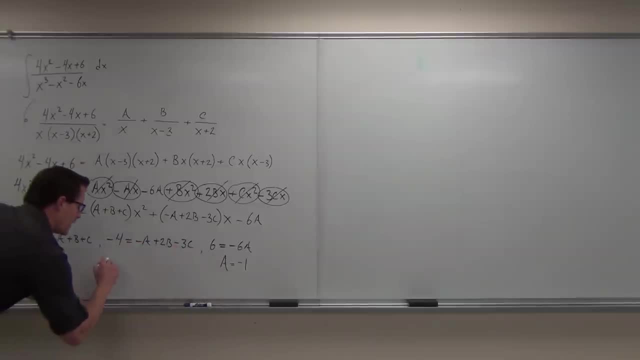 So if a is negative 1, then here we have negative 4 equals positive 1. 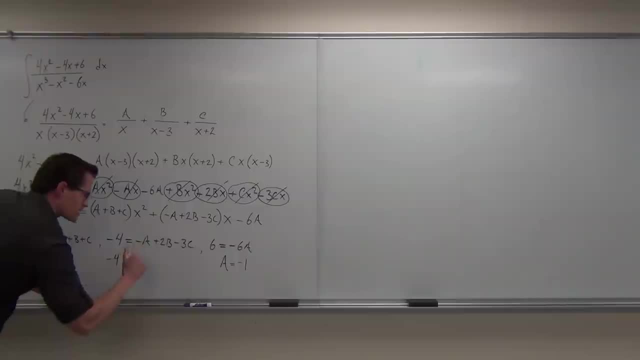 Do you see why it's going to be positive 1? Negative, negative 1, positive 1, plus 2b minus 3c. 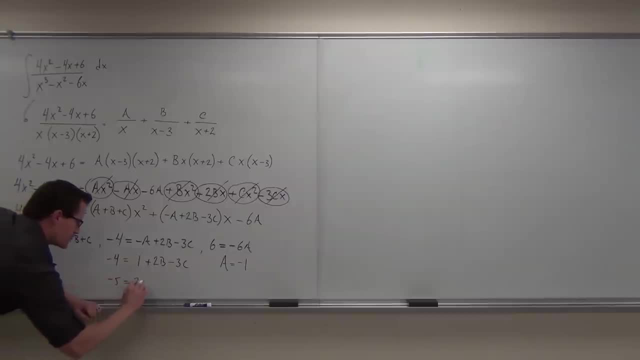 Or if I subtract the 1, negative 5 equals 2b minus 3c. Also, here's our negative 1 here. 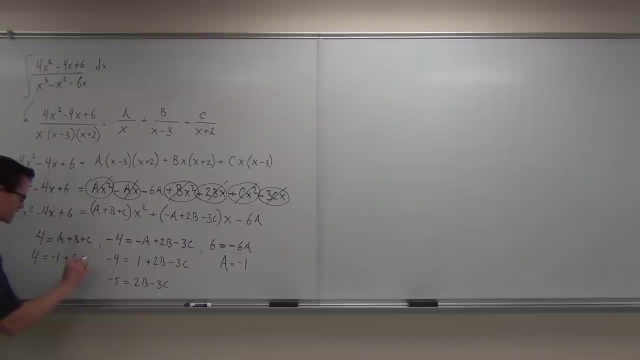 So 4 equals negative 1 plus b plus c. Or if I add the 1, what we end up getting is 5 equals b plus c. 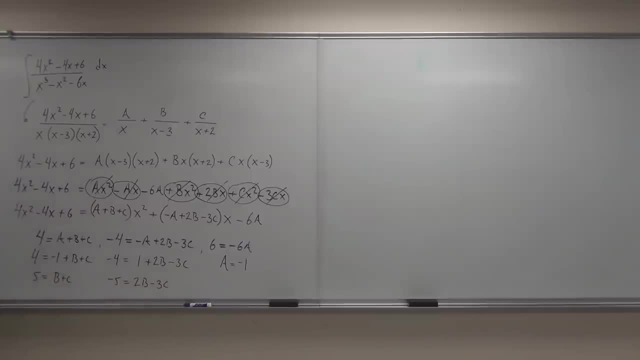 Let's see, okay so far. I'm going to have to move. Okay. 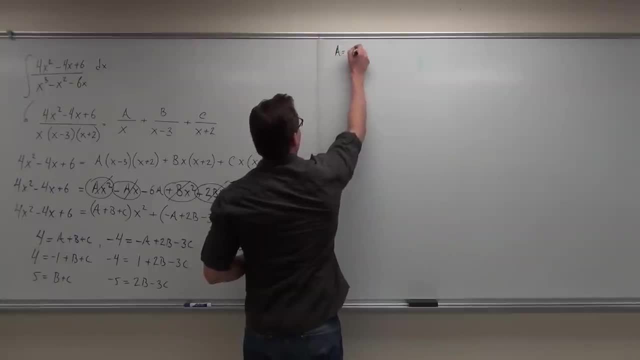 Okay, I'm gonna rewrite this a little bit. So, what I know is that a is negative one. What I also know is that I've got 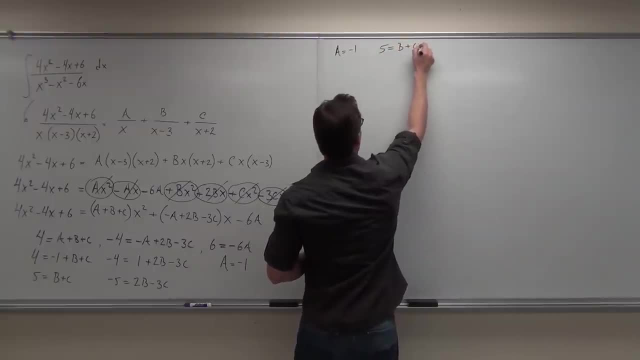 five equals b plus c. I know that negative five equals negative two, sorry, positive two b minus three c. 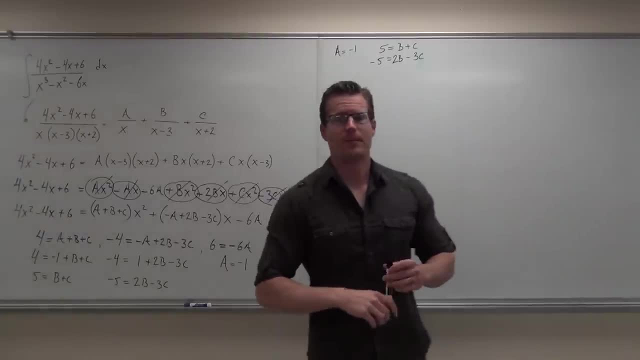 Okay, so, are you familiar with how to solve systems of equations? Yes. 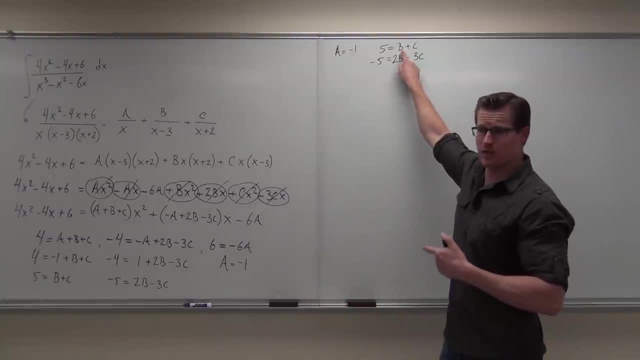 All right, so I have a to b and a not to b. How to solve this, that is the question. That's right. 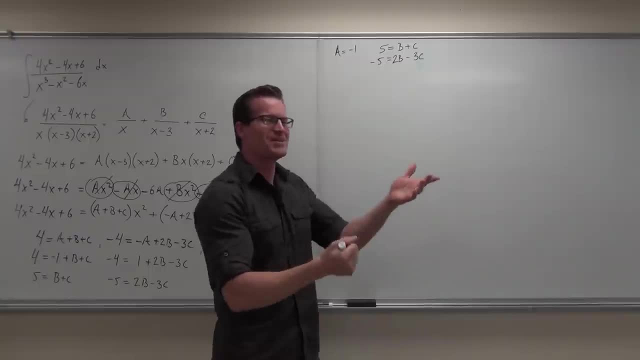 That's pretty good, right? Okay, anyway, what do I do to solve this thing? 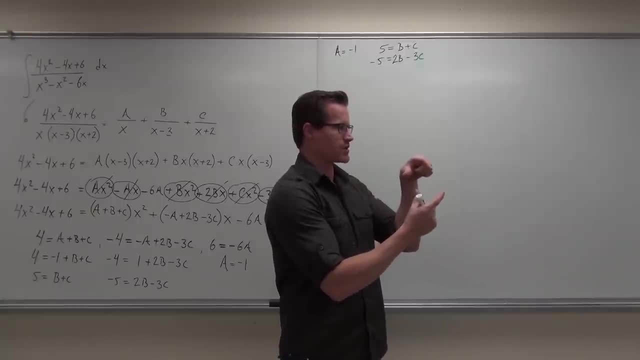 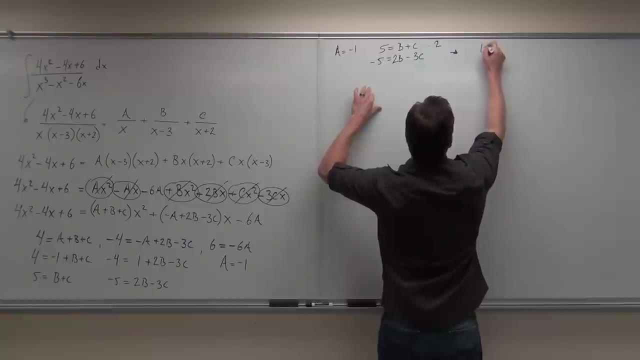 Yeah, I multiply something to get some coefficient that's the same on one of my variables. In our case, we're gonna multiply this by two. Therefore, we get 10 equals two b plus two c. 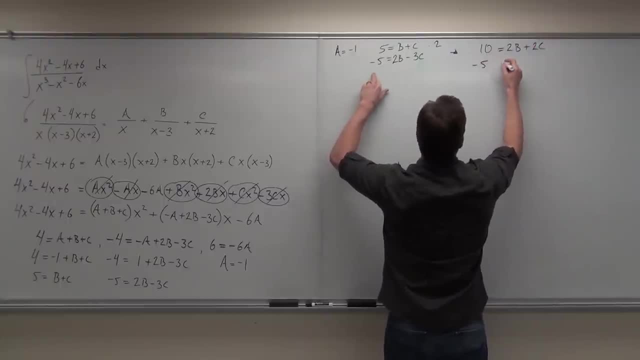 Yeah, you can do it either way. And then negative five, and we get two b minus three c. 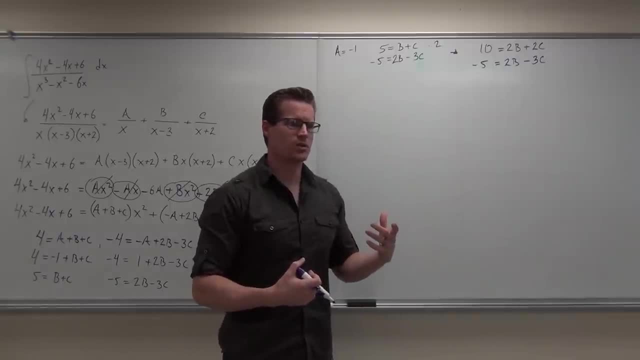 If you do that, you'll just have to subtract them. If you multiply by negative two, you would add them. Doesn't matter which way you do. Okay, I'm gonna choose to subtract them because I'm gonna get positives. Are you with me on this? You guys okay with that so far, yeah? So I'll subtract all this stuff. 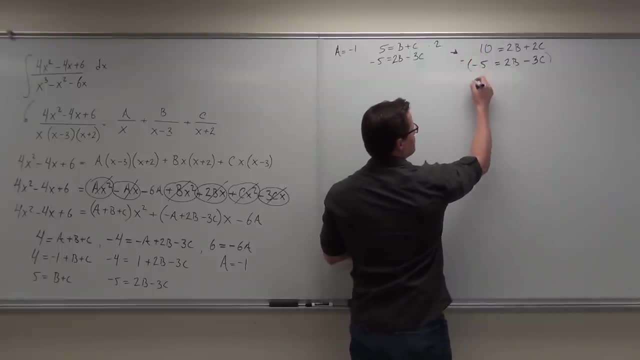 If I subtract it, 10 minus negative five is 15. Two b minus two b is zero. 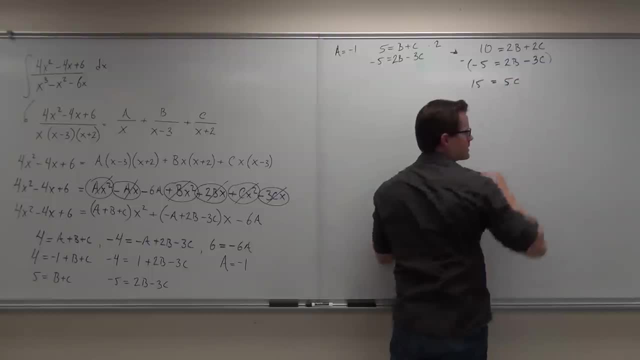 Two c minus negative three c is five c. Five c. Are you with me on that one? 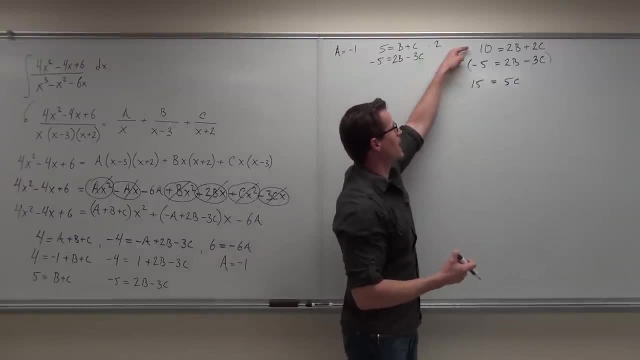 If you added it, all you'd end up getting, like if you multiply by negative two and add it, you get negative 15, you get negative five c. Are you still gonna end up with three either way? Yes. Am I going too fast on the algebra? No. Okay, I hope not. 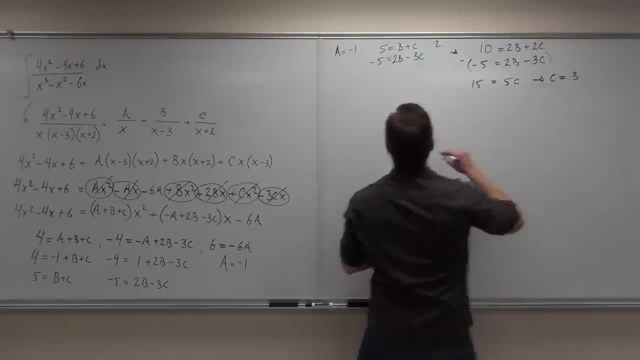 So then C equals 3. Okay, I got A equals negative 1. I've got C equals 3. Can you find out what B is? No. 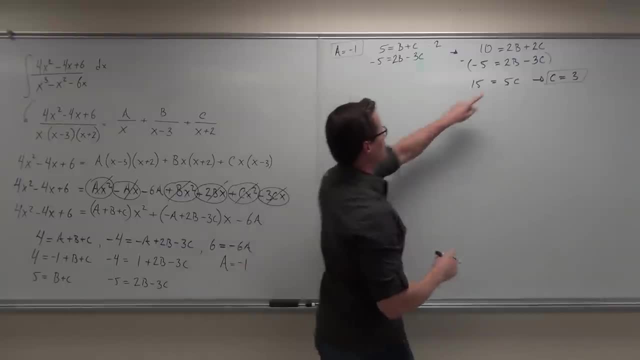 Okay, how do we find out what B is? Just plug it in, whatever equation works for you. 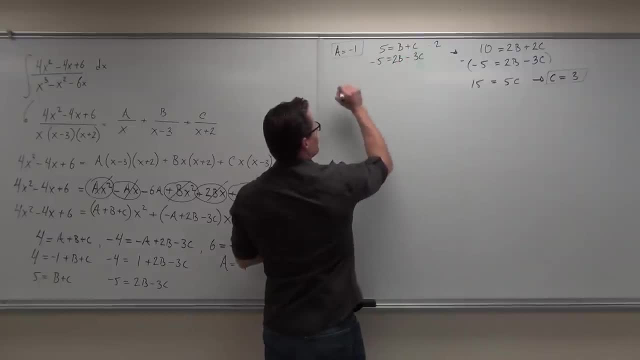 This one's going to be the easiest, so I know if A is negative 1, that's how I found out my two systems. I'm sorry, two equations. 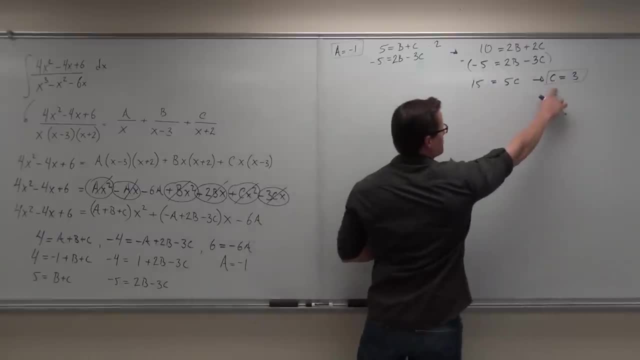 By using an elimination method, I've got C equals 3. That's great. 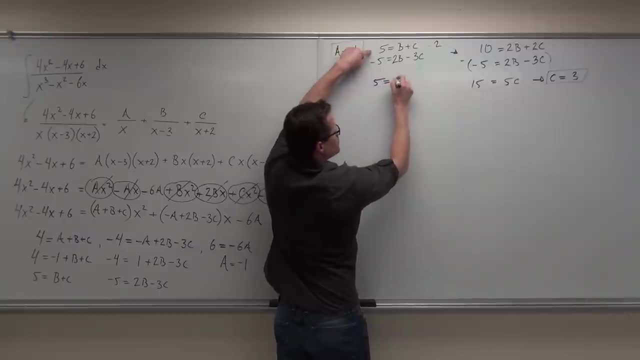 Now that I have C equals 3, 5 equals B plus 3, or B equals how much? 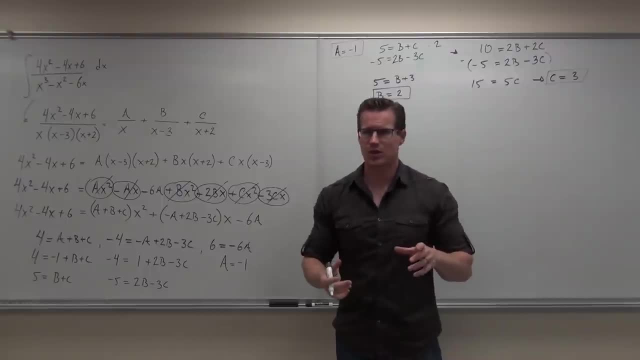 Okay, I want to make sure that we are all okay with this so far. It's just some algebra, but I know the algebra can be hard for a lot of people. I want to make sure that you guys are all right with it. So. 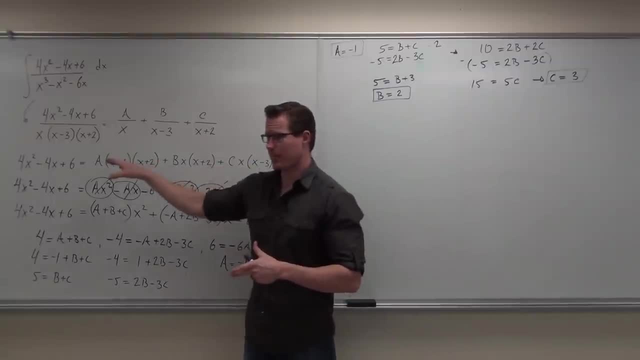 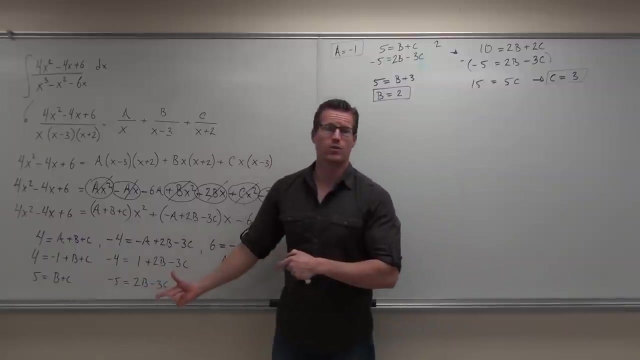 Figure out a common denominator, that way your numerators are equal. Distribute. Organize. So factor out your common terms here. So in our case, our common factors. In our case, X squared, X, and just a constant. Set them equal to the appropriate coefficient and then solve in whatever way works easiest for you. Here, this was nice. This was easy. 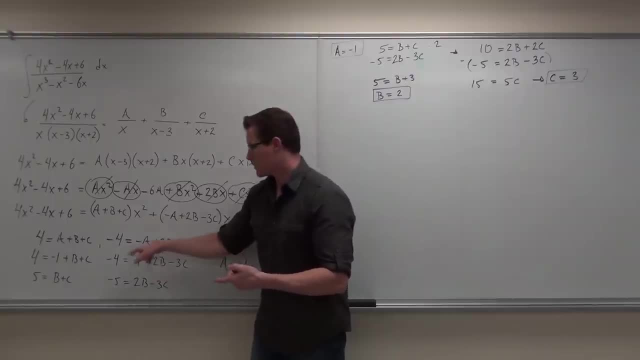 Use that. Use the easy stuff to make the hard stuff easier, okay? Now that we have a system of equations, use anything. You can do substitution. You can do elimination. I don't care. It's all going to work. 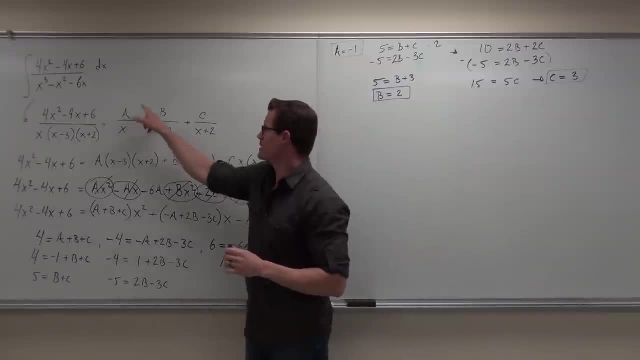 I'll do exactly the same. All you need to be able to do is find out what these letters are. However many of them you have, you need to know those letters. Feel okay with that one? 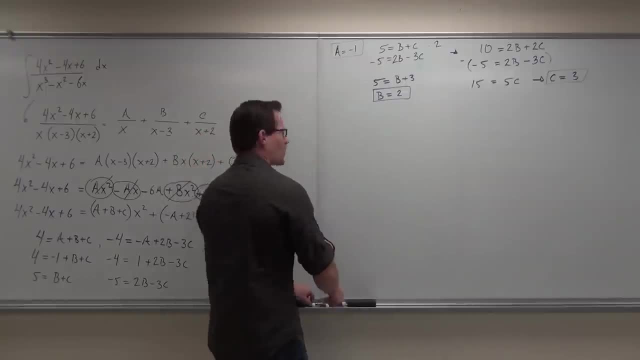 Now, here's what this means. What this means is that our original integral, this is the cool part. 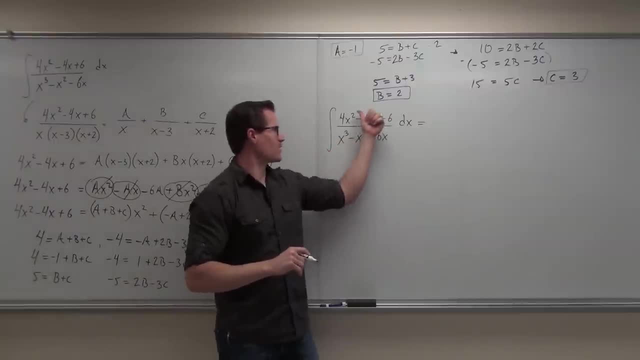 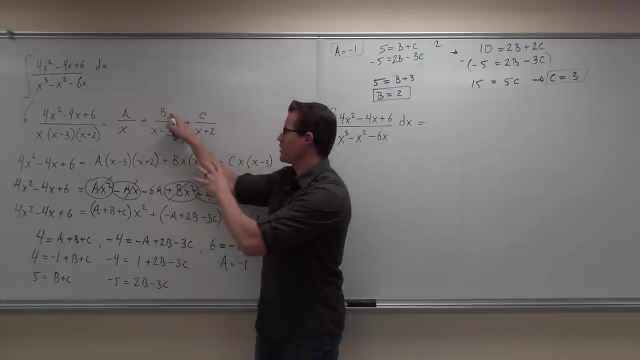 Our original integral, because our degree here is less than our degree here, it meant that I could do this. Because I did this and now I found out my coefficients, check this out. 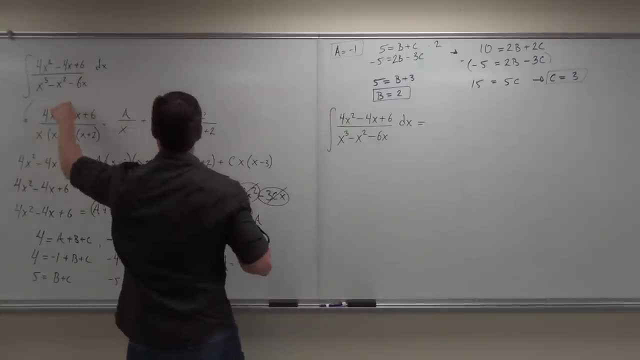 This is the awesome part. Now, this integral becomes, hey, how much is our A? 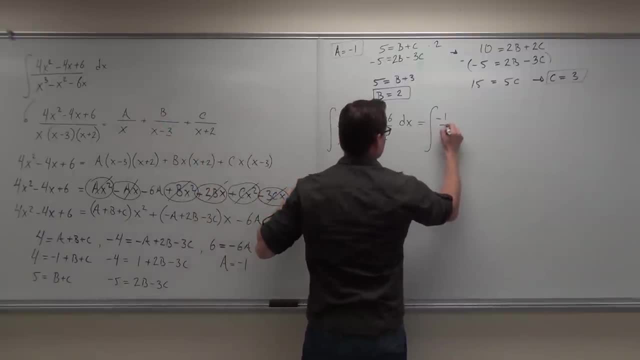 Negative 1. Negative 1 over X. Plus, how much is our B? 2. 2 over X minus 3. 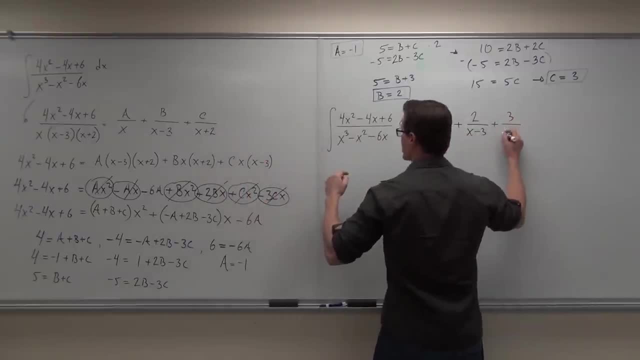 How much is our C? 3. Plus 3 over X plus 2, DX. 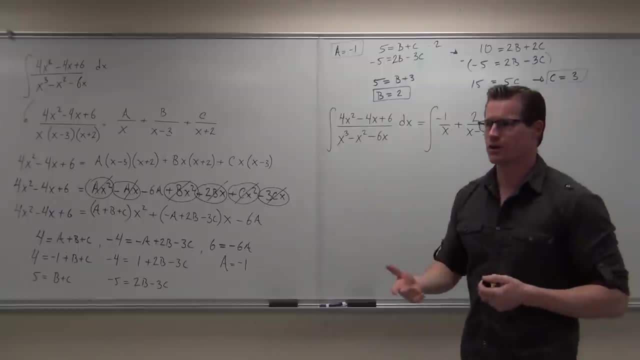 If you can make that jump, you understand how to do integration by partial fractions. Do you understand that jump right now? I need to make sure that you actually do. Show of hands if you do understand that jump. 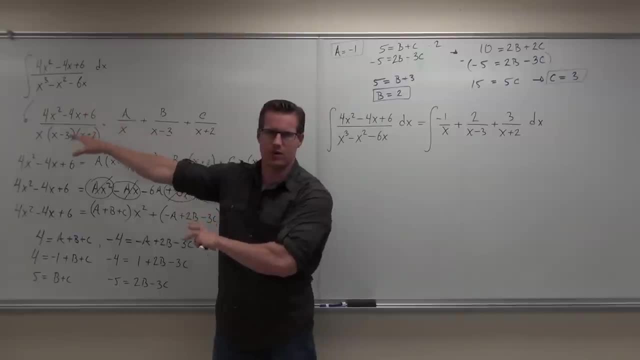 The jump is use some algebra, a whole bunch. This is the hard part. This is going to be easy, okay? 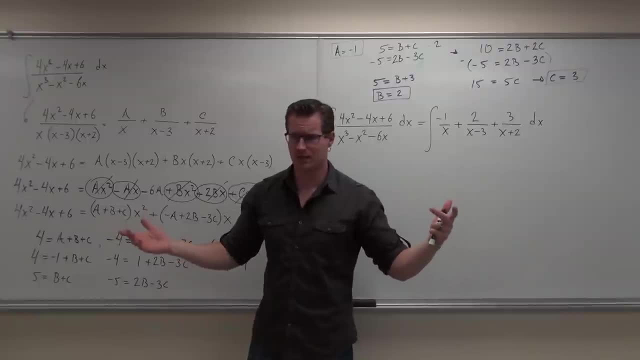 If I didn't tell you this already, you have learned every technique of integration that we are going to cover here. Then we're going to apply them to improper integrals, so it's going to be a little bit of a change. 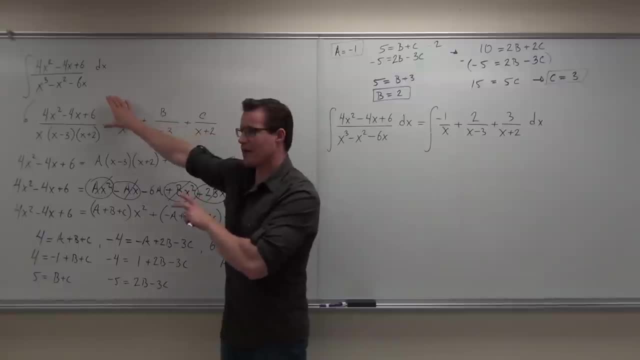 We're doing this, but this is all algebraic. So what this says is use some algebra to figure out that this is equal to this. 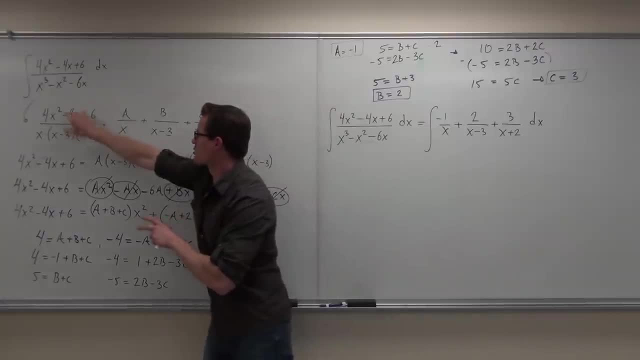 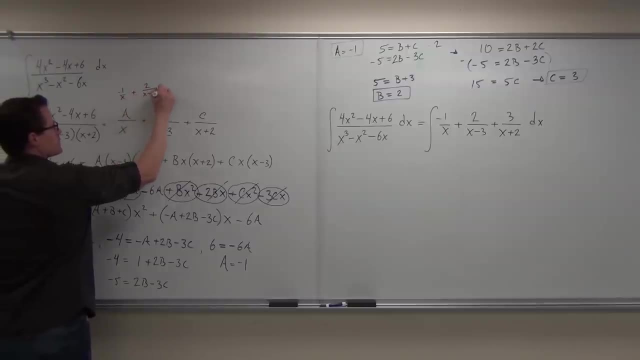 If you figure out your coefficients, A, B, and C, then this fraction is equal to negative 1 over X plus 2 over X minus 3 plus 3 over X plus 2. Hey, look at that. 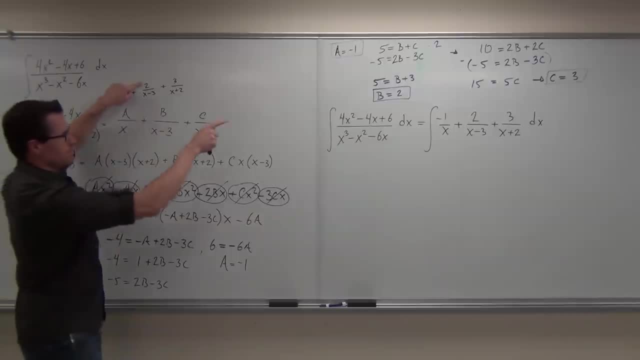 A was negative 1, right there. B is 2. 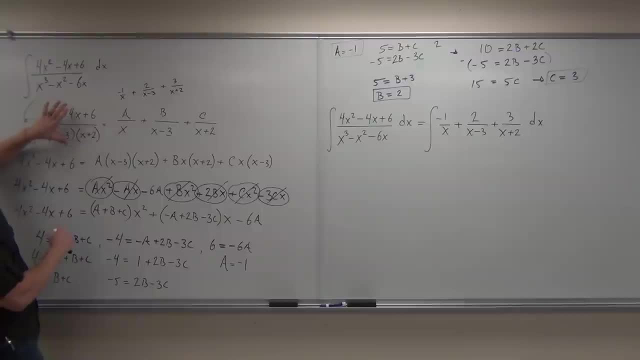 C is 3. Therefore, we have 2 over X minus 3. Therefore, since this fraction equals this sum or partial fraction, 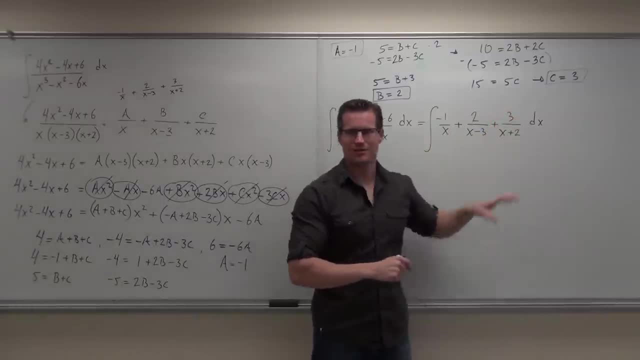 this integral equals this integral of partial fractions. So far, so good? It's kind of neat, right? 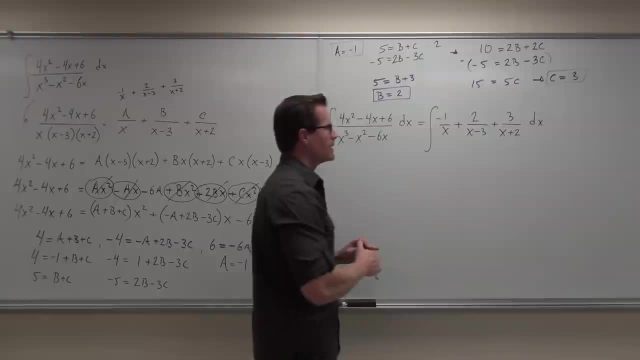 Now, the rest of this stuff is really easy, really easy. A lot of times, not a lot of times, all the time with your linear factor, with your linear denominators, you're going to get a whole bunch of LNs. 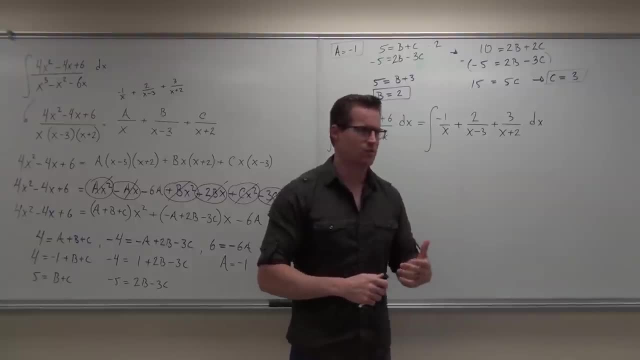 So we don't want to, I don't, I never like to write more than I absolutely have to. So when I do this, I do all these in my head, because I'm used to doing the substitution. If it takes you some substitution off to the side, do it. But here's the deal. 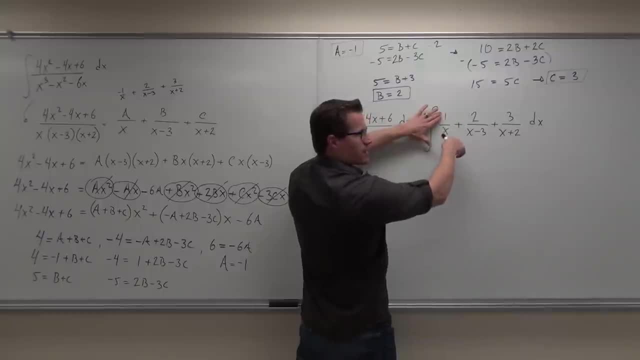 How I do this integral, I'd say, hey, look at this. The integral of 1 over X is LNX, LN, LN, absolute value, remember the absolute value? 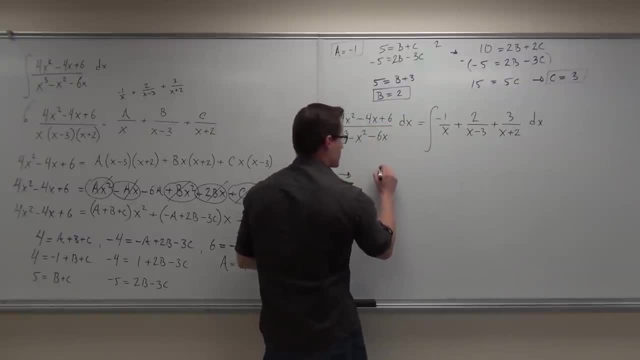 So this integral, the integral of 1 over X is LN, absolute value of X. Since it's negative, we just have a negative out front. It's a, the negative's that constant. It's a negative 1. So if we have a coefficient, the coefficient just stays there. Quick head nod if you're okay with that one. 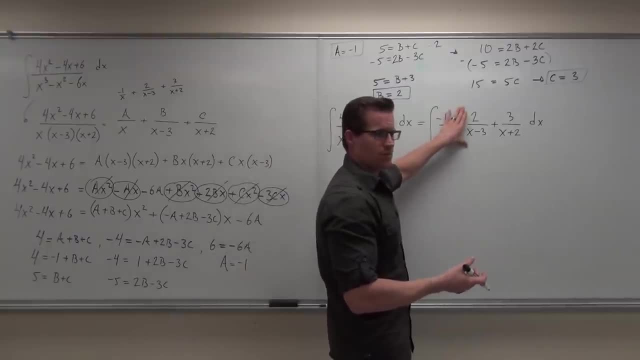 Now, this one. By rights, you should be doing a substitution, shouldn't you? 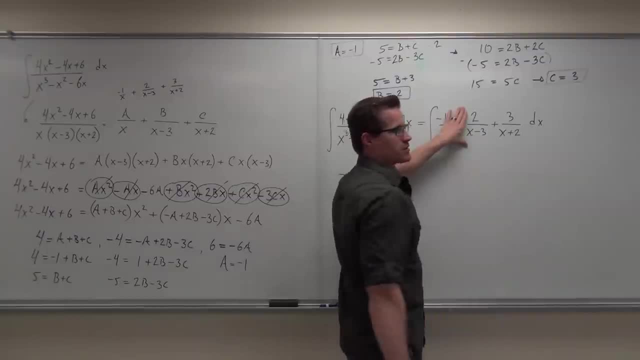 However, if you did a substitution on this, the derivative is 1, which means you're not going to be changing that coefficient whatsoever. 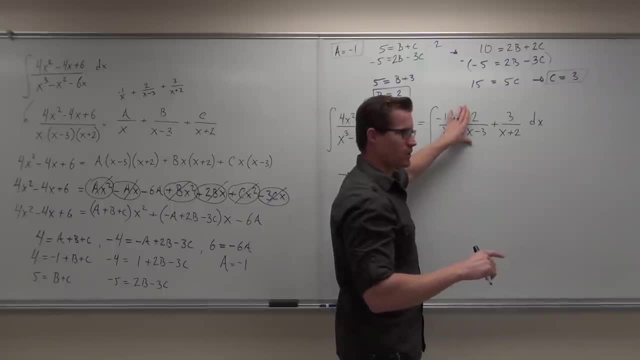 If this was like a 2X minus 3, yeah, you'd probably have to do a little something with that. I would probably still do it in my head. 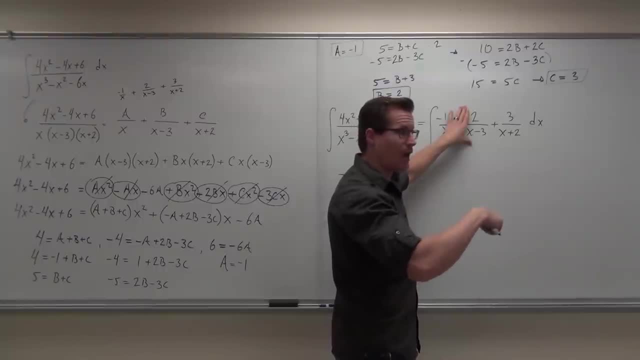 I'd do a little substitution in my head. I would know how to do that. I'd get a 1 half. 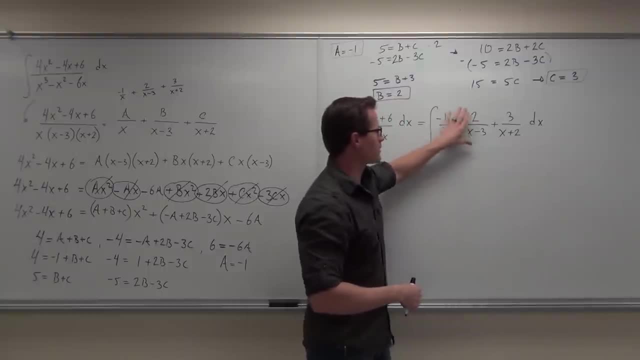 But you'd have to take that into account. But notice that if it's linear, you can always do that quick substitution, and it's still going to be an LN. The integral's still going to give you an LN. Are you following? 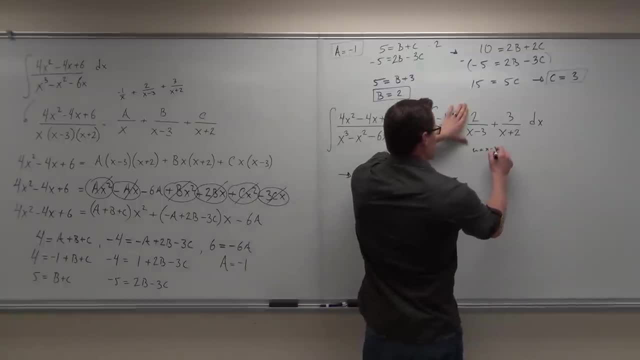 So in our case, if you had to do U equals X minus 3, DU equals DX, okay, that's fine. Do it up to the side. That's okay. 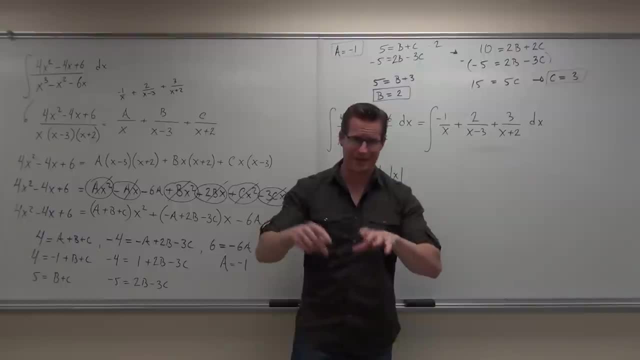 I'm going to be a little bit quicker on that because I'm going to assume at this level that you understand how to do this right now, okay? 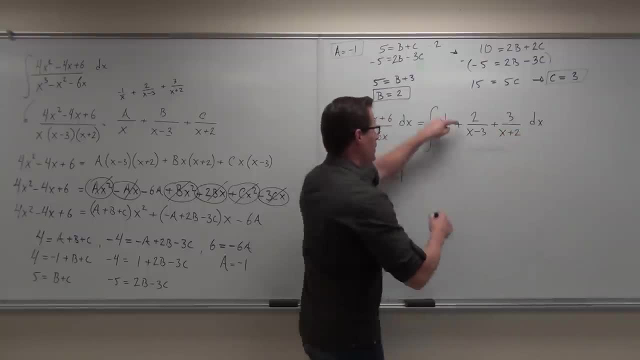 So you could split this up and do it independently of each other. Here we're going to have a plus. What's going to be out front? 2. And then LN absolute value of X minus 3. 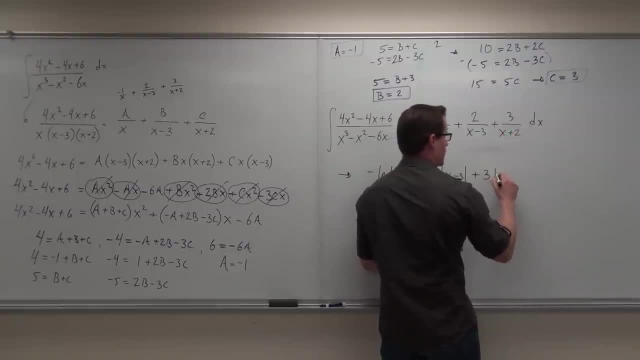 Then another plus. This is our coefficient, 3 LN integral X plus 2. 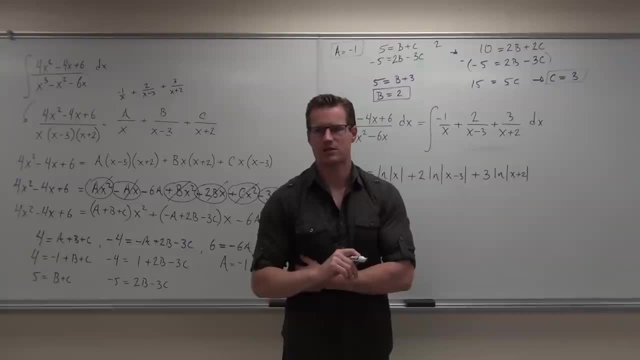 Just please, please be careful on this part. Let me have your eyes on the board here real quick. 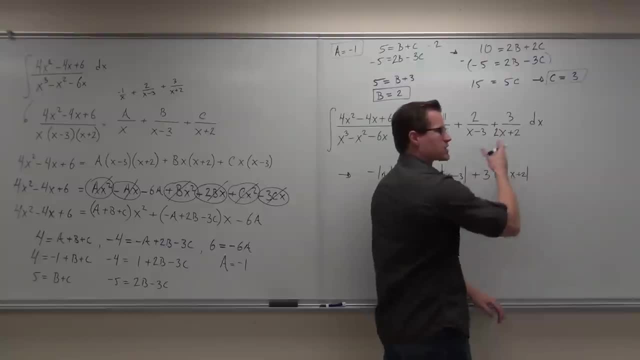 Be careful of this. If you had a 2 right here or some other coefficient, this is not the correct integral. This is not the correct answer. 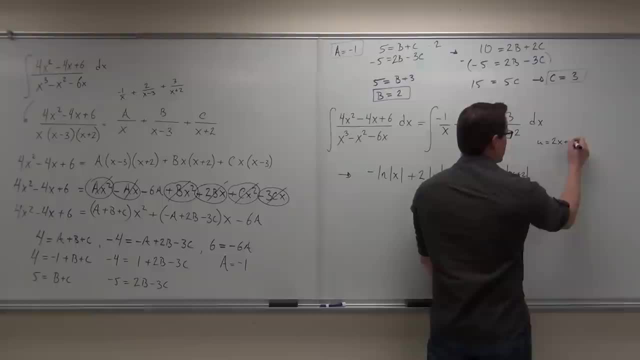 What would happen is you would do, I'd do, I'd still do it in my head, but I'd get, okay, DU equals 2 DX. That would give me a 1 half. That's what that would be. Can you follow that one? Yeah. 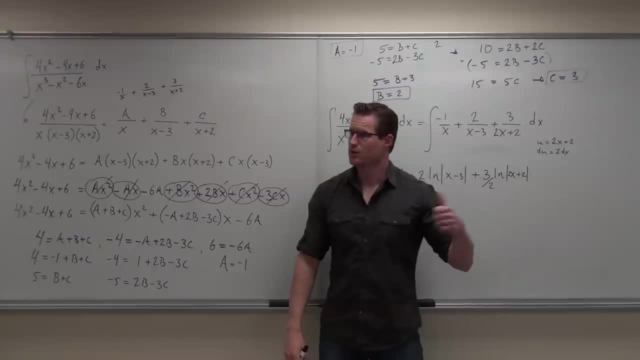 If you got that, then you're probably pretty good at this and you're fine. But if you're not getting like, wow, where's it coming from? Then take some time on your own and actually do the substitution off to the side. You can't get these things wrong. Well, you can. I mean, I don't want you to. Don't get these things wrong. The constants and the coefficients are very important here. So it makes you feel okay with this one. So do you understand that? 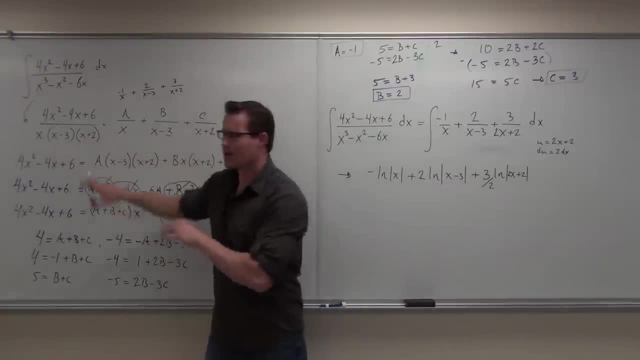 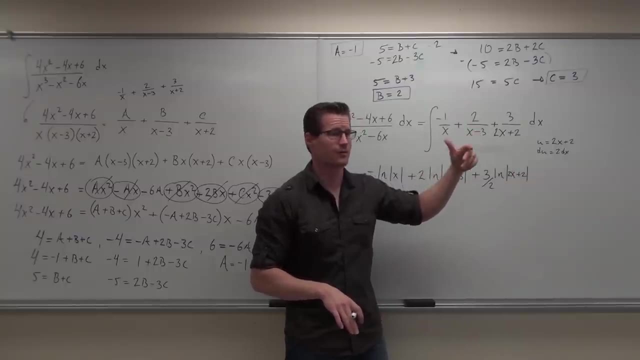 If I have linear factors, I'm going to get a lot of LNs because it's going to be 1 over a power, X to the power 1, I'm going to get a lot of LNs here. This was not the case. How do I wrap, oh, sorry, this one too. How do I wrap this up? 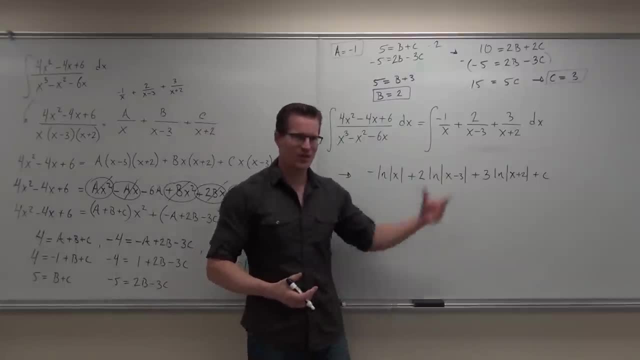 Done. That's the whole idea. What's the hard part? Is it the integral? No. Heck no. 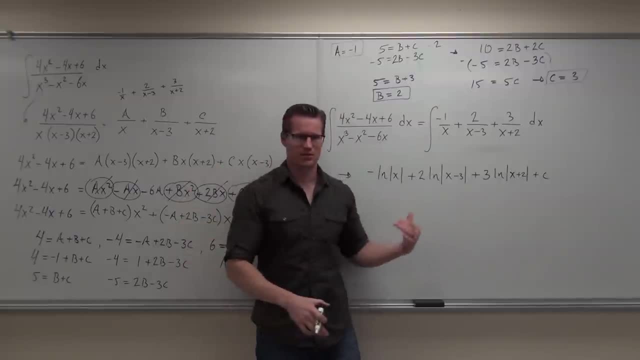 The hard part is this, doing all this stuff. Show if you guys feel okay with this one. 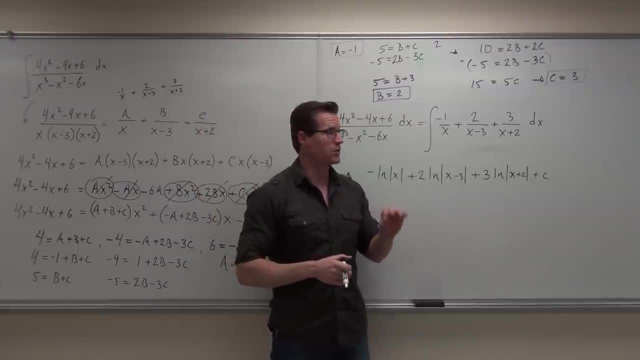 Now, would you like it if I showed you a shortcut that applies to a lot of these problems, especially the linears? You want to see that? Yes. Okay. Remember these numbers. We can cheat. We can cheat a lot. 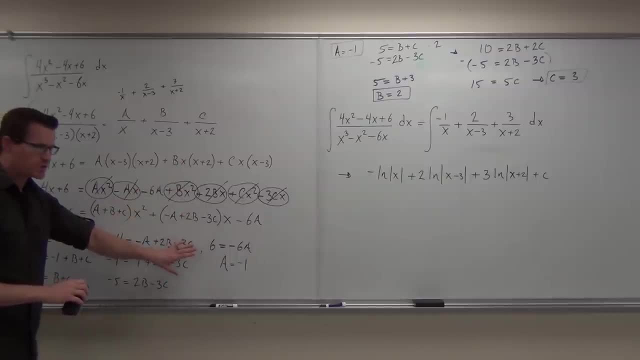 So you have this written down, correct? Are there any questions on this? Should be pretty straightforward. I wanted to give this to you. 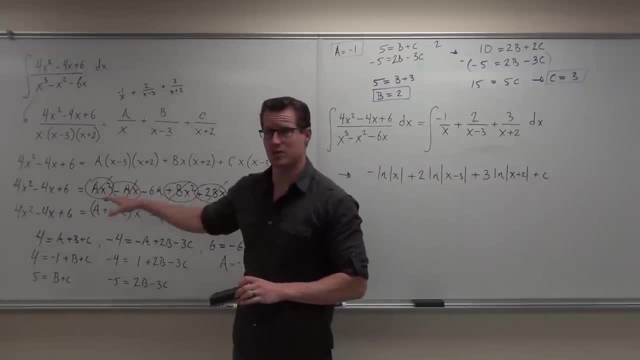 By the way, sometimes you have to do this technique because you can't do the cheating. The cheating way I'm about to give you. But with linear factors especially, cheat at it. Here's how you cheat at it. It's not even cheating. It's just being smart. 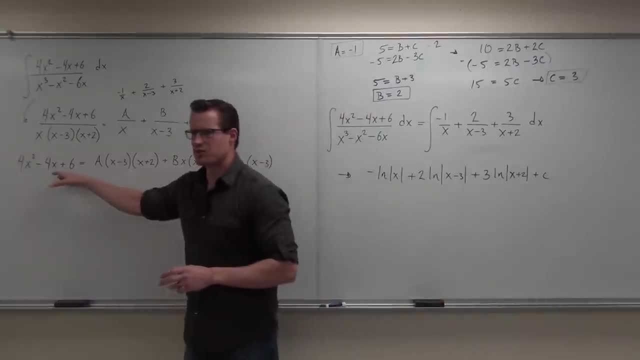 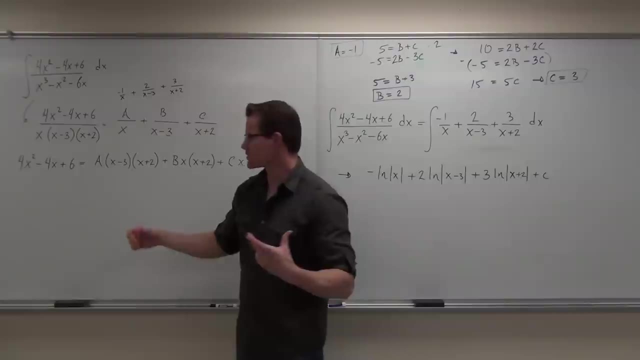 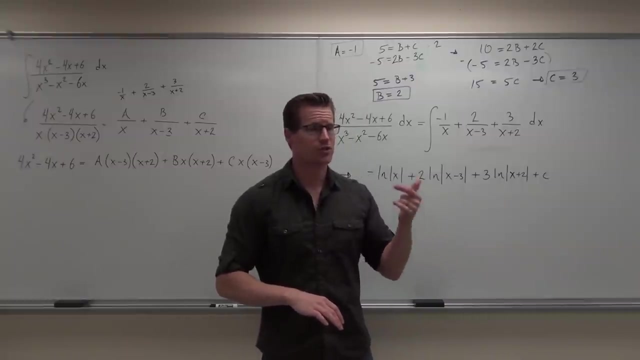 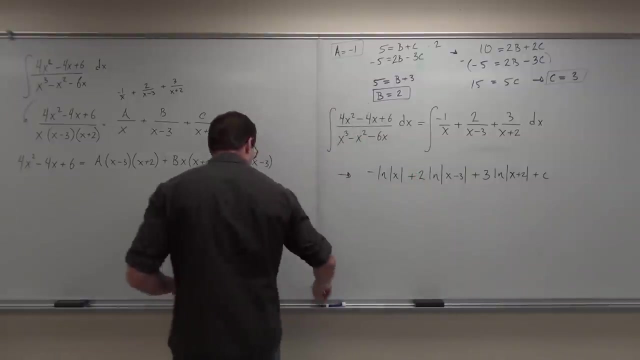 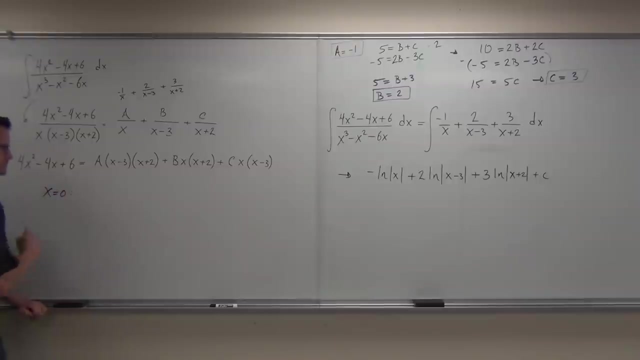 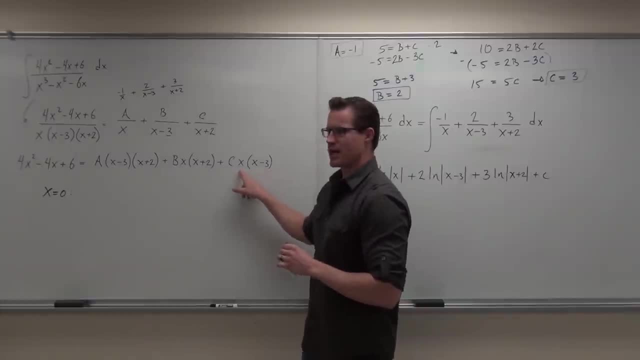 If I let x equal zero, this, yeah, it's negative 3, but which is that? This whole thing is gone. Does it make sense? This would go to zero. 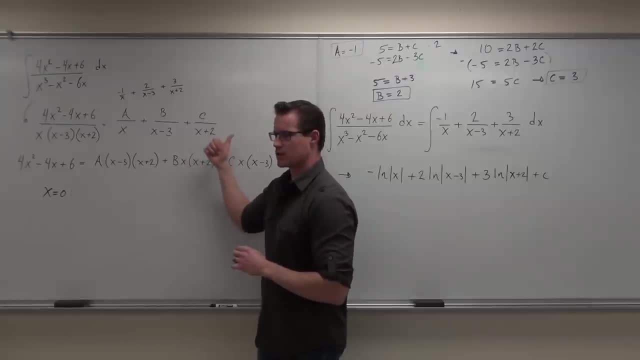 If I let x equal zero, this whole thing is gone. Does that make sense? 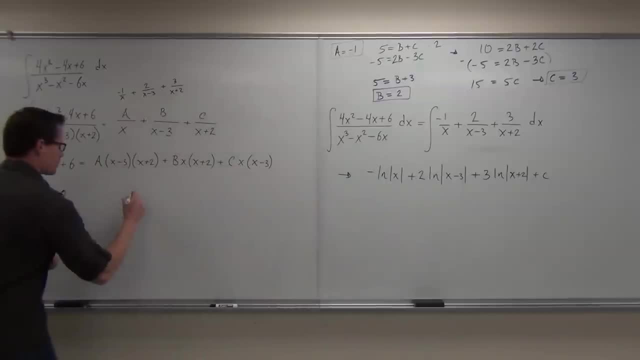 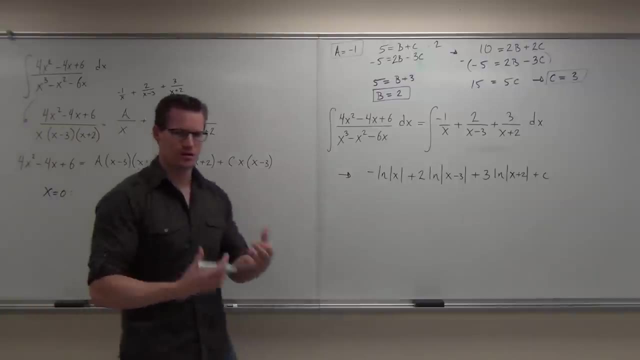 If I let x equal zero, this is a times negative 3 times positive 2, because x is now zero. You follow? 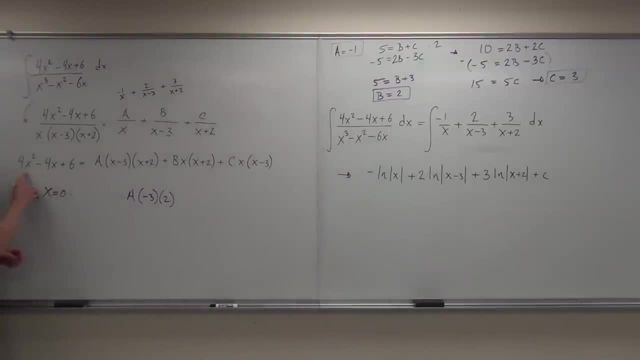 On the other side, if x is equal to zero, this is zero, this is zero, how much is that? Then we would get 6 equals a times negative 3 times 2. Let me go over it one more time to make sure you're with me, okay? 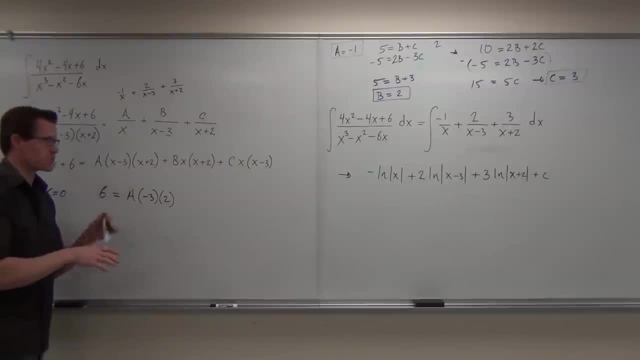 Plug in values that make some of your factors go to zero. You will have repeated factors, okay? So I'm thinking, hey, the easiest one to plug in, if I plug in zero, this is not zero, this is not zero, but this is. Zero times anything is what, folks? Zero. This whole thing is gone. Zero times anything is zero. 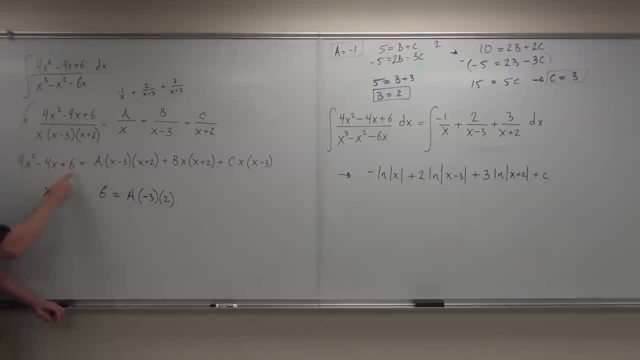 The whole thing is gone. This is also zero, this is also zero. So if I plug in zero, zero, zero, six, got it. 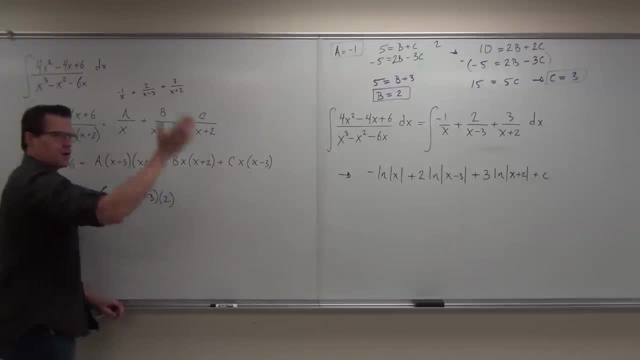 A, no problem, negative 3, no problem, 2, no problem, zero, zero, gone. Can you solve that? Yeah. So quick. 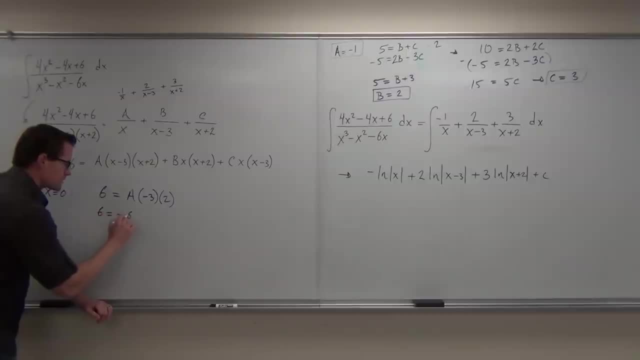 So. Six equals negative 6a, a equals negative 1. Hey, is that what we got? Yep. Brilliant. 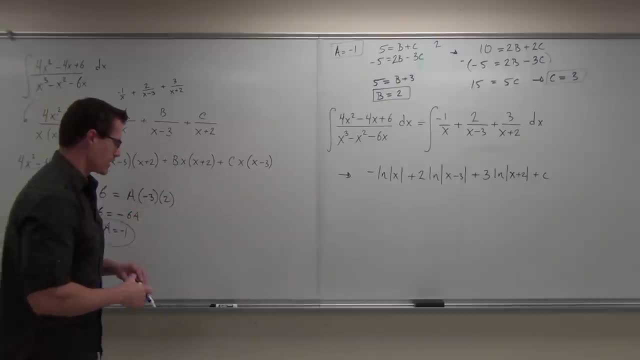 Now, we got a couple more to do. Don't do anything more with this right now. 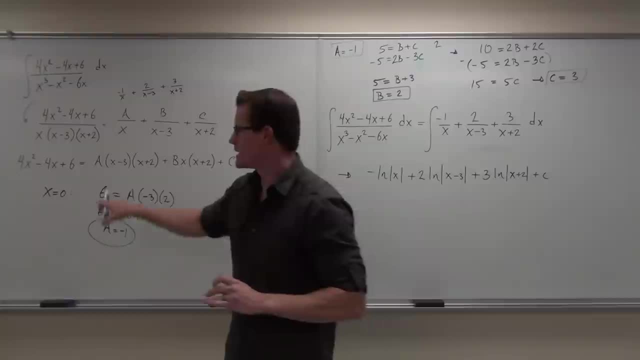 By the way, I always start with this, always. I always get as many as I can. Sometimes you'll still have to distribute, but at least you got a couple. That makes some of this kind of irrelevant. 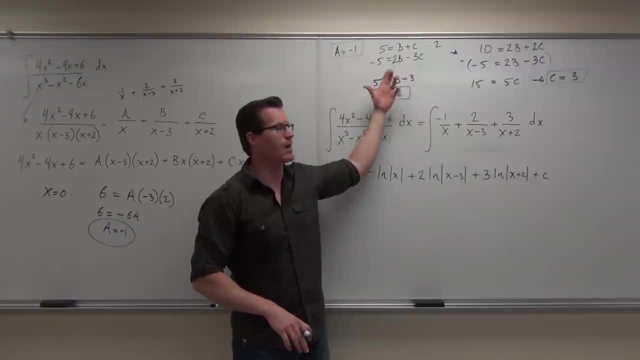 If you knew what b was, you could find c very easily without having to do systems of equations, okay? 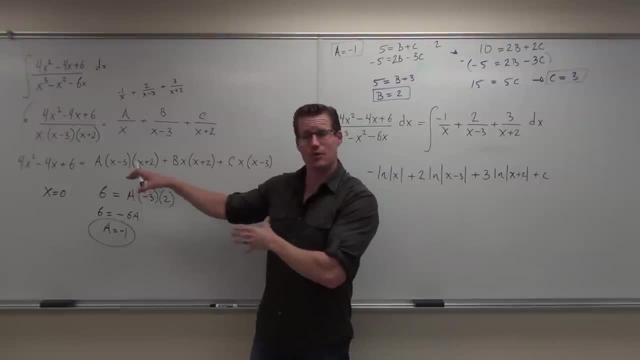 So this is a very fast. This is a much faster way of doing things, if you can. Sometimes you can't, but if you can, yeah, try plugging in some numbers. 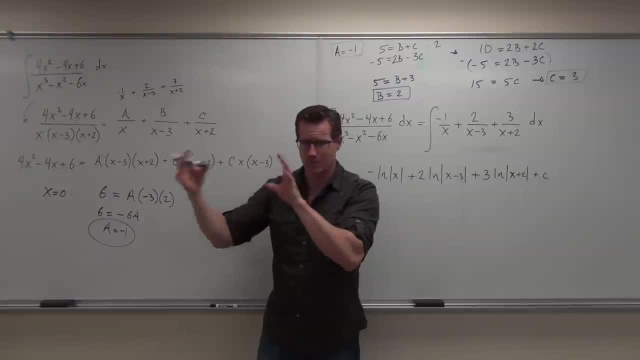 It'll give you zero, or on some of your big terms here. So big terms makes a factor equal to zero. 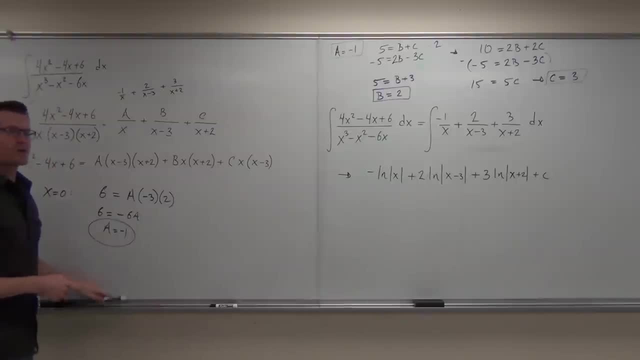 Give me another number that would work. Three would be a great number to plug in. Do you see why? 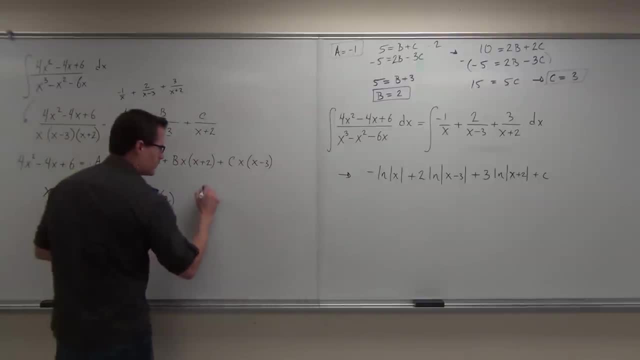 Okay, so if I plug in 3, I always put what I'm plugging in, so x equals 3, and then I put a little couple dots or a colon here. 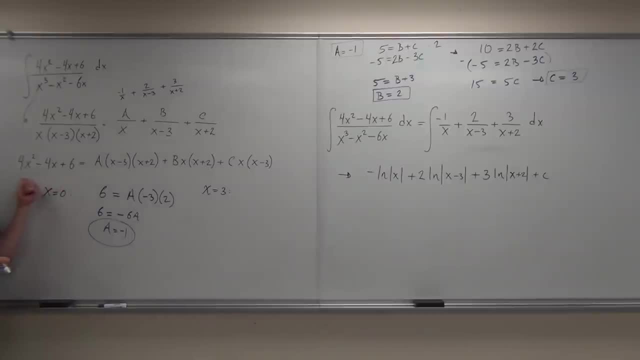 If I plug in 3, let's see. Can you figure out what I'm going to have on the left-hand side if I plug in 3? Notice I'm plugging in 3, not 0. This doesn't go to 6 again. You actually have to plug in the 3. What do you get? 30. 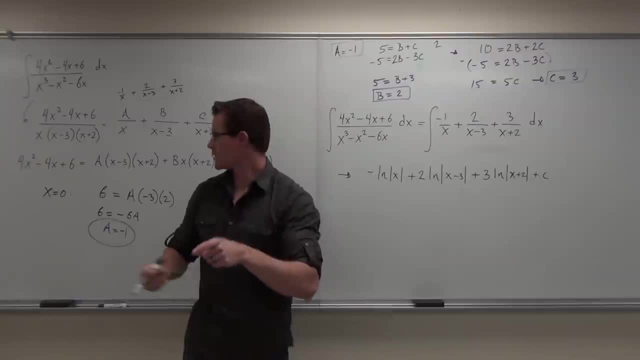 30? We're going to double-check on the 30. Do you get 30? Plug it in. Plug in 3. I want everyone to do this right now. Plug in 3. 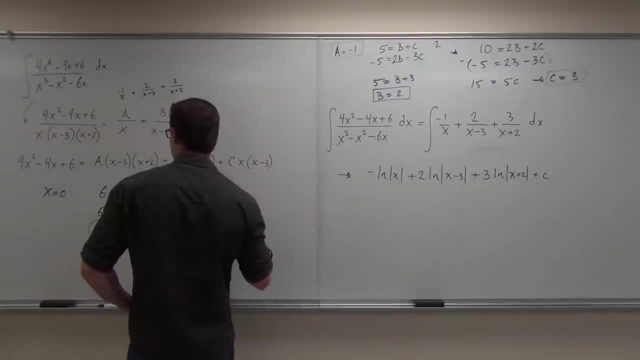 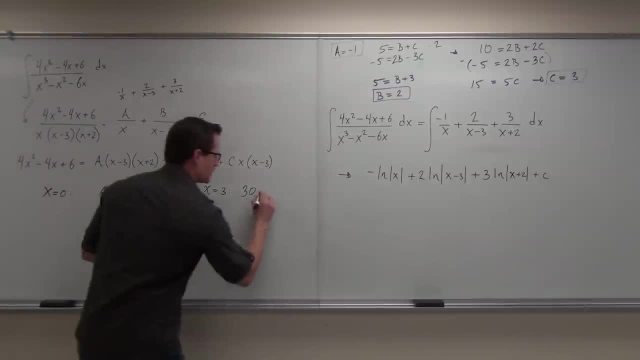 So if I plug in 3, I get 30 equals, let's look what happens. Check it out. 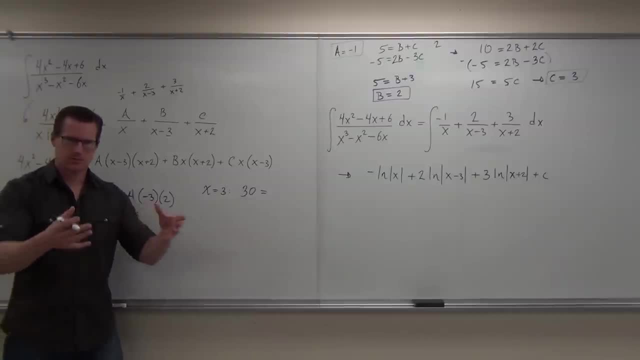 If I plug in 3, please follow me up here. This is how you're going to get this up quickly, okay? Not spend 30 minutes on just the setup. Plug in 3. What happens here? This whole thing is 0. Plug in 3. What happens here? Does it go to 0? No. 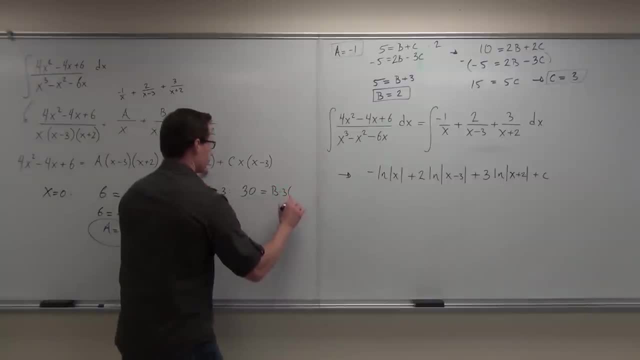 This is B times 3 times 5. See where the 3 and the 5 are coming from? 3, 5. 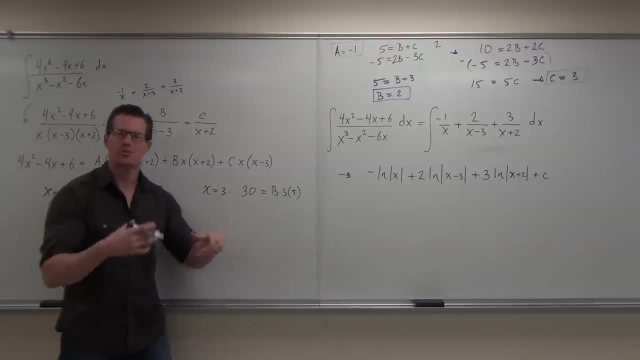 Plug in 3 here. What happens? This is why we plugged in 3, to make our factor 0. You multiply it by 0, it's gone. See how easy that makes it? 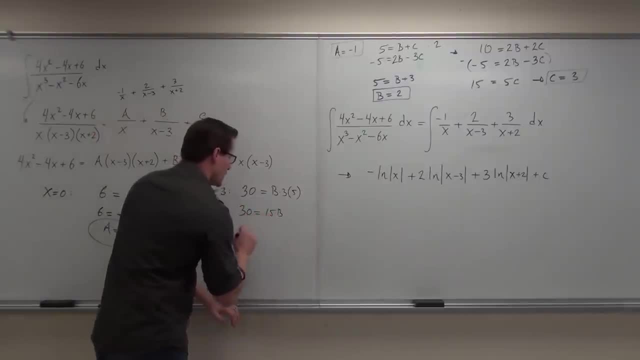 Well, now we have 30 equals 15B. How much is B? Hey, we're 2 for 2. That's cool. Why don't you do the last one on your own? What number will you be plugging in if you do the last one on your own? Negative 2. Negative 2. Yeah, very good. Not 2, but negative 2. 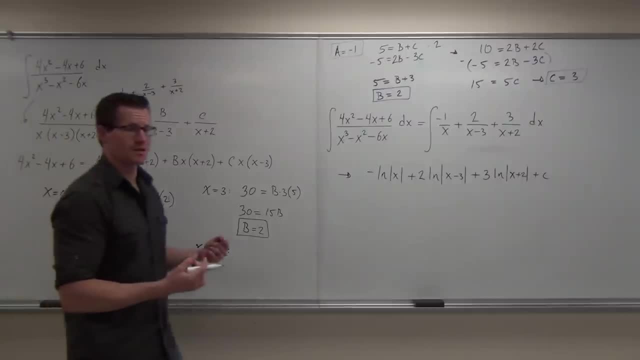 Be careful on evaluating right here. Make sure you have your signs correct. It's a big deal. 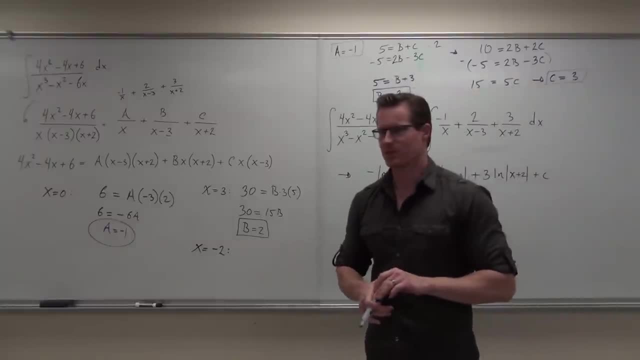 You have to get your signs correct here. I know it's algebra, but remember, people take calculus to finally fail algebra. I want that to be you. Make sure your signs are right. 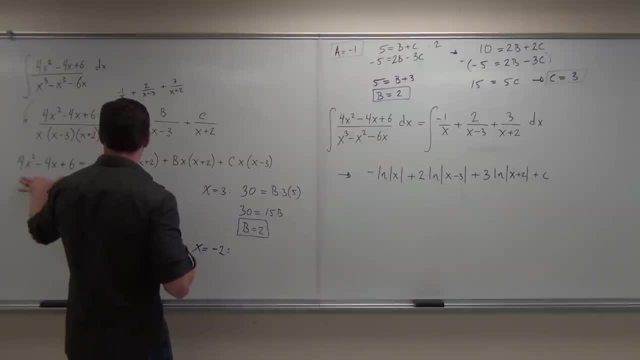 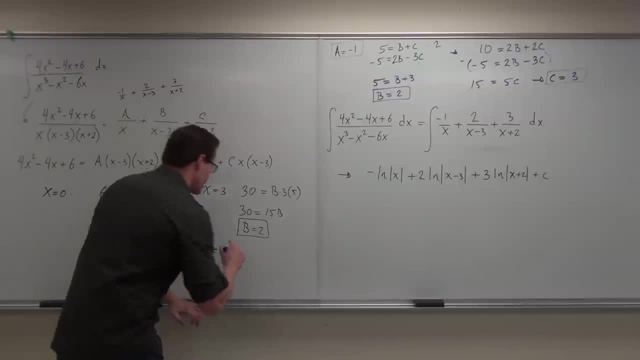 Yeah, very cool. Do you have 30? Mm-hmm . Do y'all get 30, positive 30? Yes. 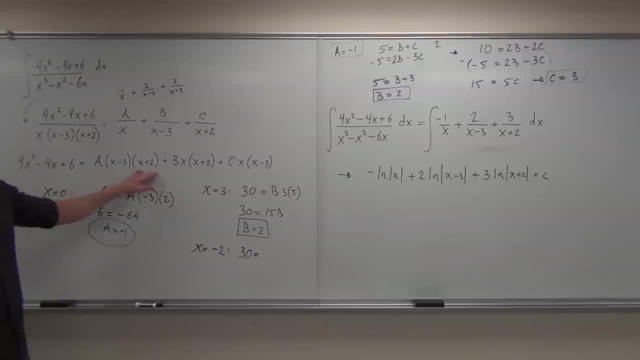 If I plug in negative 2, what happens to this term? 0. What happens to this term? What happens to this term? Negative 5 and negative 10. 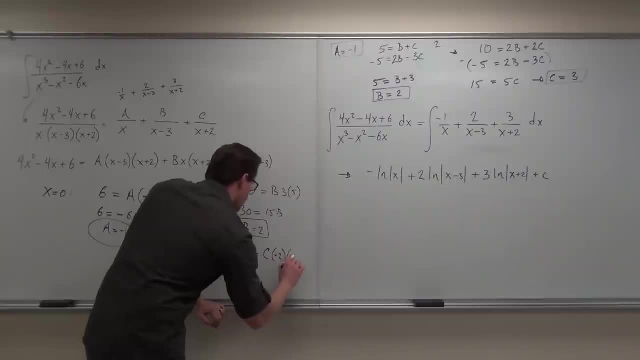 You get a C. You get a negative 2, and you get a negative 5. soothing music 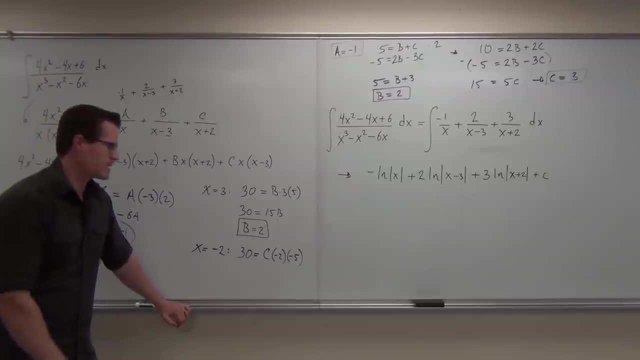 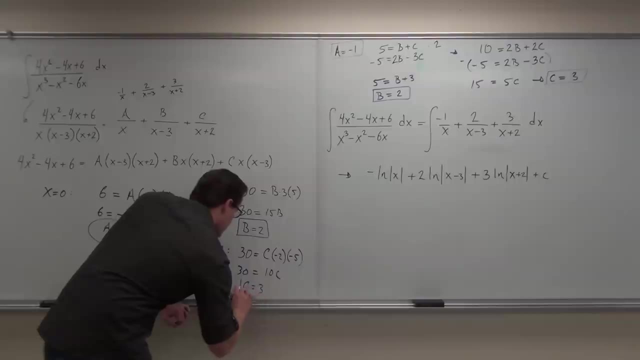 See where the numbers came from? Plug in that negative 2. Well, then we got 30 equals positive 10C or C equals 3. Did we end up getting the same numbers we got over here? Yes. Which way is quicker? This way. This way is obviously quicker. 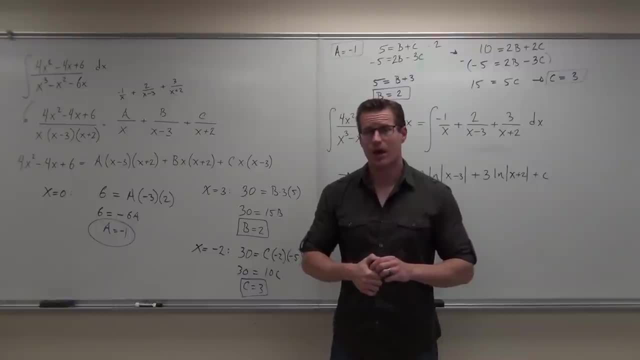 Does it work all the time? No, it doesn't work all the time, especially when you have non-reducible quadratics. Because if you have non-reducible quadratics, then you can't plug in a number that gives you 0, like x squared plus 4. Can't do that. That factor's not going to be equal to 0 ever. 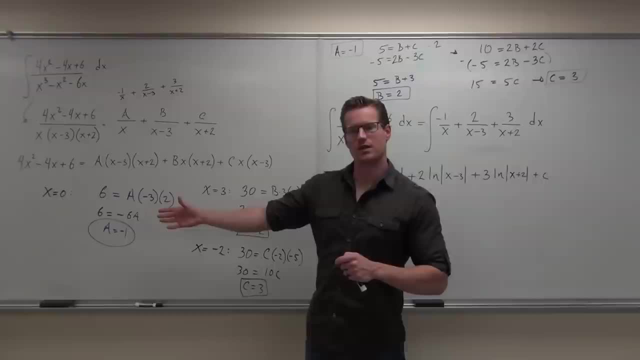 Therefore, you can't use this technique with that. You can use it for parts of it. 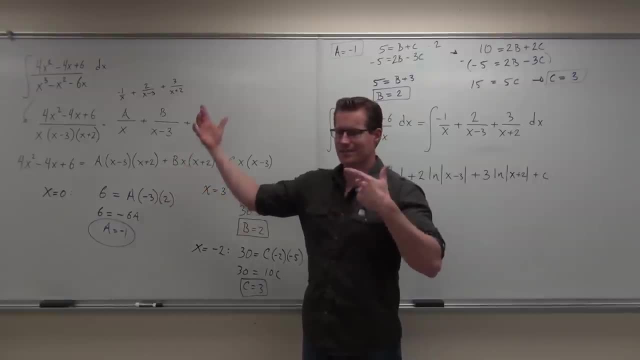 So like if you have a linear factor, man, use it for the linear factor. Make that 0. At least it gives you some of those numbers. You follow me? So you'll feel okay with this part. After that, man, you have the same stuff. 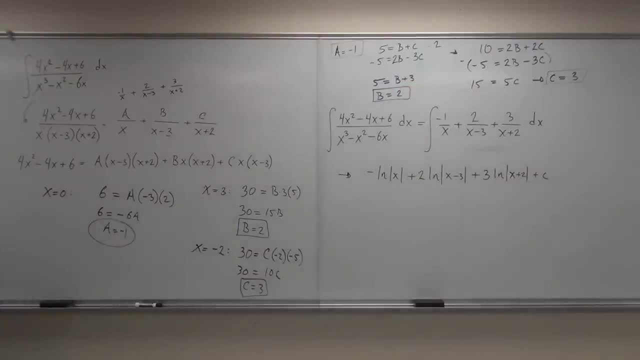 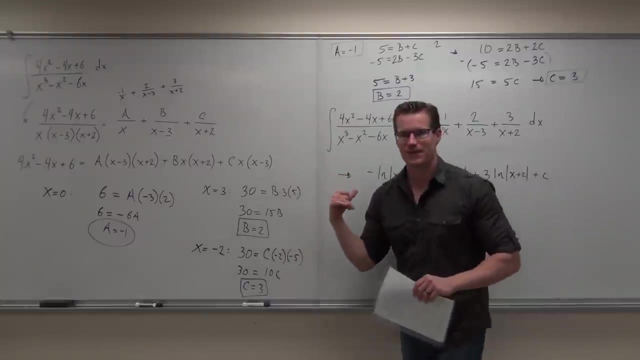 So let's try this now. I'm going to stick with this technique when I can because obviously it's a lot quicker. Well, let's do this. Let's do a different example. Are there any questions on this before I erase it all? Because we're going to need some space for this stuff. You ready? Okay, so new example. 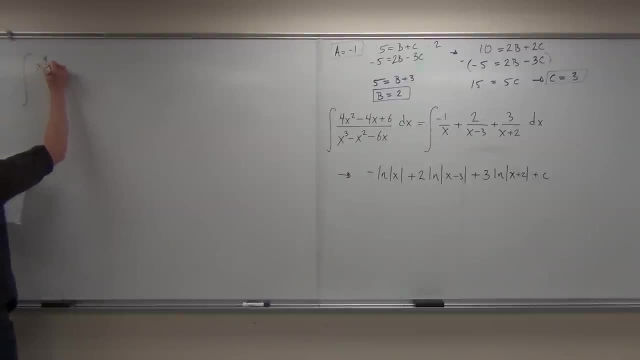 Let's talk about x to the 4th minus 3x squared minus 3x minus 2 all over x to the 3rd minus x squared minus 2x dx. 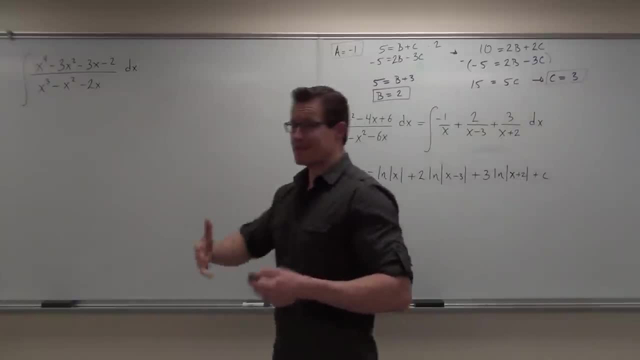 Tell me something about this problem that was different, that is different from the last one that we did. What's different? The degrees. The degrees. The degrees are different. Remember what I told you about algebra? Yes. 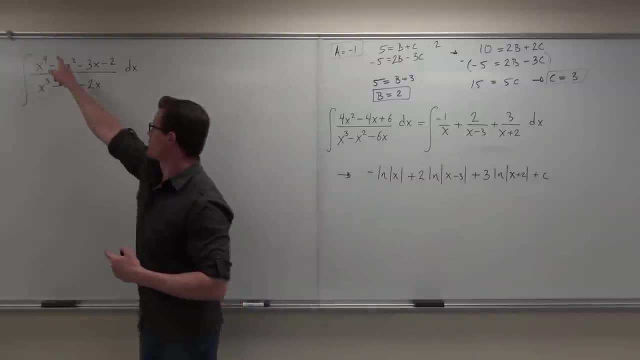 Algebra. Algebra said that if the degree here is less 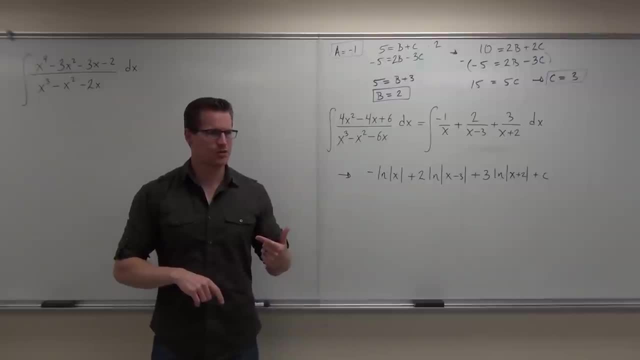 than the degree here, then it can be written as partial fractions. I said if. Is the degree here less than the degree here? No. 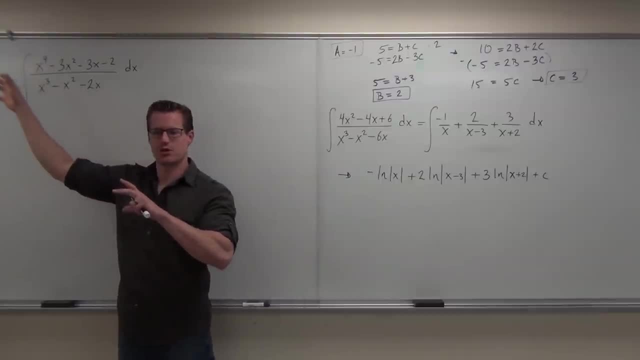 No. If it's, listen, if your degree of your numerator is larger than or equal to the degree here, so if this was even a degree 3, we'd still have to do the following step. 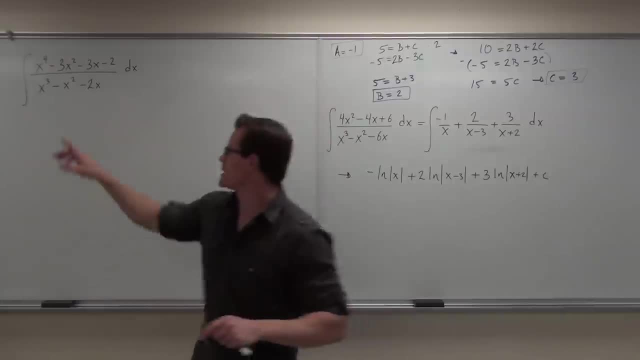 What we're going to do is, shoot, guys, I mean, think about it. If your degree here is bigger than or equal to the degree here, that means you can divide it. 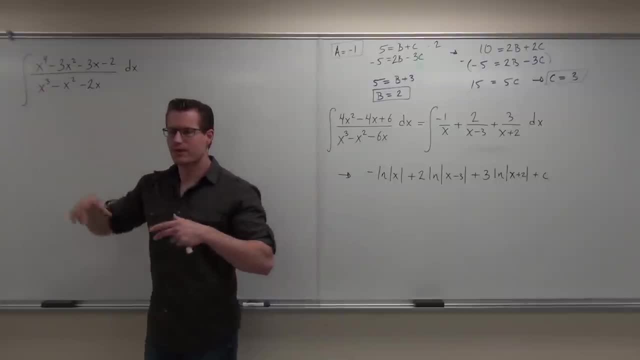 So we're going to divide it by long division, and then what that's going to do is reduce that degree. 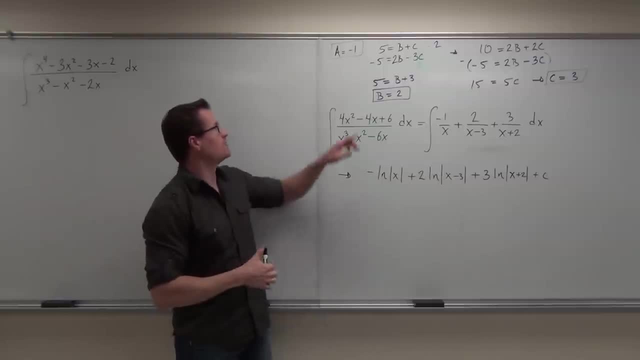 So if you have, like the last example, where the degree of the numerator is less than the degree of the denominator, start immediately, factor immediately and go for it. 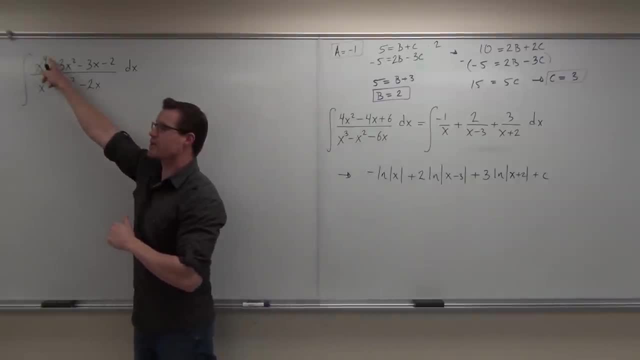 If you have, like this example, the degree here is bigger than or equal to the degree here, then you have to do long division, and then you'll get to start your problem finally. Does that make sense to you? 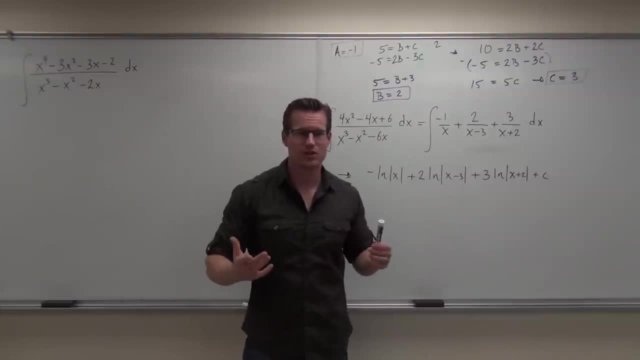 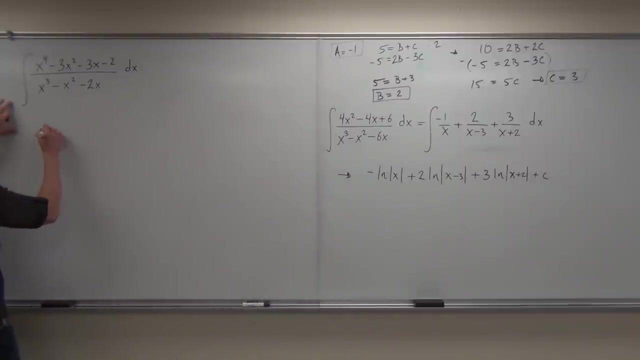 So we're going to do long division. I don't know if you are that good at long division. I'm not sure that you've seen it in a while, but here's how you do it. We are going to go quickly through it. You can refresh your memory if you want to on some of the videos I have for intermediate algebra. That's where we cover it in the appendices of that class. So here we go. I need more space. 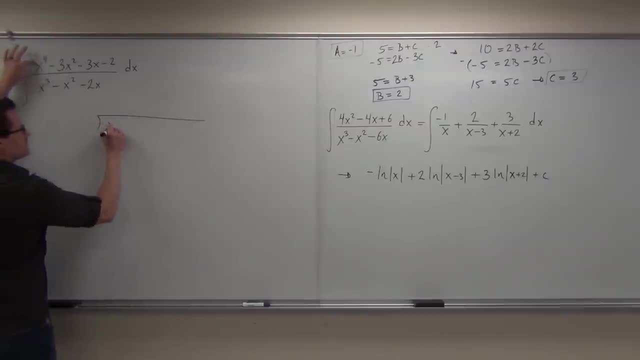 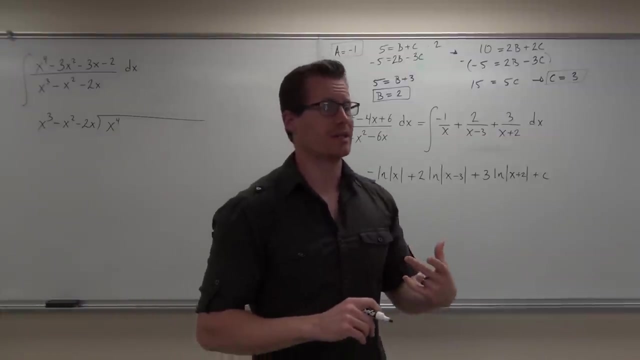 How we do long division of polynomial is we just take our numerator and we divide by our denominator. Now, when you're dividing your numerator, when you're dividing your numerator, please keep in mind, you need at least a placeholder for every potential power of x that you have. So if you do this, look at the board, please. 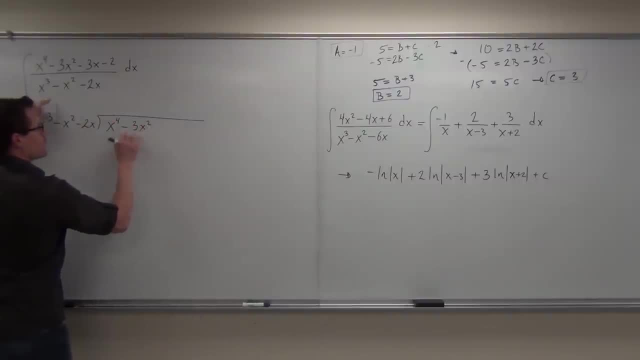 If you do this and just go right on down the line, right here you're going to have an error. 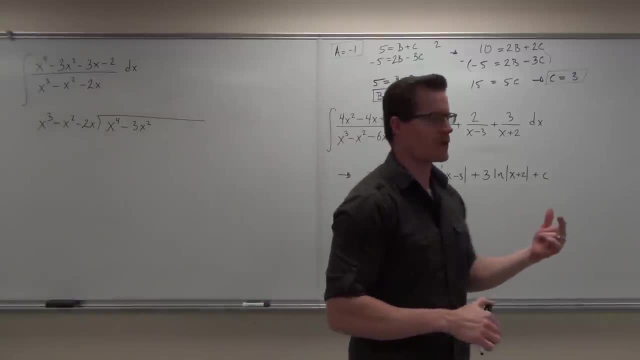 You're going to have a mistake because what happens is when I divide x to the fourth with my x to the third, I'm going to end up getting something here. I'm going to get an x to the third somewhere. 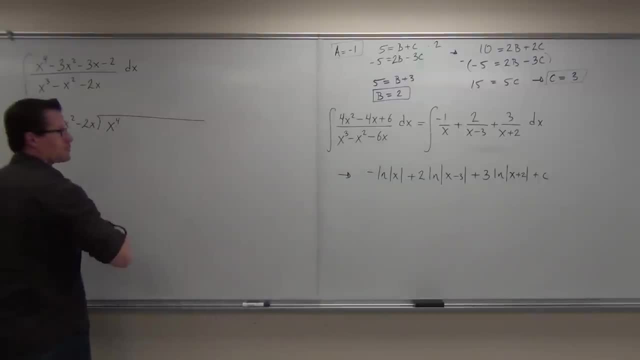 So the problem is? Zero x. Yeah. We're going to put a place. It's like a place value holder saying, hey, how many x cubes do you have? Zero. None of them. Put zero. 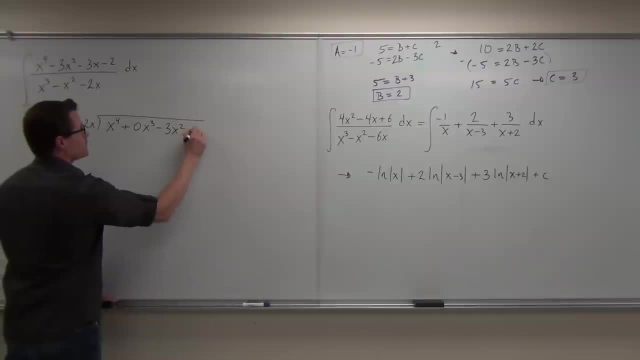 And then finish it off. Minus 3x squared, minus 3x, minus 2. 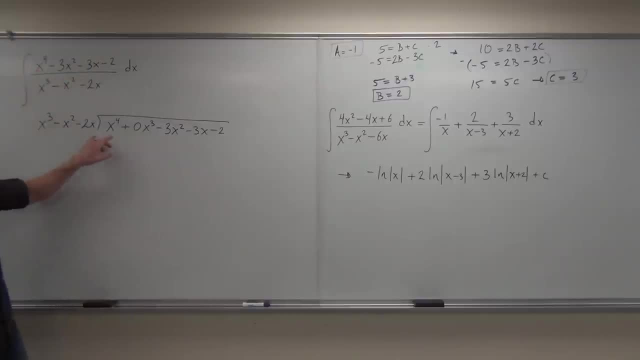 So this is the same as this. We've got x to the fourth, no x cubes, minus 3x squared, minus 3x, minus 2, and this is our denominator. So far, so good? Okay. Let's continue. 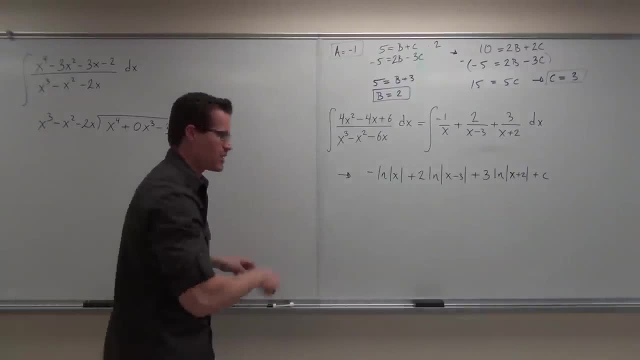 How we start this thing is basically just the first term divided by the first term. 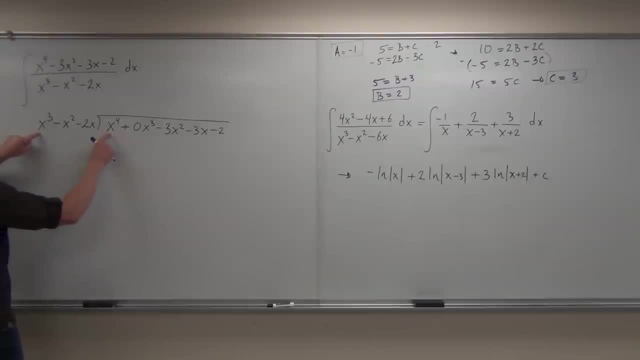 So what do I get when I divide x to the fourth by x to the third? X. 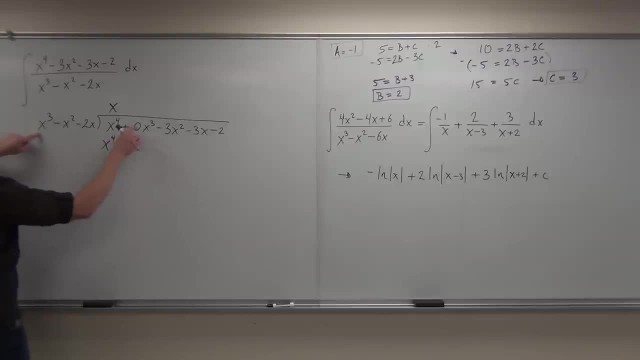 And then we distribute. We get x to the fourth. Check this out. This is why we had to have a place value holder. 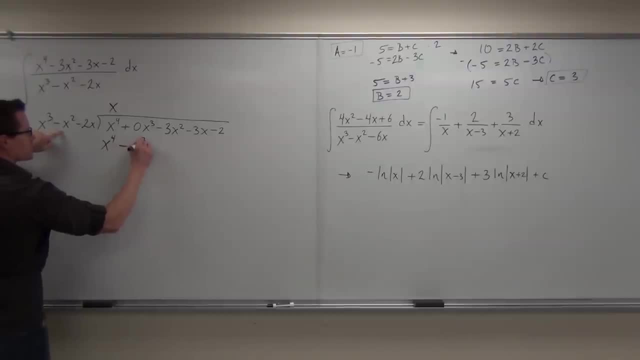 We get negative or minus x to the third, and we get minus 2x to the second. 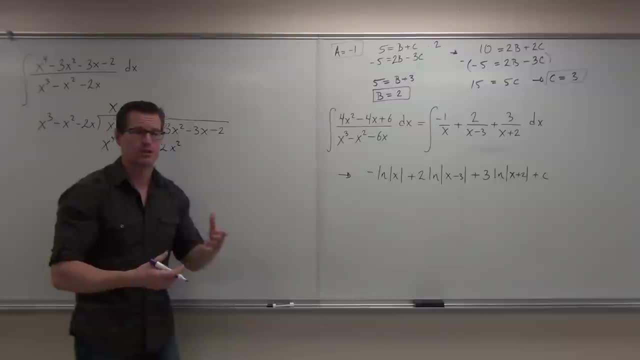 It's got to match up. If it doesn't match up, then you've made a mistake. You forgot a place value holder somewhere. 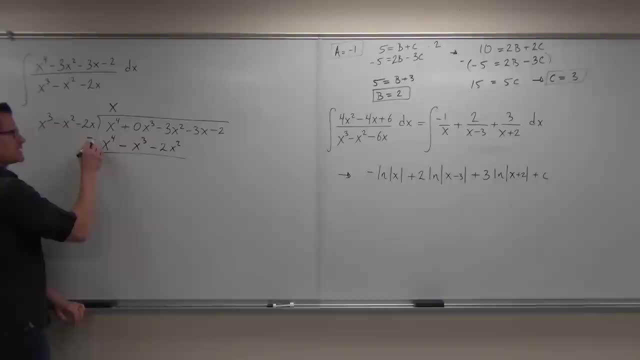 After that, what do we do? Change signs. Yeah. We're subtracting. You either put parentheses here, or you subtract and you change all the signs. I like the parentheses to show what I'm doing. 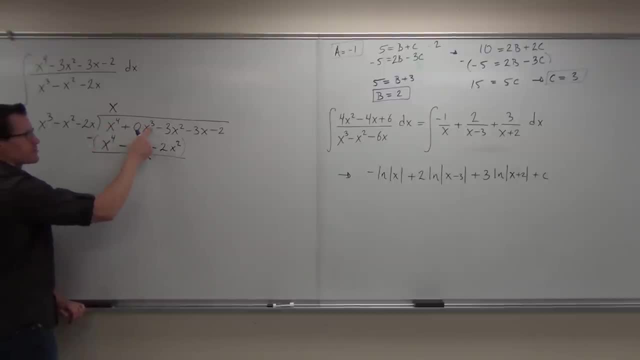 X to the fourth minus x to the fourth is zero. Zero x to the third minus negative x to the third. You can change your sign and make that a plus if you want. 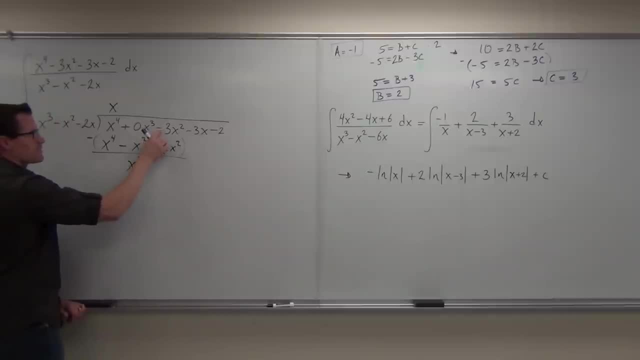 This will be positive x cubed. This will be negative 3x plus, sorry, negative 3x squared, 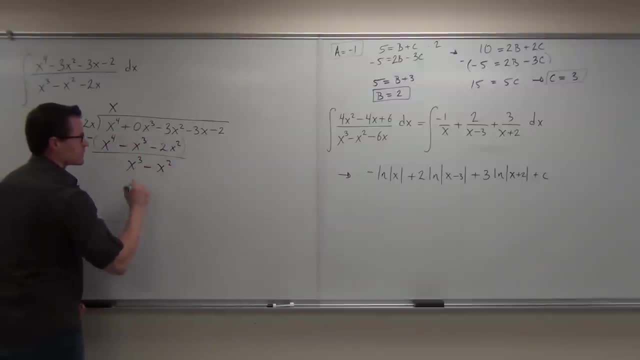 plus 2x squared is negative x squared. And then we bring down our next term. 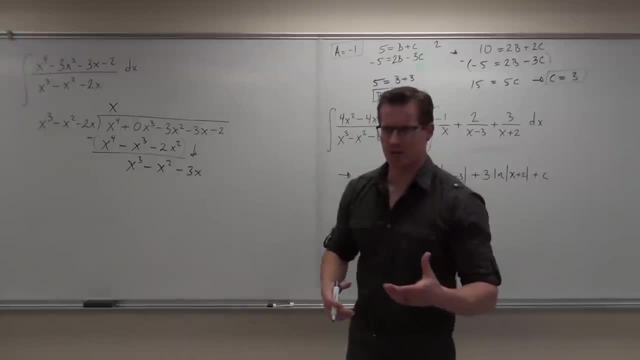 Yes, I'm going fast, but you should know at least a little bit how to do this. Are you all still with me so far? Yes. Okay. And we start over. 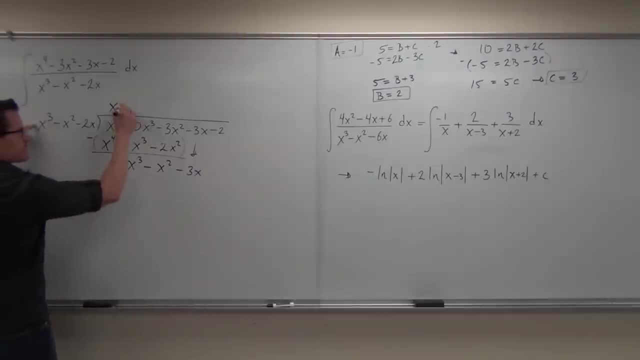 How many times does x to the third go into x to the third? One. That's positive one, so we'll put plus one. And then we distribute. We get x to the third minus x squared minus 2x. Again, we are subtracting. Again, we'll have parentheses. You either change signs or do it in your head. 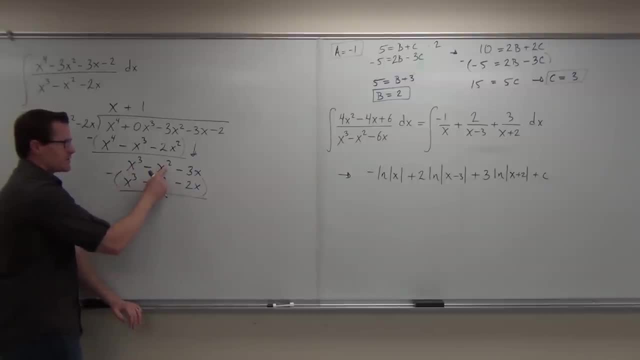 I do it in my head. X to the third minus x to the third is zero. Negative x squared plus x squared is zero. 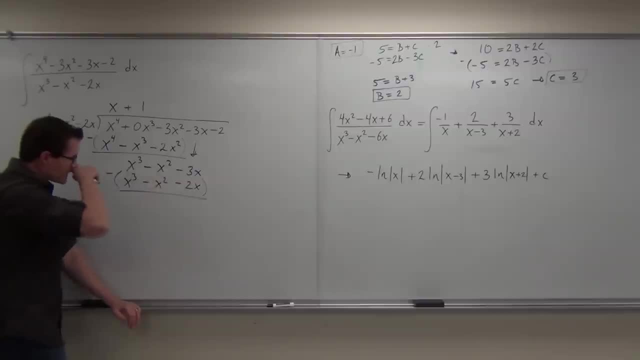 Negative 3x plus 2x is? Negative 3x. And we bring down our minus 2. And we check again. Does x to the third go into x? No. 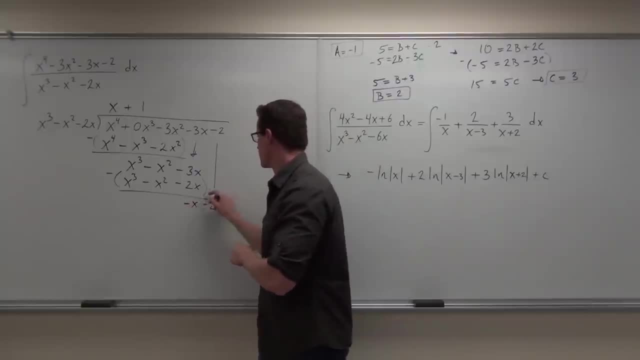 Then this is our remainder. That's our remainder. Here's how you write your remainder. 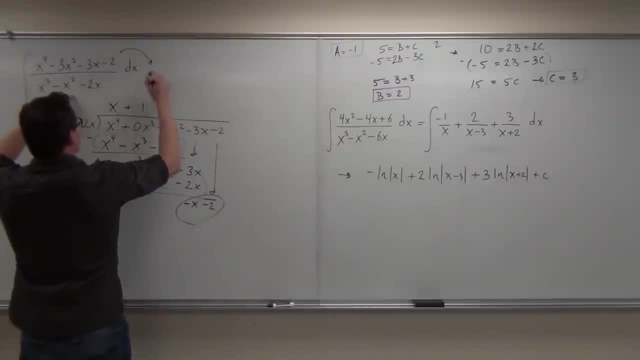 What this says is that this fraction, in this case, is negative 3x squared. It's the same thing as x plus 1. This is our quotient here. 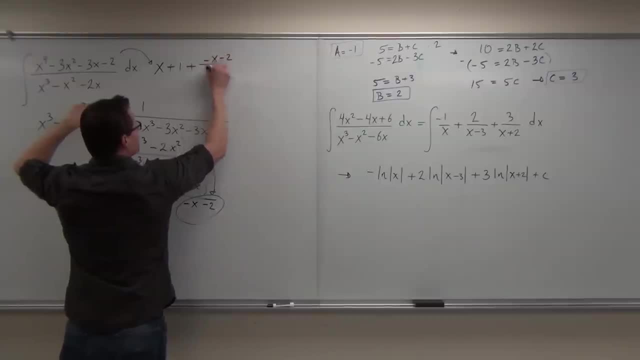 Plus the remainder of negative x minus 2 over. And when you write your remainder, it's always as your remainder over your original denominator. Are you okay with that so far? Just don't. Don't make the silly mistake of doing this. 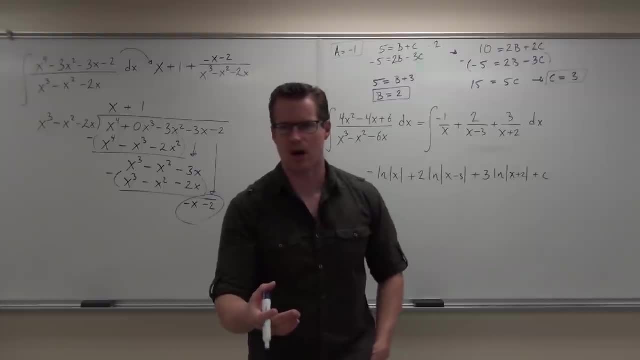 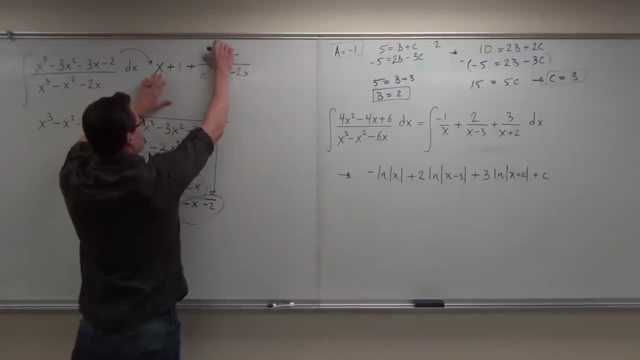 Please let me have your eyes on the board right now so you see this. A lot of mistakes here are not calculus mistakes. They're sign mistakes. They're sign errors. If you do this and you go, oh, look at that. Minus. Mr. Lawrence is silly. Why don't you just put minus? 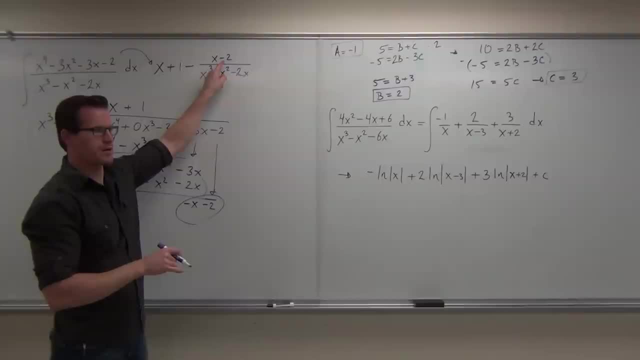 I don't put a minus there because this sign is wrong right now. Do you know that? That's incorrect. 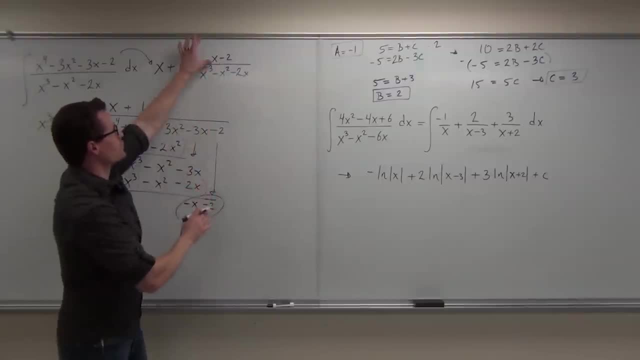 So what I'll do is I'll put a plus with my negative. I'll put this on the numerator. I'll put my plus sign there because you can always add but later. So here's what you'd have to do to change a sign. 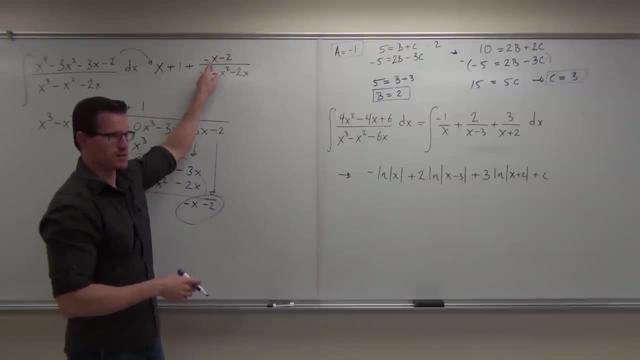 You'd actually have to factor out your negative here. Does that make sense? If you factor out your negative, this becomes negative x plus 2. And that's something that we can deal with. 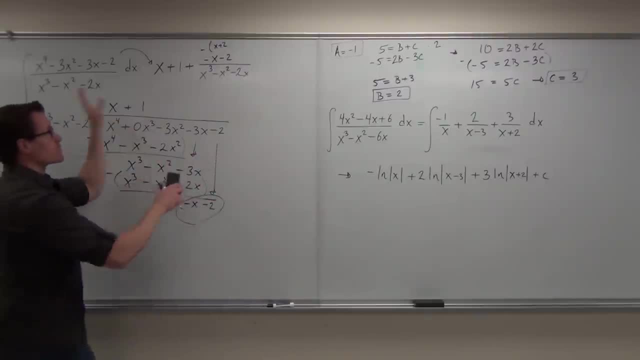 So I'm going to, any questions on long division at all? Okay. So this is what we get. 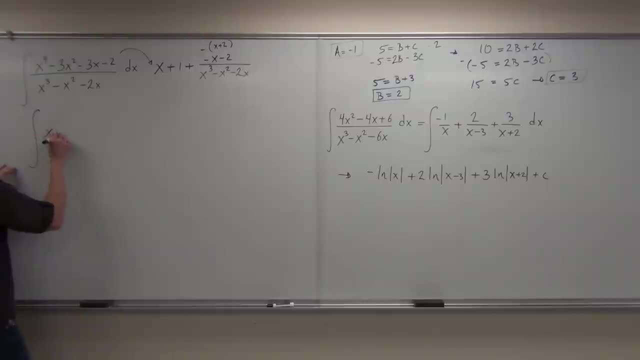 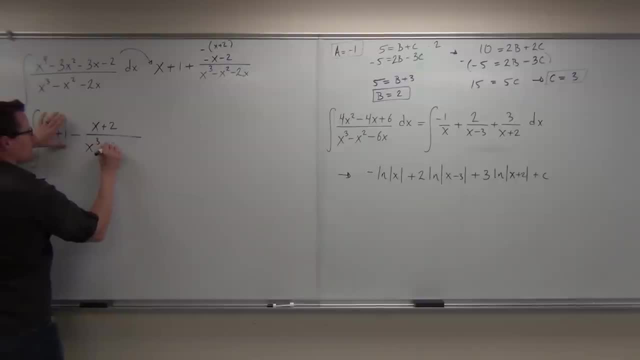 Minus x plus 2 over x to the 3rd minus x squared minus 2x, dx. 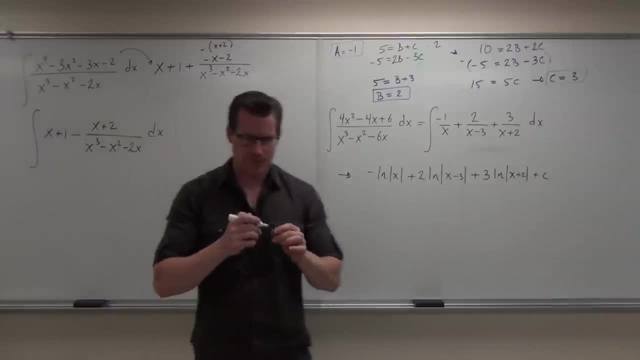 So we do long division. What long division does, long division is kind of nice with this. 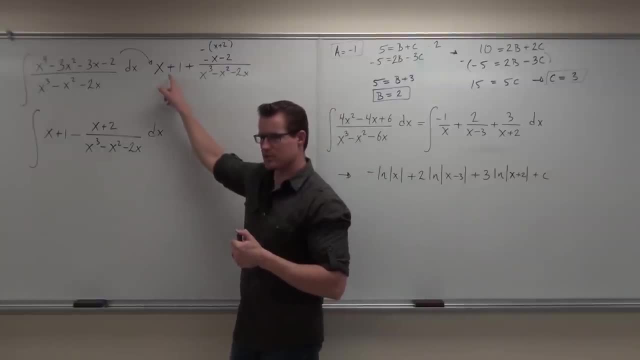 Look at this. It pulls out some terms, some terms here that are really easy to integrate. We got an x. Can you do the integral of x? Can you all do the integral of x? It's a piece of cake. Can you do the integral of 1? Absolutely. 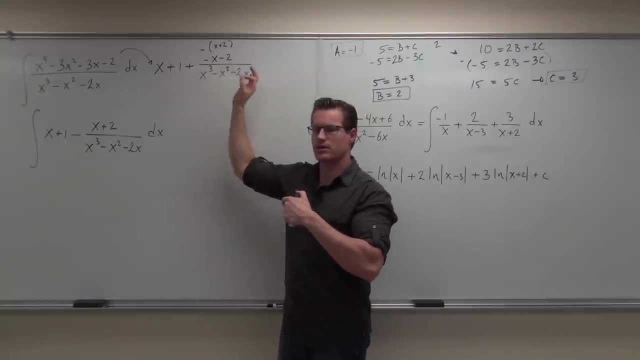 And then it gives us a fraction where the numerator, the degree of the numerator has been reduced. 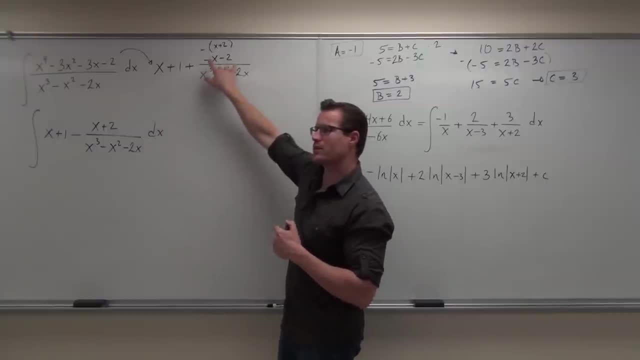 And that's the idea of division. So our remainder here is what counts. Our remainder is what makes this process a little doable for us. We have this remainder of negative x minus 2. Factor out the negative before you change that sign. That is a must. You have to do that if you have a negative there. So if you're okay with that. 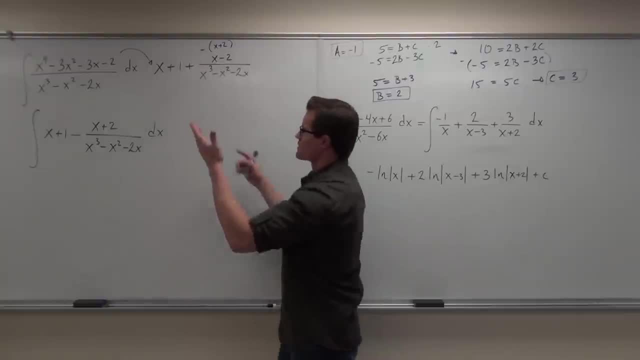 If it wasn't, if it was just a positive x minus 2, that's fine. 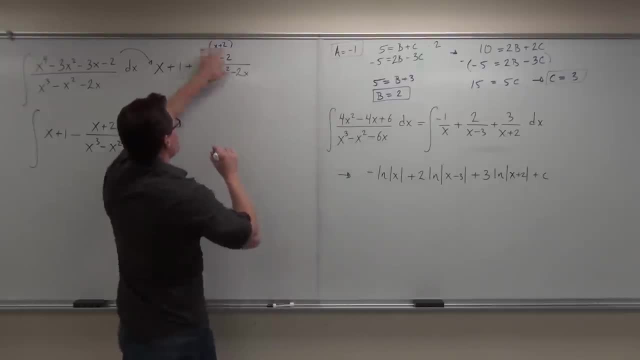 Leave it as plus. You're good to go. But if that's a negative sometime, then oftentimes I'll factor that negative out. It makes it a little bit nicer to see. Can we move on? 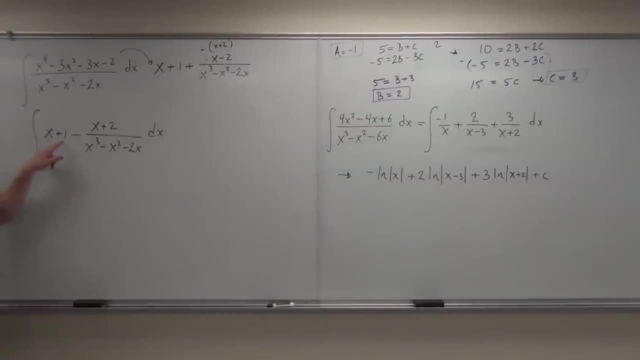 So what are we going to do about this thing? Easy, easy. Maybe split up your integral and see what's going on here. 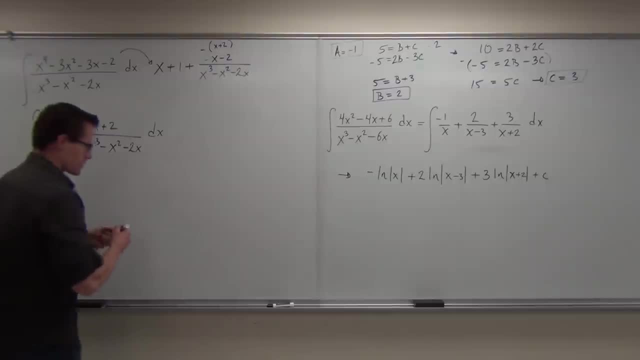 So that's what we're going to do. I'm going to take and make a little asterisk here on this part. 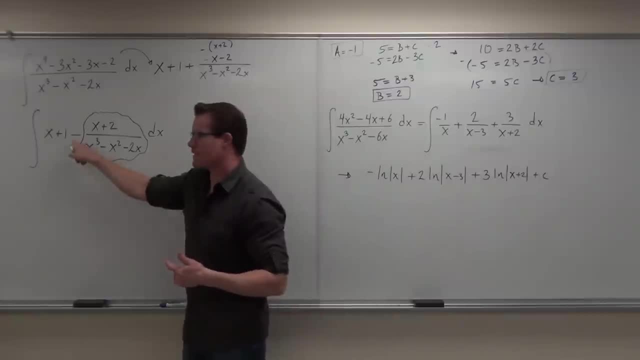 I'm going to keep the negative here. Now don't lose track that you have a minus. When you have a minus, whatever we get, listen please, whatever we get, is going to be in a bracket. This minus we're going to treat like a negative 1 being multiplied onto that bracket. It's going to change all of our signs. 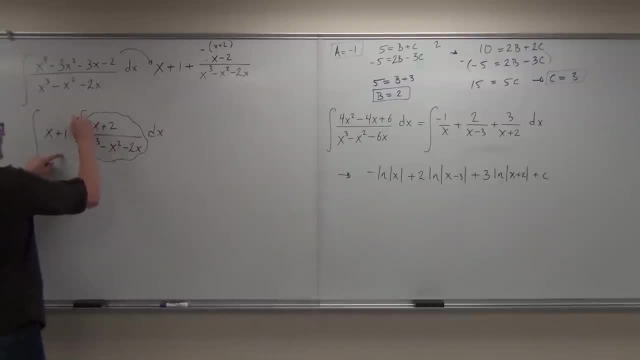 Are you following me on this one? So you can think of this, put a circle or put a big bracket right now. That's what I typically do. 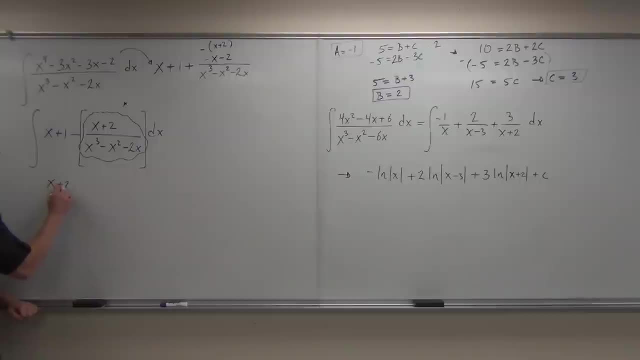 And we'll pull this off to the side and we'll work with it. So here's our piece right here. At the same time, maybe we can factor this guy. Let's factor this. What factors out of x cubed minus x squared minus 2x? If we got that, we got x squared minus x minus 2. Can I go further? Yes. 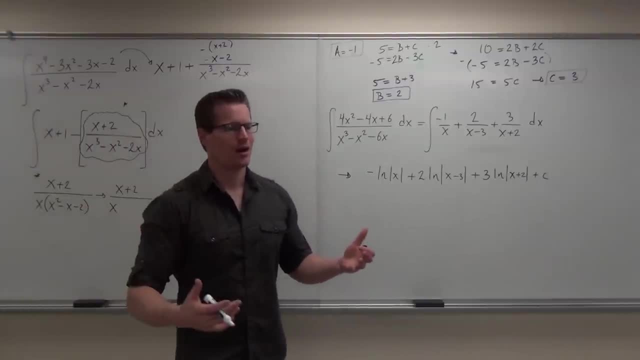 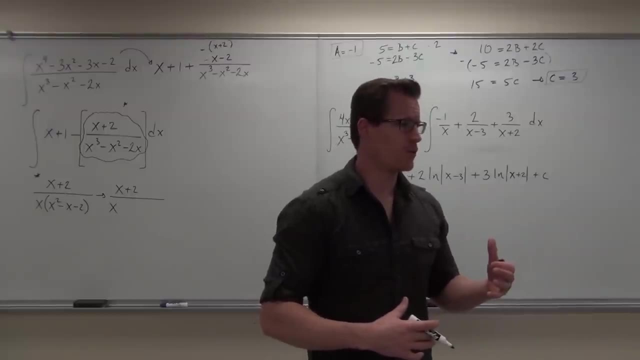 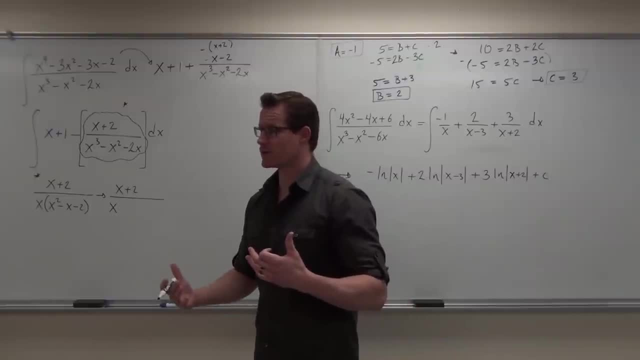 If you do a discriminant, it's negative. That means you have a complex root and that, therefore, it can't be factored. So you'd prove that or you'd at least go through it in your head. Now, this can be factored. What is it? It's minus 2x, this one. 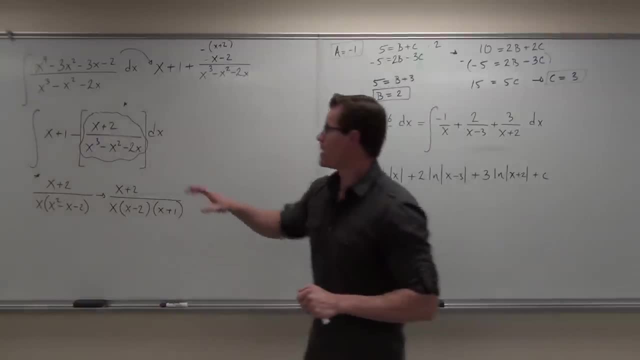 Okay. We've done a lot of work so far, but I want to make sure that we're good. So we start the problem off. We look at it and we go, oh, degree is not less than this one. 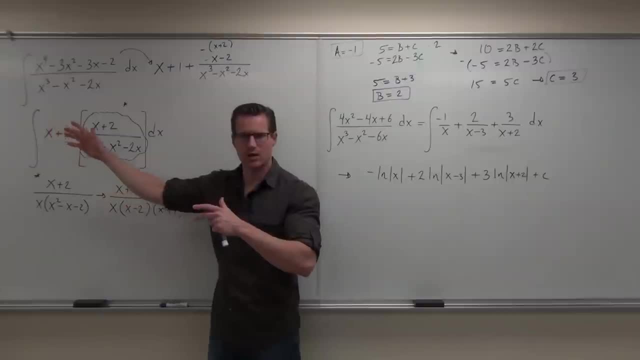 That means long division. I've done long division. I erased it, I know. 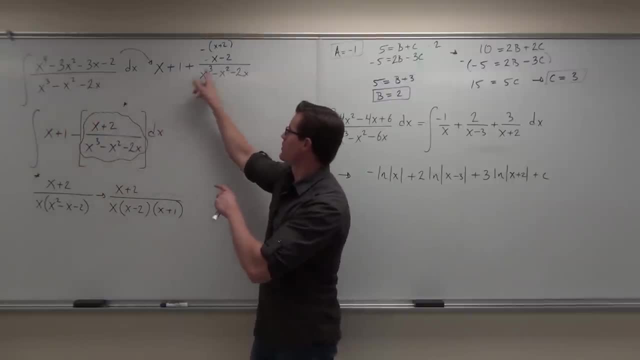 We do long division. This is our quotient of long division with our remainder of long division. 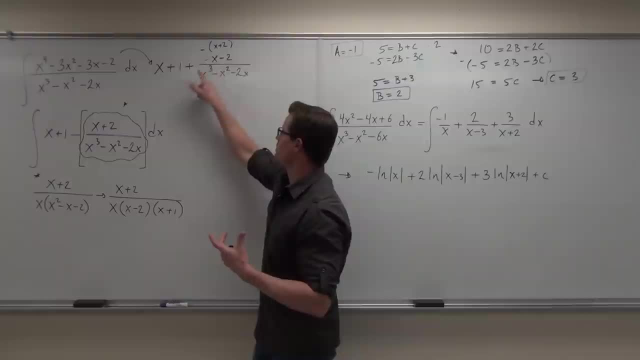 How you write out your quotient is you always write quotient plus remainder. If we have remainder over our first denominator, this denominator, then if it's a negative, maybe factor out the negative. 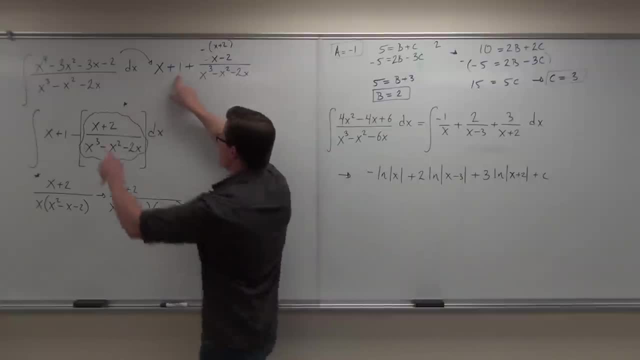 It changes it to a minus, so we get x plus 1 minus x plus 2 over our original denominator. 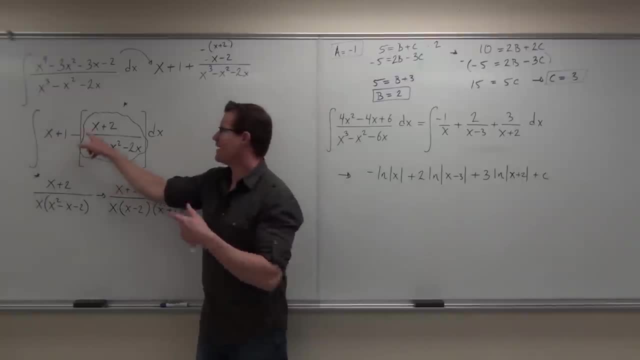 And now, easy, easy, is the degree less than the, the degree of the numerator less than the degree of the denominator? Yes. 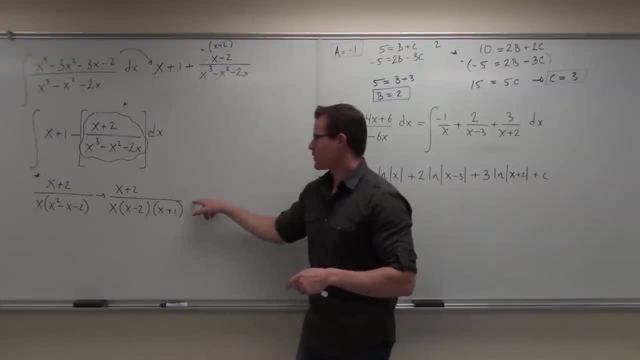 Now we can go ahead and do this. What I want you to do right now, I want you to write out what this should be equal to. Make your different fractions, however many that you need, and put the appropriate letters up top. 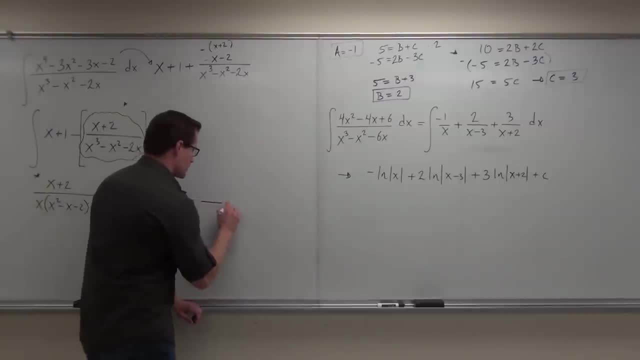 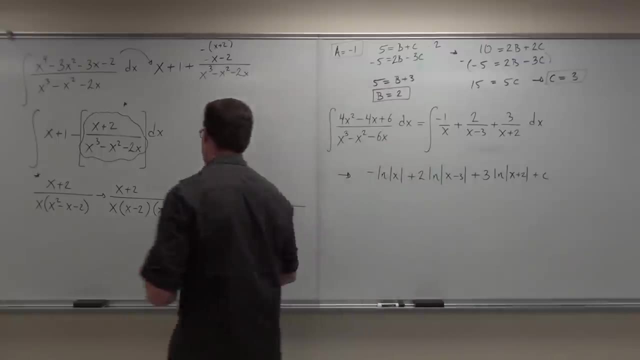 How many fractions are we going to get? Three. However many different linear factors you have, that is how many different fractions you end up getting. 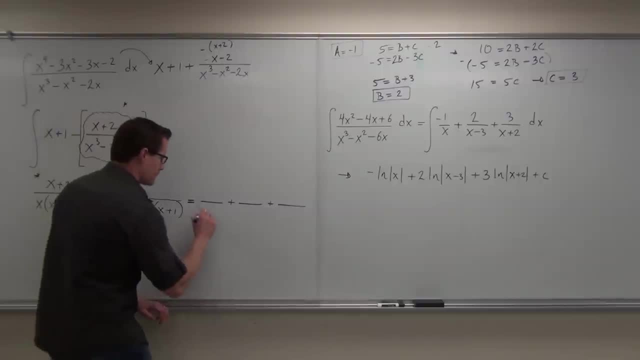 What's going to be our first denominator, please? A, b, and c. Denominator. X. X. And then? X minus 2. And then? X plus 1. 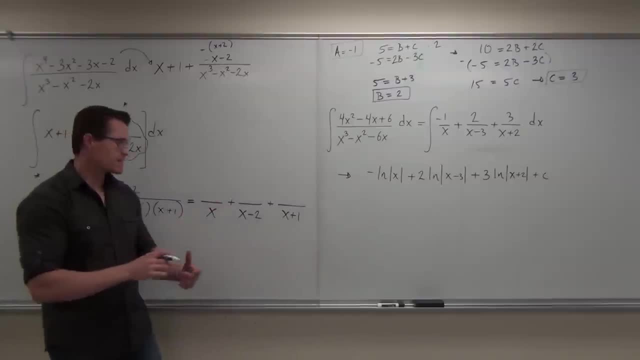 Does it matter which order you have these in? So if you factor this, well you can't factor it differently, but if you have your factors out of order compared to this one, no big deal. 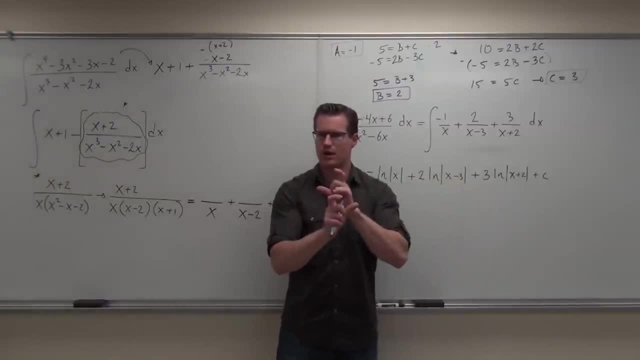 You're going to do the same thing. It's just your pieces of your integral will be a little switched around, all right? Same idea, no problem. 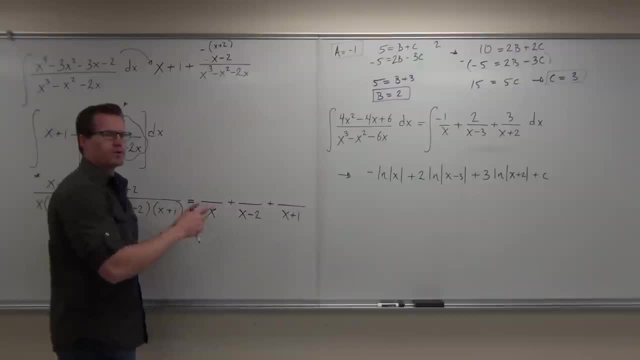 All additions, commutative, so we're good. What's going to be on our numerators? What's this going to be? A, b, and c. 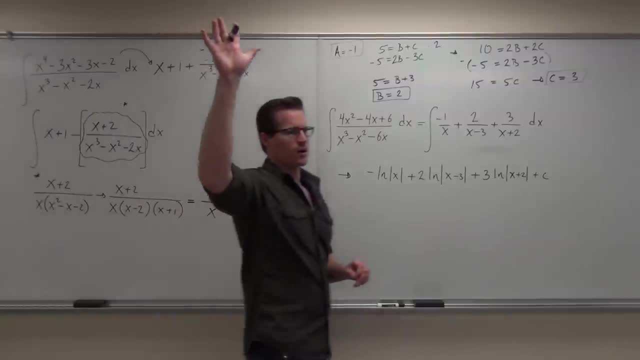 So fans feel okay with this so far? We've done a lot of algebra, huh? Have we done any calculus? No. We're not going to for a while either. 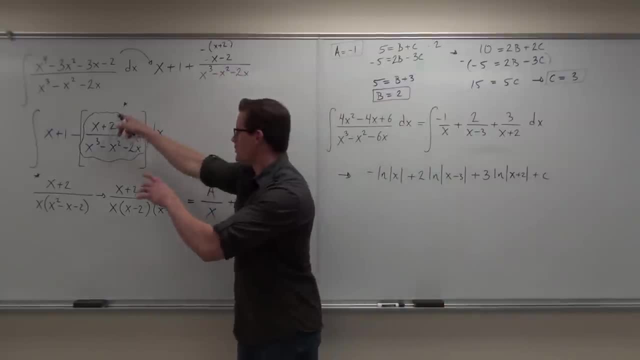 So we got long division, check it. We got this, no problem. 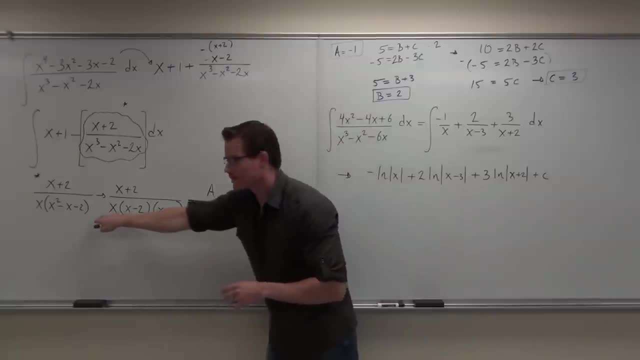 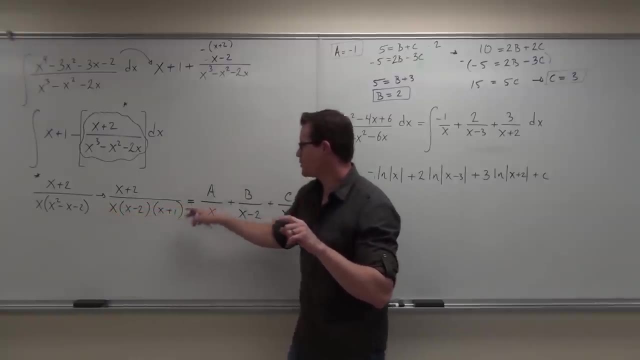 Partial fractions, we have it all set up. Remember that when you have linear, linear is power 1. When you have linear factors, we make a fraction for every different factor, and we put constants up top, a, b, c, and so on and so on and so on until we exhaust all of our distinct factors. So we get linear factors. Still okay so far? 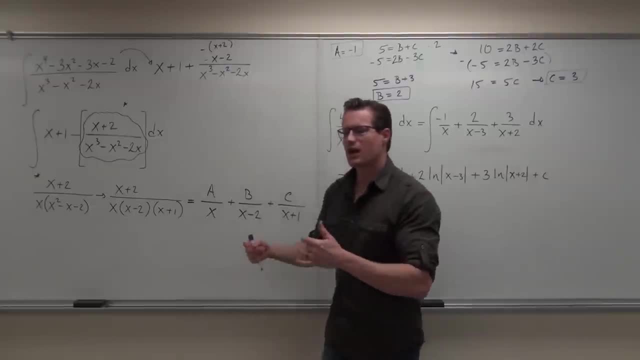 Now, go ahead, I want you to do this on your own. Create the common denominator. Use the cover-up method I taught you last time. So what I want to see next, I don't need to see one fraction equal to one fraction. 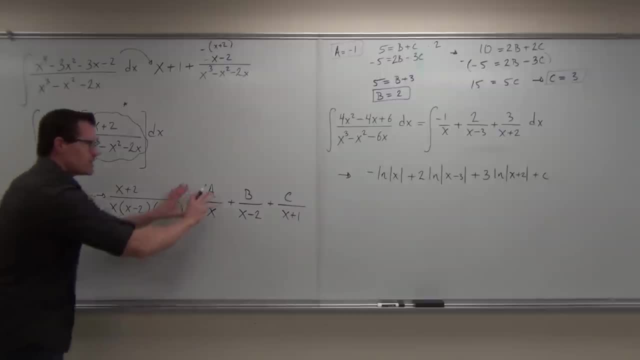 I want to see x plus 2 equals, and then just give me what this is equal to. Go for it. 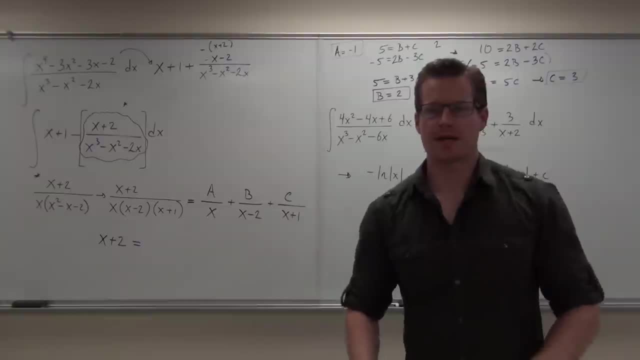 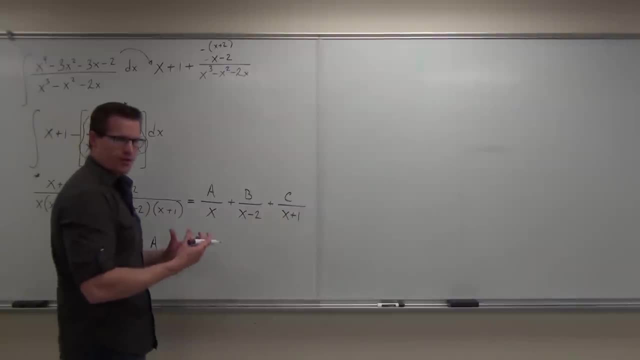 If I find a common denominator, what that is, is that you end up multiplying each fraction by the missing factors in your particular denominator. So here, I have a factor of x, I'm missing a factor of x minus two, I'm missing a factor of x plus one. 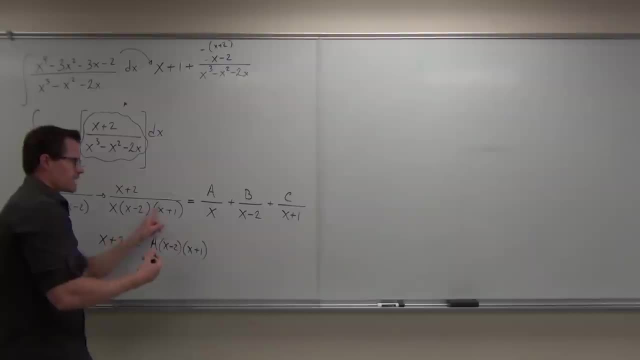 For b, in order to create a common denominator, I have the factor of x minus two, I have it already. 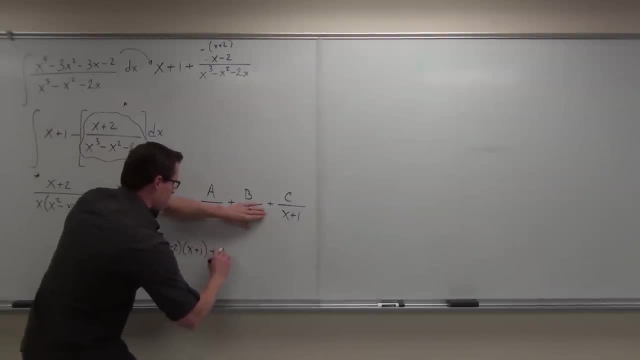 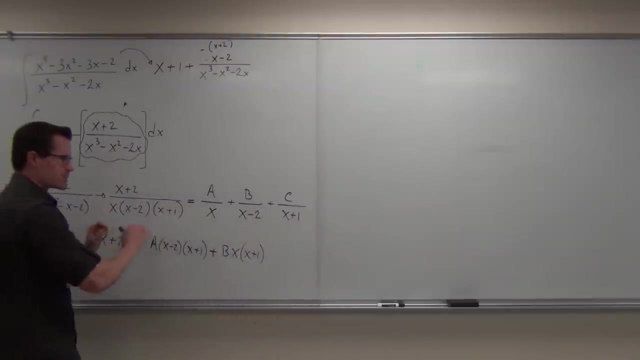 I'm missing the factor of x and x plus one. So we have plus b times x and x plus one. Just the missing factors of your LCD, of your common denominator. 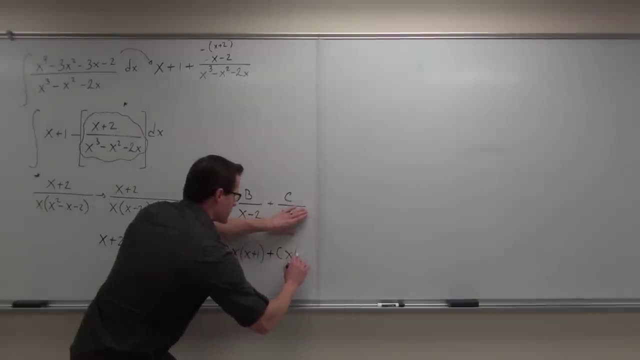 Lastly, we got plus c, I'm missing x, and I'm missing x minus two. 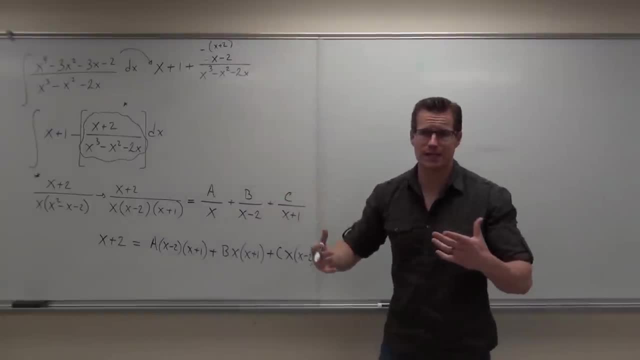 Show of hands if you got that far on your own. Good, that's fantastic, that's the whole idea. Now, can you find a, b, and c by plugging in some different numbers? 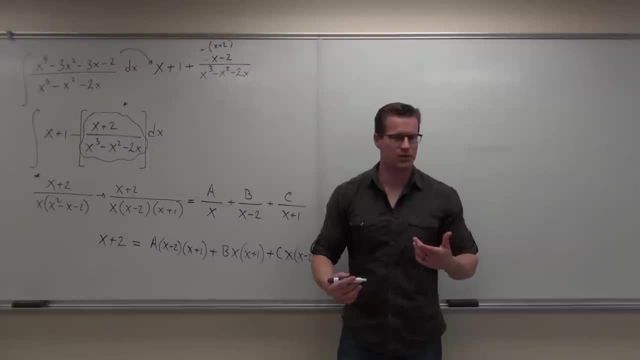 Hello, can you do that? Tell me the three numbers you'd probably plug in here. 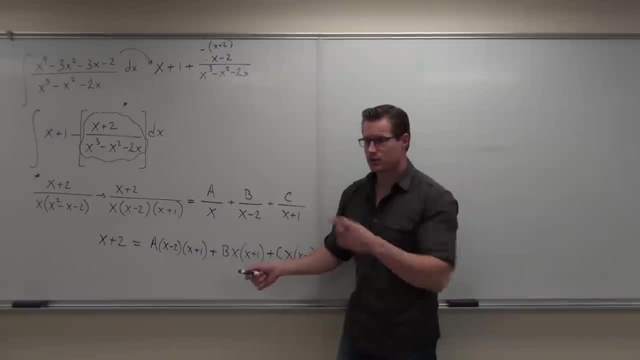 Zero. Zero, for sure, and then what? Negative one. Two would be one, and then the other one? Negative one. Yeah, plug those numbers in. If you haven't done it already, go ahead and do that. 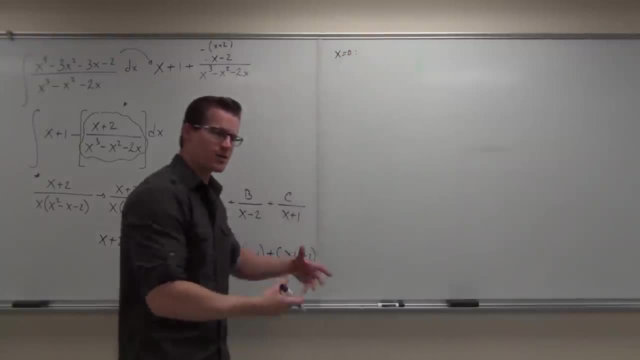 So when x equals zero, that's nice. Some of your factors are gonna go, some of your terms, actually. 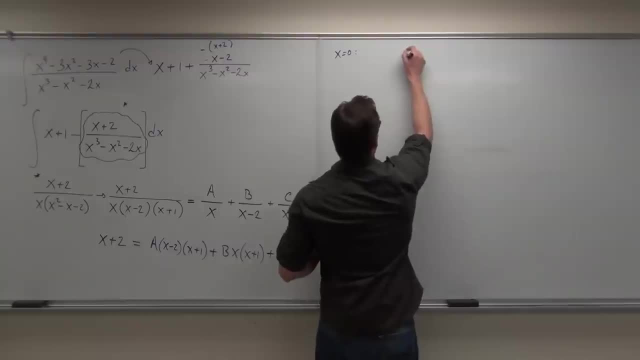 Some of your terms are gonna go to zero. When x equals two, some of your terms are gonna go to zero. When x equals negative one, some of your terms are gonna go to zero. 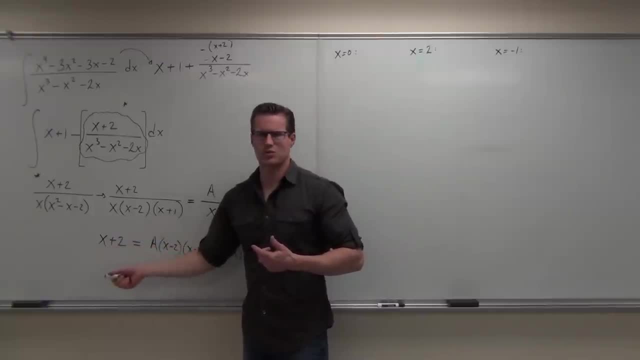 Fortunately, man, you gotta, this is nice to plug stuff into, right? There's a square over there, that's beautiful. 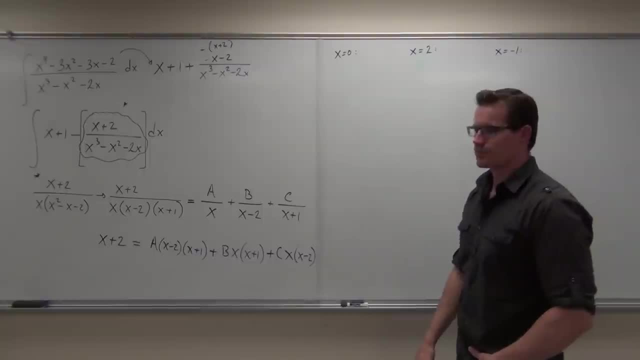 I'm gonna start working on this for the sake of time, but I wanna know if you guys understand the idea here. 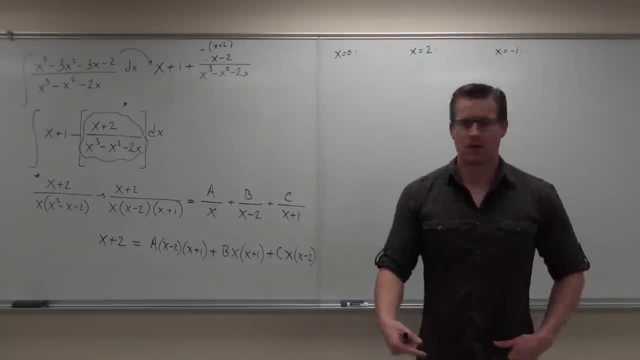 So we're checking for numbers that change some of your factors to zero. If your factors change to zero, some of your terms are gonna go to zero. 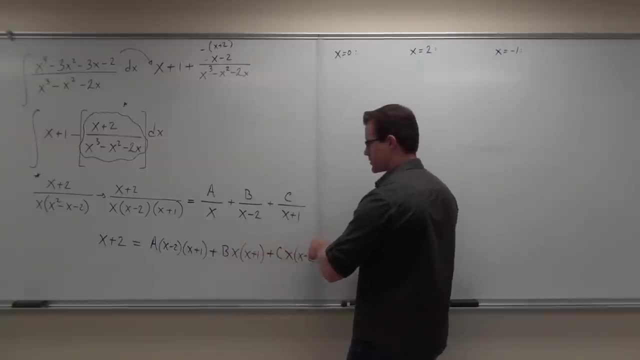 So when I plug in zero, start from the left. Zero plus two is two. 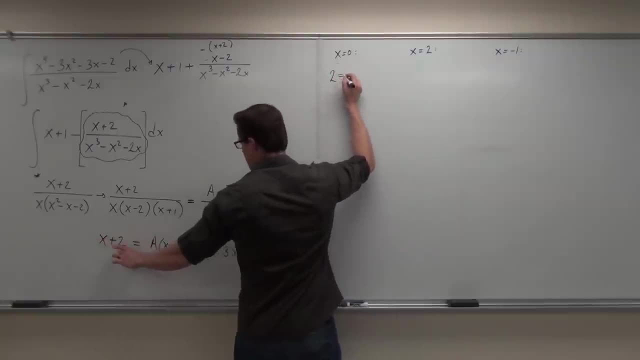 A, okay, if I plug in zero here, I get negative two. So I'm gonna plug in zero, and I'm gonna plug in negative two. I'm gonna plug in negative two. I get negative two, and I get one. 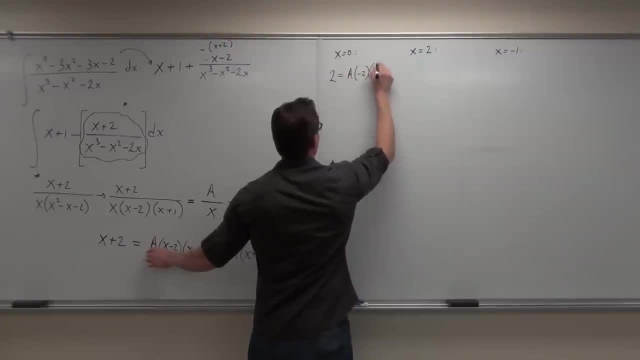 So this is A times negative two times one. Plus, well, that's a zero now, I'm plugging in zero. This goes to zero, this goes to zero, I'm good to go. 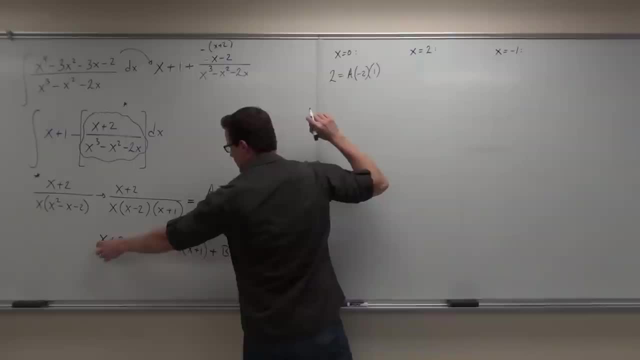 Now let's plug in two. If I plug in two, don't forget, you have to actually plug it in here. 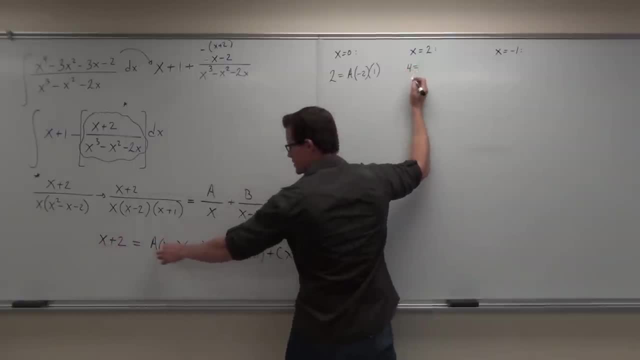 Two plus two is four equals, if I plug in two, two minus two is zero, this whole term is gone. 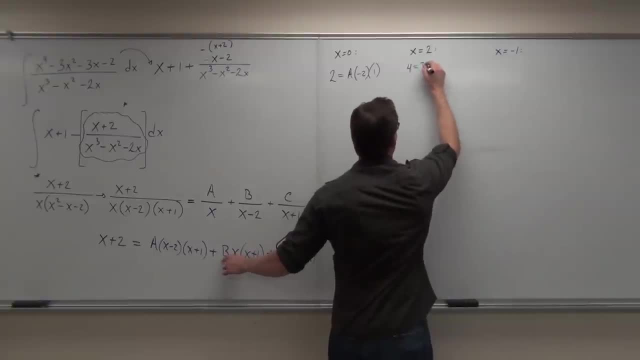 Two minus two is zero, this whole term is gone. I get B times two. 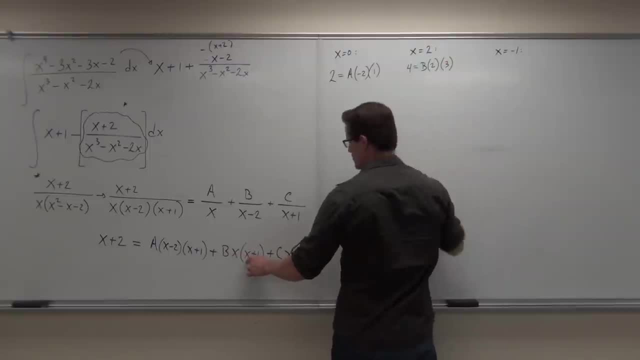 B times two times three. Did you get two times three? B times two times three? Yes. Good. Lastly, if I plug in negative one, remember to actually plug it in. 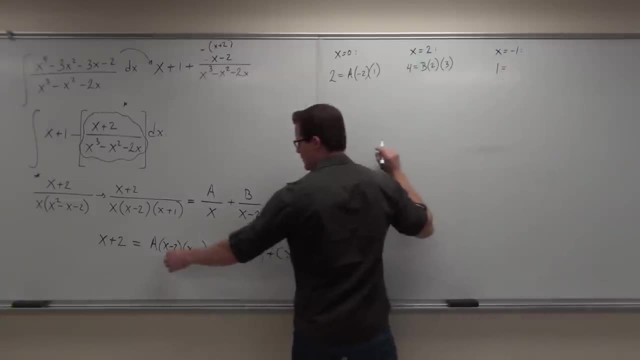 Negative one plus two is? One. 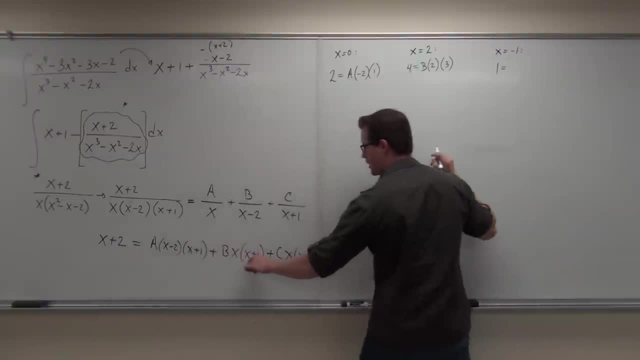 If I plug in negative one here, this is zero. Whole term gone. This is zero, whole term gone. 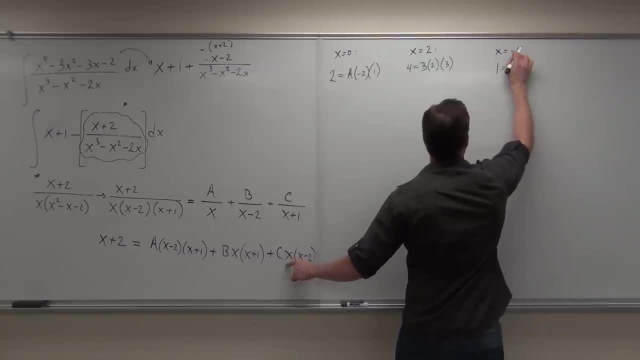 This is not zero. I get C times negative one, that's what I'm plugging in, times negative three. You should know the answer if you made it that far. 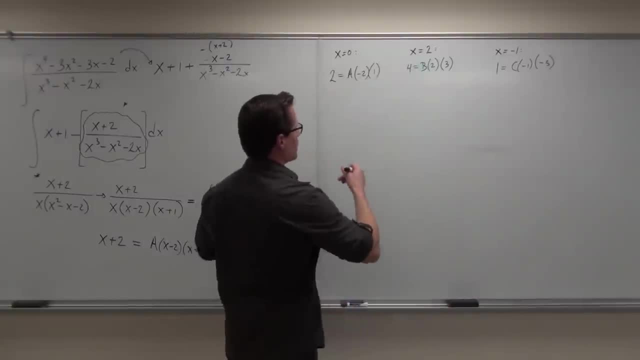 Good deal, now we're almost done here. So, simplify it a little bit. 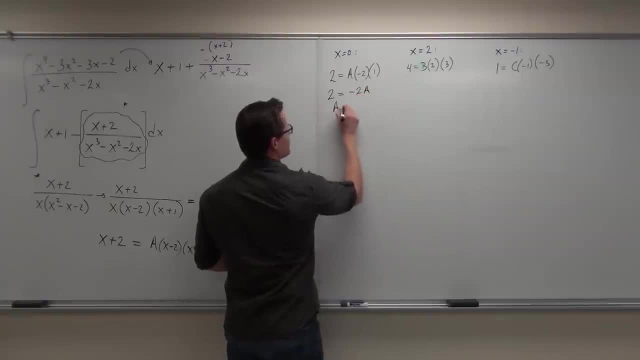 Two equals negative two A, therefore A equals how much? Negative one. 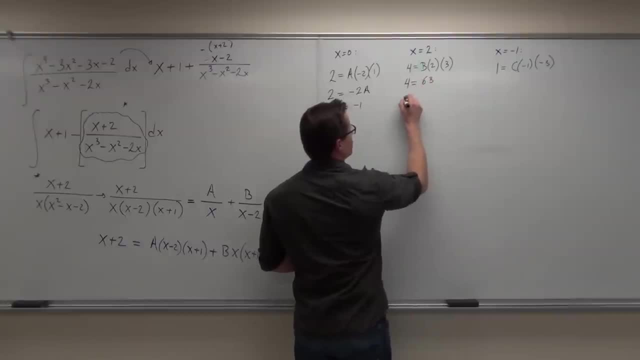 Four equals six B, therefore B equals how much? Two-thirds. Is it okay to get a fraction? Yes. Don't worry about it. 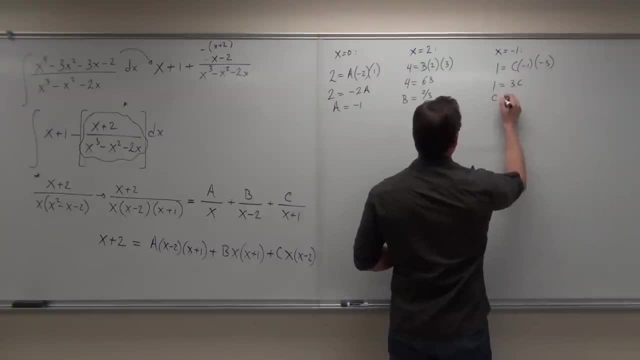 One equals three C. C equals one-third. Hey, look at that. 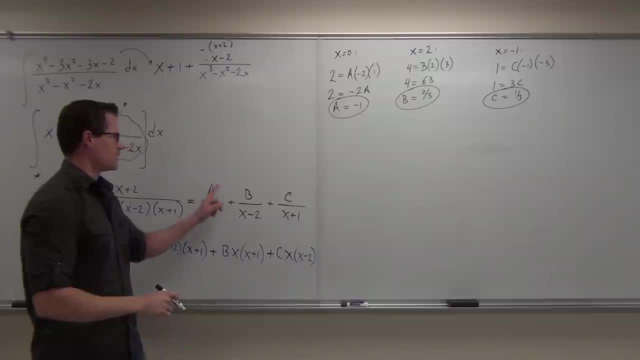 Those were the three constants I was looking for. A, B, and C. 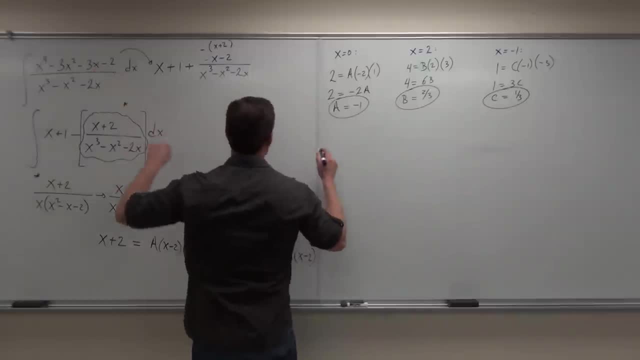 What that means is that our original, actually right here, our original integral changes to this. Please watch very carefully on how I do this. 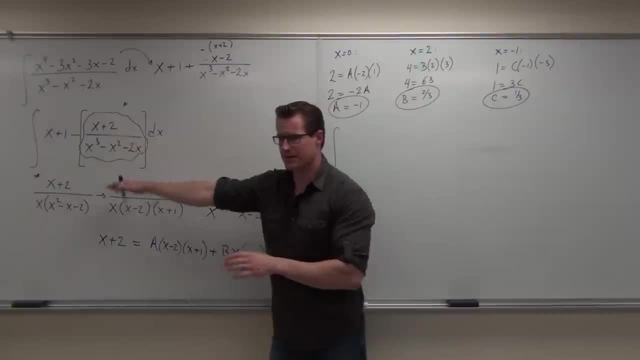 I want to make sure all our signs are correct. You guys are okay to this point, right? Did this make sense to you? 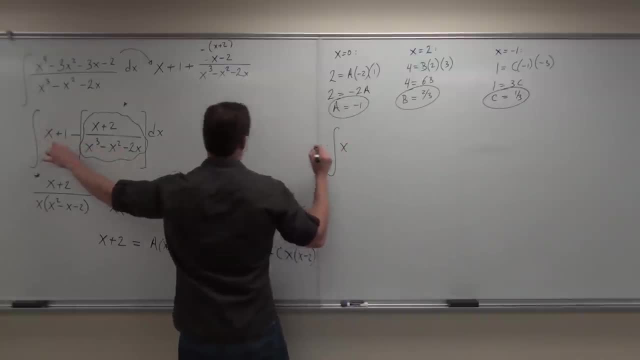 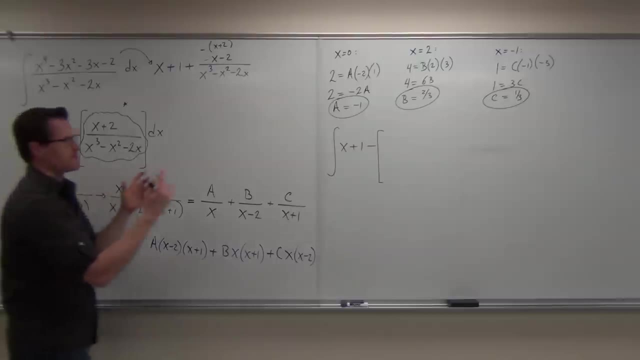 What I know is that our integral is X. Don't forget about this stuff. Plus one minus, I put my big bracket, so this should look identical. X plus one minus. Big bracket. Now inside that big bracket, we just did a partial fraction of this thing. 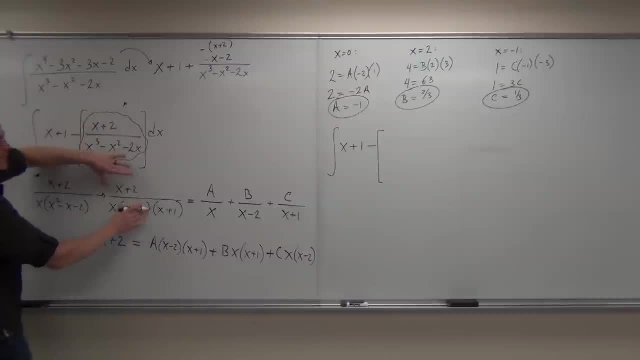 What I know is that the partial fraction of this thing right here equals A over X plus B over X minus two plus C over X plus one. Do I have my A, my B, and my C? Yes. 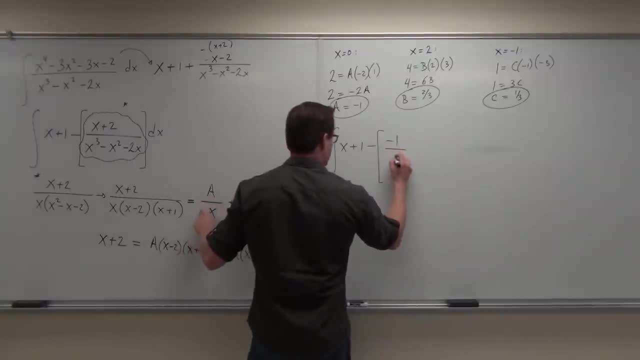 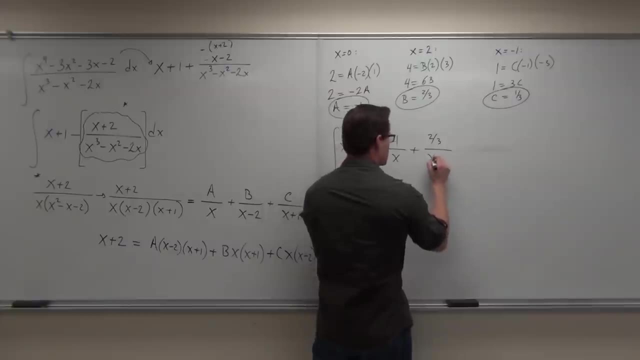 Then what this is equal to is negative one over X plus, just do the fraction like this. Two-thirds over X minus two. Don't worry about that. 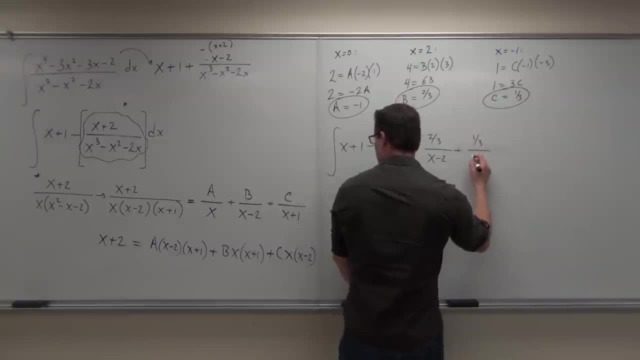 What's that? Plus one-third over X plus one. 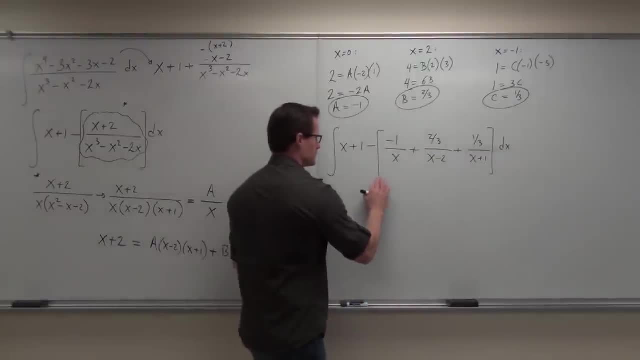 Dx. That would be the bracket. 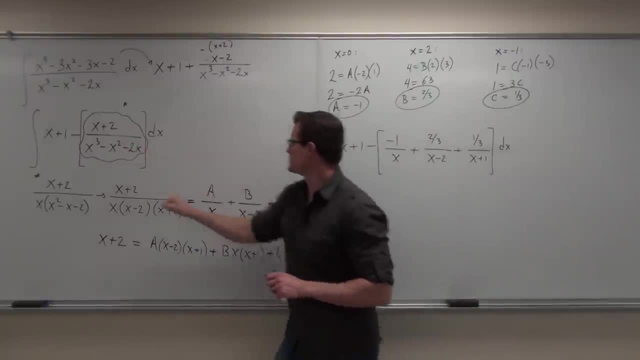 Let me double check to make sure you guys are good with it. Do you see how this becomes these three fractions? 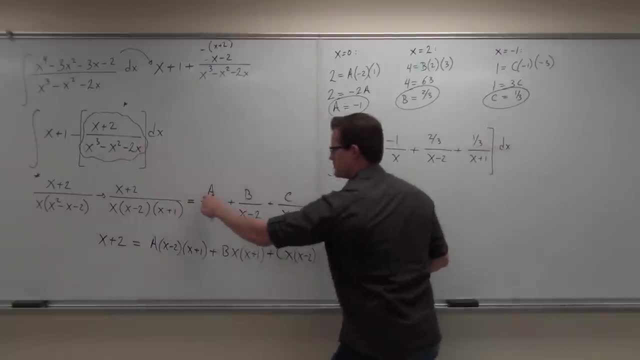 Yes. We found A, B, and C, right? So if we know this is equal to A plus B plus C over these relative denominators, we got negative one over X. Good. 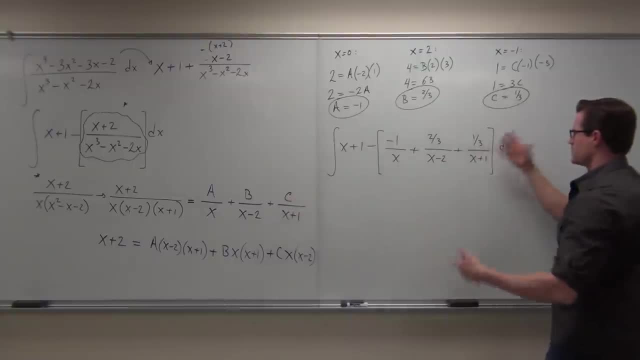 We got two-thirds over X minus two. Got it. We've got one-third over X plus one. 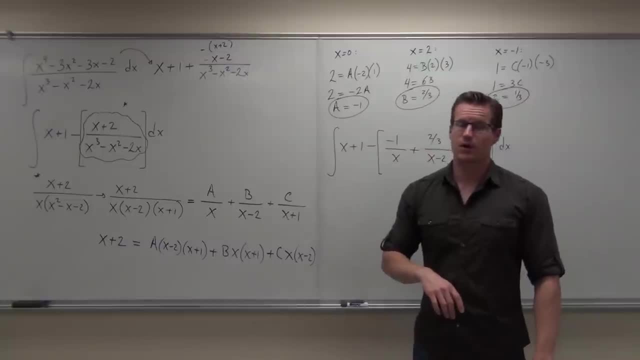 Not a problem. What are we going to do next? We're not going to integrate. No, we're not going to integrate now. We're going to make sure all our signs are correct. So what are we going to do now? Distribute. 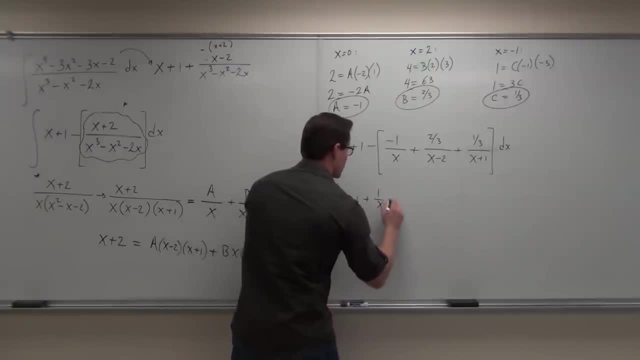 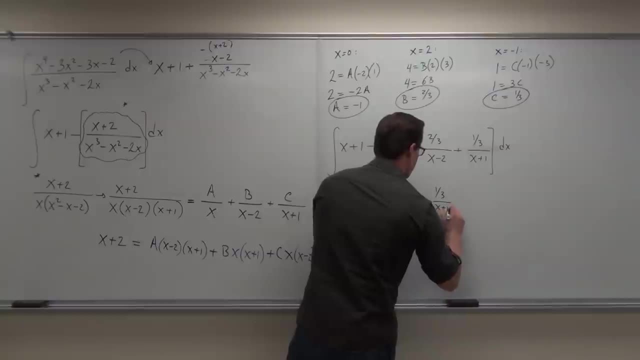 So X plus one plus one over X minus two-thirds over X minus two minus one-third over X plus one, dX. On the whole. Okay. 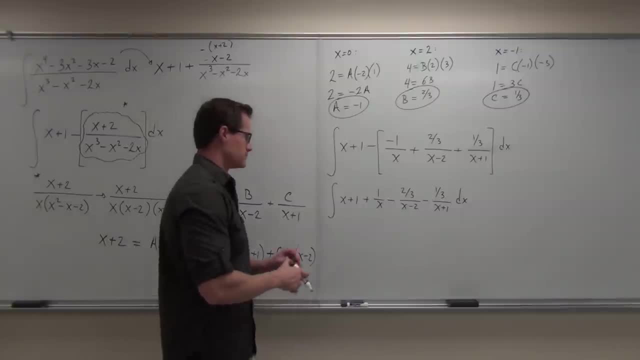 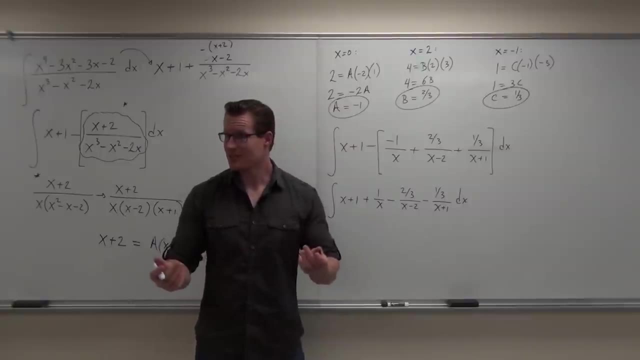 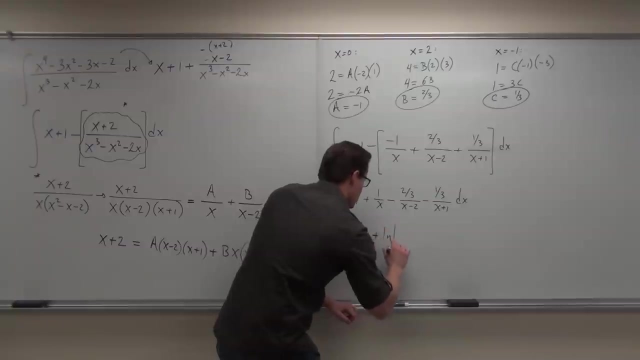 thing are you ready for the last little part yeah interesting interesting we can actually do it huh kind of weird but all it is is algebra it's saying it's rational break it up into fractions not even a big deal now that you've broken up into fractions these are all easy to do what's the integral of X I'm gonna write that as 1 half x squared you okay with that what's the integral of 1 what's the integral everybody should know this integral of 1 over X cool we got this one we got this one we got an L in absolute value of X we're gonna have a minus sign here's how you deal with this look at the board real quick you keep 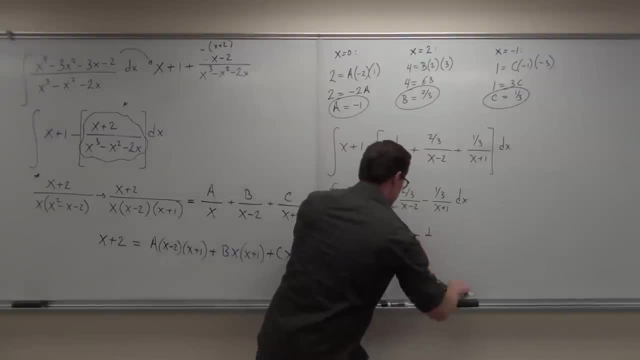 your constant just like we did in the previous example so this will be 2 and write it correctly I thought it 2 3rds 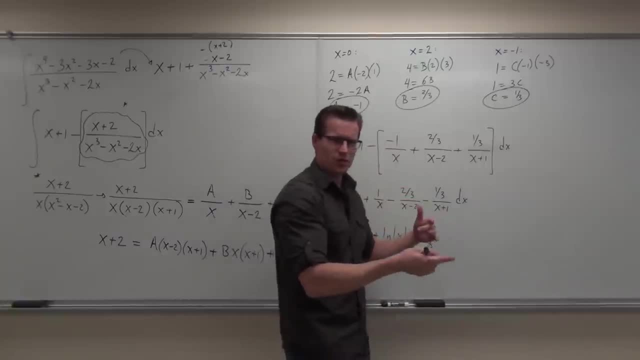 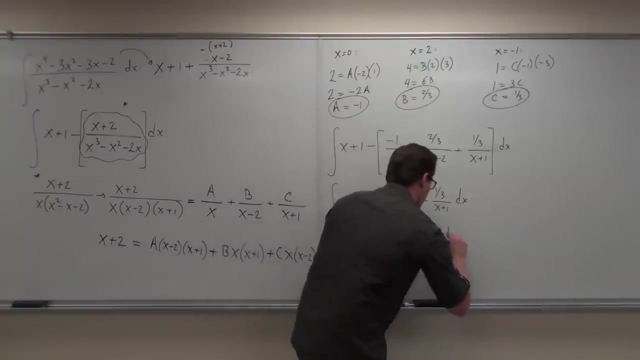 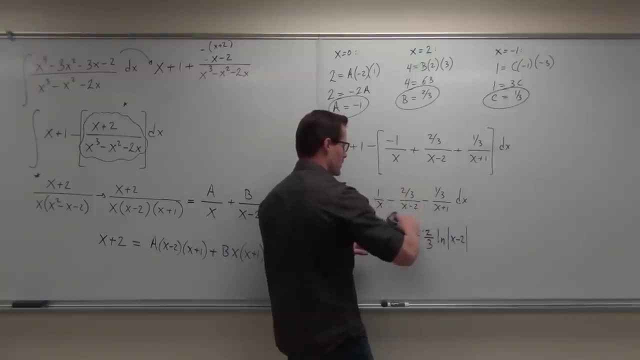 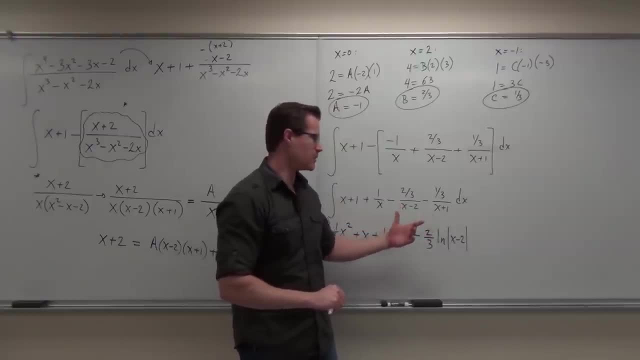 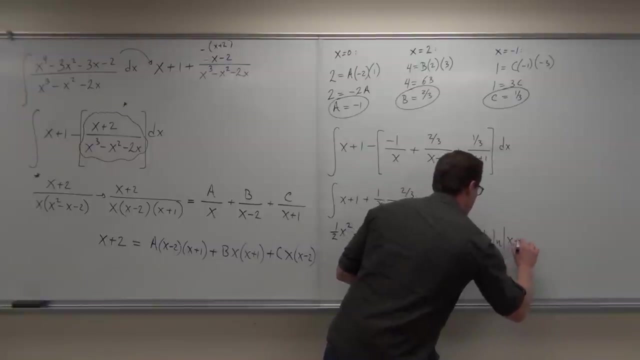 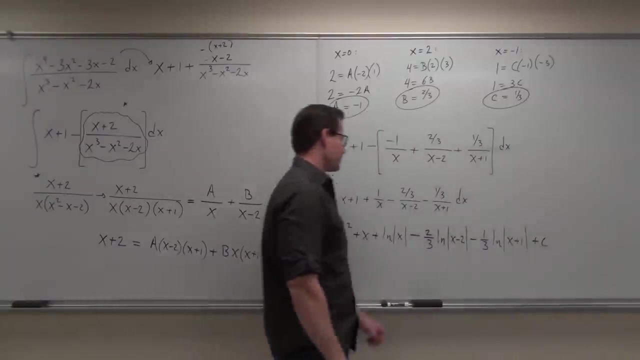 this in your head otherwise we spend forever doing this stuff so yeah if you need it do it but if you don't if you can do it like this that's that's fine we've learned enough about this to be okay with that minus minus what are you supposed to forget those absolute values no absolutely not and then let's see 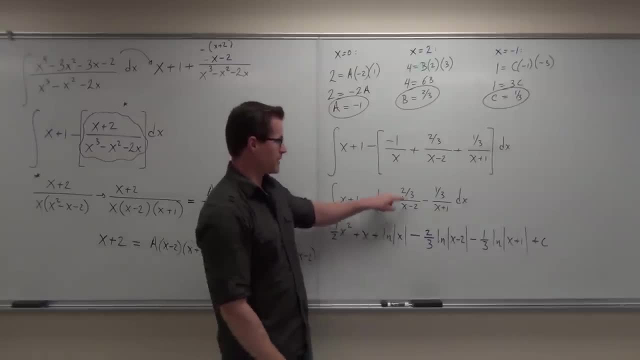 one half X squared X L and absolute value X 2 3rds comes forward another L in one 3rds comes forward another L in and show parents feel okay with what we've done awesome 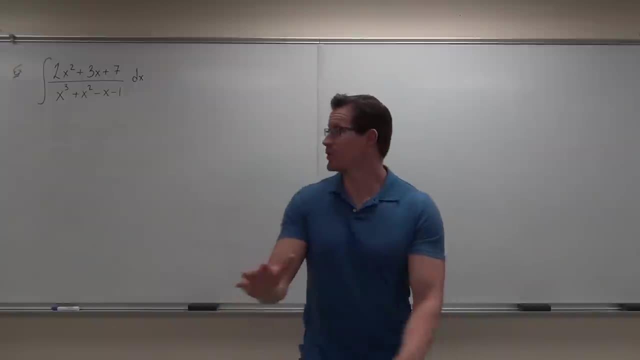 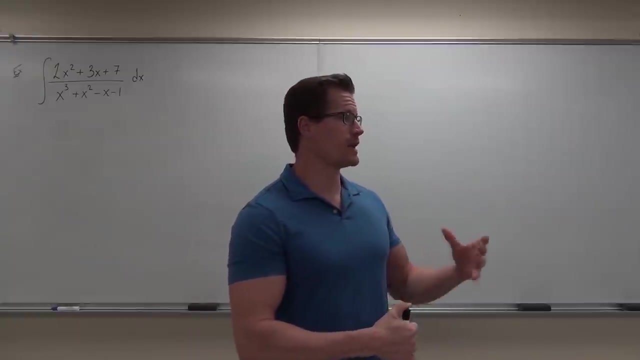 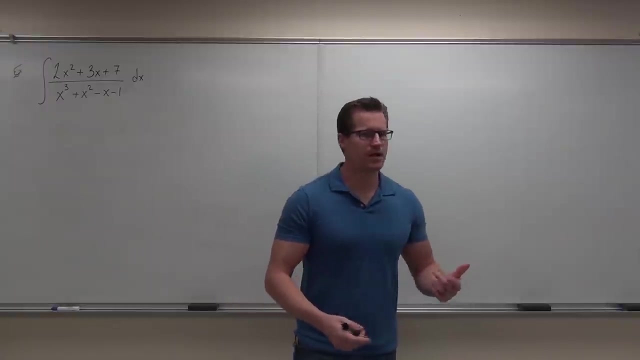 all right we're on to our next example let's take a look at this integral now of course the first things we check for this just like any integral is does it fit anything we can do that's easy does it fit a substitution of course not does it fit integration by parts no it doesn't trig trig sub no not that one nothing like that then we start thinking about okay think about this as a rational as a partial fraction is the degree here less than the degree here 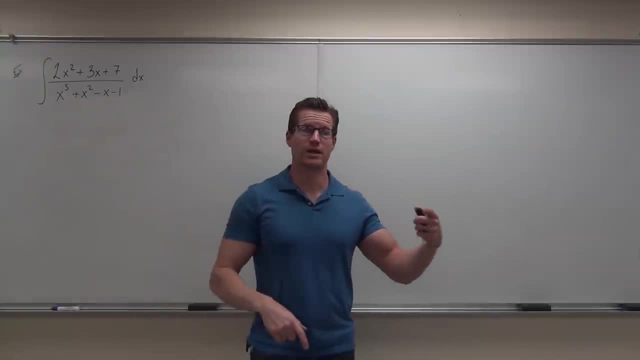 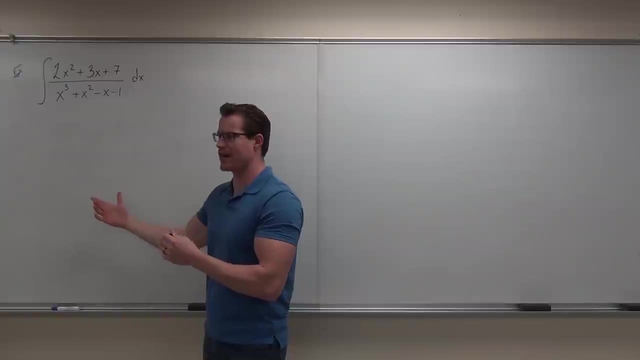 well that's great when it wasn't what do we have to do when it's not if we do our long division then it reduces the degree of the numerator and we go for partial fractions after that I believe our last example was like that one right okay so 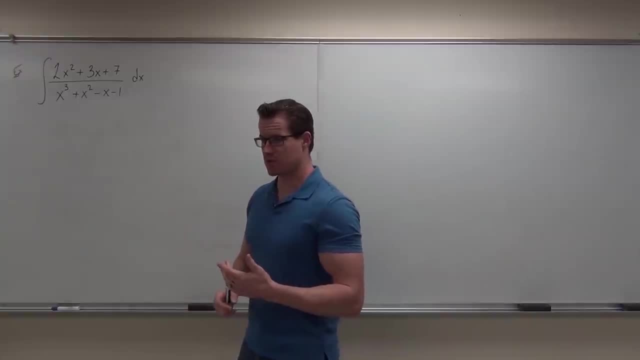 if we don't have something that we have to do long division with we jump 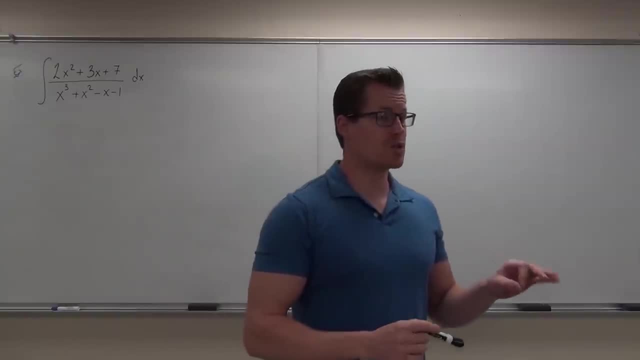 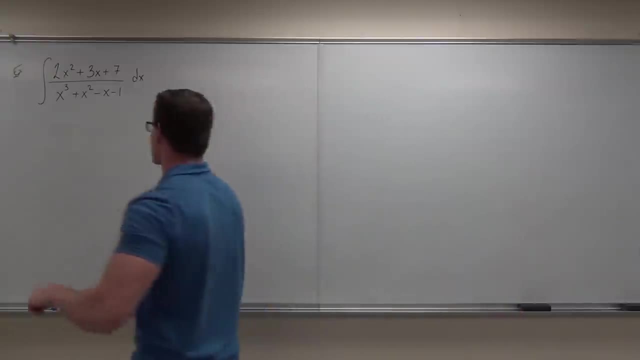 straight into the partial fraction what's the first step in doing partial fractions factoring yeah not the numerator I don't care about that but denominator for sure so let's go ahead let's factor the denominator can you 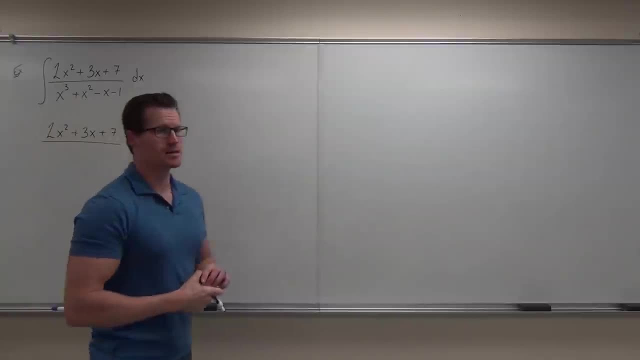 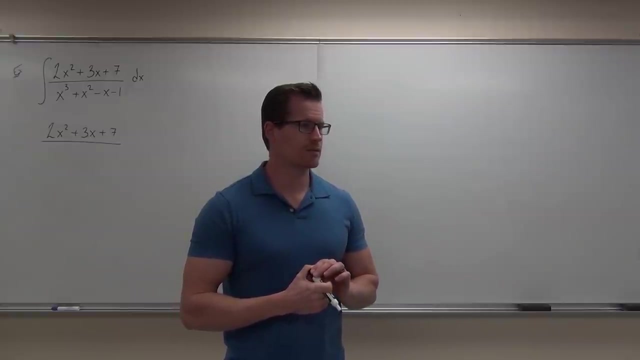 factor x cubed plus x squared minus x minus 1 I can can you factor what do you do when you have four terms try grouping it unless you see an 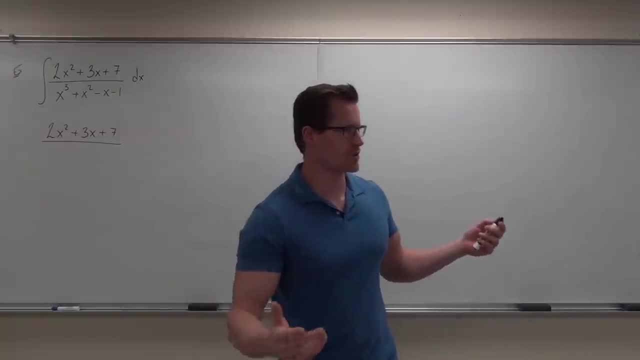 obvious factor like of course a GCF like X or a number or something yeah okay cool factor that but if you don't see that try factoring by grouping for four terms if that doesn't work you have to find a root so you'd have to guess and check for a root or find some other method there are more advanced ways to factor I'm not going to teach them here that's in a higher class on how to factor cubics and quartics and to prove that quintics are not factorable it 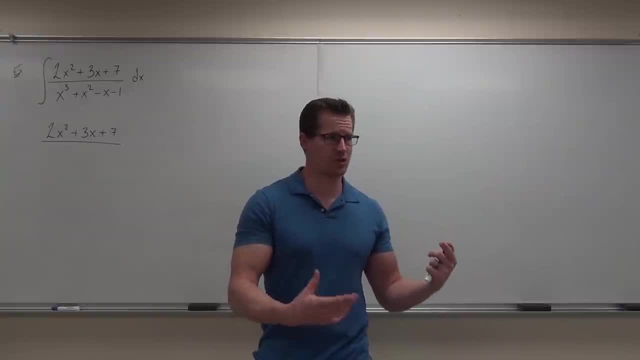 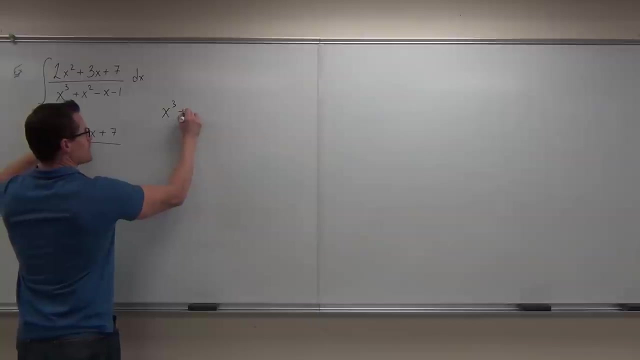 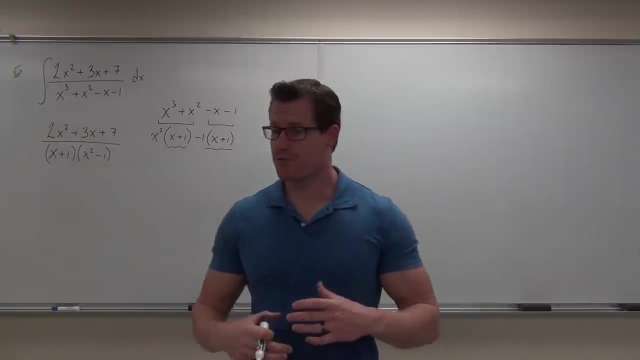 takes a long time to prove that but you prove it for five and higher you can't generally factor it for four and lower you can't there's formulas for it but for for us to make it easy you factor a GCF first if you can like an X if it goes into all the terms if not try factoring by grouping if not then you have to come up with something that actually works like a number that gives you zero and then you can factor X minus that number but that's the idea you can do that by division or synthetic division so anyhow for grouping we'd have our X cube I'm going to erase this in a second so make sure you have this down minus X minus one grouping works like this you group the first two terms and you factor out the GCF you group the last two terms and you factor out the GCF notice when I factor out negative one it changes my sign and then you factor this out and we get X plus one and we get X squared minus one we okay with that so far now is this good enough for us what's the problem with that okay so when we say factor we mean we imply factored completely 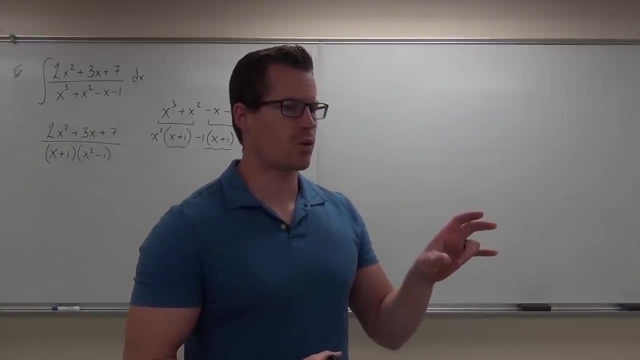 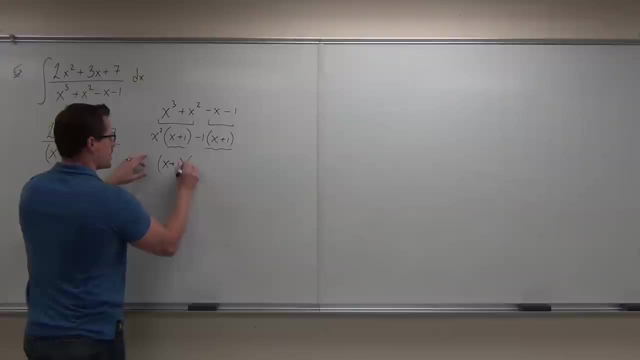 factoring means this factor means linear and or irreducible quadratics so if I end right here with X plus one and X squared minus one this one's great that's cool that's linear linear means power one that's X to the first power you with me this one this is quadratic that would be cool if it was plus if it's plus you're done do you see why you can't factor X plus X squared plus one but if it's X squared minus one that means you have to keep going so we do X plus one and we do X plus one X minus one so if I just feel okay with that one now when you factor something we do want to make this in simplest form 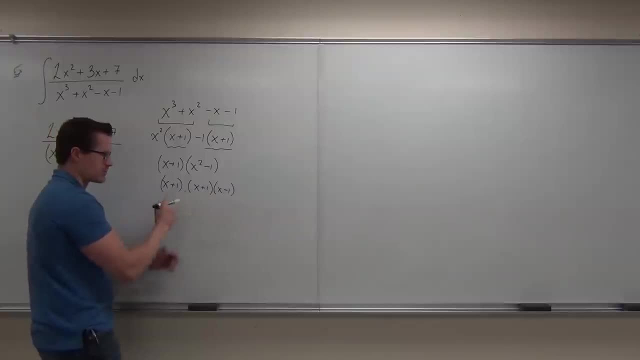 so what we're going to do I'm going to write this up a little bit backwards I'm gonna write X minus one then I'm gonna write X plus one 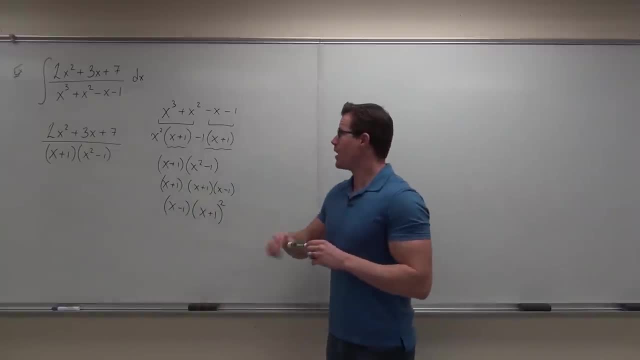 listen I know it's basic algebra but I want to make sure you're okay with it are you okay with factoring by grouping do you understand that we are not going to stop right here with this thing we're going to factor as much as we possibly can until we get down to linear or irreducible quadratics so we're going to factor as much as we possibly can until we get down to linear or irreducible quadratics 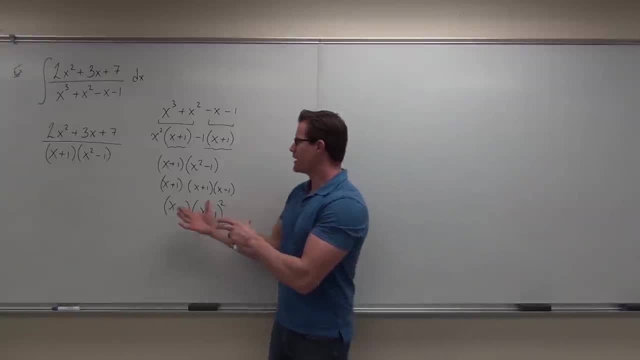 so if we get down to linear or irreducible quadratics okay I'm okay with that so far then I like to to get down to linear or irreducible quadratics rewrite it as linear factors first everyone does this linear factors first and then powers of linear factors and then irreducible quadratics and the powers of irreducible quadratics is typically the way that we we write these so we've got linear and then linear to the second power you guys okay with that so far someone changed this I'm gonna say no no this is not good enough this is actually X minus one two and then X plus one two or four certain is make orientation And then x plus one to the second power. Any questions on this before I erase it? So we have factored by grouping. 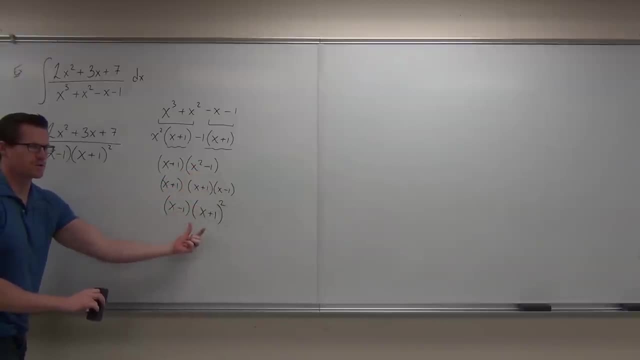 We continue to factor. We grouped our factors that were the same. So x plus one would be squared. 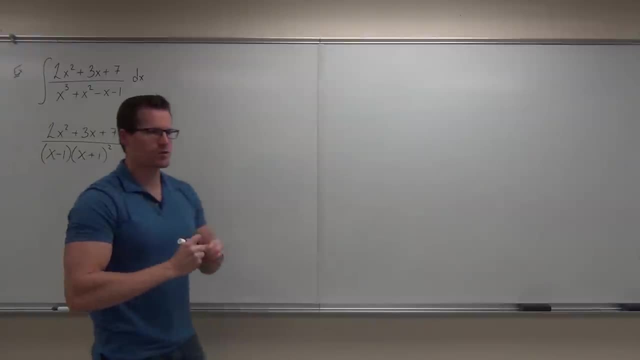 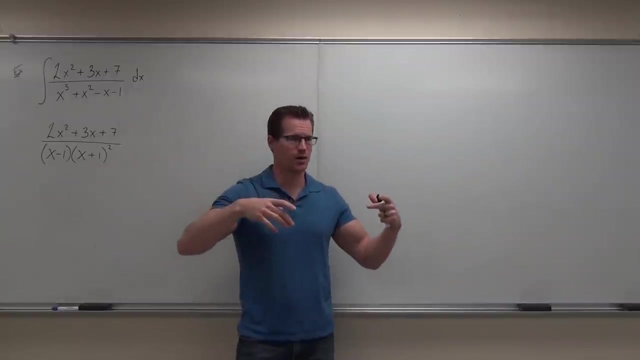 Now this is different. You see, before what we had was we had unique linear factors. Remember that? And we set this up as a over x minus one. And then b over x plus one. Stuff like that. 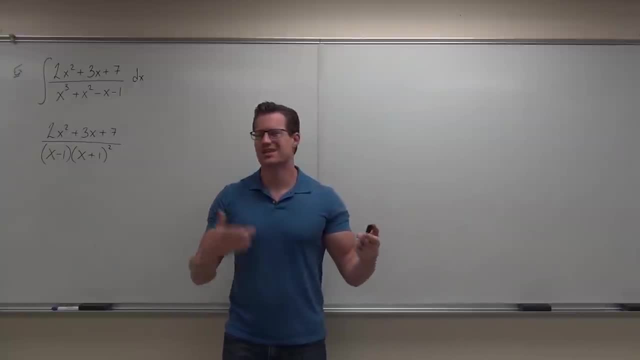 Well, when we have these repeated linear factors, that's actually case number two. 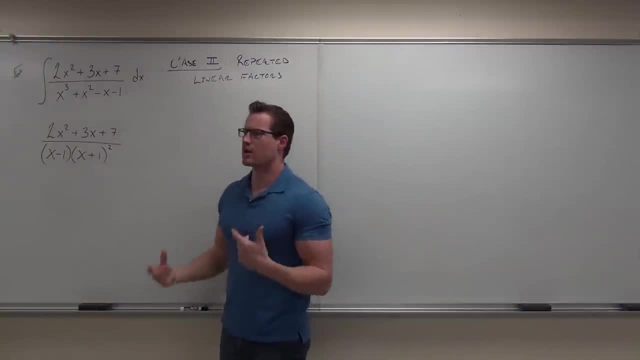 Here's what we mean by repeated. It means that you have linear. You have more than one of them. So for instance, we have x minus one. We had an x plus one. And we had another x plus one. That's why we had this x plus one squared. 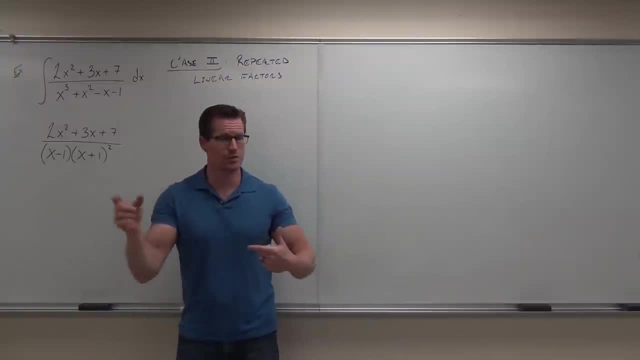 This factor was repeated. Hence the square. If it was repeated again, we'd have it to the third power. You guys with me on this one? 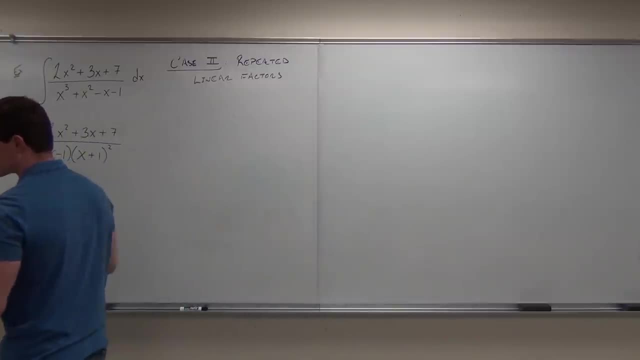 So here's how you do it. With any repeated linear factors, what we end up doing is we write a1 over the first factor. 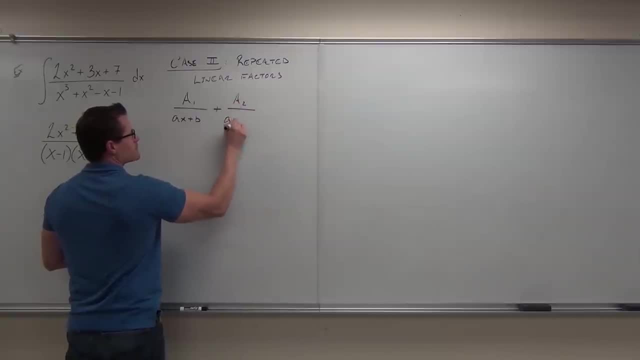 Plus a2 over that factor to whatever power we have. And we continue until we run out of the repeated factors. So for instance, if this was to the fifth power, what you'd end up doing is you'd have a1 over whatever linear factor you got. 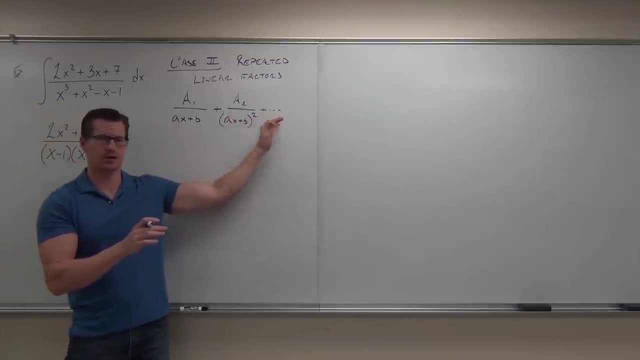 Okay? And you'd exhaust those powers of linear factors. I'll show you in a minute how to do that. If we had a to the fifth, you'd have a1 over the factor. A, a different one. So b. You'd have b over the factor squared. Then c over the factor squared. Then d over the factor to the third. Then d over the factor to the fourth. Then e over the factor to the fifth. 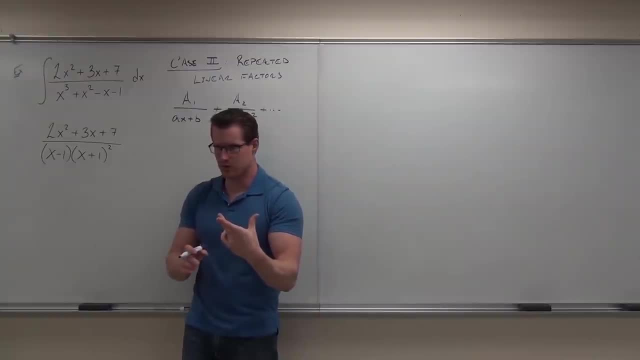 You have every single different power of that factor. Are you with me on this one? 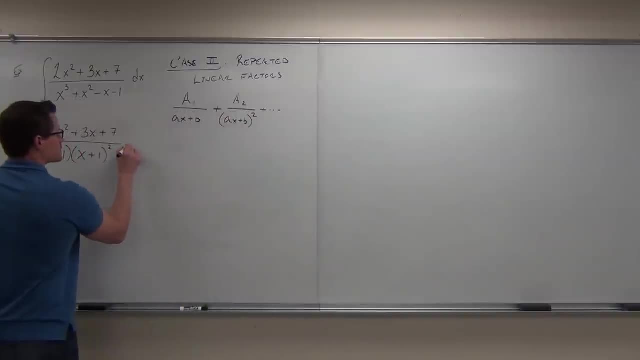 Let me show you how it works here for us. So in our case, what we're going to end up getting is how many fractions do you think we're going to get here? 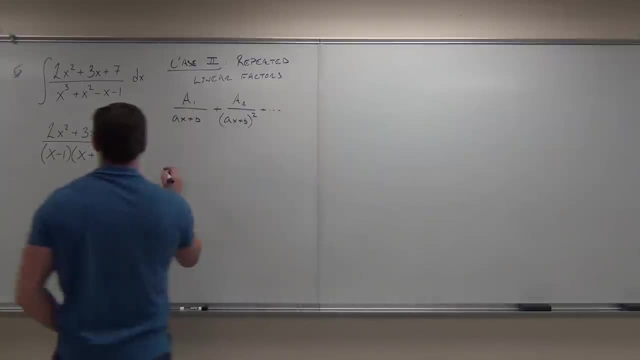 We're still going to get three. That's right. So we're still going to have one. Look at this. Two. And again. 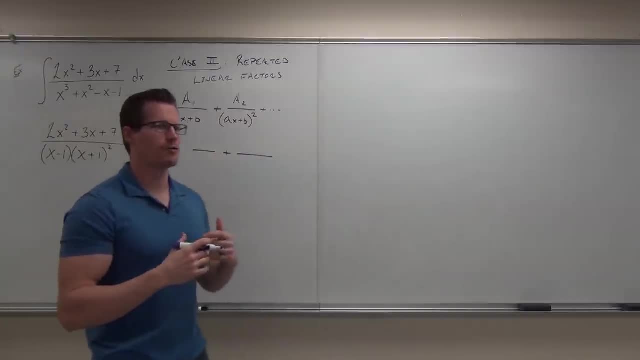 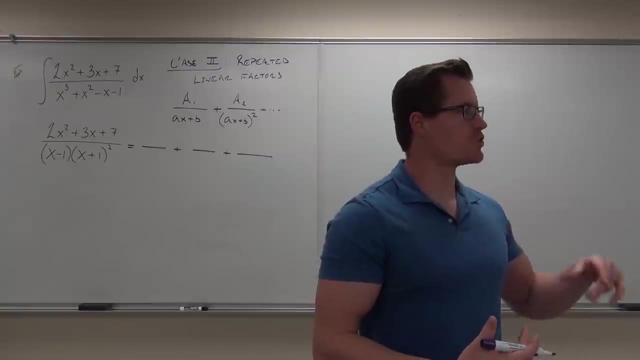 Three. To understand why we have three fractions here, we still have those three factors initially. We still do. It's just one was repeated. 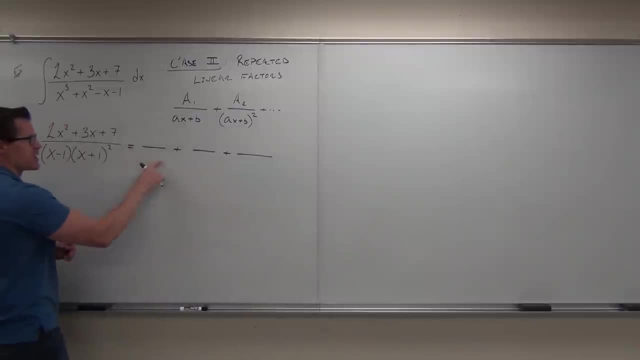 And so what we're going to have, what do you think is going to be my first denominator? X minus 1. X minus 1. X minus 1 is going to be there. Are you guys with me? And then what we do is we say, oh, okay, have we exhausted all the powers of x minus 1? Yes. There was just one of them. We're good. 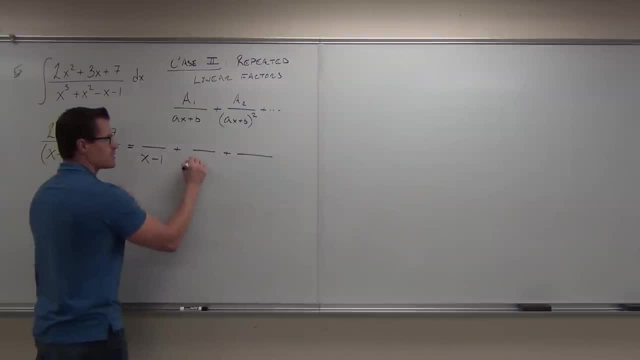 Now we move on to the next one. X plus 1. X plus 1 has got to be here. 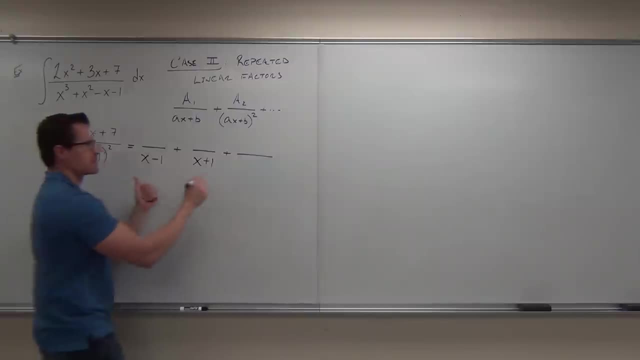 Have we exhausted all the powers of x plus 1? No. No. So we go x plus 1. Square squared. Very good. Okay. Let's see if you're paying attention. What if this was to the fourth power? Keep going. Two more. I'd add x plus 1 to the third, x plus 1 to the fourth. Does that make sense to you? So this one, hey, we're done with that one. 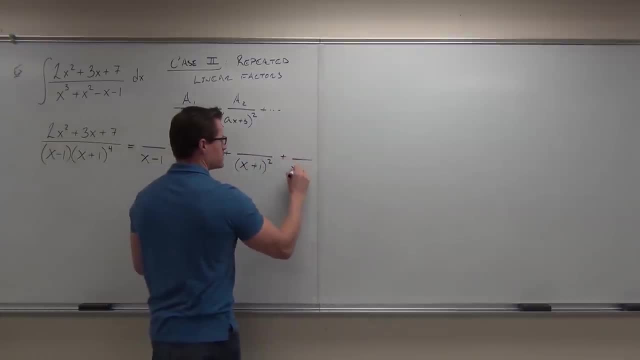 This one would be to the first, then to the second, then to the third. 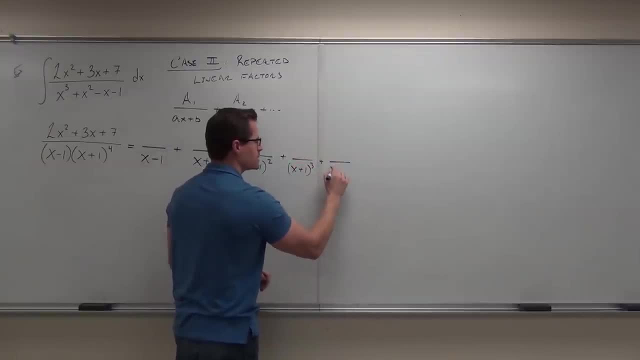 Until you get all the powers up there, until you exhaust all of them. You with me on that one? All right. 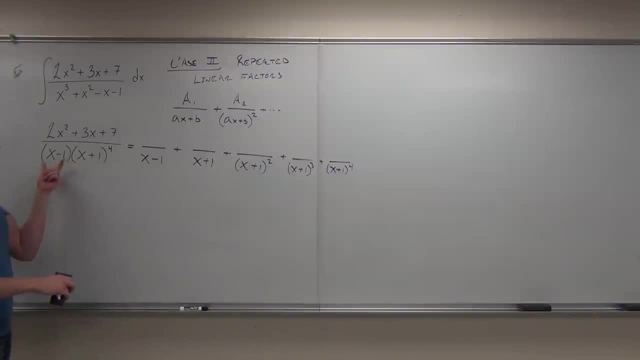 Because we have these different factors, if you had this, you'd really have x plus 1 and then another, I'm sorry, x minus 1, then x plus 1, times x plus 1, times x plus 1. You'd have five factors there. 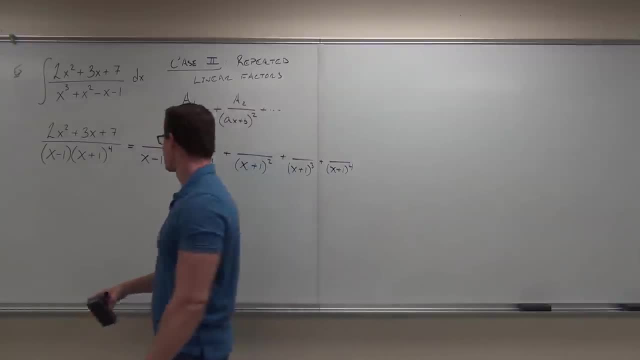 We show those powers to show those different possibilities of those factors. Now, where did I stop? X plus 1. What was that one? Square. It was a 2. Okay. 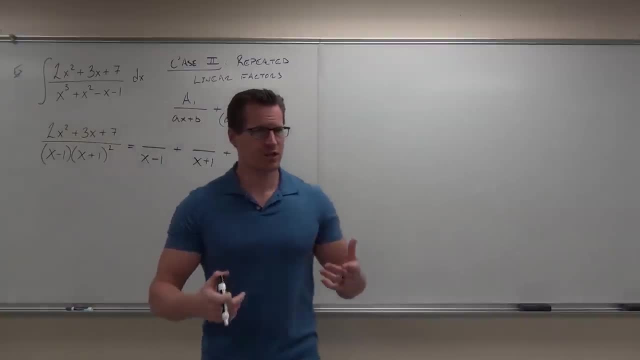 Now, fortunately for us, they're still linear, right? They're still linear. So all we need on the numerators are a and b and c. 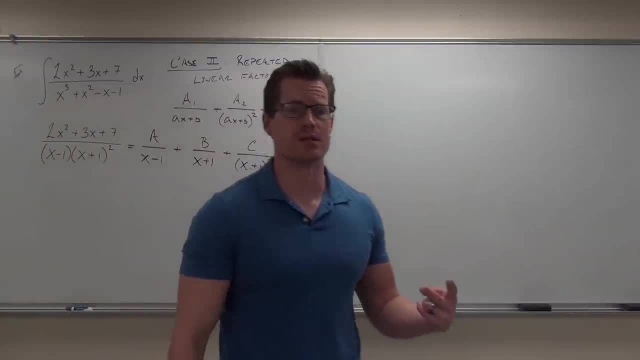 And then we do exactly the same thing we did before. So now we have two cases. 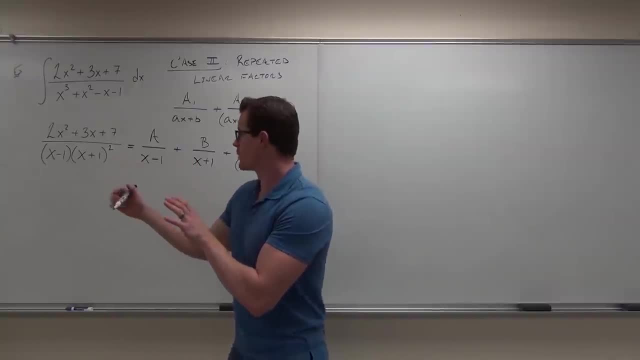 We have the cases where we have distinct linear factors, where we have a and b. We have x plus 1, and it doesn't happen again. 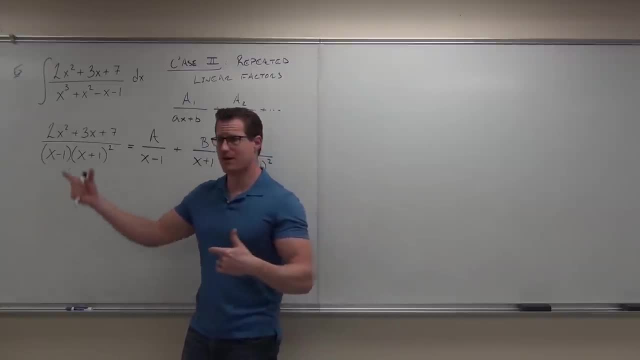 That was our first case. And that case is pretty straightforward. We just have every different factor on the denominator, a, b, c, d, e, whatever, until you exhaust them. You guys with me on that one? Then, now we have the second case. 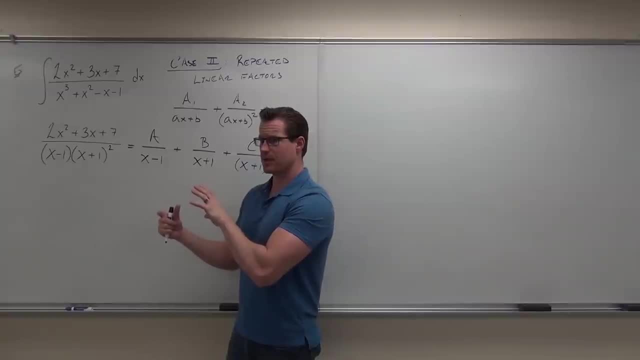 We've got the case where we might have some repeated linear factors. For those linear factors that aren't repeated, do the same thing. Exactly the same. 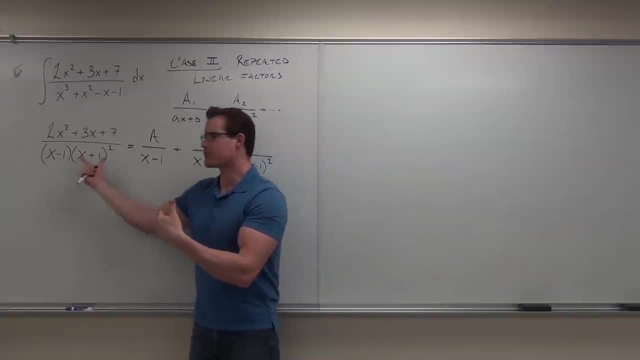 For those ones that are repeated, have the first power, then have the second power. This is the answer. 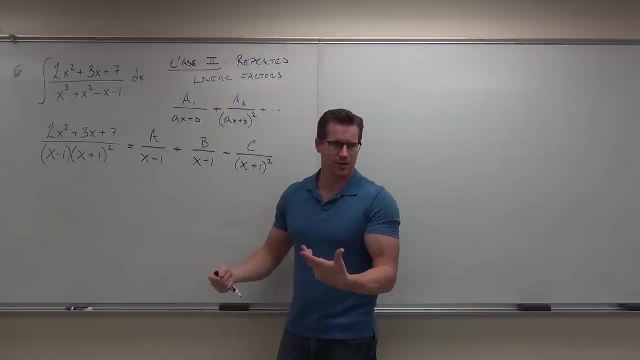 The idea of partial fractions is how it works. You guys okay with it? 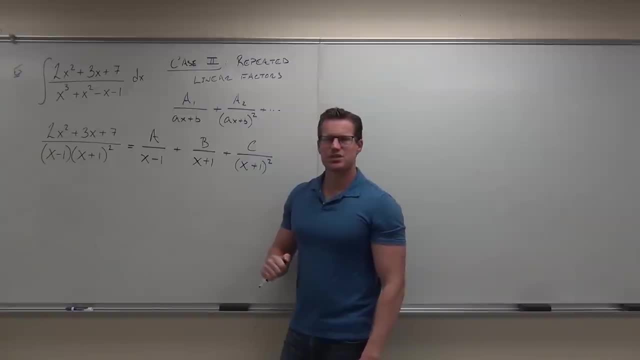 Now, can we make a common denominator still? Be smart about it. 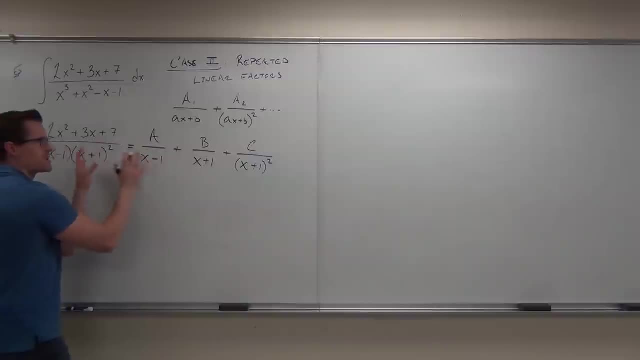 When I'm making the common denominator, remember the idea is make a common denominator, then ignore the denominator. 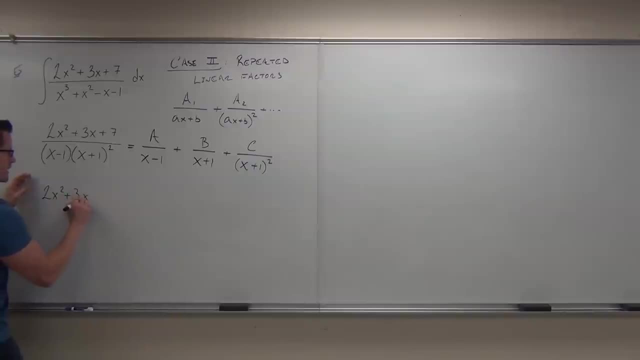 So ultimately, we're going to have 2x squared plus 3x plus 7 equal to whatever I get upon finding my common denominator. Here's the whole deal, though. Listen. Listen and look. 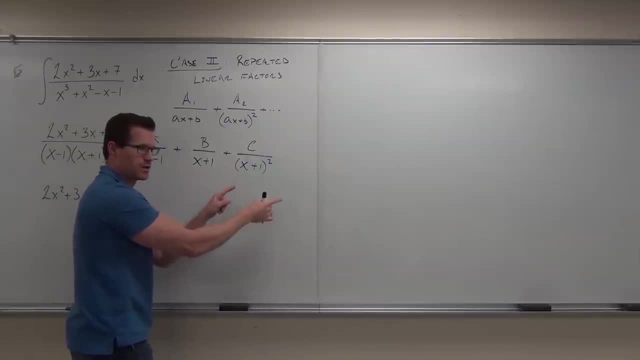 You're going to have, with repeated linears, a lot of the same things, aren't you? Use the largest power here. So when I find my common denominator on this fraction, of course I'm not multiplying by this guy. 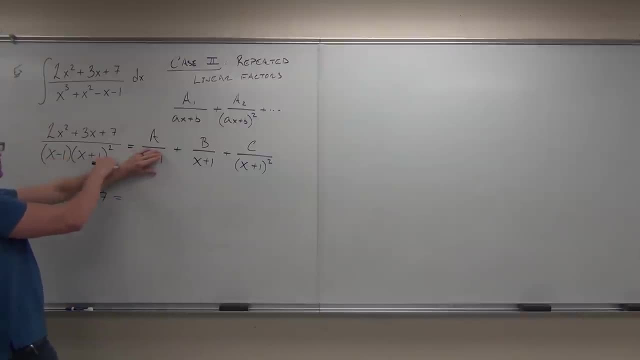 I already got that guy. But look over here. I need to match this up. I'm not missing the x minus 1. 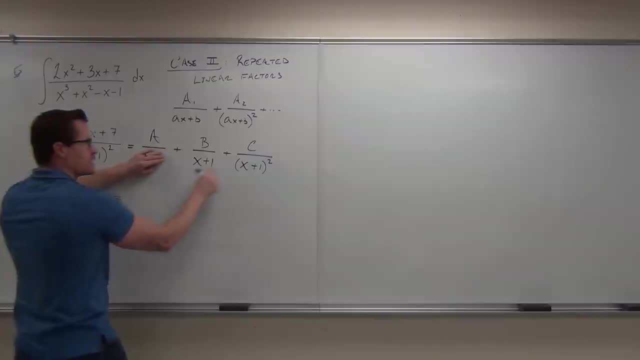 I'm missing the x plus 1 squared. Don't take both of them. Just take the largest power. Does that make sense to you? So I don't need this and this. 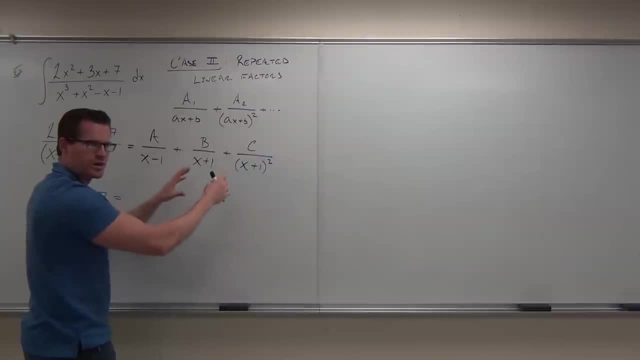 This one kind of counts for this one as well. This is the only factor I'm missing. You can see that on this previous fraction. In order to find a common denominator with this, I would just have to multiply it by x plus 1 to the third or to the second? Second. To the second. So far so good? It's just algebra, but I want to make sure you're good with it. 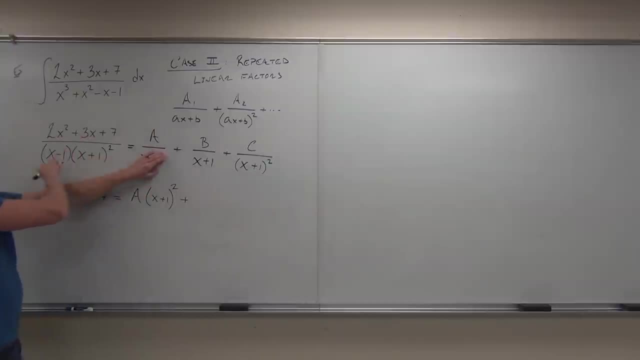 Plus. So we covered up. We take the largest power. That is what's given us our common denominator. 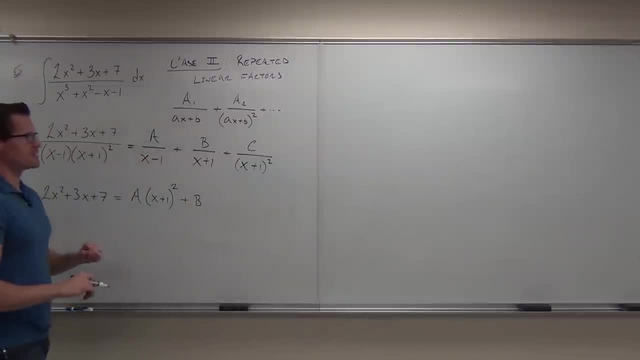 Now we move on to the b. What's missing on this b fraction? x minus 1. x minus 1 is missing. Look. You can look here. If I cover that up. What's missing here? Well, x minus 1 is missing from there. What else is missing from here? The squares. The squares. 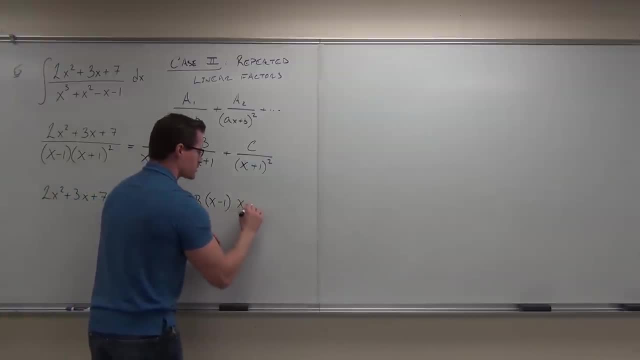 Okay. So do I multiply it by x plus 1 squared? Would that be a good idea? No. No. Don't do that. It's way too much. What should I multiply by? You're only missing one factor of the x plus 1. Are you guys getting that? So this, no. 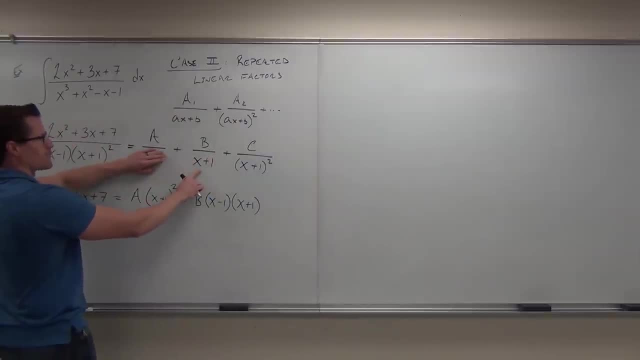 So when I look here, yeah, I was missing x plus 1, but more than that, I'm missing x plus 1 squared. That's why we're multiplying by this. I'm missing this whole factor here. With the b, I've got one factor of x plus 1 already. I'm only missing one more. This, look at this. 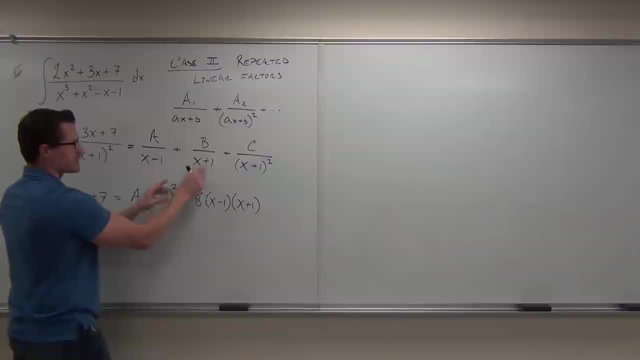 This would give us the x plus 1 squared, and this would give us the x minus 1. So I'm missing x minus 1 and one factor of x plus 1. From the c, let's look at the c. What am I missing from here to here? What's missing? x minus 1. That's it. So I wouldn't take this one. I've already got it. It's like trading cards. 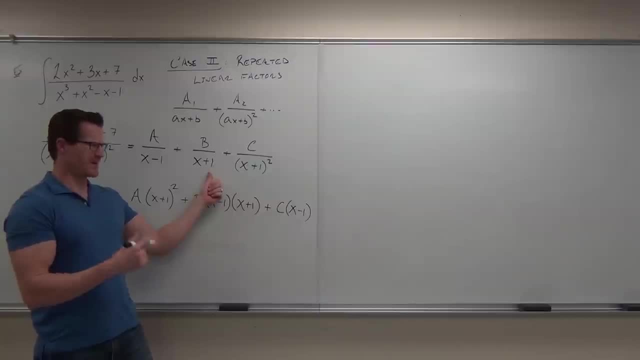 You go, I've got two Jose Cansecos. I've got another Jose Canseco. Do you need it? No, I've only got two of them. I don't need another Jose Canseco. 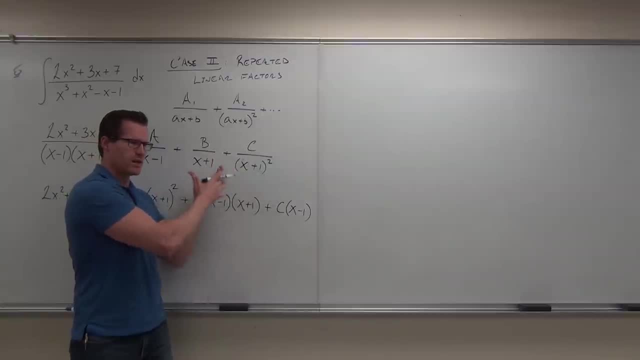 I just want to make some money and sell cards, but we already got those. We don't need an extra one. We have enough of our Jose Cansecos. 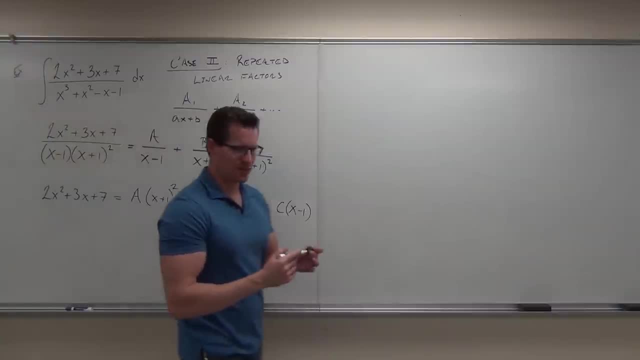 That was a weird analogy, wasn't it? Anyway, question? 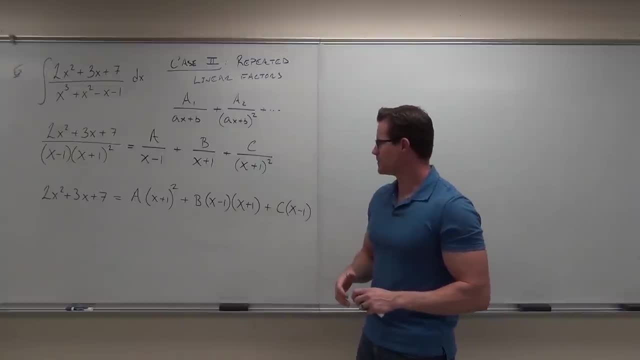 So because you already have the x plus 1 squared on the bottom, you only need x minus 1 for c? That's correct. 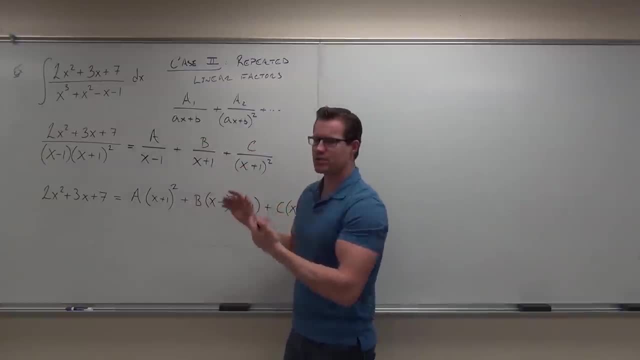 Basically, we're looking at these fractions, and some people teach it, cover this up, take the rest of it, okay? 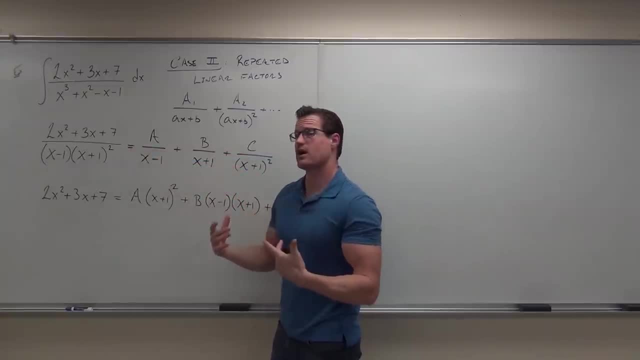 Not this one, but the largest power. I prefer you to think of, we're finding the common denominator. 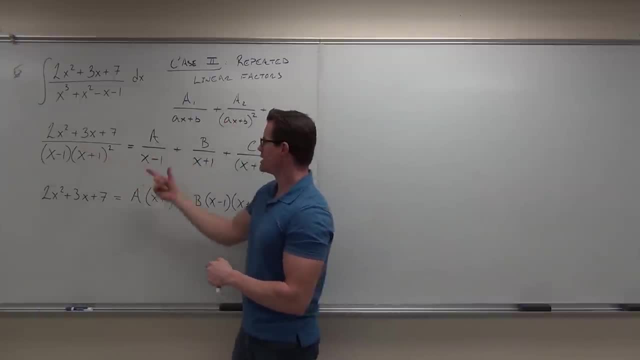 So look here, look here. What's missing between here and here? 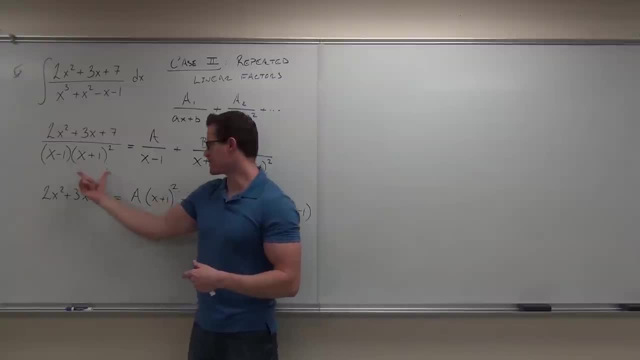 x plus 1. x plus 1 to the second power is missing. We need x plus 1 to the second. Look here, look here. What's missing? 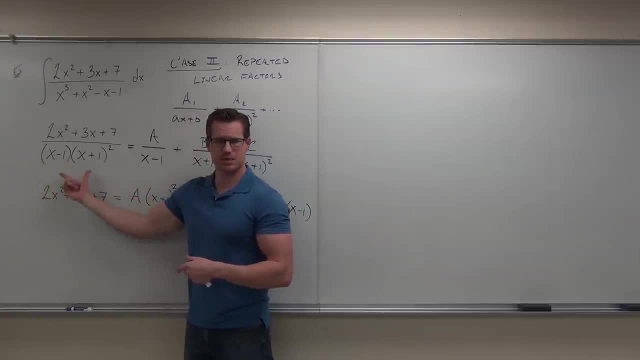 x minus 1 and 1 factor of x plus 1. Does that make sense? Look here. Look here. What's missing? x plus 1. That's it. Not x plus 1. You already have the x plus 1 squared. Honestly, Jose Canseco, you're okay with that so far. 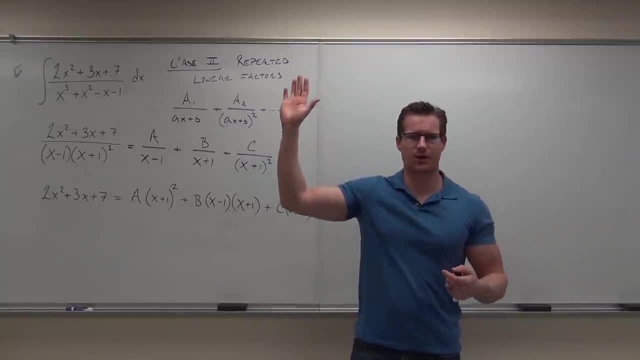 Now, did I teach you the plug in and end up, the cheating way? Yes. Is the cheating way going to work for here? No. Why not? Can you make this 0? Yeah. Of course you can. Can you make this 0? Yeah. Can you make this 0? Yeah. Can you make this 0? Yeah. Then why wouldn't that work? It works for linears. It works really well for linears. All right? 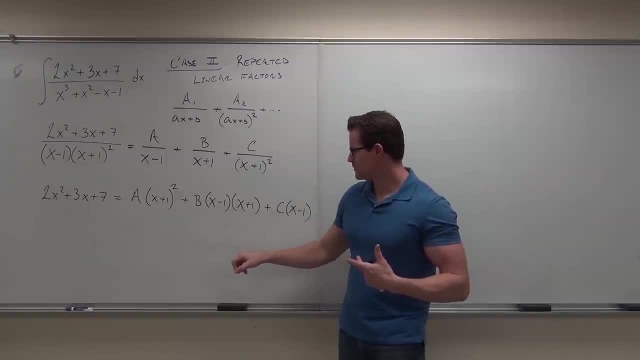 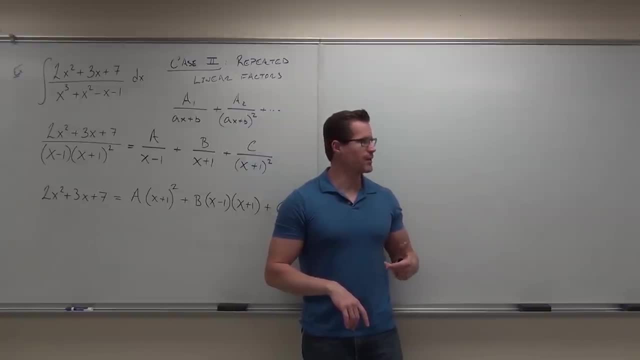 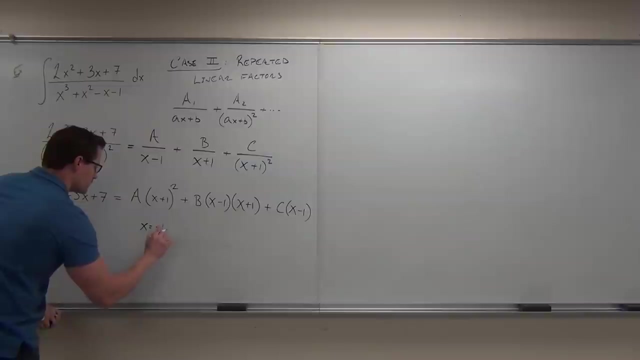 1 and definitely negative 1. 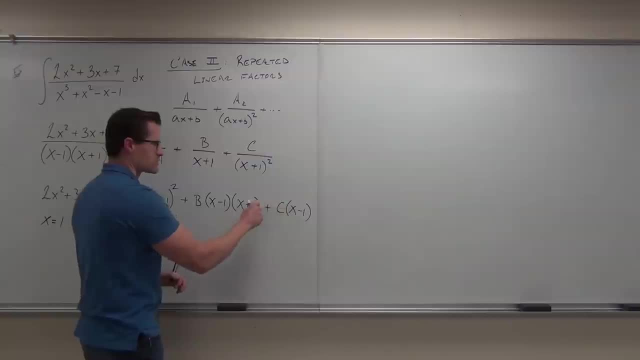 We try those right off the bat. Because, negative 1 is going to give us some zeros. 1 is going to give us some zeros. 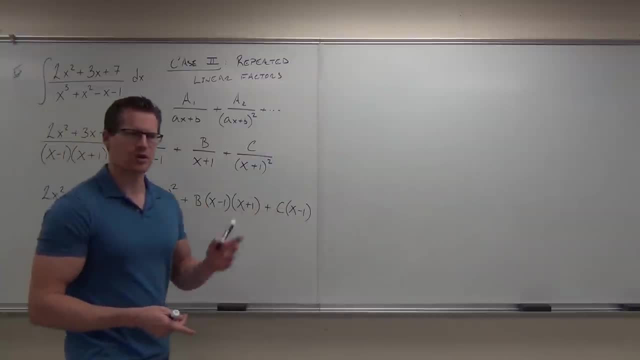 going to give us some zeros we'll be able to find at least two of these things for the last one i'll teach you how to do that in a minute so plug it in what did you already do them 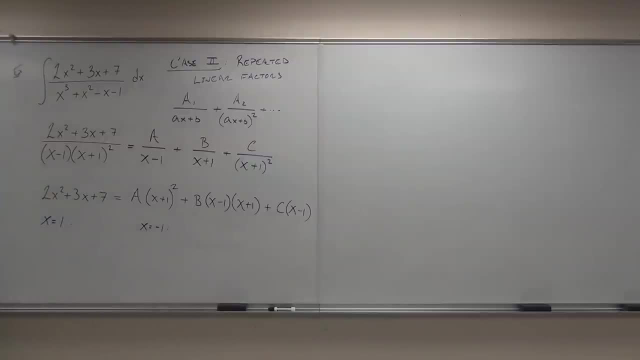 go for it i really want you to try it 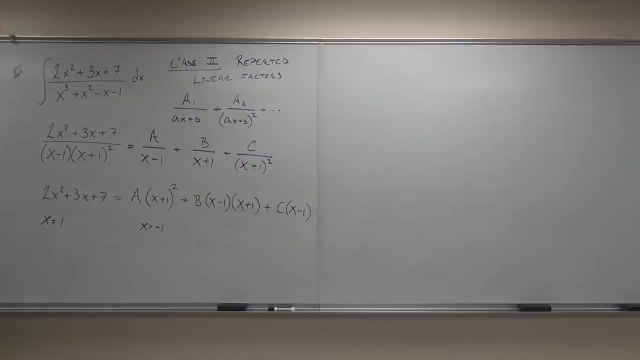 plug it in one if i plug in one one minus one is zero this is gone one minus one is zero this whole thing is gone one oh one plus one that's two squared 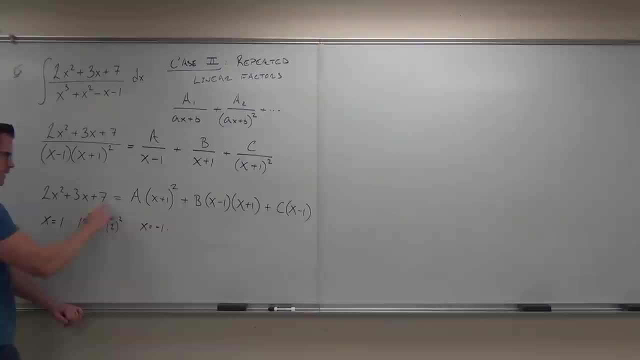 so all i know is that 12 equals a times two squared did you guys get that as well 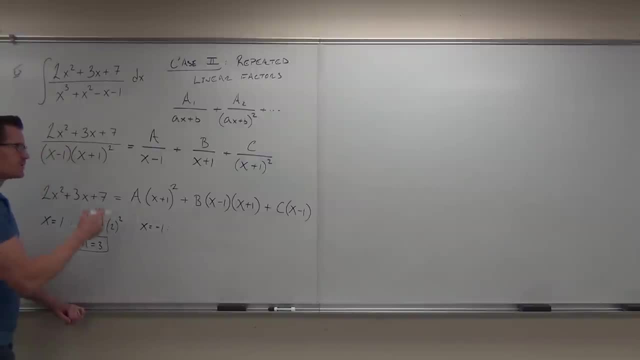 i think ace three did you get ace three yeah awesome now do negative one do the easy ones 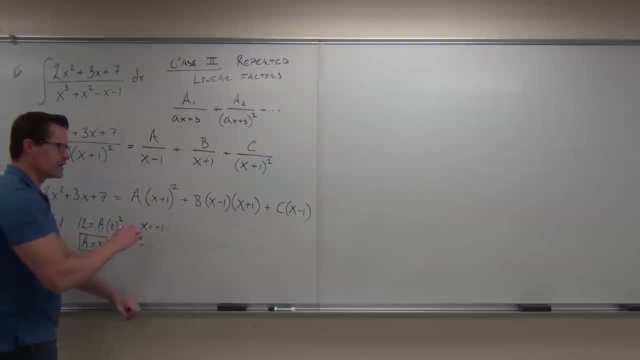 first first so negative one if i plug in negative one what i know is that on this side i get oh man what is that two minus three plus seven how much did you get six okay so if i plug in negative one negative one plus one is zero whole term gone negative one plus one is zero whole term gone negative one oh negative one minus one how much is that negative 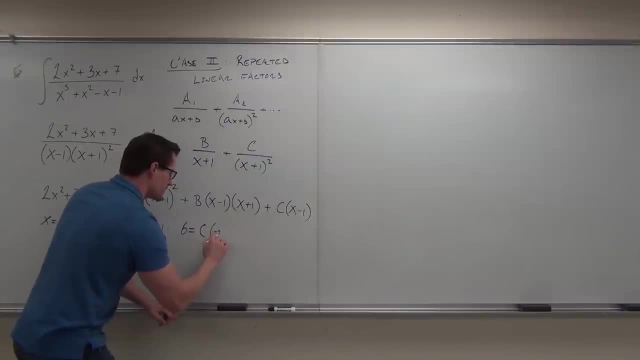 two so c times negative two what's c equal it's negative and here's an issue 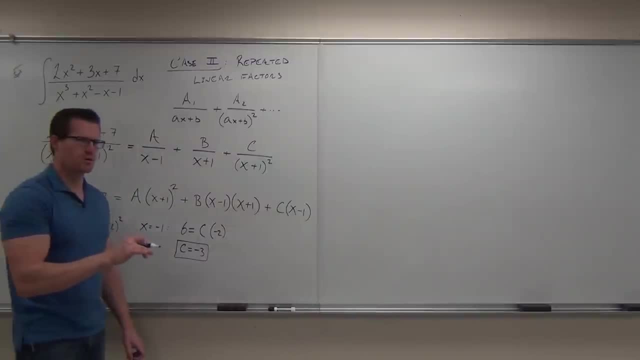 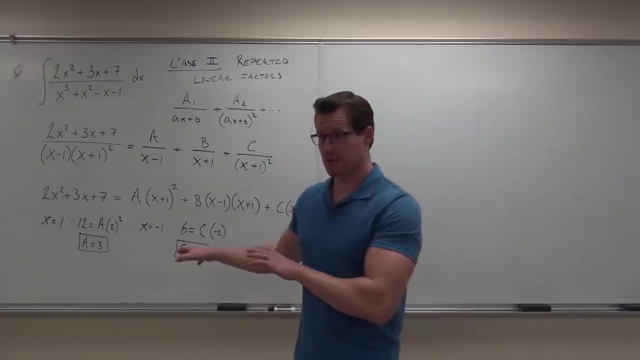 did it give you b so i plugged in the numbers that give me zero i got a and c i didn't get b you're going to get zero here's a little trick when you get down here like wait a second with these repeated uh linears this happens a lot okay because you're going to have stuff that looks like this where there's not a number there's no x there's no number you can actually plug in 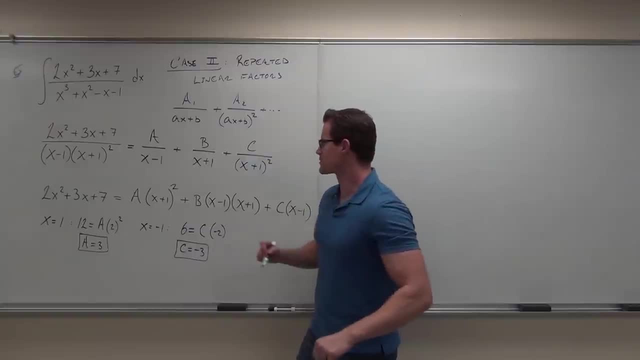 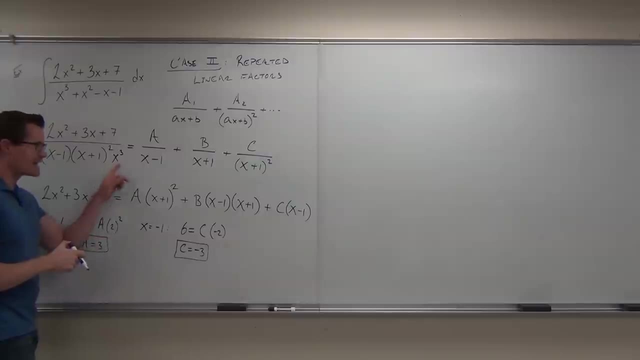 oh you know what while i'm thinking of it as well so if you think of this right now if i had x to the third power like this if i had x to the third that would count as repeated linears this is not irreducible quadratic it's repeated linears, you'd have something over x plus something over x squared plus something over x to the third. 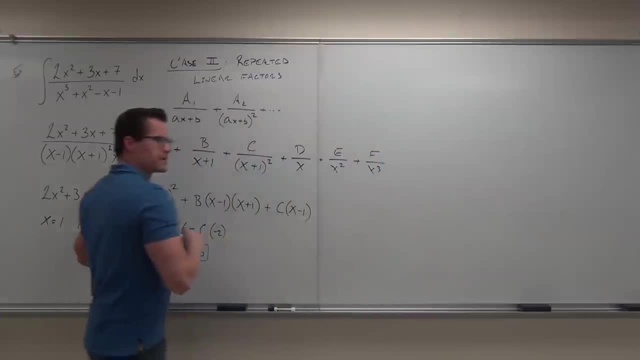 You'd have a d and e and an f. Does that make sense to you? So x to the third is repeated linears, x and then x squared and then x to the third. Okay? Just while it was on my mind, I wanted to clear that up. I know some of your problems are like that. 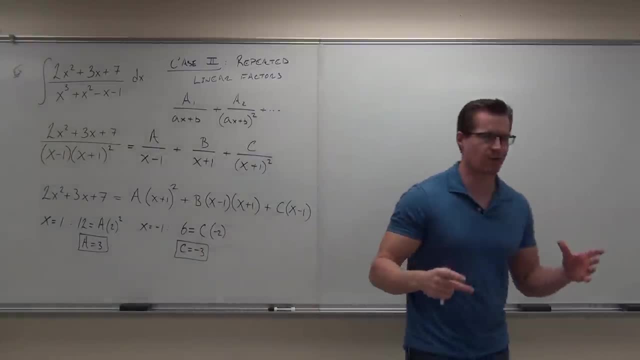 So let's say that we don't have a number that gives us zero for one whole term. Just pick another number to plug in. Something easy. I would plug in probably zero. Just plug in zero. 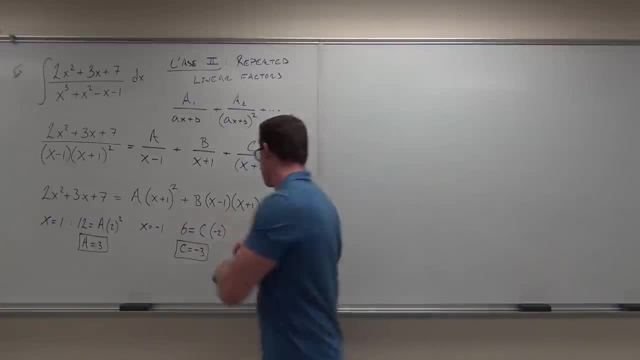 You can plug in any number you want, correct? If I plug in zero, yeah, it's not going to get rid of anything, 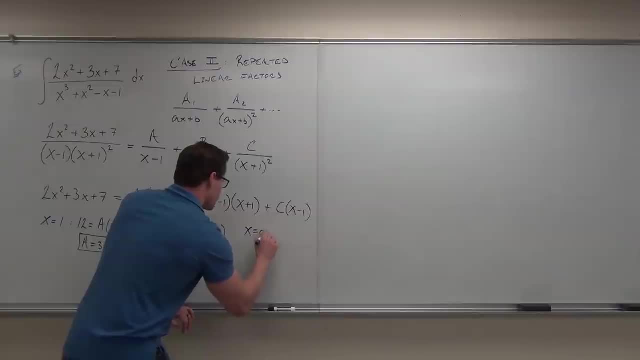 but it's going to make it easier to do. So I'd plug in x equals zero. Check it. If I plug in x equals zero, what happens on the left-hand side? 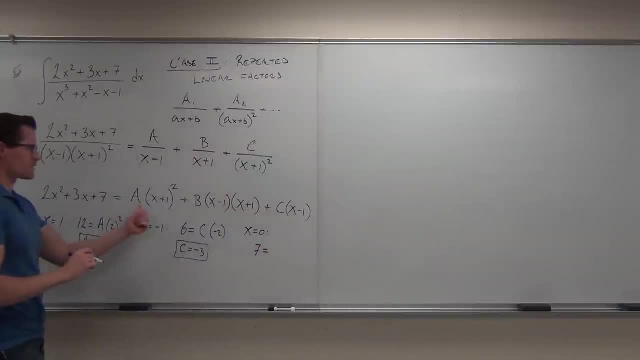 If I plug in x equals zero over here, well, all I'm going to get is a times 1 squared or a times 1. 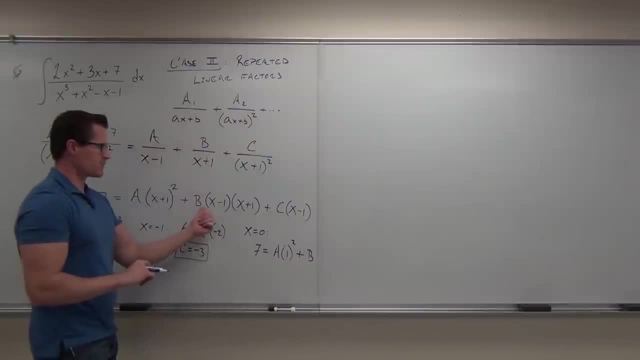 Then I'm going to get b times, let's plug in zero here. 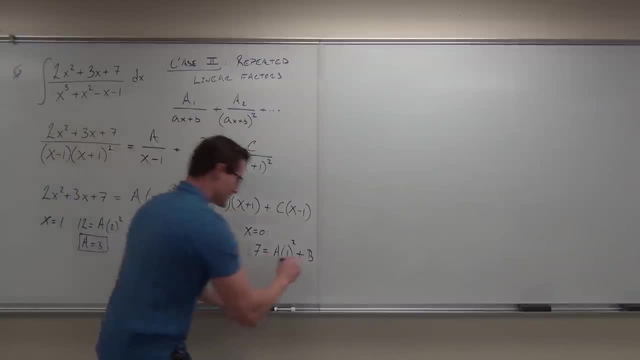 If I plug in zero, I'm going to get negative 1. I'm going to get positive 1. 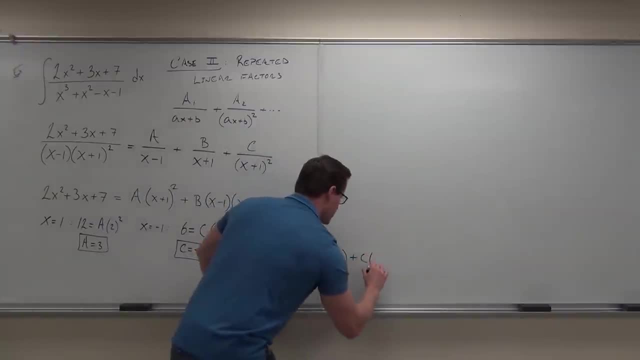 Plus. If I plug in zero here, I'm going to get c times negative 1. Ladies and gentlemen, did you follow that? 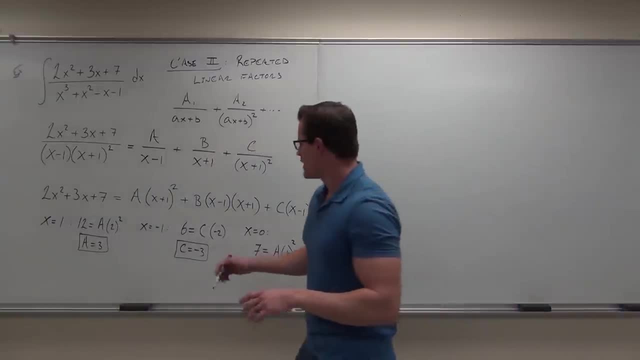 Just pick another easy number to plug in for these linears. It's kind of nice. If I plug in, well, not 1. I already dealt with that. Negative 1. I dealt with that. Those were the easy ones, right? Those give us lots of zeros. 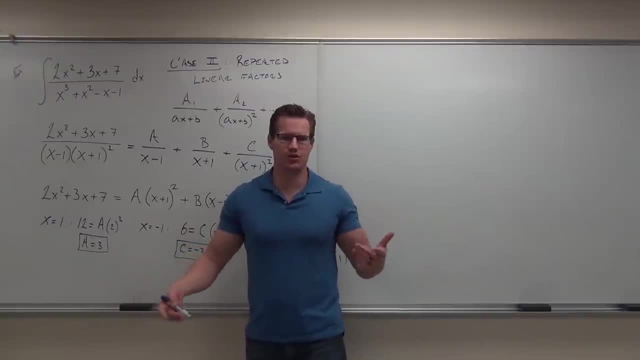 Take another number. You plug in anything you want to. You plug in 7 or 12 or negative 15 or 1. Well, you already did it. 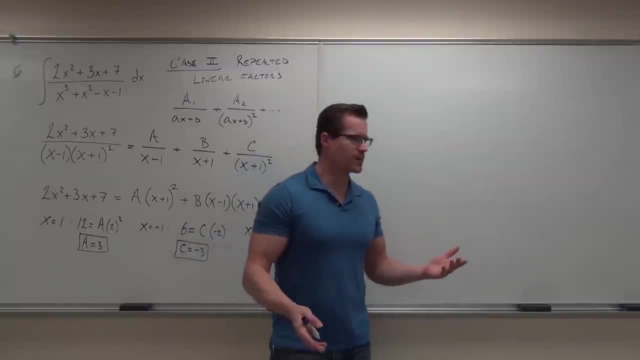 Or zero, 1 in a different case, but plug in whatever you want. And that way, you get, well, an equation. 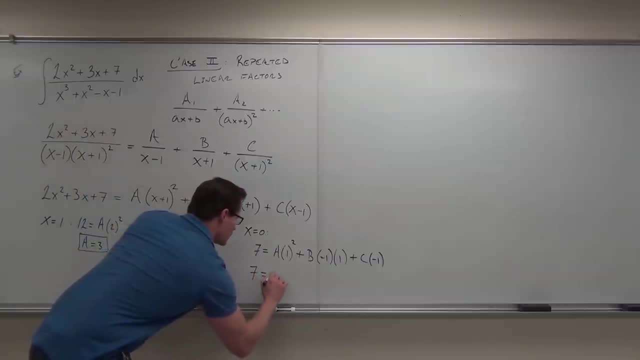 Seven on the left-hand side. Over here, we get 7 equals a minus b. A is why we did this first. Do you know how much a is? Yes. Do you know how much b is? Yes. Do you know how much c is? No, not b. Not b. Do you know how much c is? Yes. Yes. Plug them in and find it. 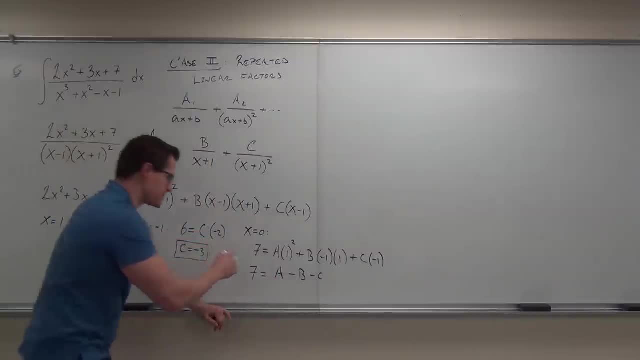 So once you deal with a couple of these factors, the rest of them become pretty darn easy as far as linears go. 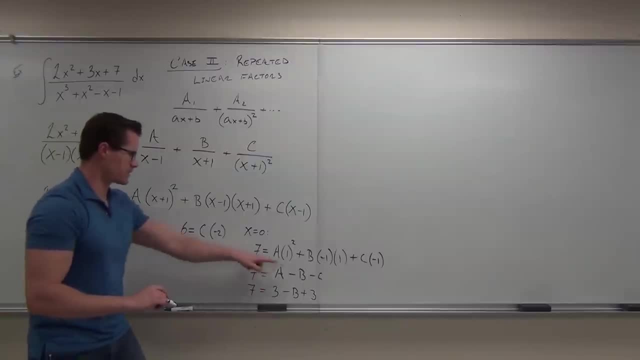 So we've got 3 minus b and then plus 3 because we have minus a negative. Looks like we're going to get. What? 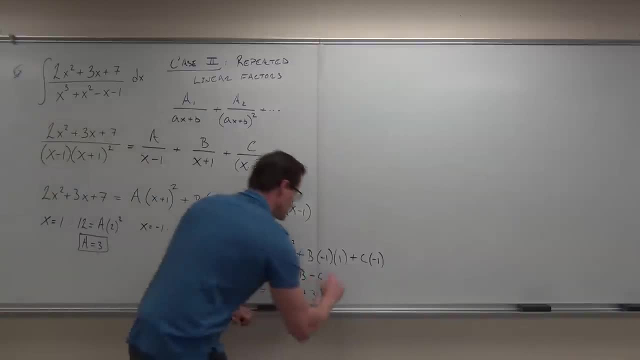 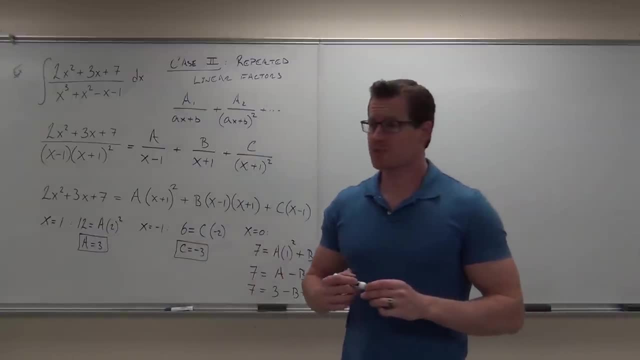 Honestly, that's the hard part, finding out the a, b, and the c. At this point, hey, we're ready to split this thing up. So can you guys feel OK with this so far? 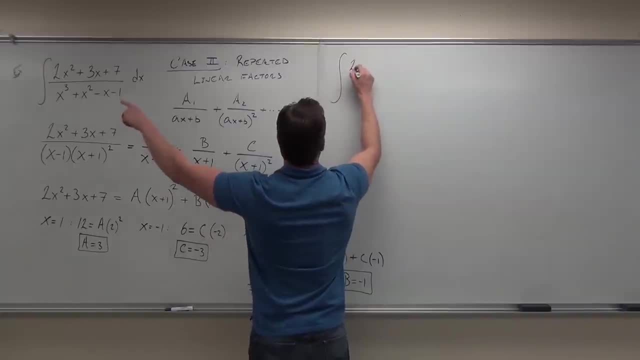 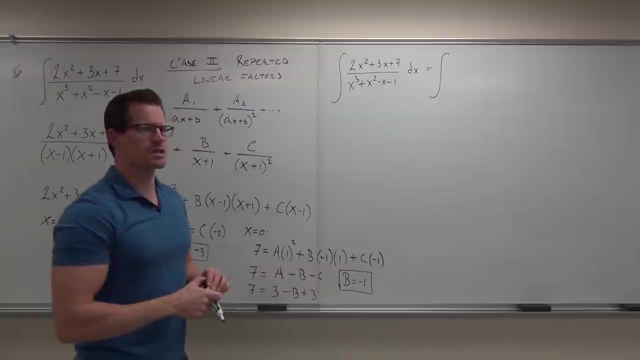 So what we know is that our original integral of 2x squared plus 3x plus 7 equal over x2, the third plus x squared minus x minus 1 dx is now equal to a brand new integral. Let's put this thing all together. 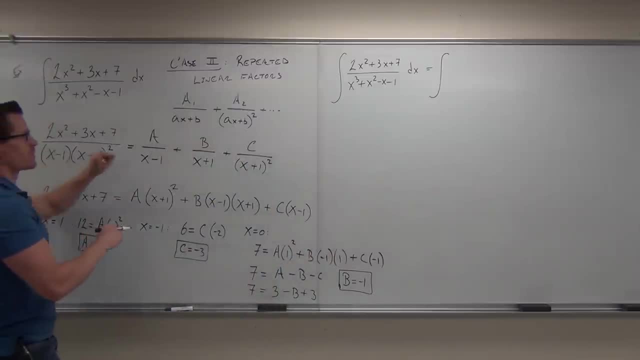 What we knew is that partial fractions said this can be broken up like this. 1, 2, 3 fractions. 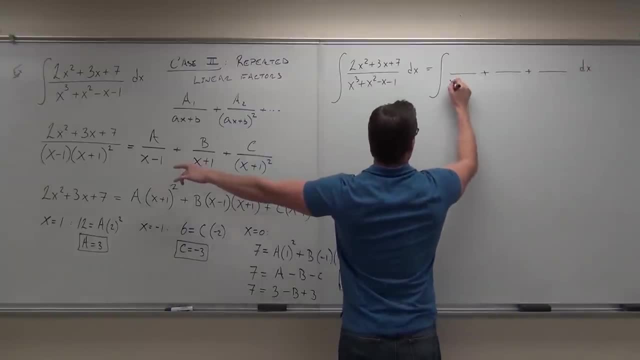 What it said was my denominators are x minus 1. That's going to be easy. x plus 1. That's going to be easy. x plus 1 squared. A little different, but not such a big deal. 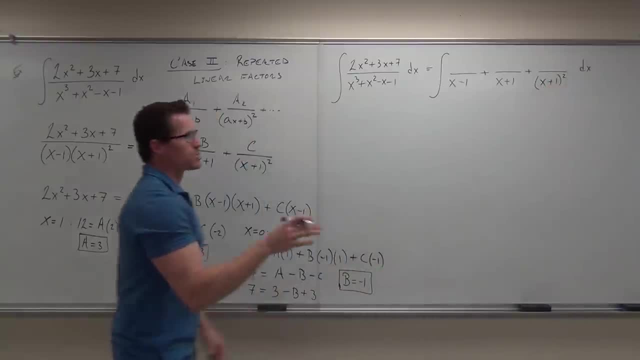 On the numerators, it said that, well, provided you find a common denominator, we did, and can solve for these coefficients, a, b, c, we did, then you know the coefficients of your fractions, or basically the numerators of your fractions. 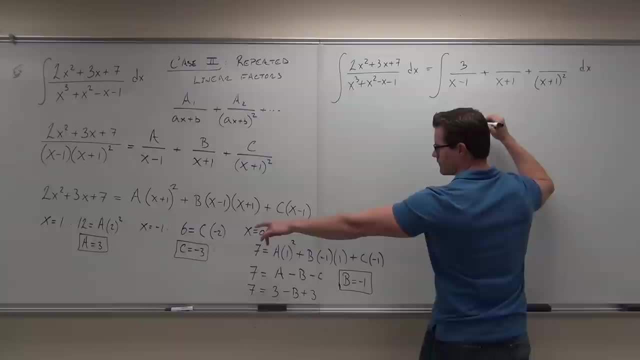 3. Don't get these out of order, OK? 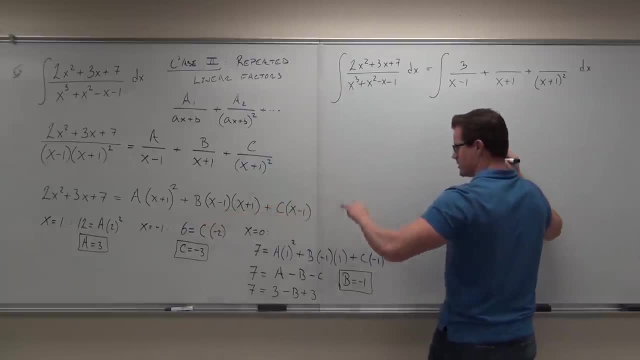 3 from a, and then? Negative 1. Yeah. 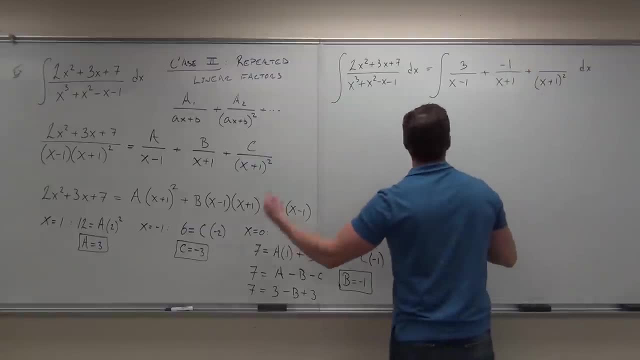 Negative 1 goes here. You guys OK with that? And then lastly, it's? Negative 3. Oh, man. OK. 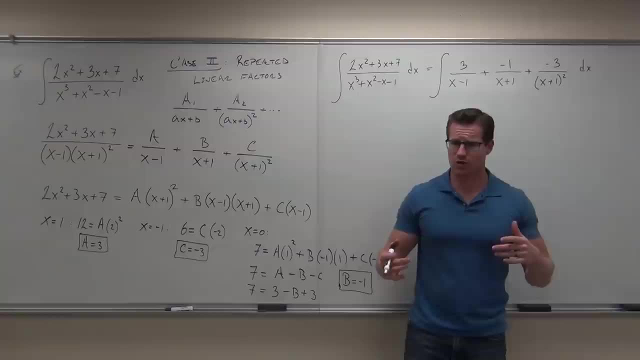 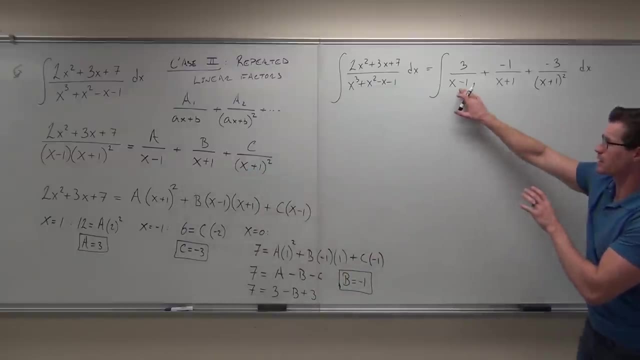 I'd probably clean this up a little bit. We just want to make sure our numbers are correct. So put them in the same order you did it, OK? So x minus 1, x plus 1, x plus 1 squared. We're going to double check. x minus 1, x plus 1, x plus 1 squared. We want a over x minus 1. 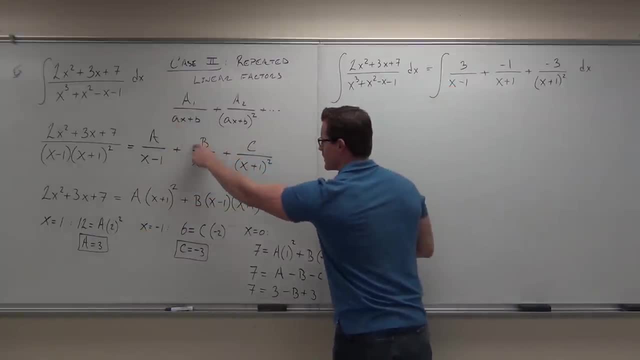 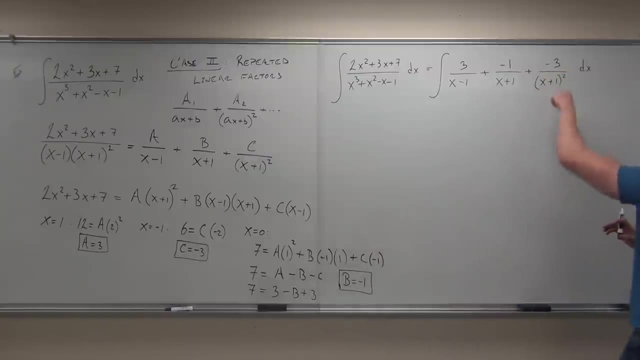 So 3 over x minus 1. We want b over x plus 1. So negative 1 over x plus 1. We want c over x plus 1 squared. Negative 3 over x plus 1 squared. So far, so good? 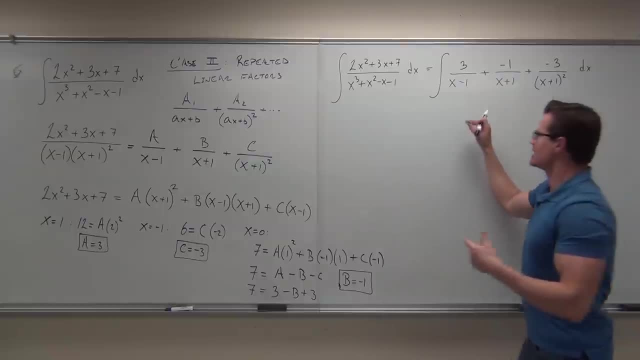 Maybe clean this up, because it's kind of ugly looking. So it said plus negatives. Plus negatives. 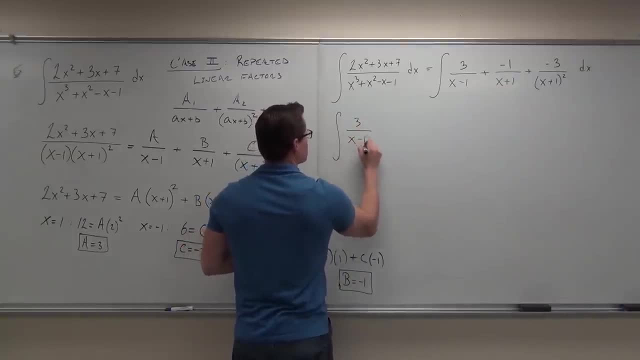 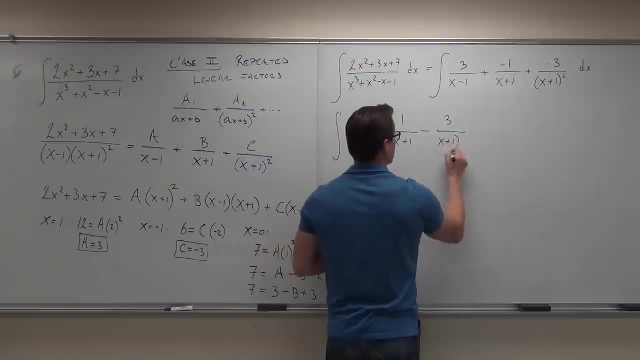 Let's make this integral of 3 over x minus 1 minus 1 over x plus 1 minus 3 over x plus 1 quantity squared dx. 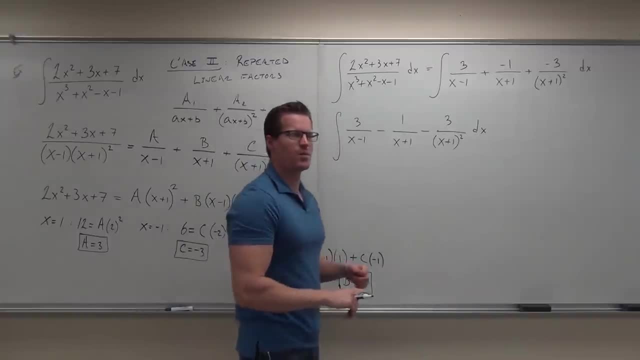 Let's see if you remember how to do these. Remember how to do this integral? Yeah. That's not bad at all. What's that going to be? 3 over x plus 1. Absolutely wrong. 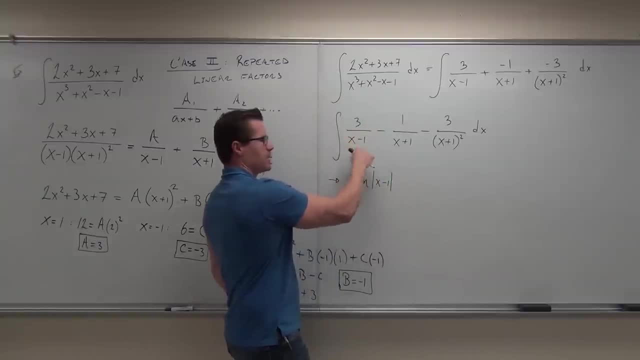 x plus 1. Sure. It says u sub. We do it in our head. The derivative of x plus 1 is simply 1. 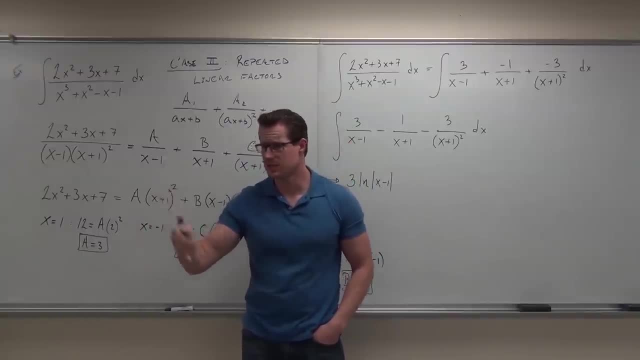 So dx equals du. It'll be d. So this would be a constant 3 ln x plus 1 in absolute value. So far, so good? Yeah. 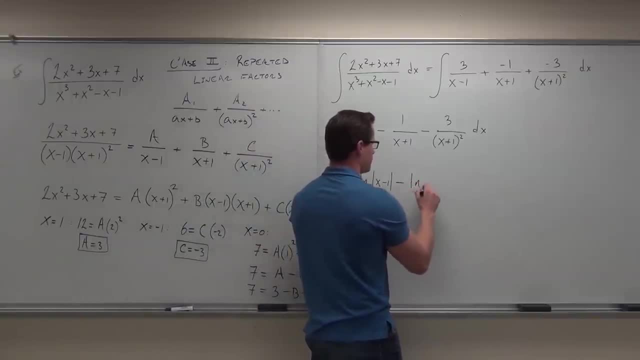 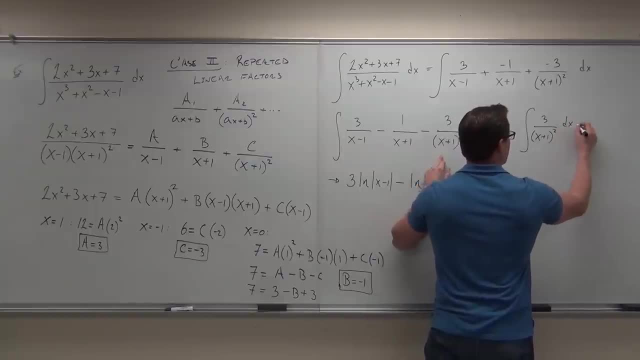 They teach you substitution in calculus 1, don't they? Yeah. Yeah. Yeah. Yeah. Yeah. Yeah. 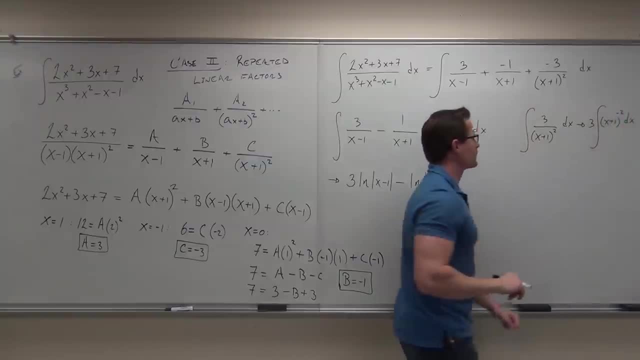 Yeah. 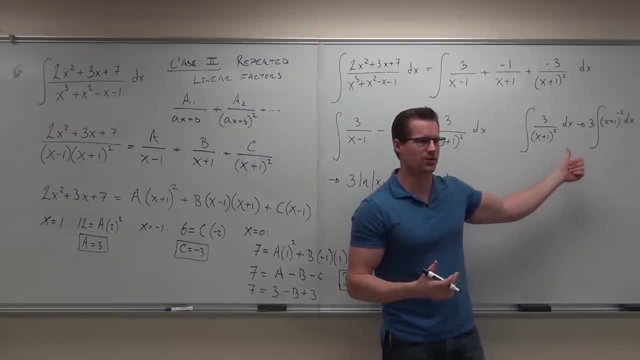 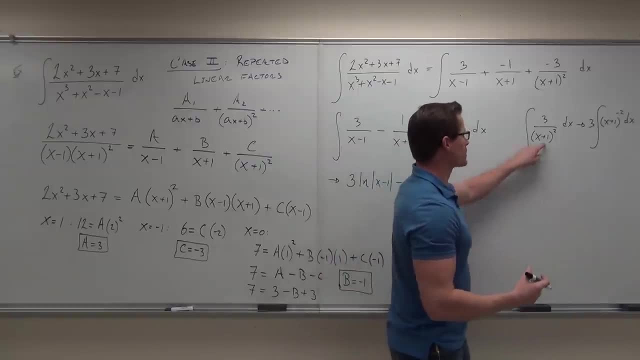 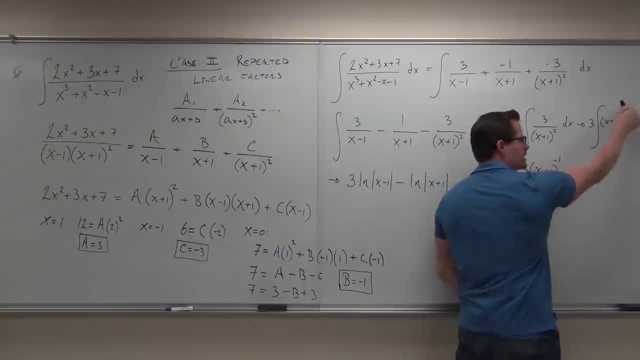 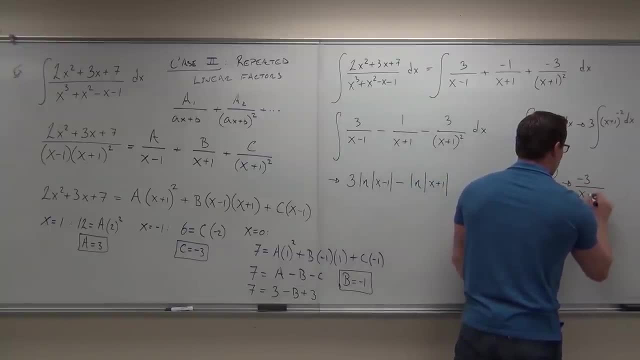 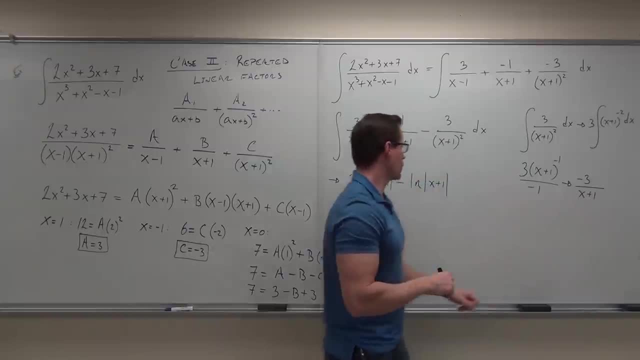 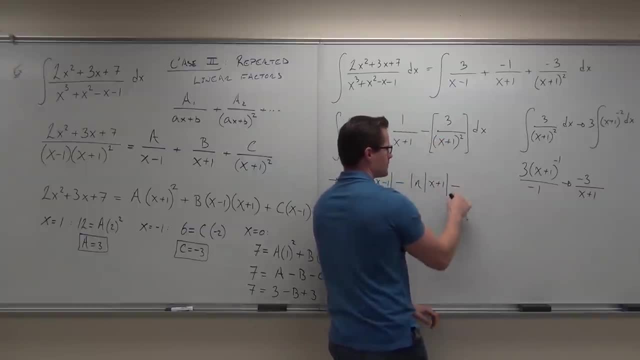 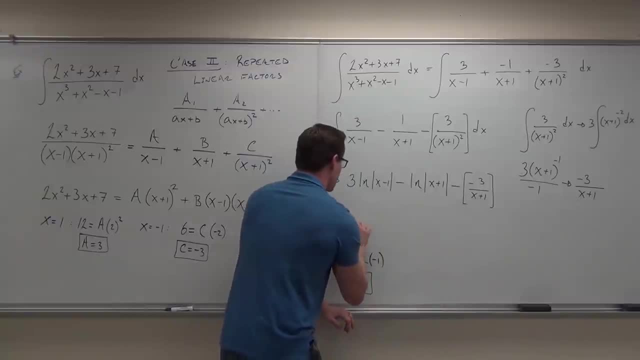 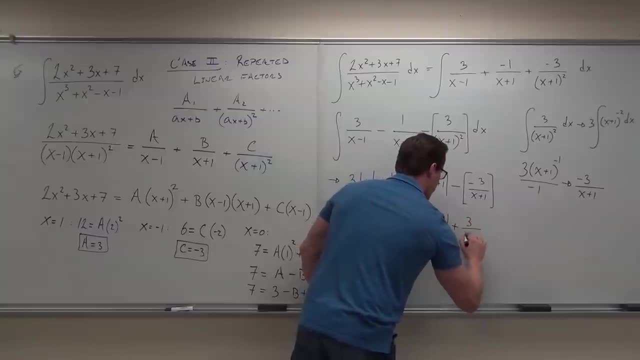 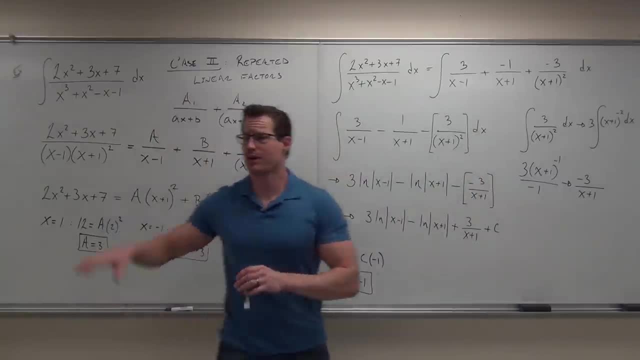 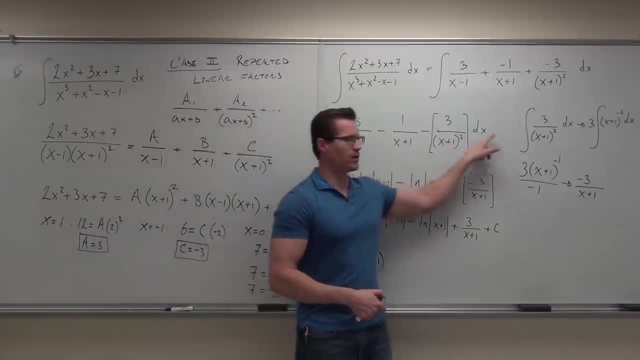 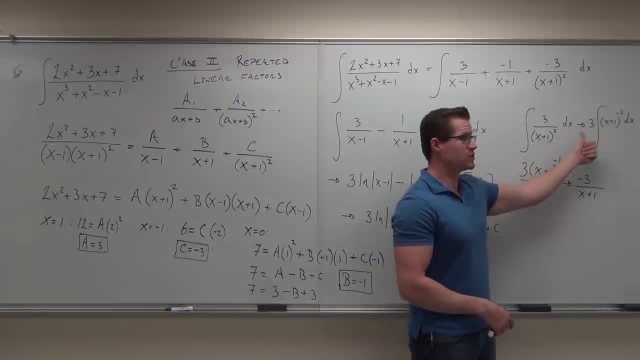 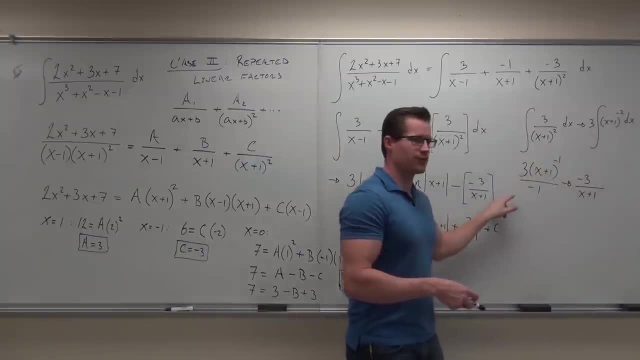 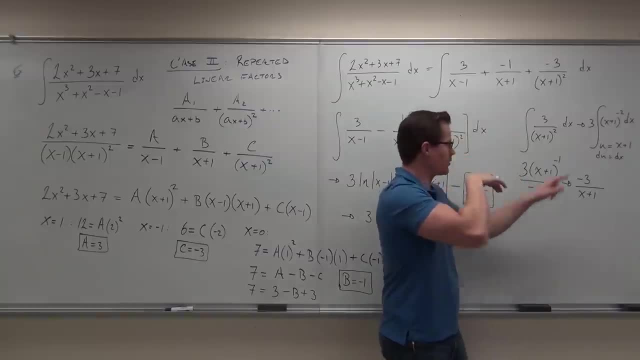 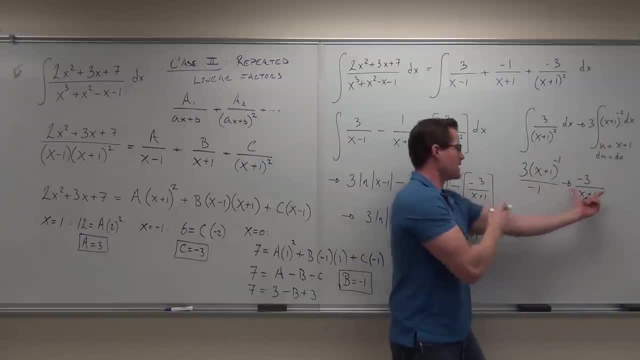 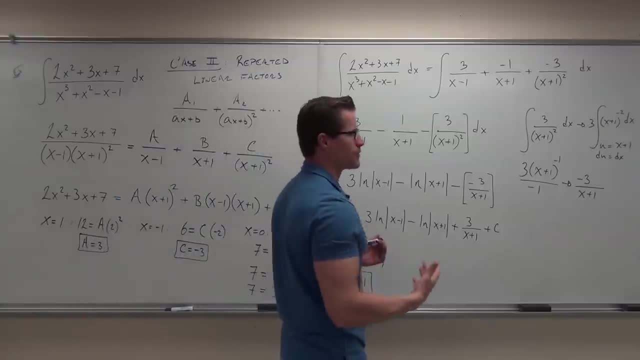 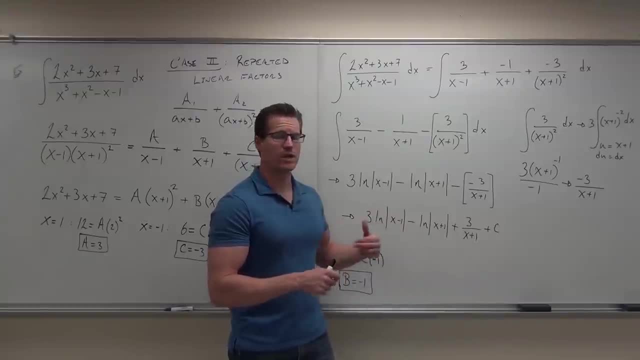 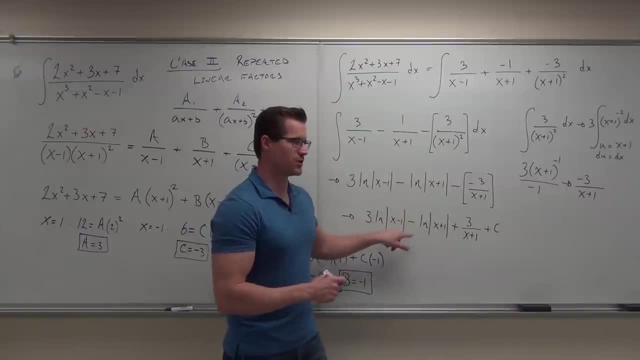 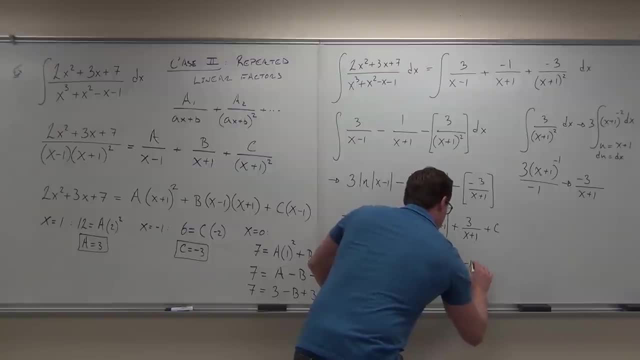 Yeah. Yeah. Yeah. Yeah. We have a problem here. That was a problem. Let's all face it then. To the other way. The other place. Right. Right. Both. Yes. Good. Then I have a problem. Let's do a top charter and a diagonal. Okay. One couple we'll show. One couple. Let's take this. The other one is Jacob's formula. It has a pedir. that's gonna x go around x minus one. 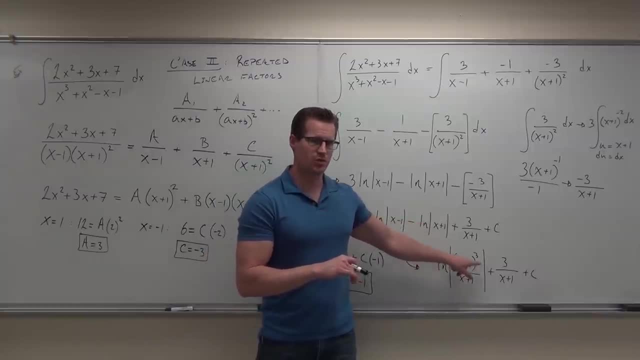 Subtracting two ln's is a division problem. Notice the cube does not go to both, it goes just to this first one, your numerator. 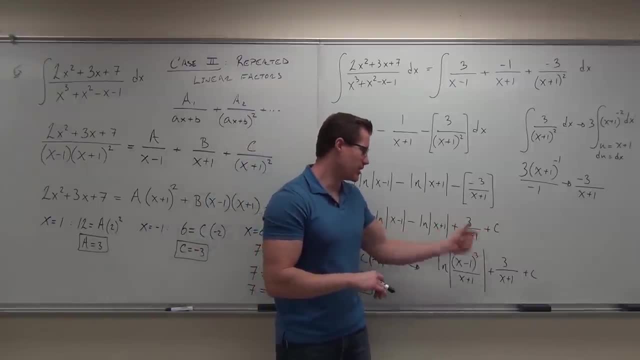 Are you okay with that one? Can't really do much with this one, so you leave it, but that's another way you can see the answer here. 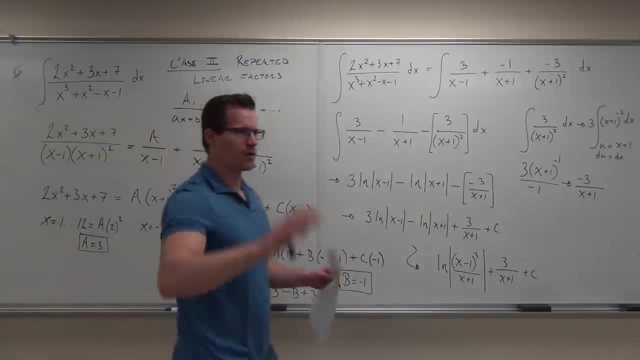 We sure we okay with that? How many of you feel all right with that one? You guys ready to move on a little bit? Are there any questions, comments, or concerns? Am I making this straightforward enough for you guys to understand it? 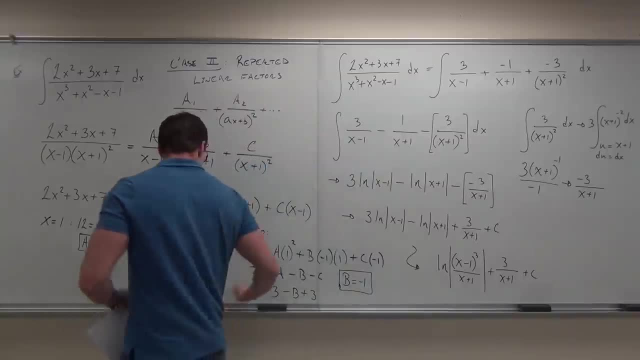 Okay, well, there's a couple other cases that we gotta master, so let's continue moving on. 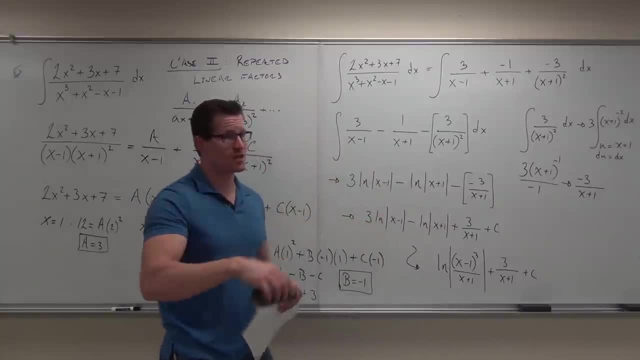 Most of these are gonna take us at least one space of the board, so if there's any questions I need to know now, I'm gonna erase most of it. You got it? All that nice work. 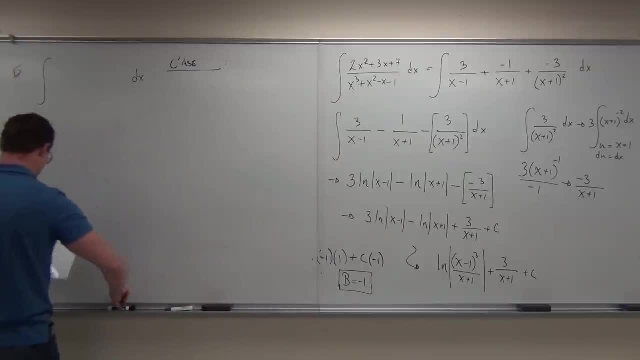 All right, here we go. Oh my, okay. Well, that looks fun. 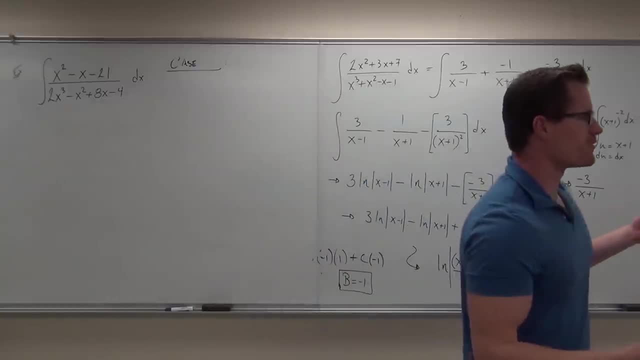 Let's go ahead and do that one. Let's run through the whole process of solving integrals, all right? 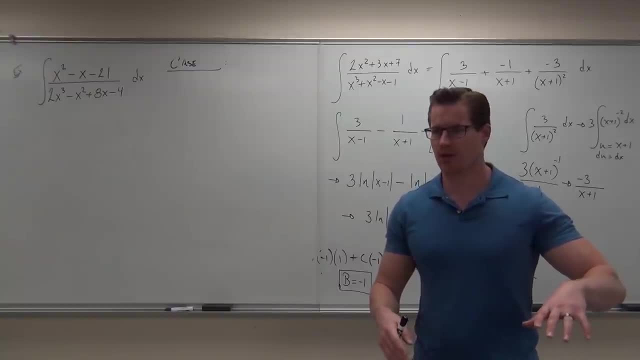 Because on your test that I'm gonna give you, I'm not gonna tell you what to do. You're gonna look at it and go, oh, yeah, okay, I know what to do here. 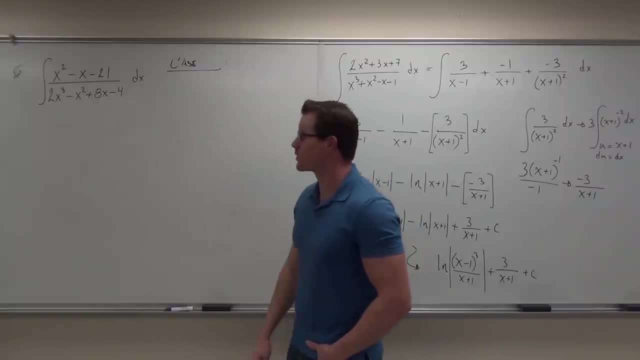 So let's pretend this is a test situation. You look at this problem and go, go ahead and do it. And you go, what do you check for first? 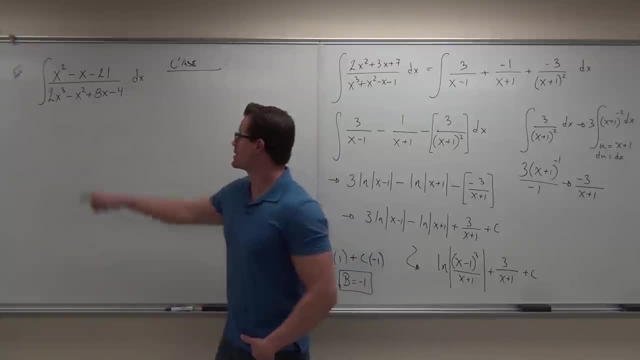 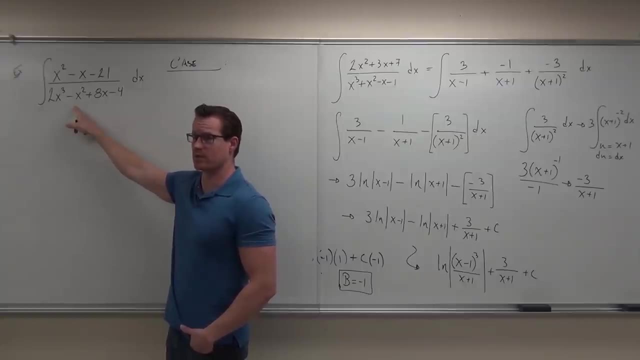 I would check for substitution. Honestly, that's what I would check for. Is this the derivative of this thing, disregarding constants? It's not, but I'd check that first, because if it is, that's an easy problem. That's really, really fast. You with me? I'd check it first. 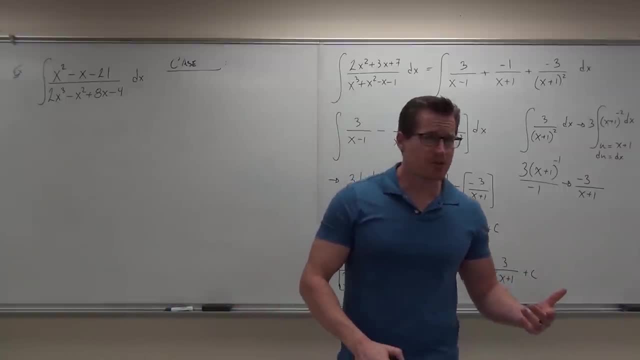 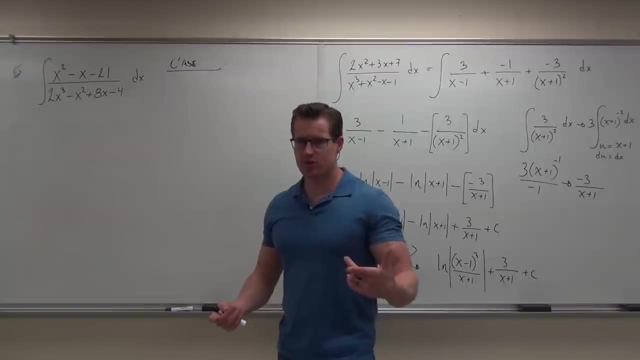 Anything like a integration by parts? It's not a product. Those are typically products. Does it have any trigonometry in it? Any square roots or something we can turn in trigonometry? Any completing the square? No, it's a cubic. Partial fractions. 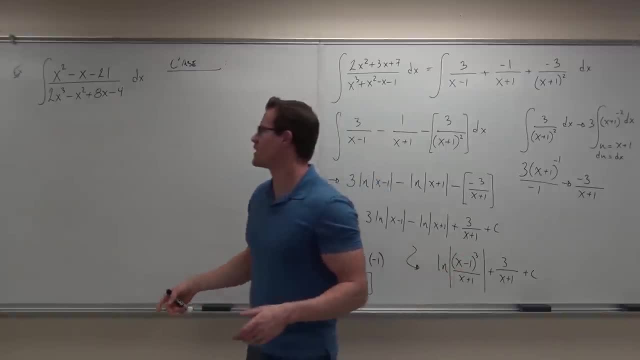 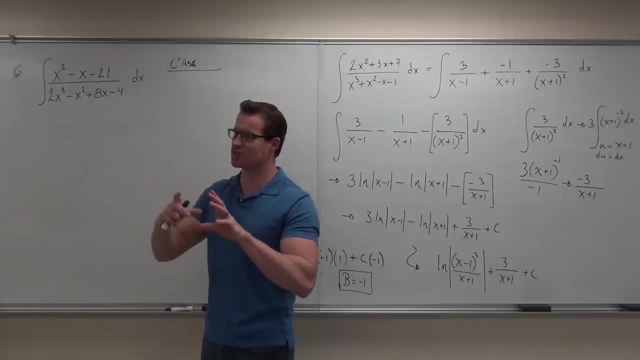 Yeah, looks like a partial fraction to me. Something we could use partial fractions for. The first thing we check, I think you guys said it first, what do we check? The degree. Yeah, degree on the numerator has to be less than the degree on the denominator, or you do what with it? A function. 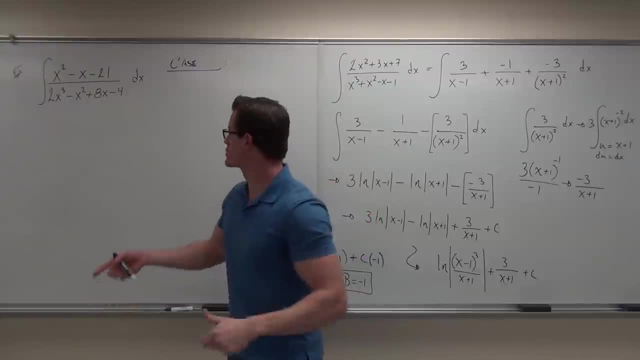 Yeah, and that reduces the degree of the numerator for you. So that's great. So here, we're good to go. 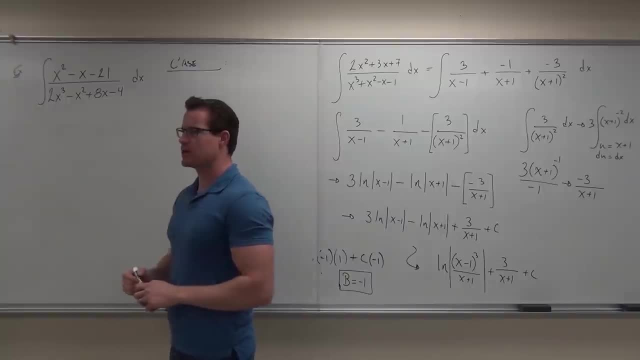 No long division necessary, thankfully. Okay, now that we've determined that we're gonna do partial fractions, what's your first step? Grouping. Break it up. 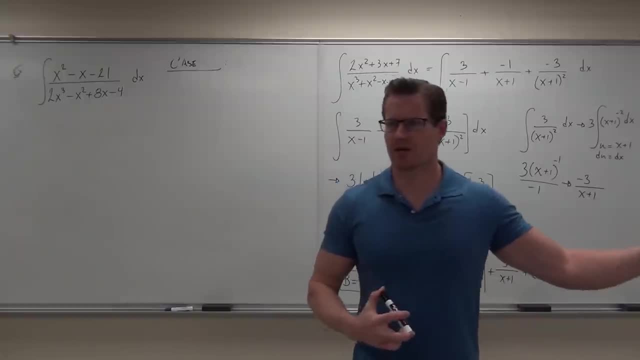 We're gonna get it factored. Yeah, we're gonna factor it, and we're gonna factor by, Aaron said we're gonna factor by grouping. Why don't you try and factor by grouping? Go for it. Okay. Okay. I'm wondering if you got the same thing I did. 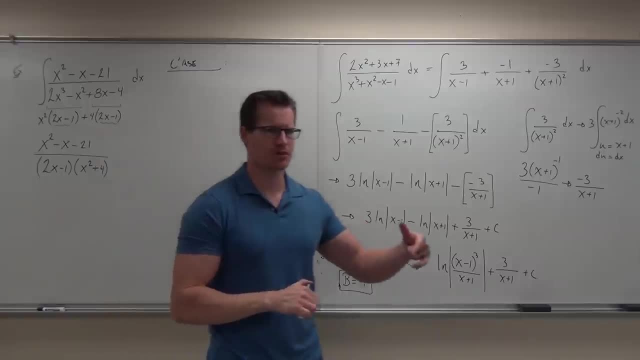 Did you get two x minus one, and then did you get x squared minus four? Yeah, plus four. Oh good, I was texting you. You passed. Did you get a plus four? Yeah. If you got, let me have your eyes on the board here, real quick. You guys okay with the grouping? 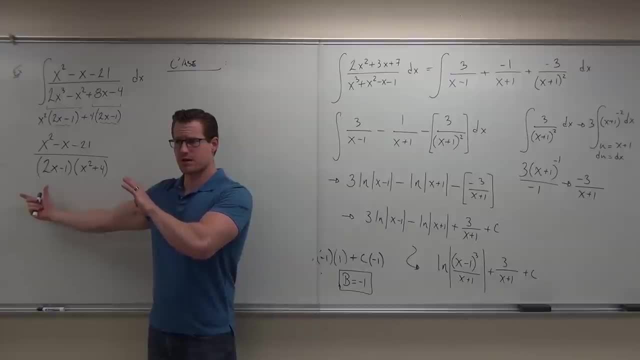 By the way, you'll notice what I'm writing is the linears first. You see that? 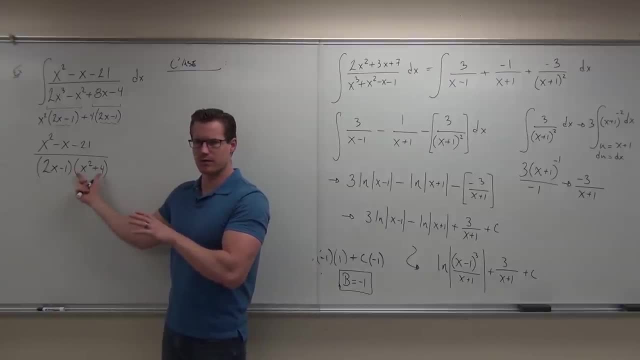 Now, if you had an x squared minus four, would you stop right here? If you have an x squared plus four, do you continue going? Can you factor x squared plus four? No. 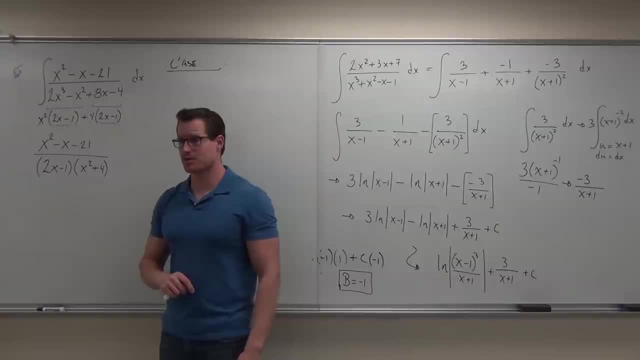 If you start factoring this as x minus two x plus two, your problem's going down the poopy hole. 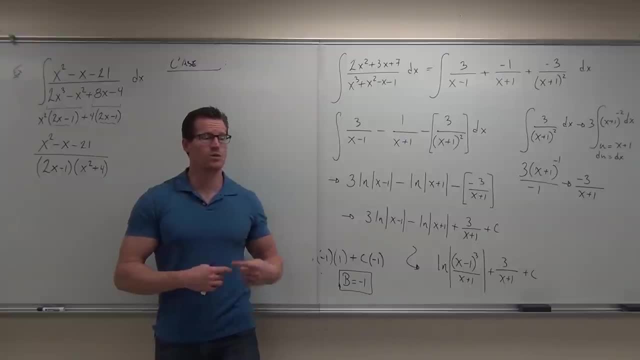 All right, that's not good. We can't start factoring like we don't know what we're doing here. 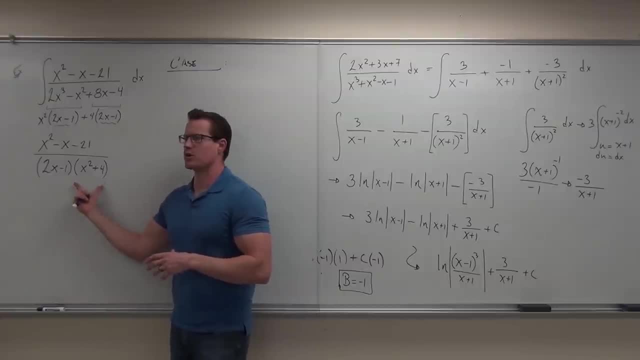 So, this is your first case. This is your first case of an irreducible quadratic. That's this next case right here. Case number three is when you have irreducible quadratics. 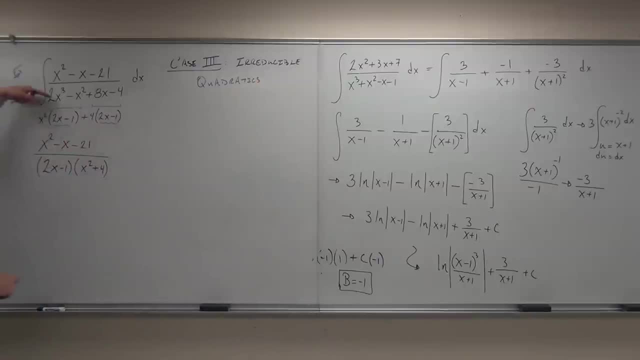 Irreducible quadratics. So, we've factored by grouping, it worked. 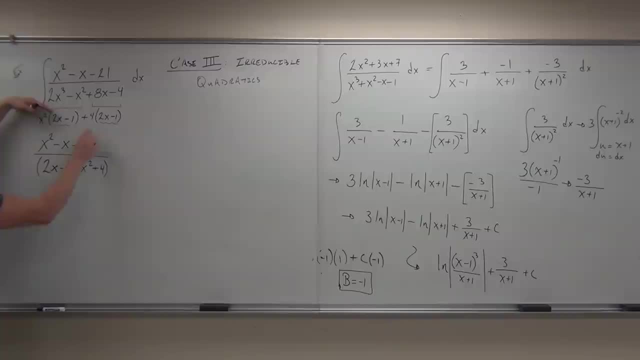 We have two x minus one, no problem. The remaining factor is x squared plus four. 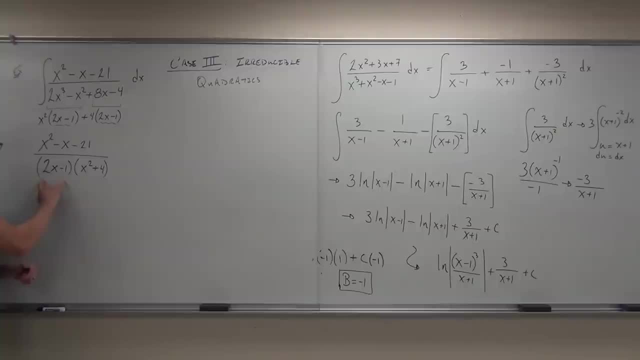 This one, okay, what is this? Is this a quadratic or is this a linear? Linears, you're automatically done. There's no more factoring in that. You're done. 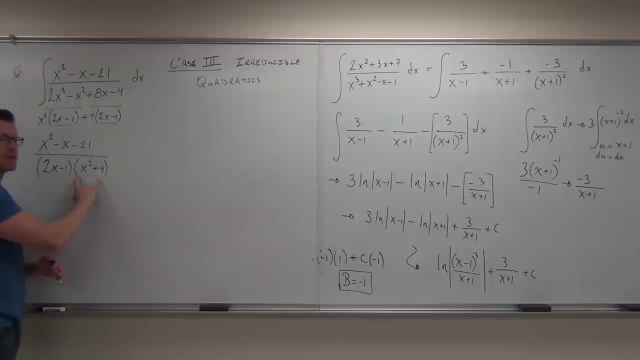 Is this a linear or quadratic? Quadratic. Can you reduce it more? Then it stays an irreducible quadratic. we write the irreducible quadratic. 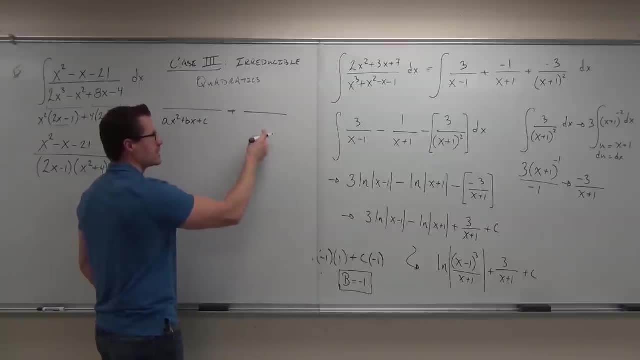 If we have powers, we'd write it again and again. So, we write the first irreducible quadratic, then the second irreducible quadratic. 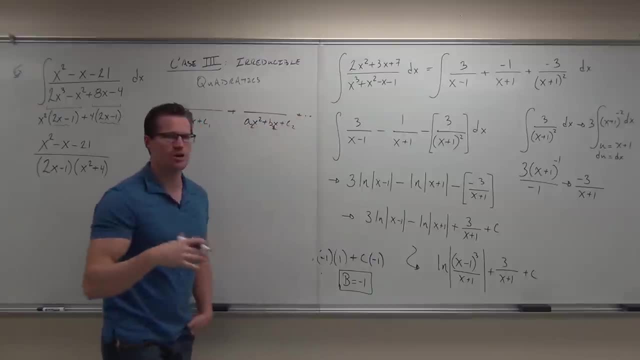 Two, two, two. And then the third one and so on until we exhaust all of our irreducible quadratics. 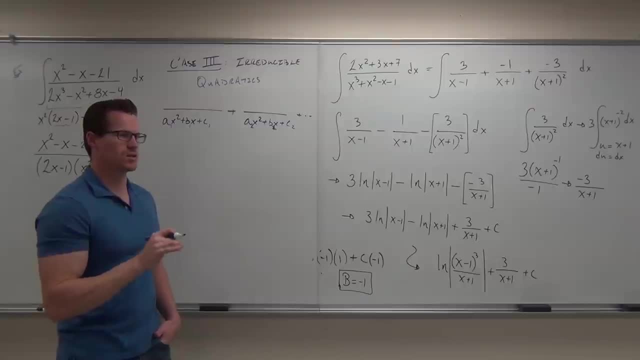 And on the numerators, hopefully this makes sense to you. 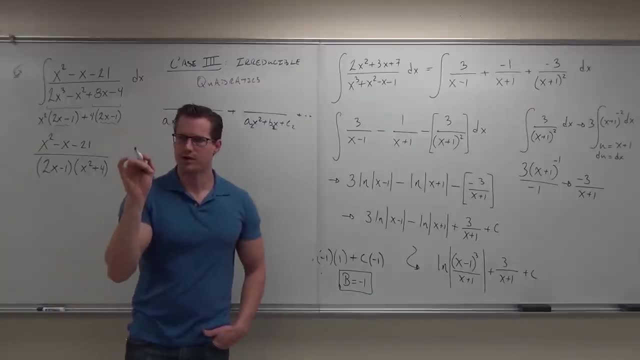 Whatever factor you have, your numerator should be one degree lower than that. So, for linears, one degree lower than a linear is a constant. One degree lower than a quadratic is a linear. 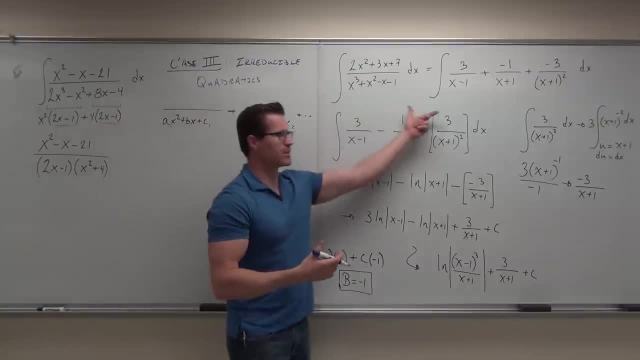 So, for linears, we'd have, that's what we had here. We had a, we had b, we had c. One degree lower. Does that make sense to you for our linears? 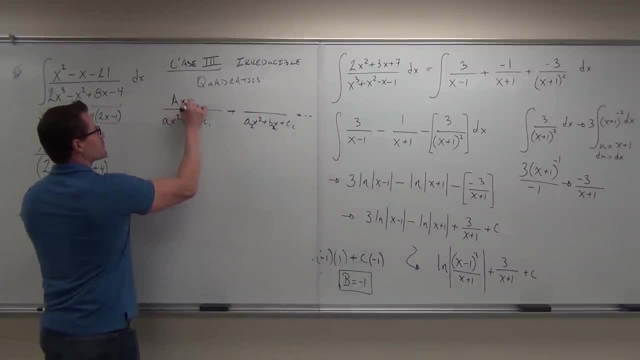 For quadratics, we're gonna have linears. Ax plus b. 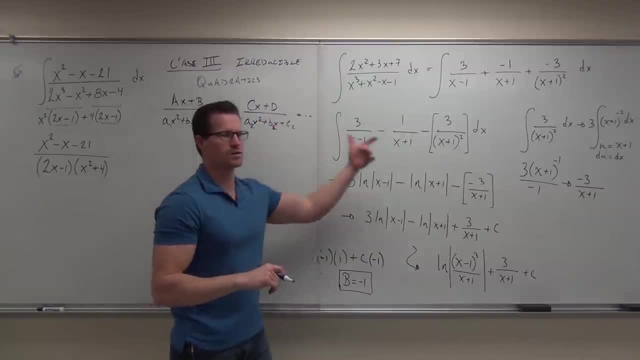 Cx plus d. And so on and so forth and so on and so forth. This is the idea here. 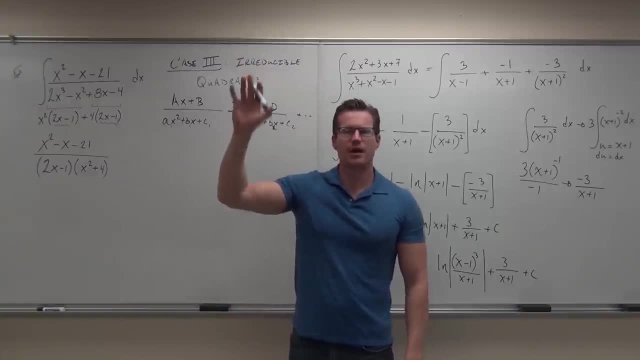 So, if you feel okay with that one. Now, let's put that into practice with our problem here. 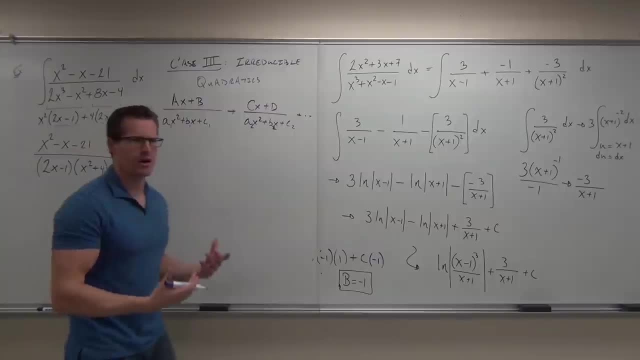 So, notice how our cases are kind of, they're building, right? We're building on what we already know. 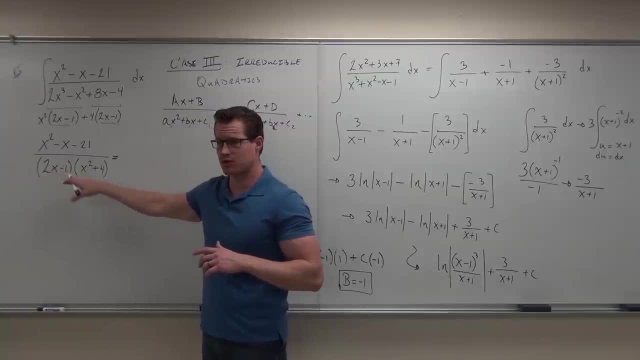 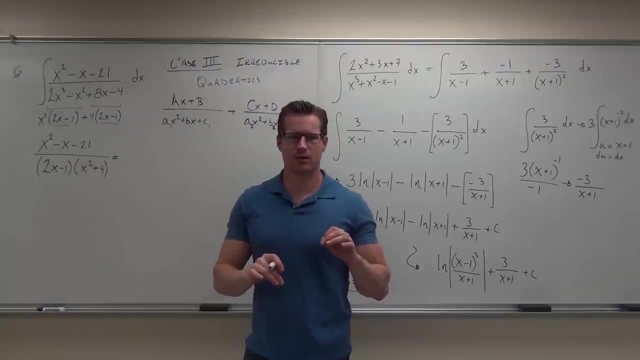 So, if you have a linear and you have an irreducible quadratic, you can do two different things in the same problem. How many fractions are we going to have here? What do you think? 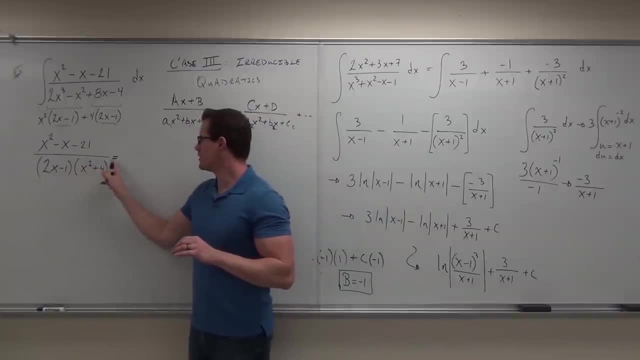 Are there any factors to a power? No. Okay, so this is one factor. This is another factor. Are they repeated? No. Okay, that's our next case, okay, is when you actually repeat these. So, is this repeated? No. That's just one factor. 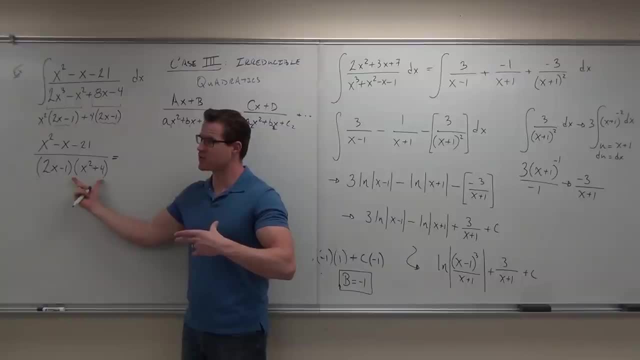 Is this repeated? No. That's just one factor. You can't reduce it, right? So, it's irreducible quadratic. That means you're gonna have two fractions. 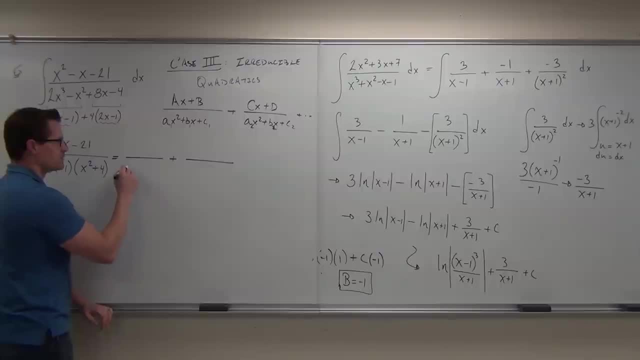 Okay, tell me, folks, what's gonna be on my first denominator? Two times minus five. 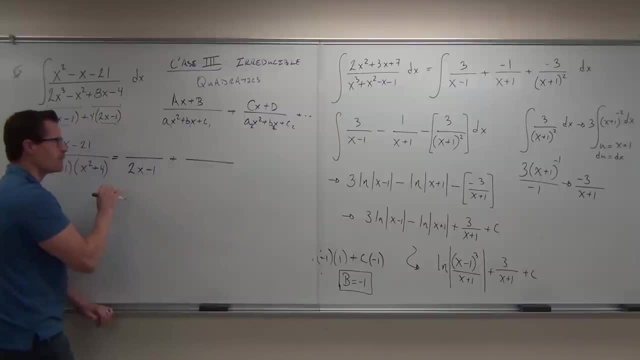 Is that linear or quadratic? I know I've asked it, but is it linear or quadratic? Linear. Okay, what's on my next fraction? A third fraction. Linear. Is that linear or quadratic? Quadratic. And it's irreducible. 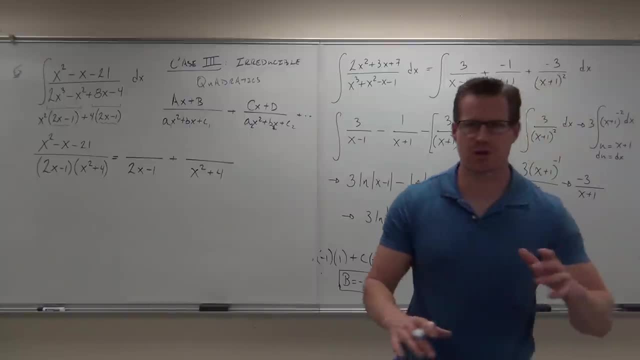 Remember, you gotta make sure that you have simplified this or factored this as much as possible. Show of hands if you're okay with this so far. It's the same idea. 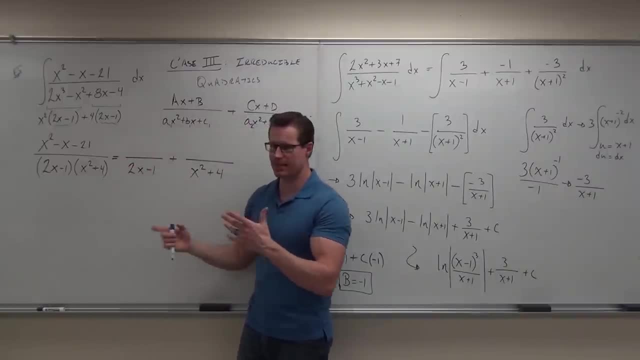 You have a number of factors. Make a fraction for each factor. That's it. 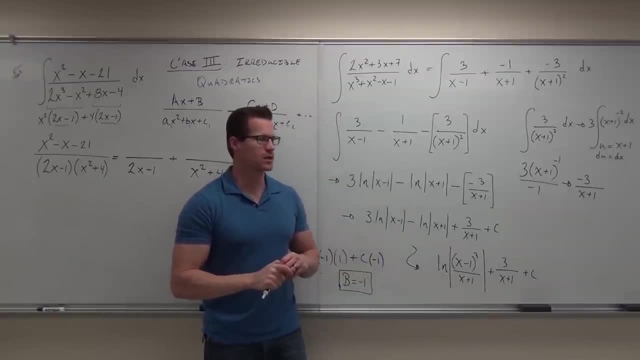 Now, on the numerators, it's important you get this right, get it correct. 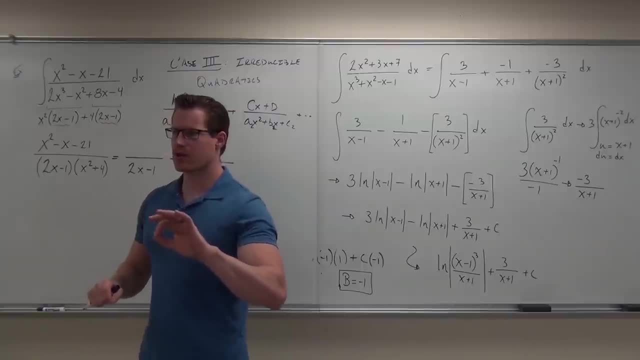 For every linear, we put a constant. For every quadratic, we put a linear, one degree lower than what we have. We do that for every single fraction. 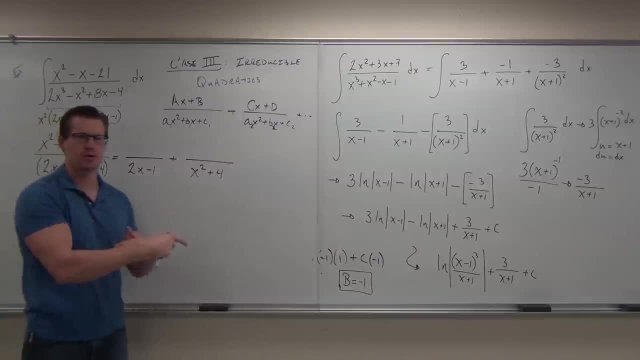 Typically, this is why I write my linears first and then my quadratics so I don't lose any. 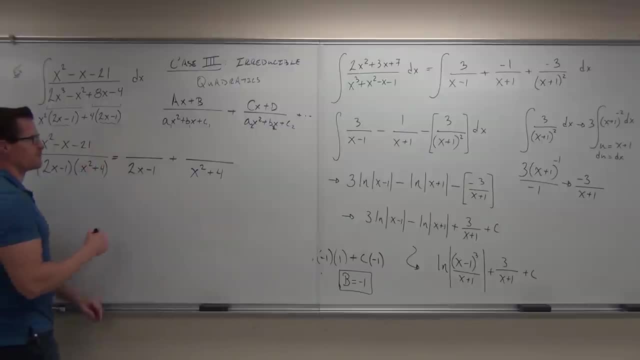 Okay, so I'll have to go back and forth. So here, what's gonna be here? A. That's right. What do I want? Do you want AX plus B? No. No, it's linear. I want a constant for linears. How about this one? 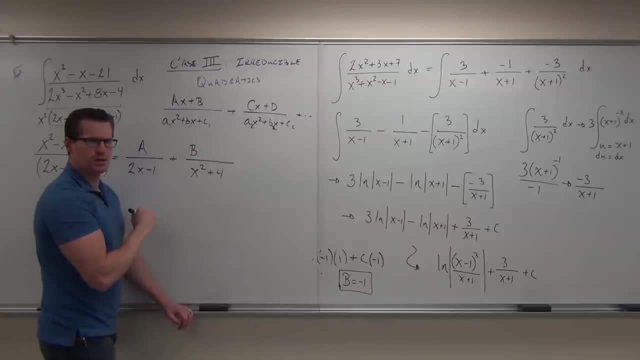 B plus C. Just a B? BX plus C. Good. 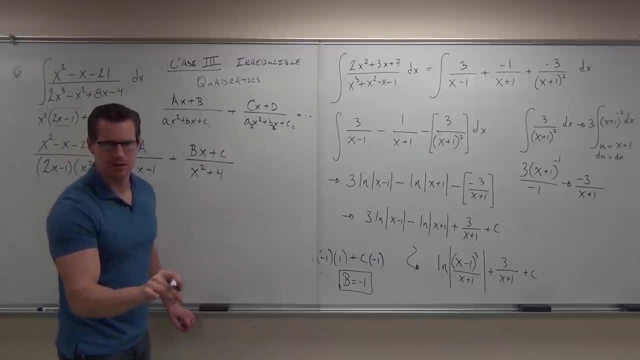 What I want is a linear for a quadratic. So, constants for our linears. That's what we've been doing here, folks. 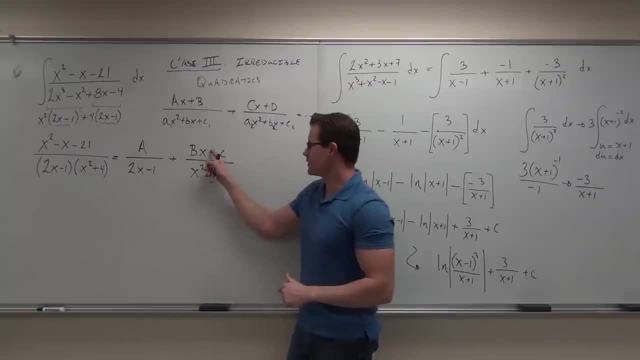 That's what this is. Then, a linear for my quadratics. Notice how the degree is one lower. This is X to the first and this is X to the zero. This is X to the second. 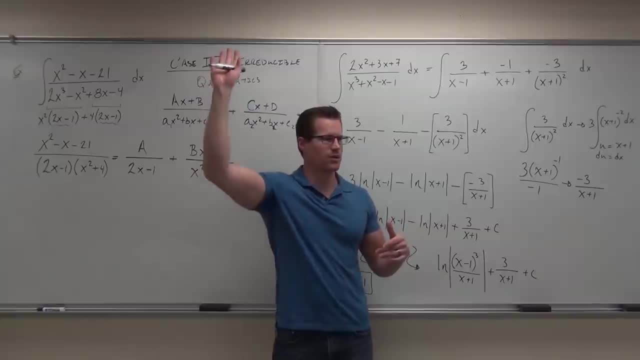 This is X to the first. It's one degree lower. That's the whole idea. So, you guys feel okay with that one? Then you're good to go. That's it. 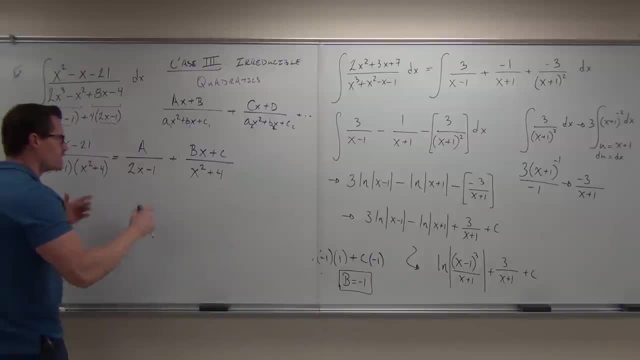 Same stuff after this. So, why don't you guys go ahead and tell me what I would do to get a common denominator on my first fraction. 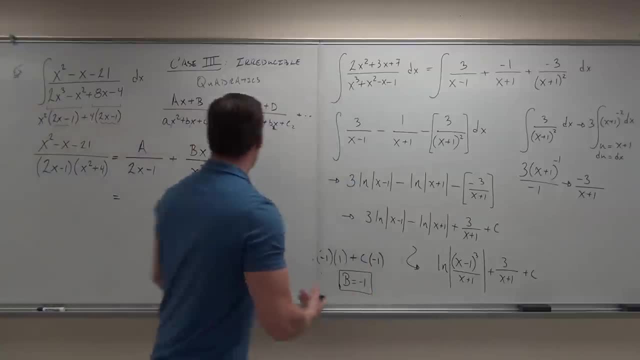 What's the missing factor here? Remember the way I do it? I look here. And I look here. What's missing from here to here? 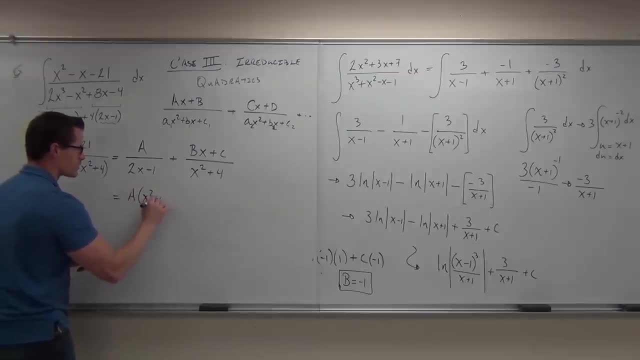 X squared plus four. So, I have A and X squared plus four. 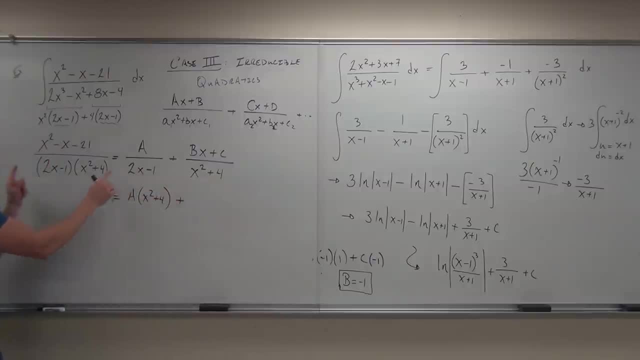 Plus. I look here and I look here. 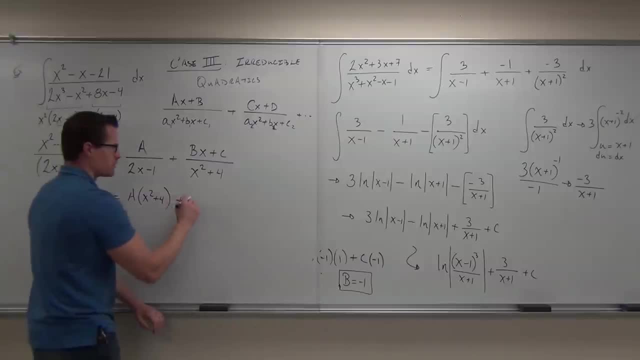 What's missing from here to here? Two X minus one. So, the way this looks is BX plus C. Remember, it's the whole numerator. I'm sorry, what's missing there? Two X minus one. 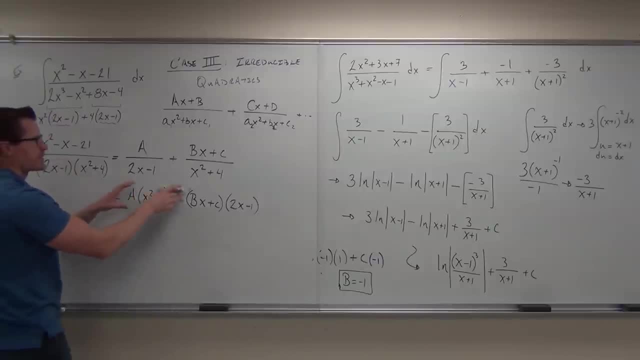 So, again, for the last time, hopefully, we find a common denominator. We multiply by the missing factors on both the numerator and denominator. We do. The missing factors are X squared plus four. 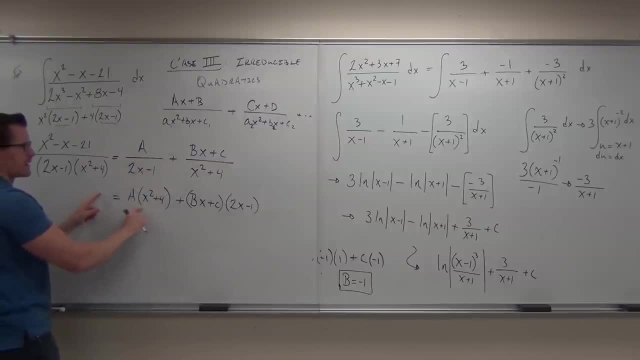 We have this one. We're missing X squared plus four. So, that's why we got our A times X squared plus four. 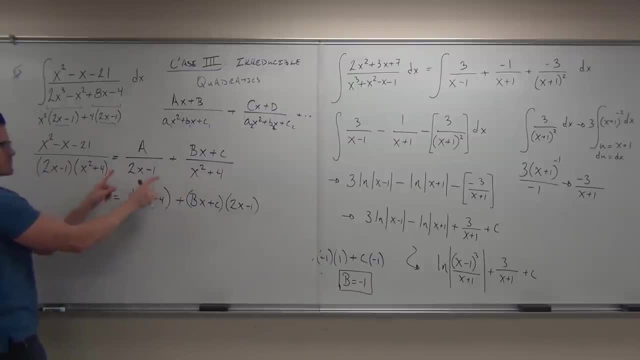 Here, we're missing the two X minus one. We already got this. We're missing the two X minus one. That goes here and here. 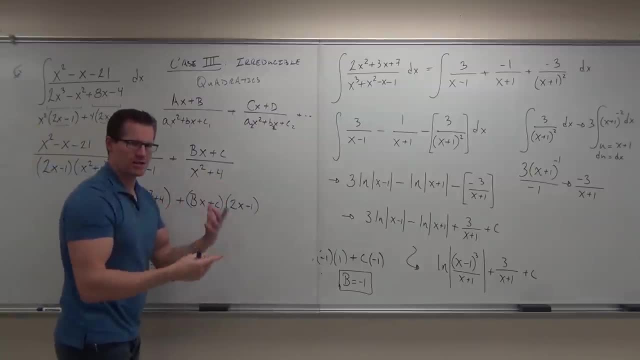 As soon as we get that common denominator, we ignore it. We just set the numerators equal to each other. So, this numerator 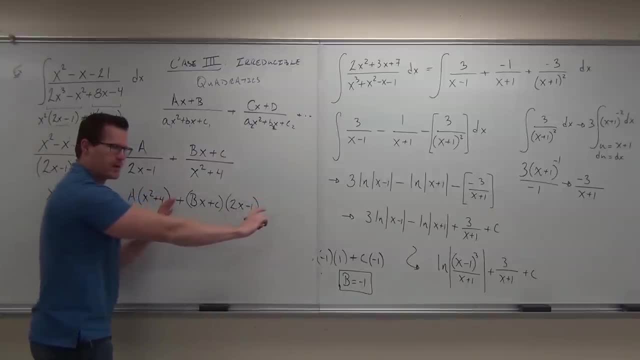 equals this new numerator. This would be the numerator. You follow? Just keep in mind, it's A times this one, this X squared minus four, and then it's this whole BX plus C times the two X minus one. 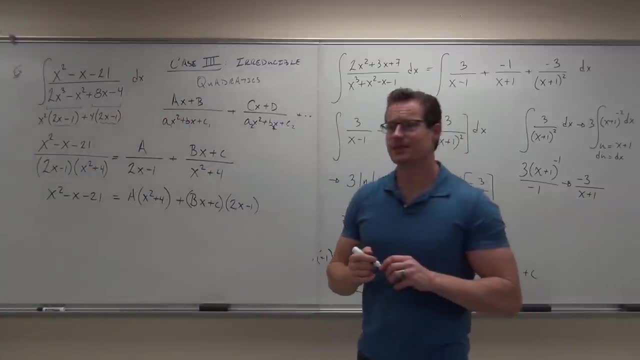 So, you'll be okay with that one. Now, this is what I was talking about 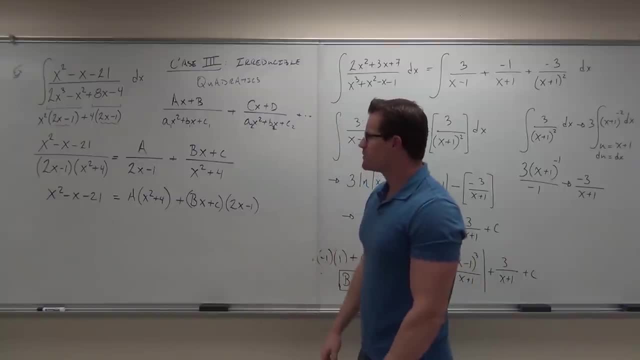 as far as sometimes you can cheat and sometimes you can't. Right now, it's gonna be pretty difficult to cheat at this thing and plug in a number that's gonna work. The reason why it's gonna be a little difficult to cheat is because if we plug in stuff like, oh, I don't know, a number to make this zero, we'd have to come up with one half. 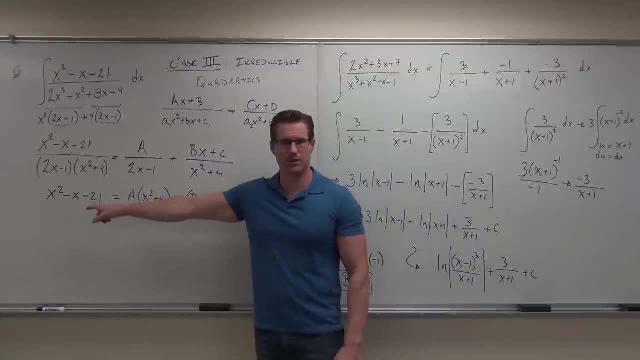 One half's gonna be difficult to plug in here and difficult to plug in here and difficult to plug in over there, okay? 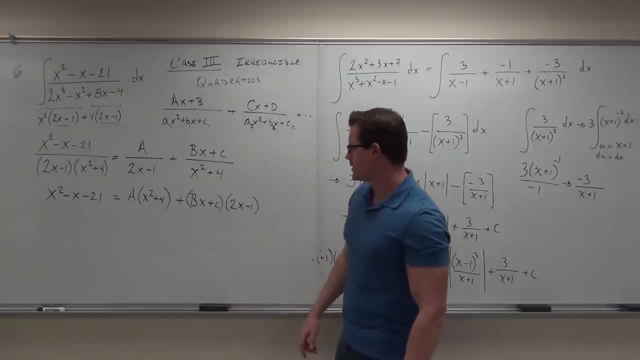 You can do, you can try it. You can't plug in things like zero if you want. 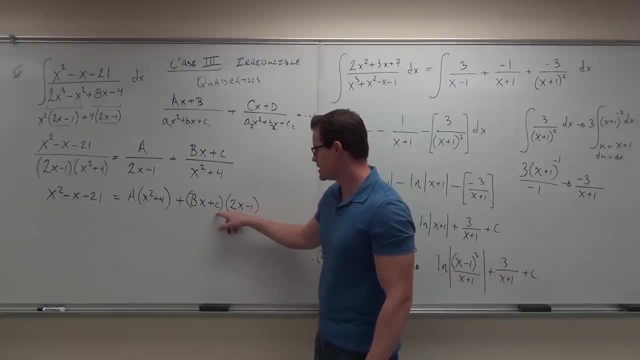 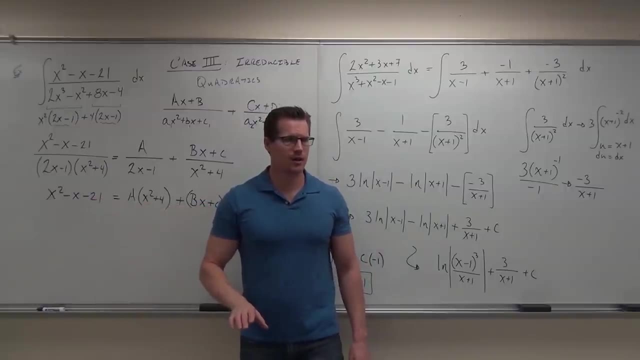 So, zero would give you negative one times C and it would give you four A, and it'd give you equals negative 21, but it's not gonna eliminate everything, all right? 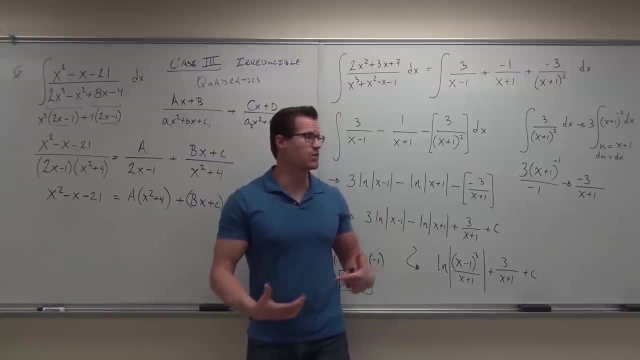 So, sometimes, one of the easier ways to go is just to distribute and actually see what happens. So, that's what I want you to do right here. If you want to do it right now, if you want to plug in some numbers and sometimes you get lucky, do it. That's what I would try every time. 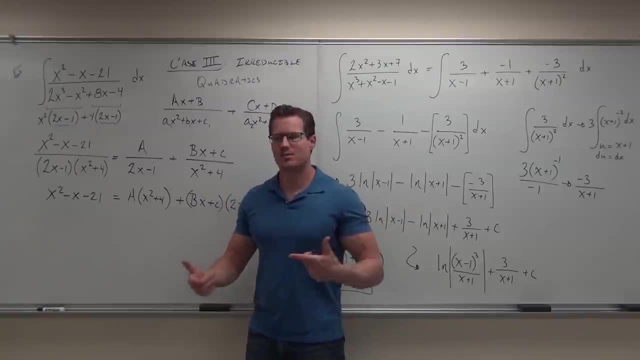 If there's an easy number to plug in, man, do it. But if there's not, sometimes you're left with actually distributing, combine your terms, and going for it. 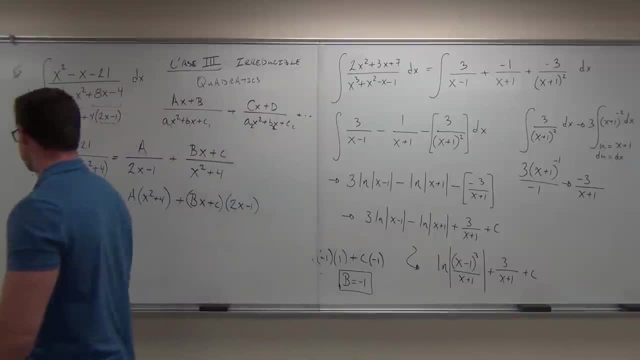 So, go ahead and do that now. Distribute, combine your terms. I'm gonna do it while you guys are doing it. 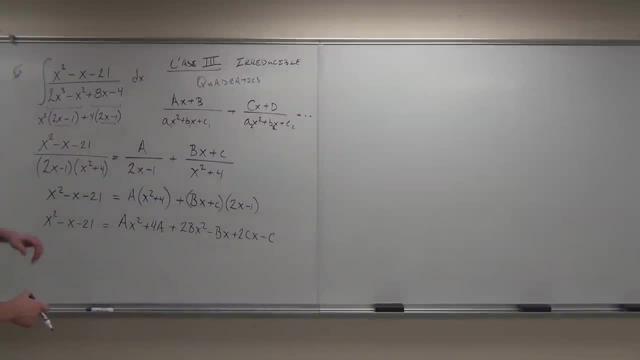 So, let's go ahead and do that. I'm gonna do that. I'm gonna do that. I'm gonna make sure I got that A squared squared. Two BX squared. Two BX squared. 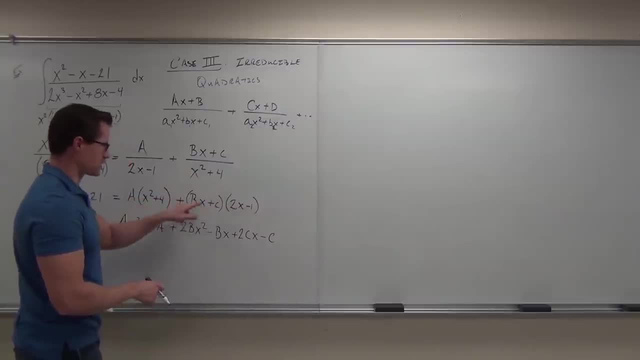 Minus BX. Plus two CX. Did you get the same thing? Yeah. 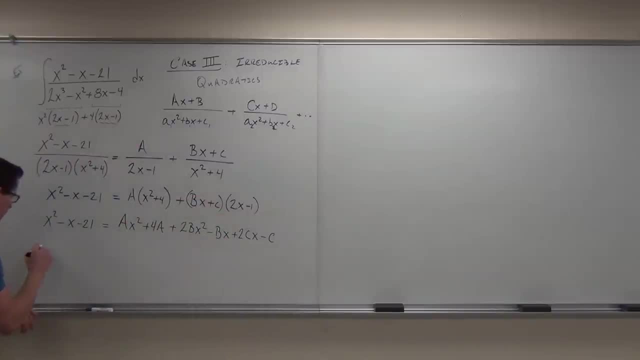 Collect your terms. I see a couple X squares, so I'm gonna have A plus two BX squared, plus two CX squared. two v, x squared, collects some x's. 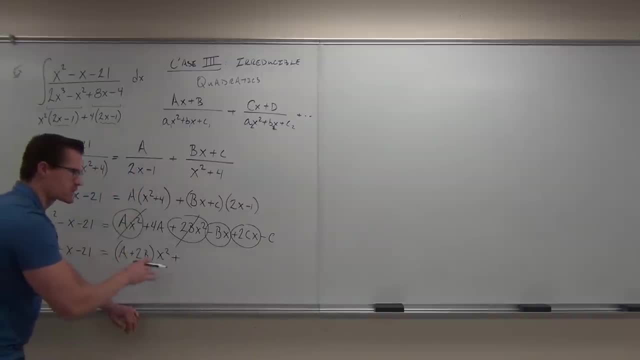 Again, how I do this, I always put a plus, makes it easier for our signs. When we factor, we'll have negative v plus two c, x. 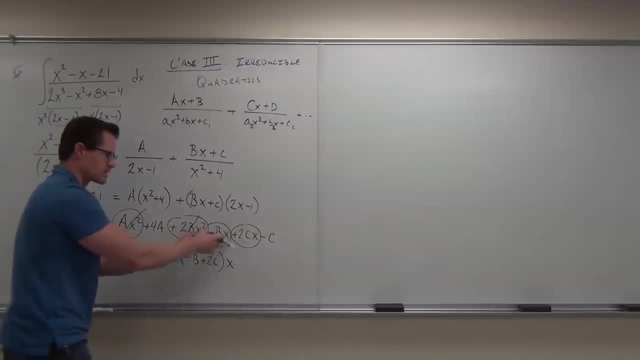 So you guys see what I'm talking about there? We put a plus and then we collect our signs inside of our parentheses, negative b and two c. Lastly, we have plus four a minus c, 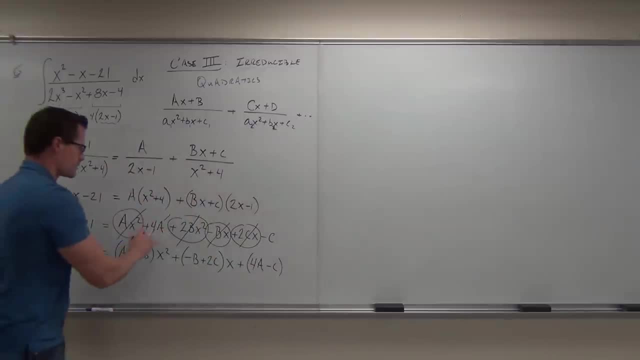 that's our constant, and we got those ones. Did you make it that far on your own? Fantastic. 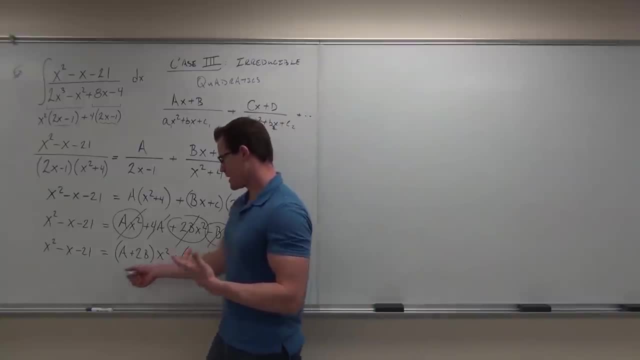 What's nice about this is when we collect our terms, we have x squared, hey, we match it up over here. We've got x, we match it up over here with our coefficients. 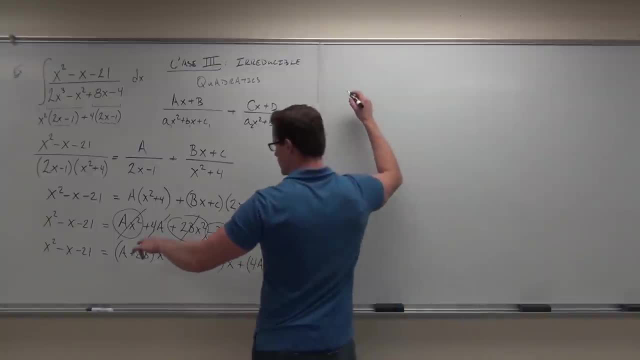 We've got a constant, we match it up with our constants. So you tell me, hopefully you can figure this out, 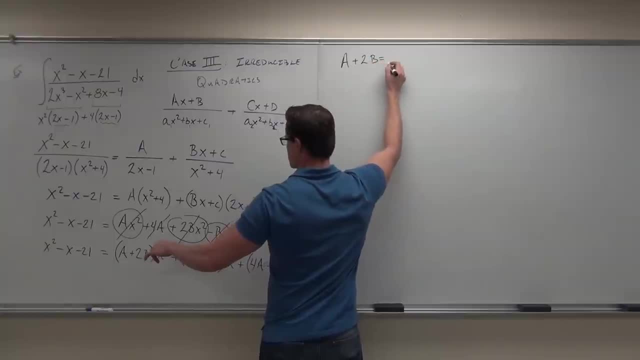 if I put a plus two v, how much is that equal to? One. Where are you getting that one from? From x squared. 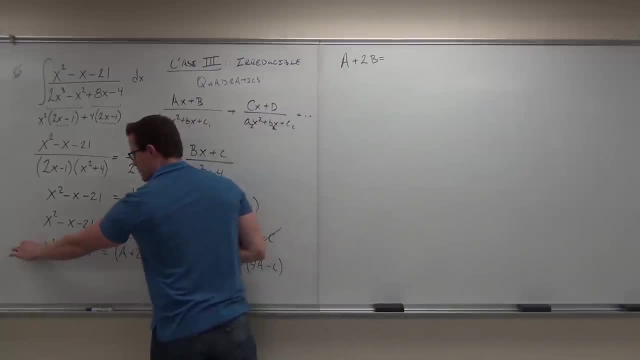 This is the coefficient of x squared, isn't it? This is the coefficient of x squared, isn't it? It's gotta be equal. So one equals a plus two b. 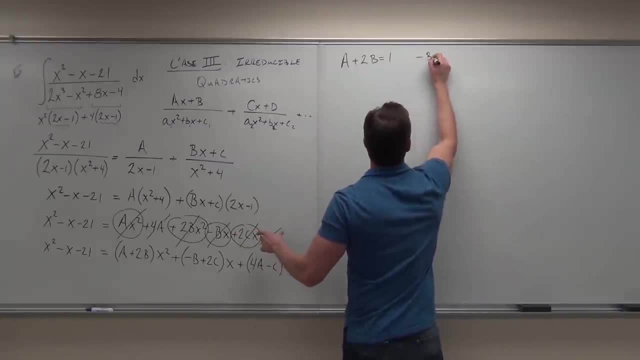 Let's do the next one. If I put negative b plus two c, 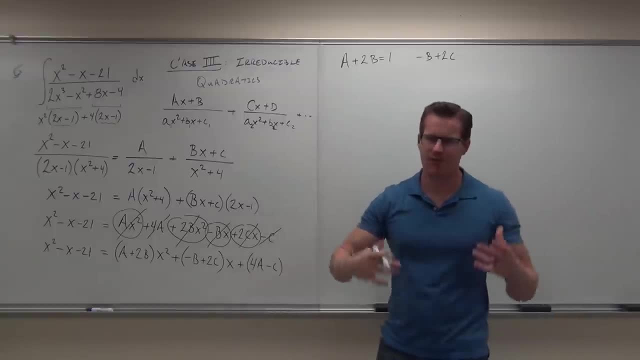 negative b plus two c, how much does negative b plus two c have to equal here? Negative one. 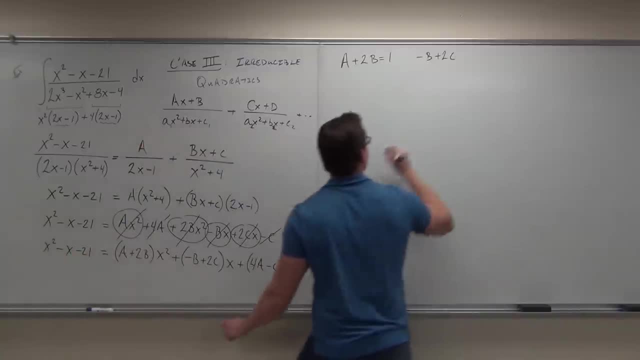 Since this is the coefficient of x, and this is the coefficient of x, you're right. 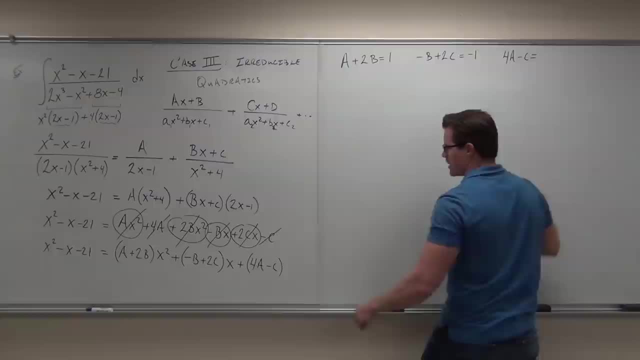 Now, if I put four a minus c, how much does four a minus c have to equal? Negative 21. 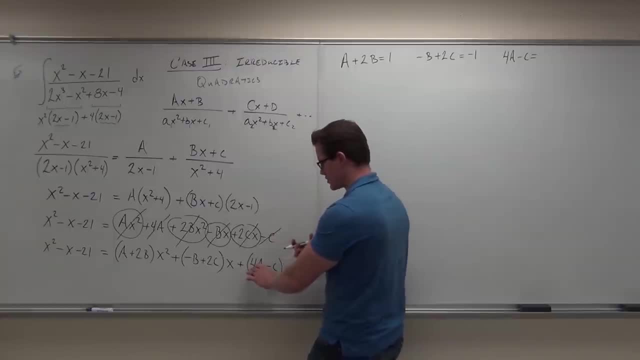 The reason why we use pluses here, it keeps our signs correct. That way you just look here, and here, and here, and set an equal to the coefficients themselves. 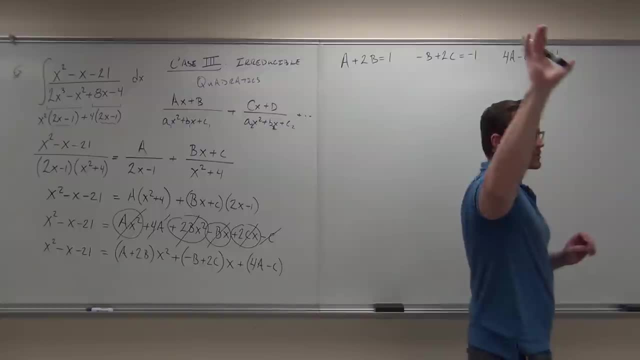 So this has gotta be negative 21. So I think you're okay with that one so far. 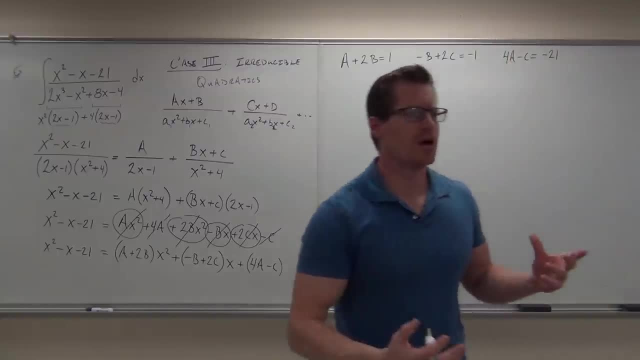 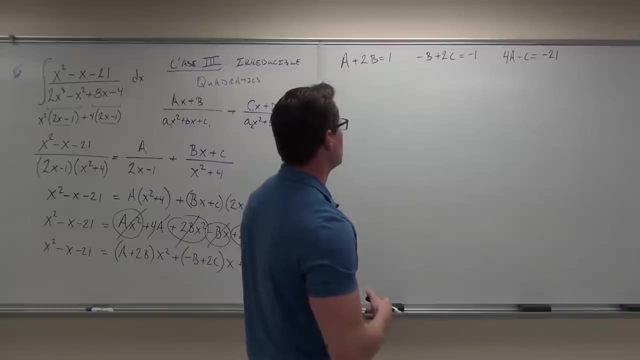 Okay, now, you can solve this in a variety of ways. The best way I think I've found to solve this, um, I would probably do a substitution. I'd probably set this one. 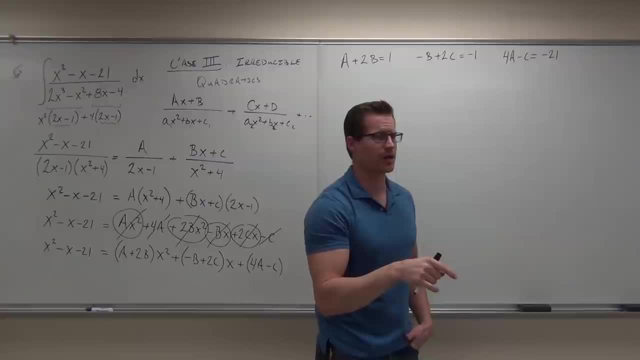 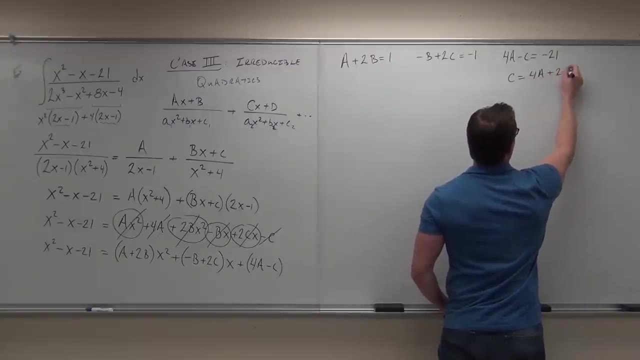 I'm gonna do a lot of math quickly in my head, because I don't want to spend a lot of time teaching you algebra, okay? So what I would do is I would add the c, subtract, add the 21, I would get c equals four a plus 21. Does that make sense? 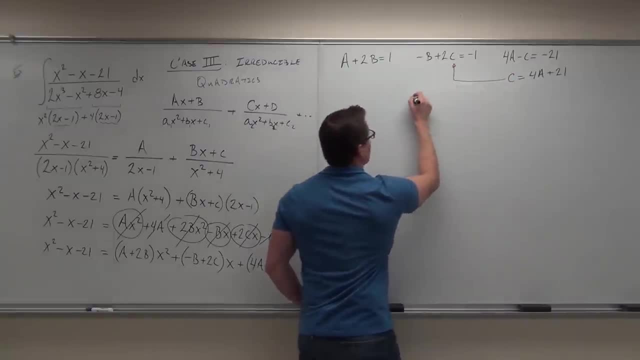 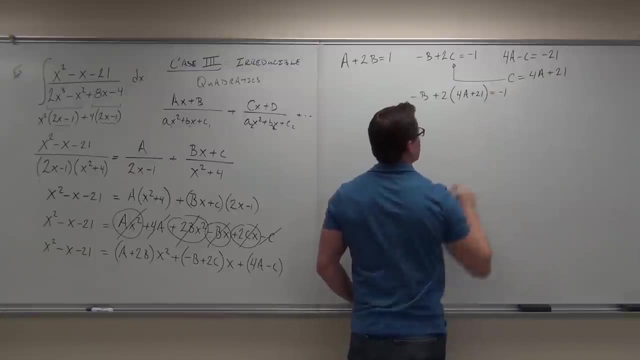 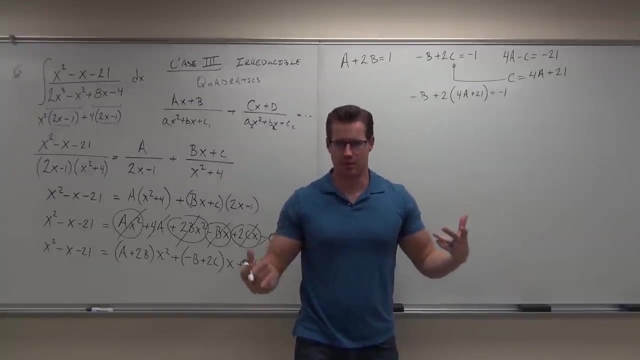 I would do a substitution here. I'd get negative b plus two times four a plus 21. That equals negative one. The idea being, I can get a's and b's, I can combine it with this a's and b's, and create a system of equations, and that will let me solve it algebraically. 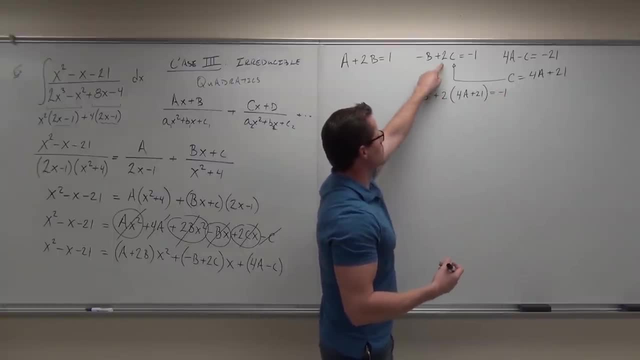 So do our substitution, no problem. We got negative b, cool. Two, no problem. Four a plus 21, that's our c, equals negative one. 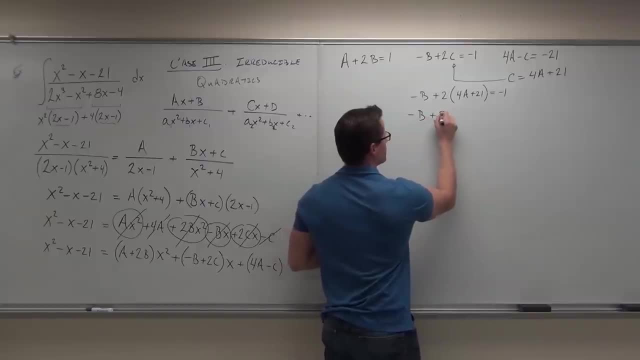 Let's do a little distribution. So negative b plus eight a plus 42 equals negative one. 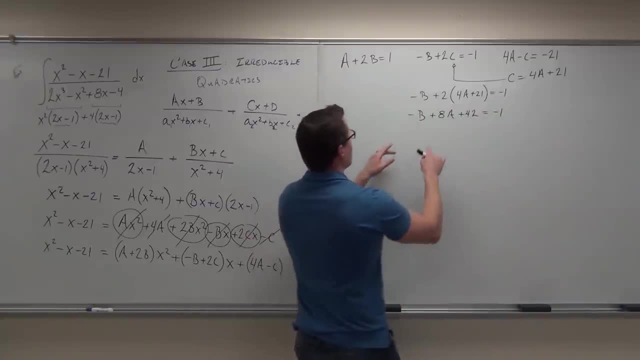 Are you still with me, folks? Okay, now, I'm gonna get my a's and b's on one side, I'm gonna get my constants on the other side, because that's how this one looks. 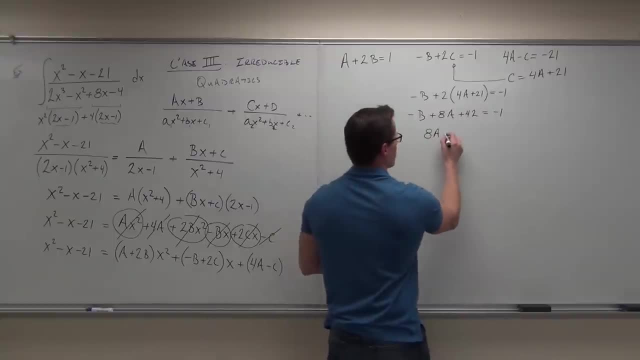 I'll probably write my eight a first, because that's how this one looks. My minus b equals negative 43. You still okay with that? Yeah. 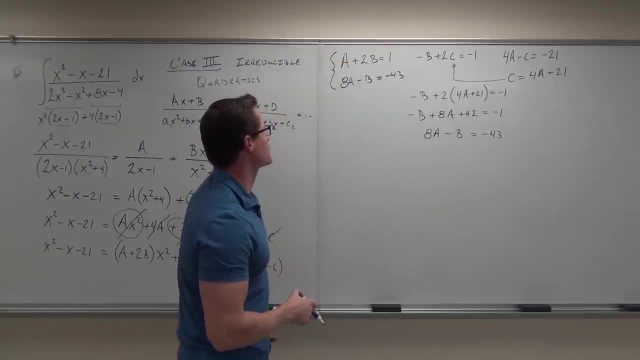 This is what we have now. A plus two b equals one, eight a minus b equals negative 43. You guys should know how to do systems of equations in one of two ways. 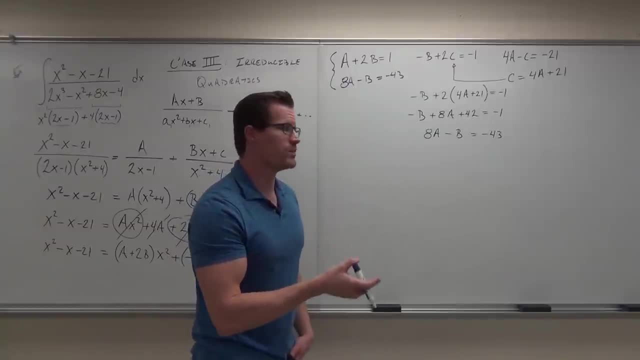 Either you do a substitution, which would work here just fine, or you do elimination, which is what I'm gonna do here, and that's gonna work just fine. 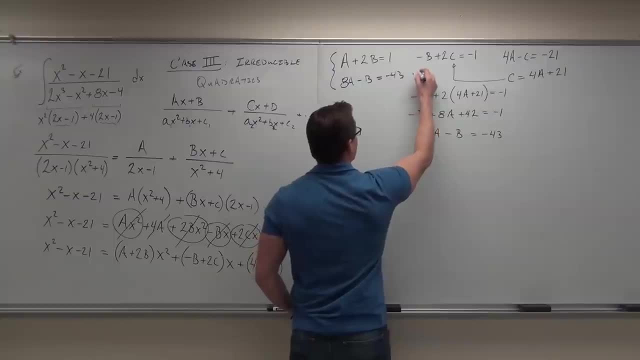 So if I did elimination, I'd multiply this by, I'd multiply it by two. 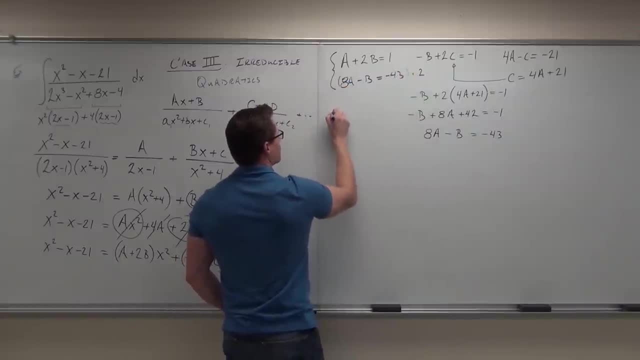 So if I multiply it by two, we get a plus two b equals one. 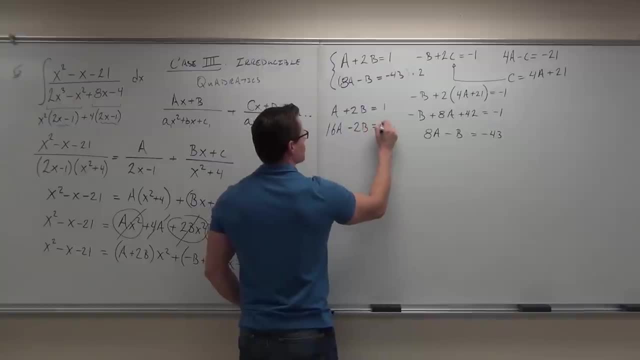 We get 16 a minus two b equals negative eight a plus two b, 86, if I've done that right. Have I done that right? Then what do we do? 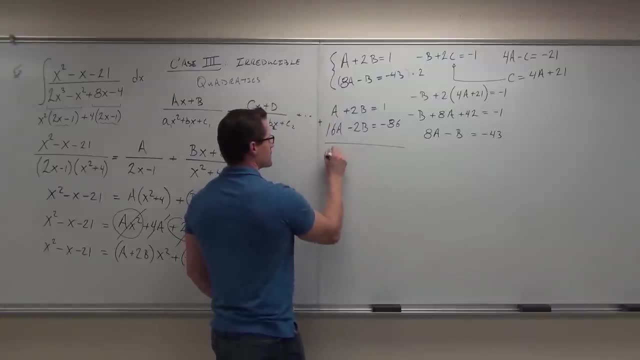 In this case, we add. We get 17 a, this is gone, equals negative 85. Man, this is kinda nice. Now, let's solve it. How much is a? Negative 85 over 17, what is it? Five. Five. Five. Negative five. I'm just tellin' what you give me. What is it? Negative five. Oh, okay. Does it matter? It doesn't matter, right? I mean, it matters. It matters. It doesn't matter. It doesn't matter. From here, can you solve the rest of them? Yes. Piece of cake. If a is negative five, then I'll proceed. Solve for all? Solve for all? Solve for b. Solve for whatever you want. You can solve for c by this one. By this one, actually, would be nice. You can solve for b by this one. That's what I would do first. 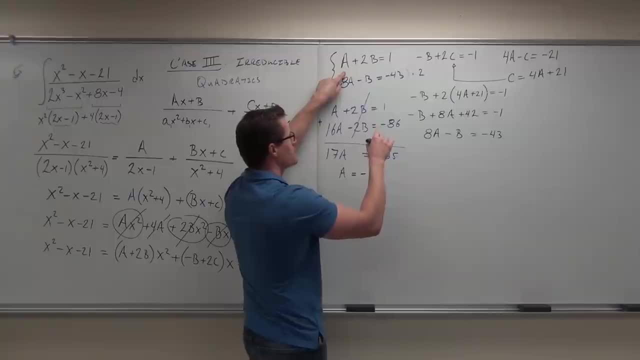 So, if I plug in negative five here, I'd be adding that and dividing by two. B is how much? Three. 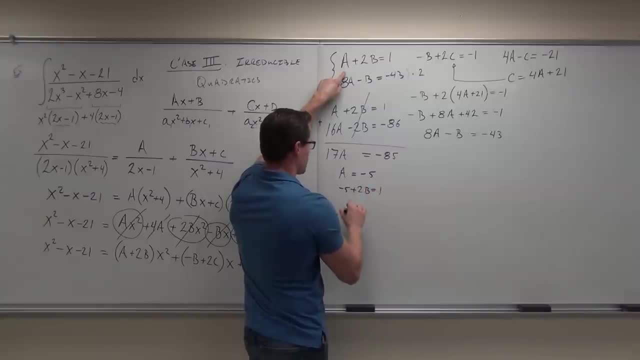 Sure, negative five plus two b equals one. Therefore, b equals three. 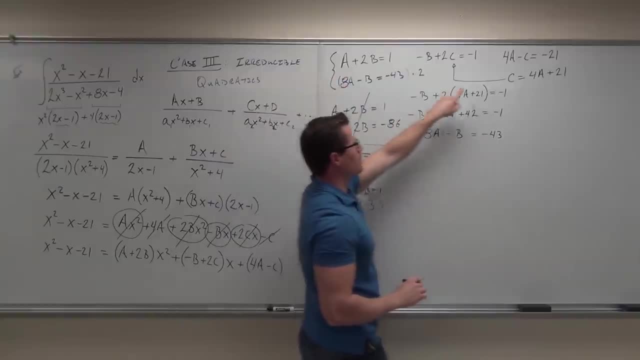 So, I get this one, and I get this one now. Workin' over here, I do this for our c. Okay. 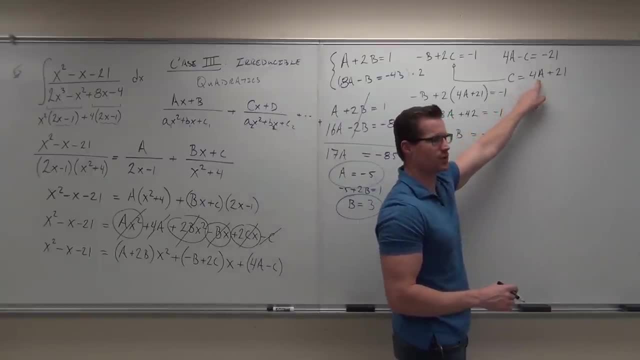 If I plug in negative five there, hey, look at that. Four times negative five is negative 20. Negative 20 plus 21 is? One. One. That was relatively painless. Not so bad, right? 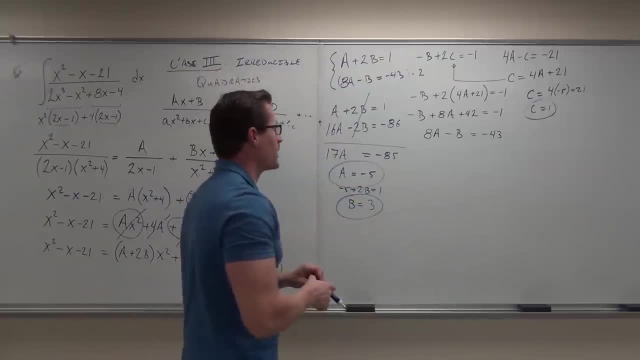 Not as easy as plugging numbers in, but not horribly bad. 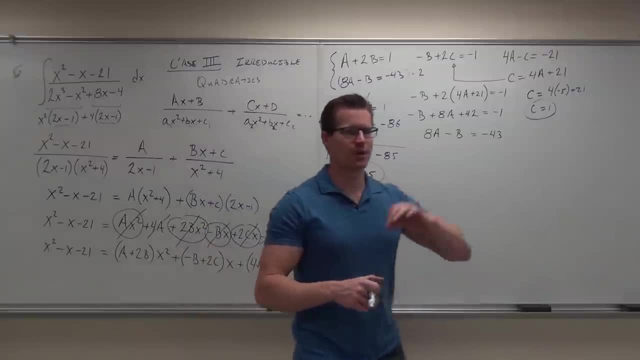 Hey, now that we have our coefficients, can we rewrite our integral? I know we've done a lot of algebra, okay, but I'm gonna come right back to here. So, our integral, we've done a lot of algebra. So, our integral, 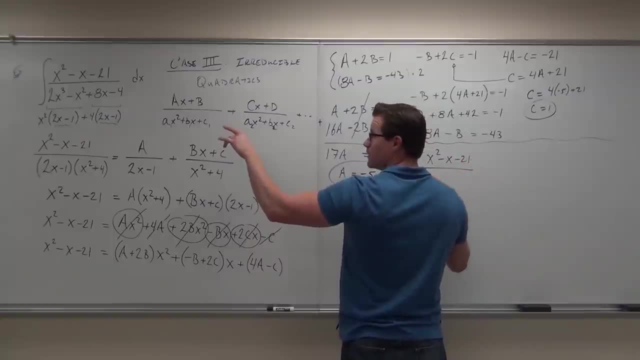 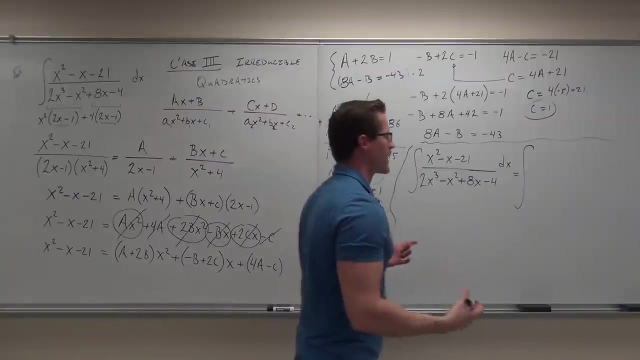 x squared minus x minus 21 over two x to the third minus x squared plus eight x minus four, dear goodness me, equals an integral of two fractions now. 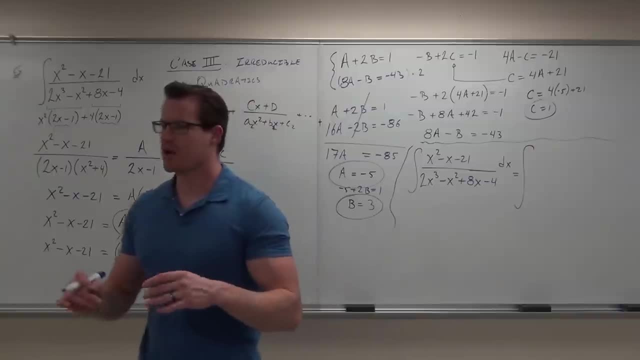 Notice we have three coefficients. We have three constants, but we don't have three fractions. We have two fractions. 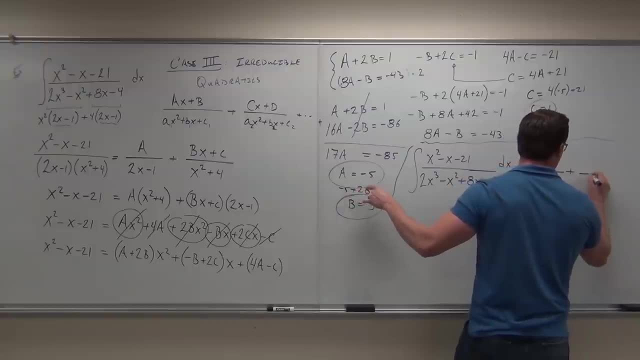 We have two fractions. The first fraction is over what, please? A. Now, the first fraction is over what? Two x to the third minus one. The second fraction is over? 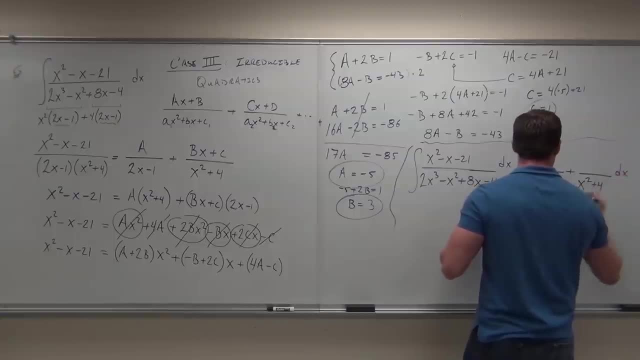 X squared plus x squared minus one. Dx. 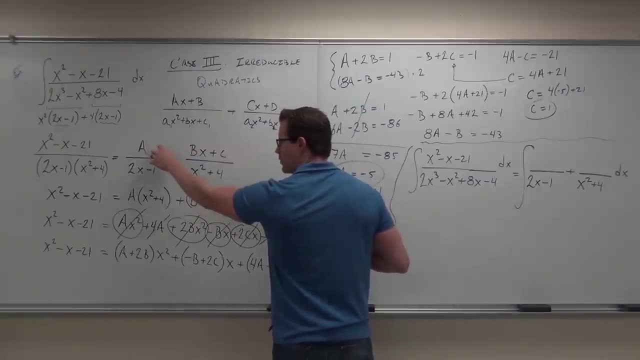 On the numerator of our first fraction, it says that we're supposed to have only an a. 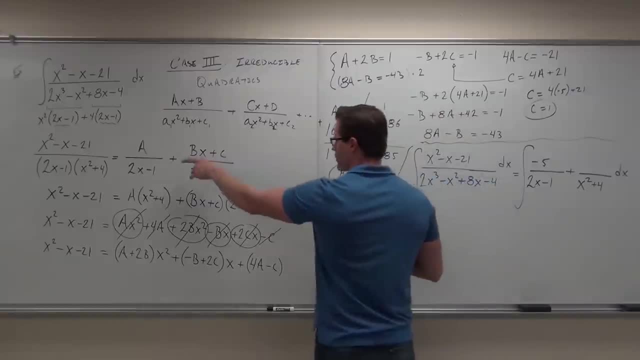 What goes here? Negative five. On the numerator of our second fraction, we're supposed to have a bx plus c. Bx plus c. Three x plus one. Three x plus one. Beautiful. We knew that this fraction could be broken up. 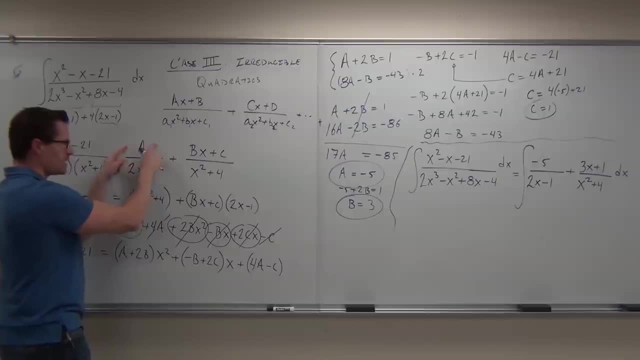 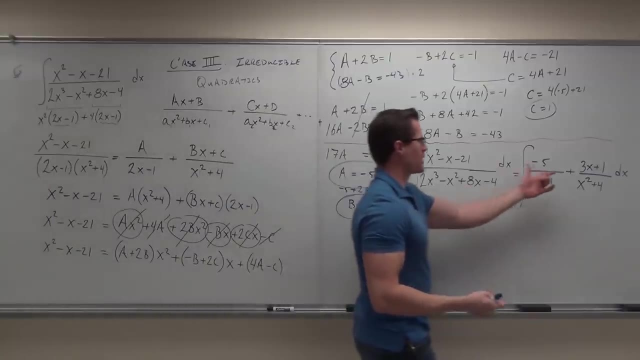 We just showed it. We know that a is negative five. A, negative five over two x minus one. We know that b is three. We just showed it. We know that c is one. Plug those numbers in. We get three x plus one over x squared plus four. It should eventually be okay with that one. 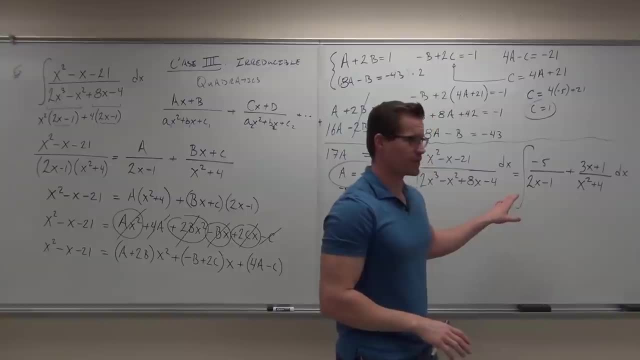 Now, I've gotta erase this stuff. Do you have any questions so far on this? Are you sure? Okay. Very straight forward. Very straight forward. This is gonna be an ln. Do you guys see it? Linear ln. 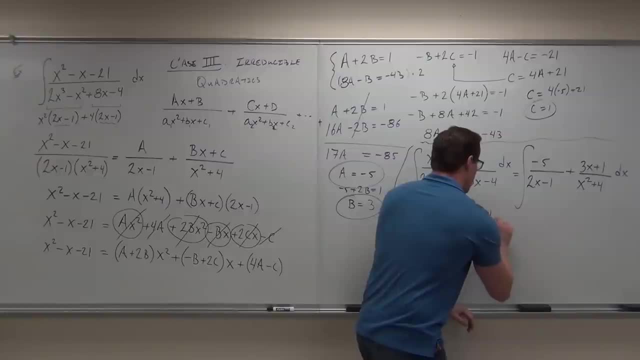 The only difference is this is not gonna be negative five ln absolute value of two x minus one. 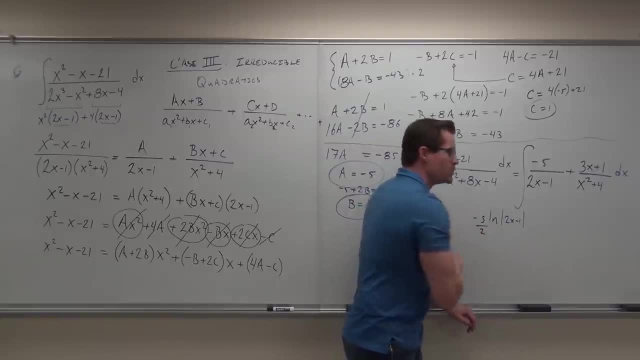 This is gonna be negative five ln absolute value of two x minus one over two. 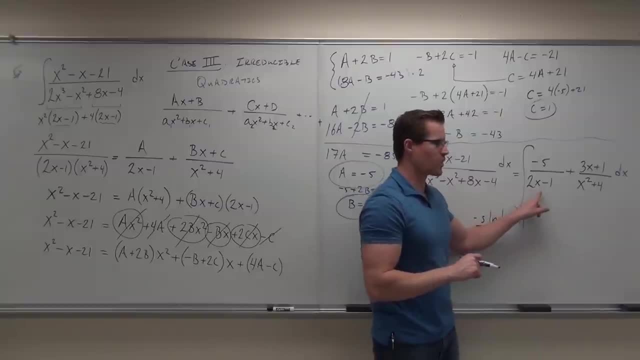 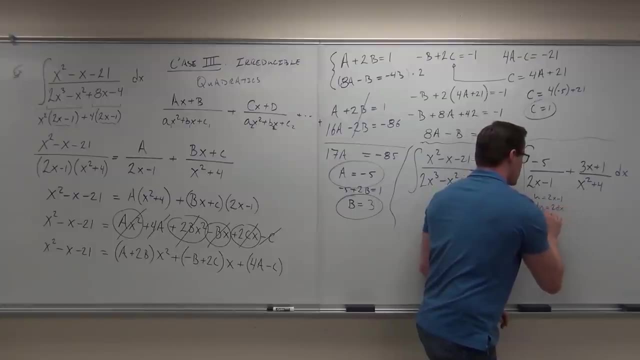 Do you see where the over two's gonna come from? It's a little u sub right here. If u equals two x minus one, du equals two dx. Or du over two equals dx. 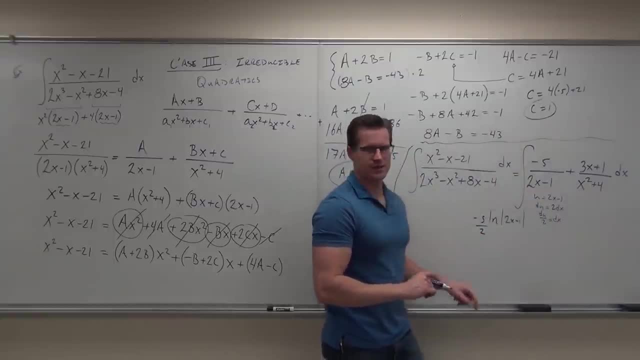 The over two. The over two is from right there. Does that make sense to you? 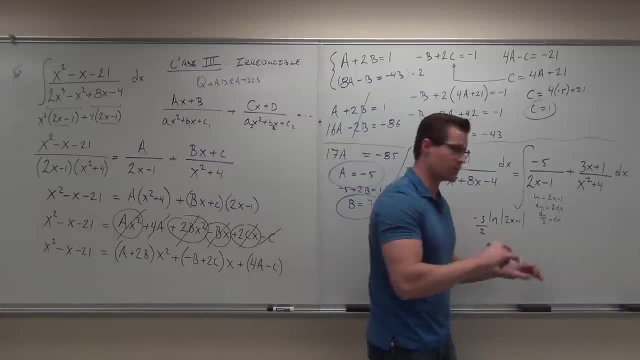 I do those in my head. If you need to show your work, you show your work. Don't get those wrong. Now, I'm gonna show that to you in a little bit. 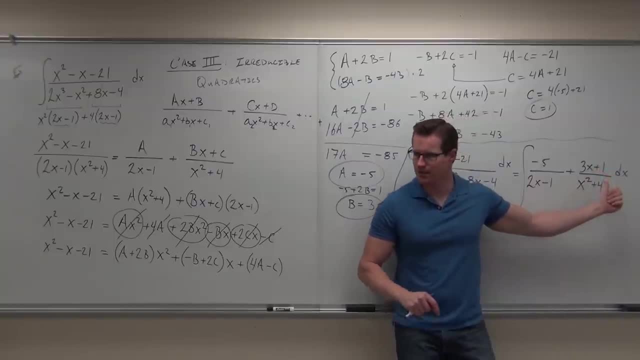 This one. Some of you guys are struggling with concepts like this. 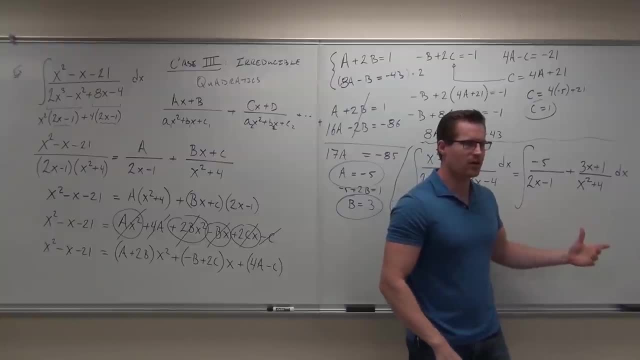 Man, how in the crap am I gonna do, what am I gonna do there? 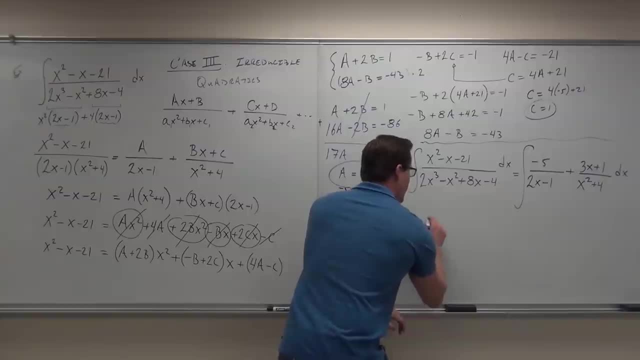 Think back to what fractions are made up of. Fractions 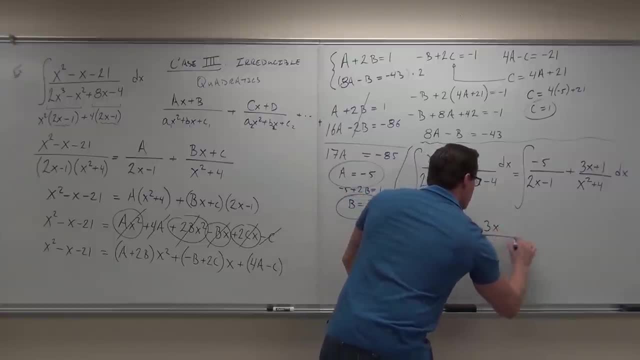 can always be split up. You split it up. Always. Now, let's think it through, okay? Think it through. 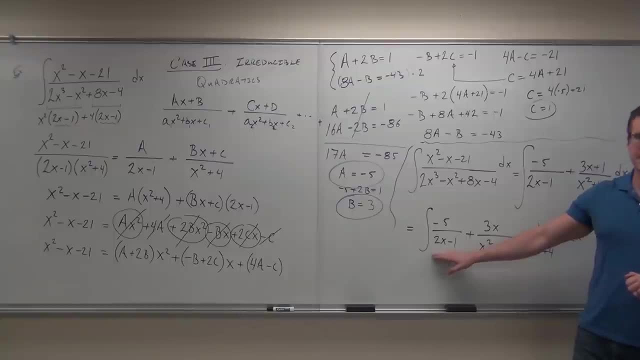 What would you do here? U sub, a u sub. Basic u sub. Or just do it in your head. 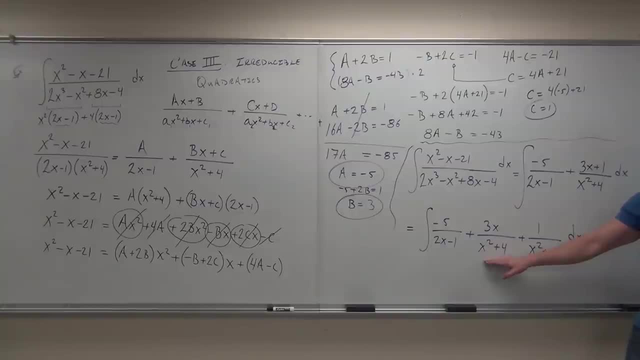 Look at this one. What would you do here? Write u sub. That's a u sub. 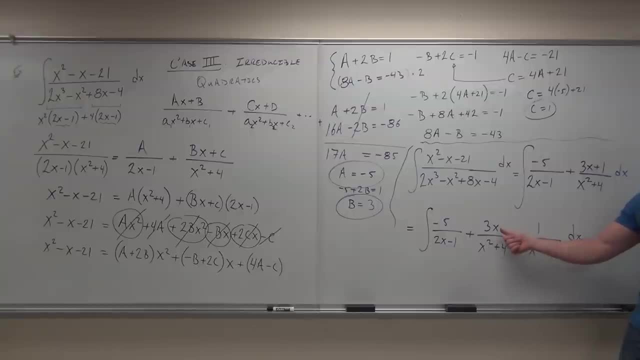 What's the derivative of an x squared? This is y. I don't care about the questions. 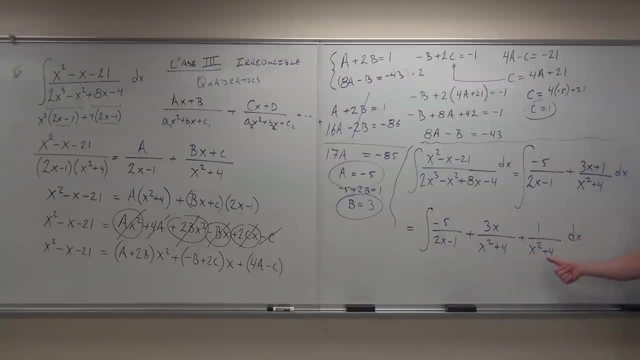 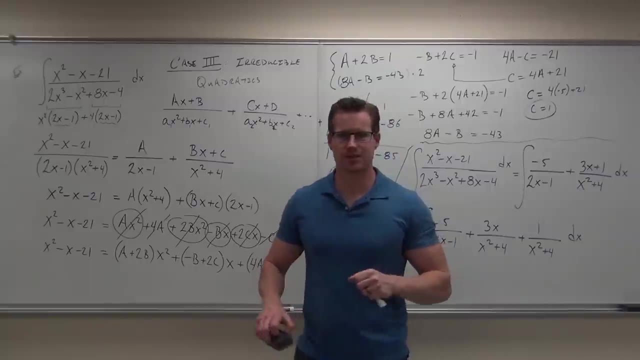 of the constant, it's going to be an x. Do you guys see what I'm talking about? How about that one? Let's think about that one. OK, we're going to do this over here. Do you guys want to finish this problem today? Yes. OK, it's going to take us about three minutes. Did you have questions on that? Too late. 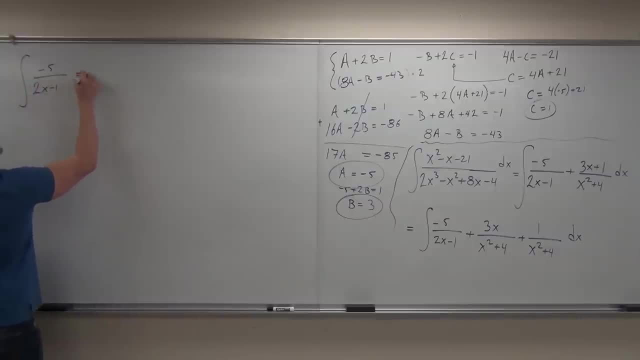 OK, let's just run down there. I'm going to split these up because we're going to, this is crazy, but we're going to use three. 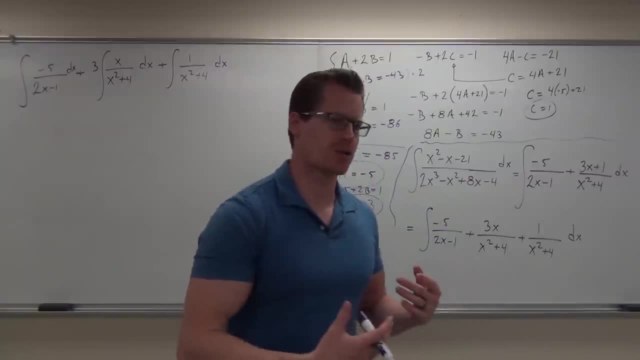 We're going to use three different techniques on each of these three integrals. So to show this accurately in mathematics, you don't want to just do this all as one, OK, because you have two different substitutions here. Are you following me? 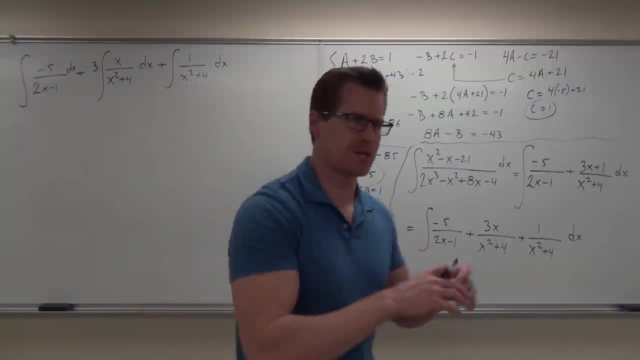 So you're going to, actually three, you're going to split this up into three different pieces. 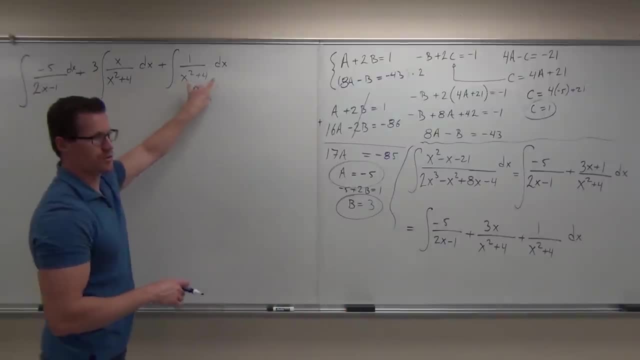 So integral of the first one plus integral of the second one plus integral of the third one. 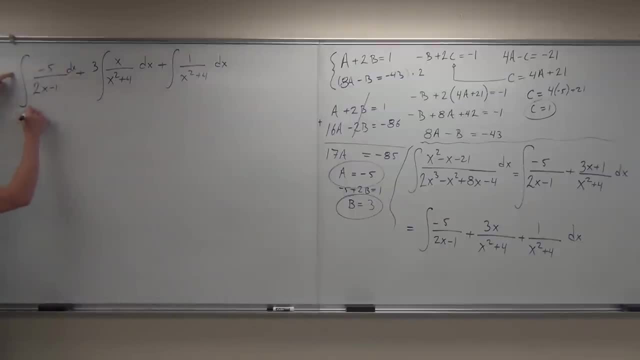 You could have pulled out the negative five as well. This integral is fairly straightforward. Our u equals 2x minus 1. Our du equals 2dx. Our du over 2dx. 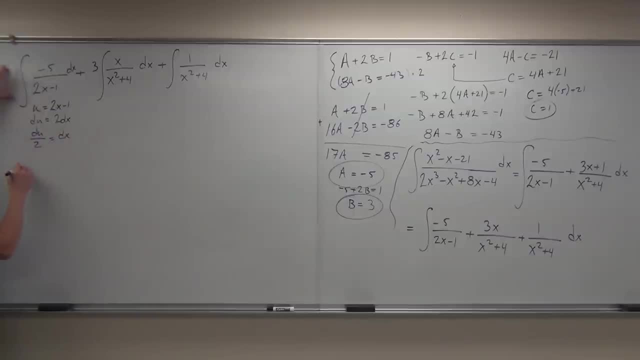 Therefore, when you do your integral, we get negative 5 halves, 5 halves, ln absolute value of 2x minus 1, and absolute value. 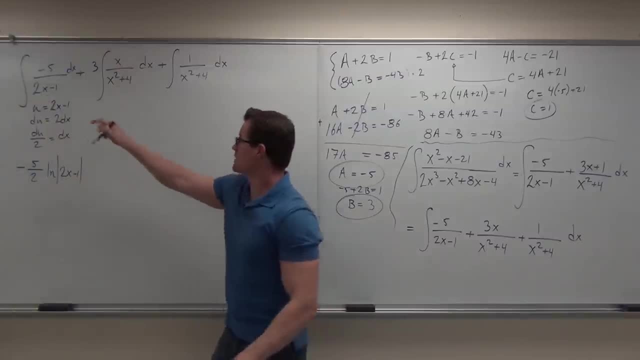 I need to show if I should be OK with that one. 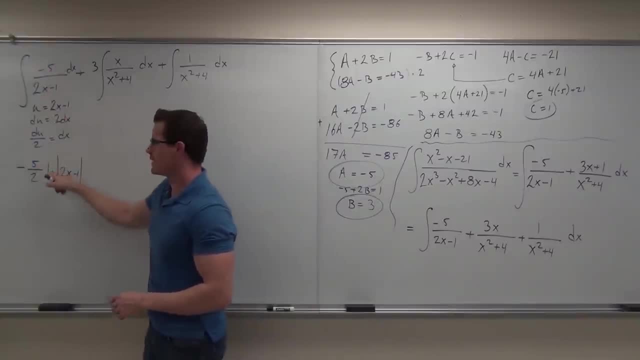 This would be negative 5 over u. That would be negative 5 ln absolute value u. You plug back in for your u, and the du over 2 gives us our 5 halves. So negative 5 halves over u. You plug back in for your u. And the du over 2 gives us our 5 halves. So negative 5 halves over u. W, ln, u. 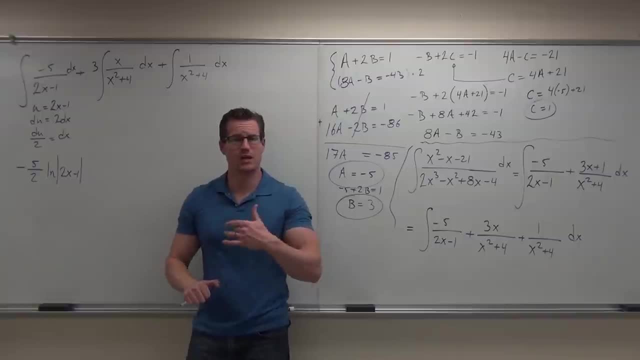 OK with that one? No, we're going quick, but if you need a refresher on that, 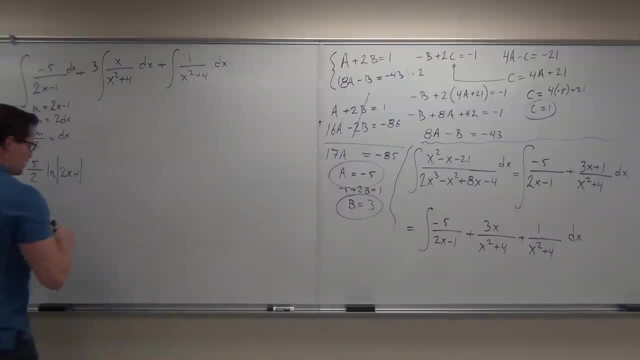 go back and look at that section online or on the video. The line. OK, next one. 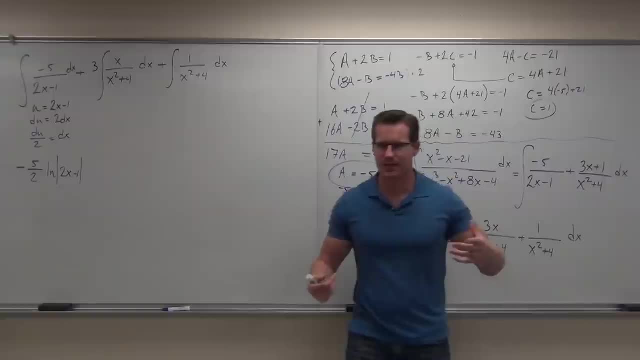 Don't let these things escape you like this. If you're stuck, you go, man, I can't do that one, try splitting it up. Then it makes a really easy integral doable for you. 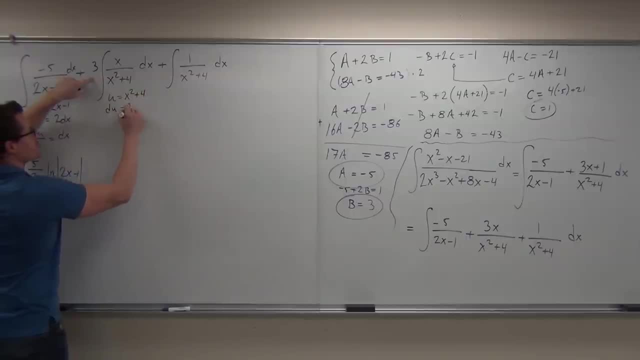 That makes it easier. Do a basic u sub. All right ? That was easy. How can I limit that? 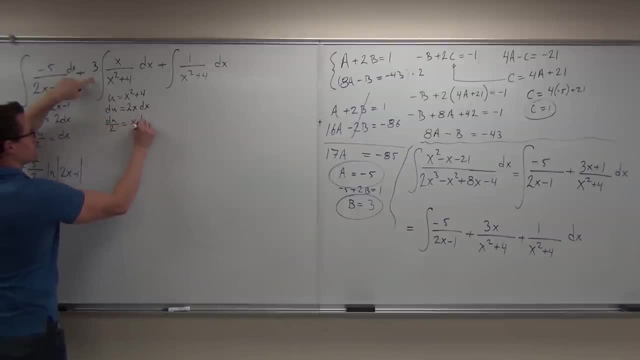 Here, u equals x squared plus 4, du equals 2dx, du over 2 equals xdx. There it is, right there. 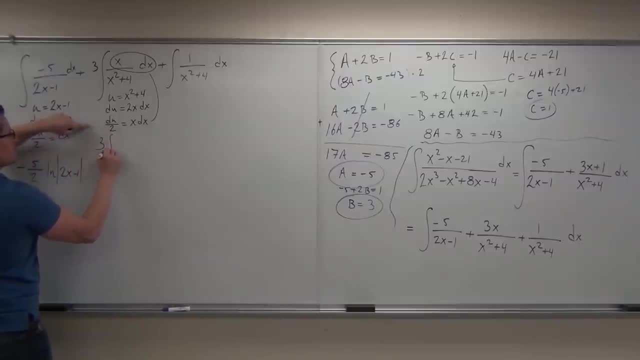 That means that we have 3 integral 1 over u du over 2. Are we okay with that one? 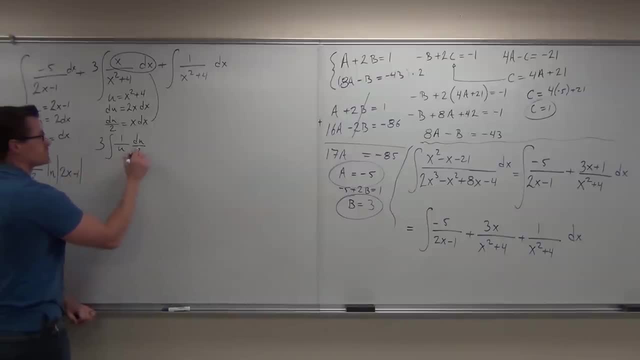 Okay, well that means that we're going to have 3 halves ln absolute value u. 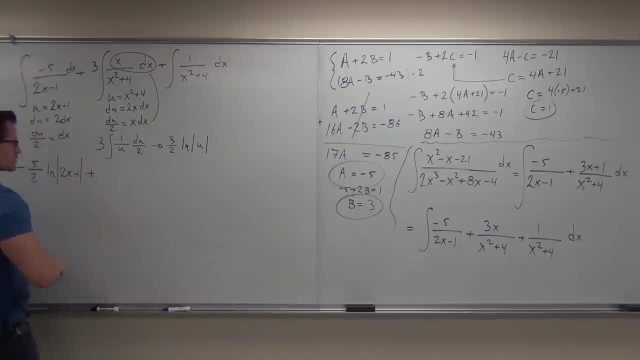 So this will be plus, I'm going to use purple here to show that, same thing, plus 3 halves ln absolute value of what goes in there? And that's the value. I want to make sure you guys are golden on this stuff. You guys okay with the first one? Negative 5, got a little substitution. That's where the over 2 comes from. 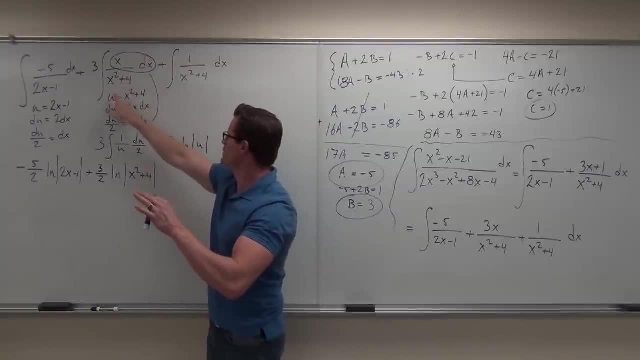 Here, basic substitution, all basic. du equals 2dx, du over 2 equals xdx, this is du over 2. Therefore, we're going to have a 3 halves. That's the over 2. 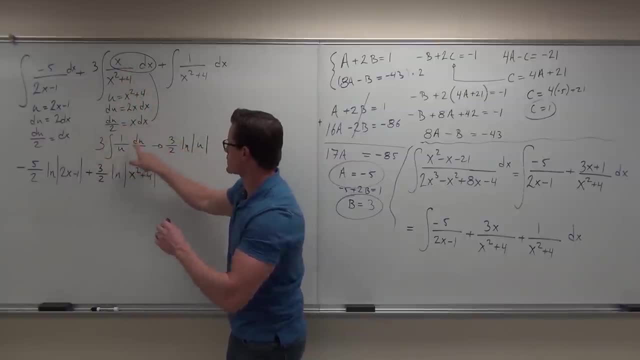 We're going to have integral of 1 over u. So we're having 3 halves, ln absolute value u, plug in back for the u. 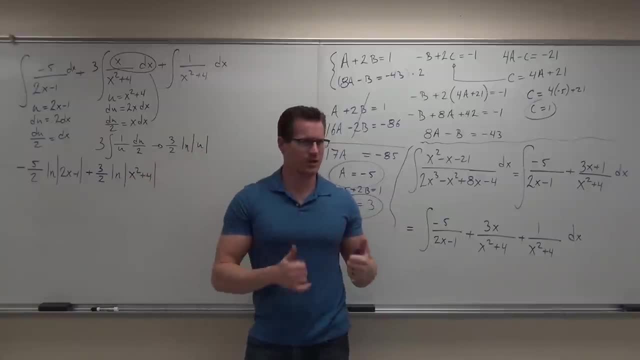 u is x squared plus 4, we got our integral. Am I explaining this well enough for you guys? 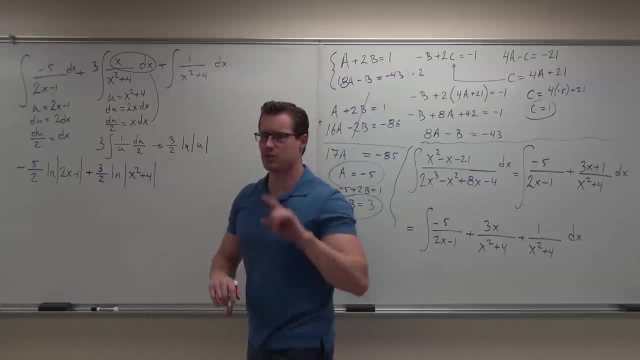 Okay, next up, you can actually do this two ways. I'm going to show you a very cool idea here that you're going to be using. 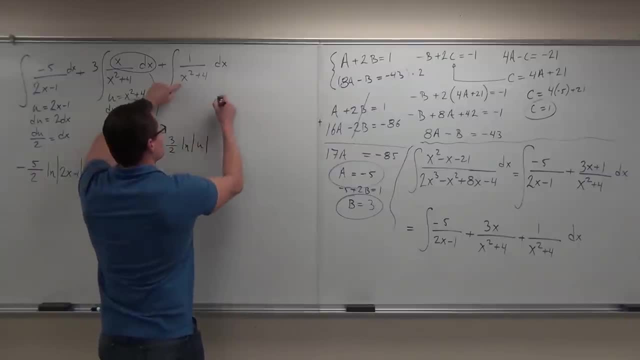 One idea is you understand that I could make this 1 over, I could force this to factor as x over 2 squared plus 1 times 4. 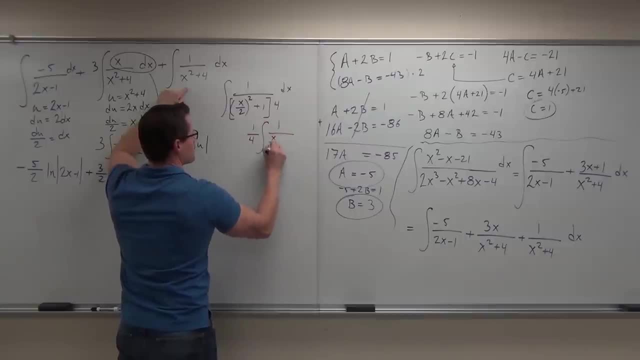 That would be one-fourth of the integral of 1 over x over 2 squared plus 1. 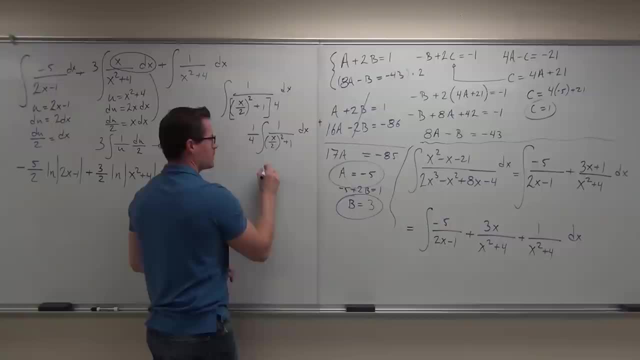 And then you realize that's tan inverse. And you go, oh, look at that. That's tan inverse x over 2, 1 half, because you have a little u-sub there. You can do it that way. If you didn't catch that, don't worry about it so much. I'll show you a different way. Hope that's right. We'll see. My constant might be up there and you'll know fast. 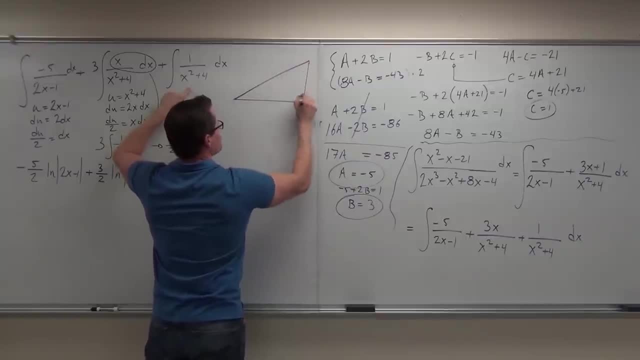 This almost, almost looks like a trig sub. Do you see it? Yeah. What's missing? Square root. Ignore it. Ignore the missing square root. 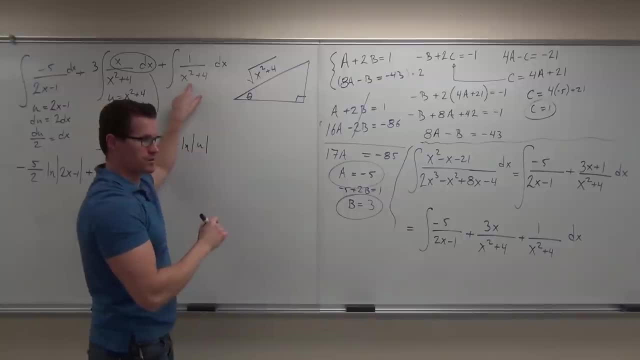 If you were to write it as a square root, that would be the hypotenuse. Missing the square root. Do you get that? You can still do. That's a sine. No, that's a secant. That's a tangent. 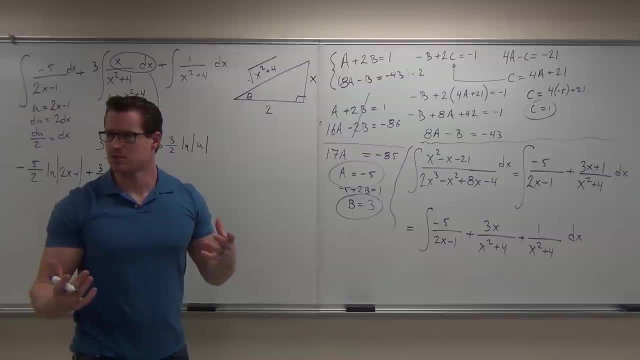 You can still do the two missing sides. Do you follow that? If you do the two missing sides. 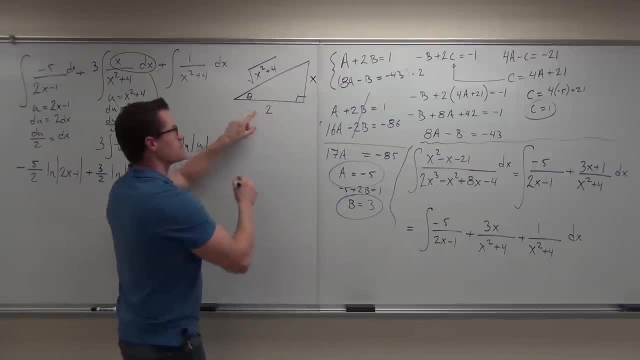 This would give you the x. This would give you the two. You can still do the substitution. 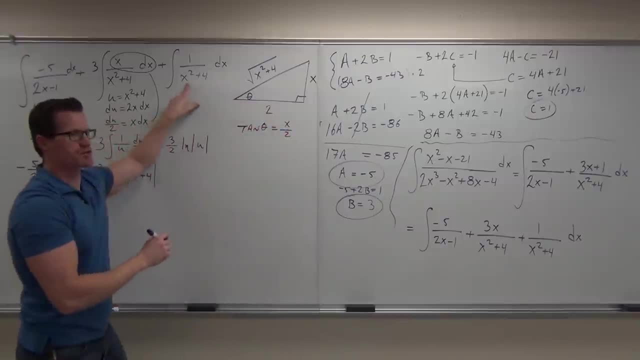 Tan theta equals x over 2. So who cares if it doesn't have a square root? You can still do this. No problem. This is x. This is 2. 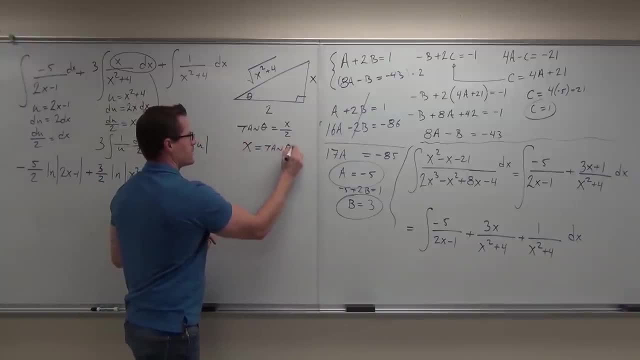 Then x equals tan theta times 2. dx would equal 2 secant squared theta d theta. 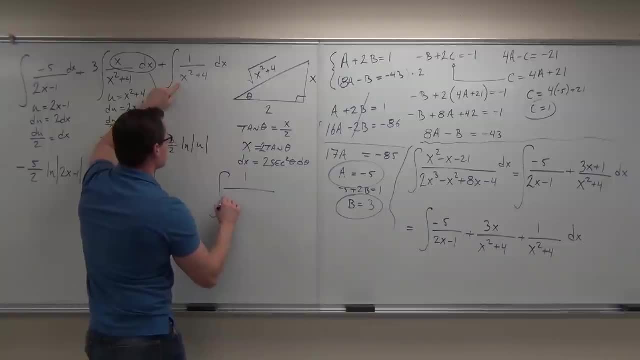 Our integral would equal. 1 over 2 tan theta squared plus 4. 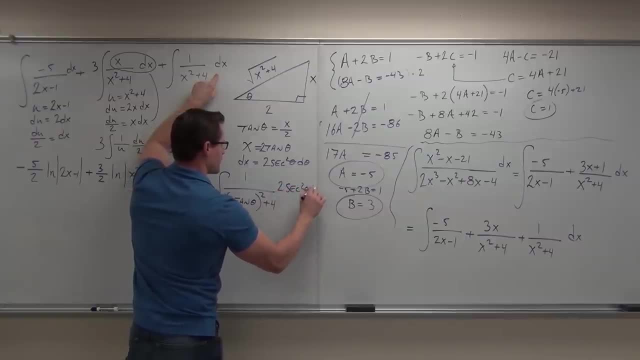 Our dx would equal 2 secant squared theta d theta. 2 secant squared theta d theta. I know I just went really fast on this. Are you following that one? You sure? 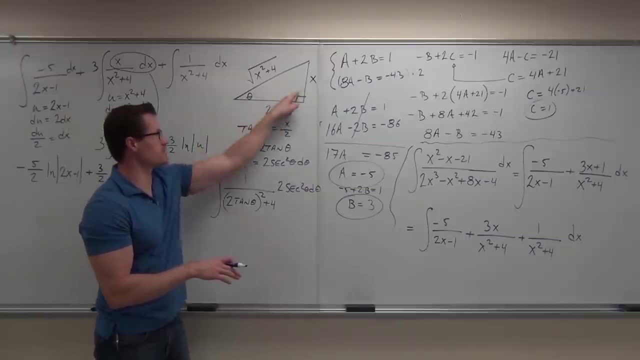 The triangle is the hardest part, right? Then we do, hey, tan theta x over 2. No problem. 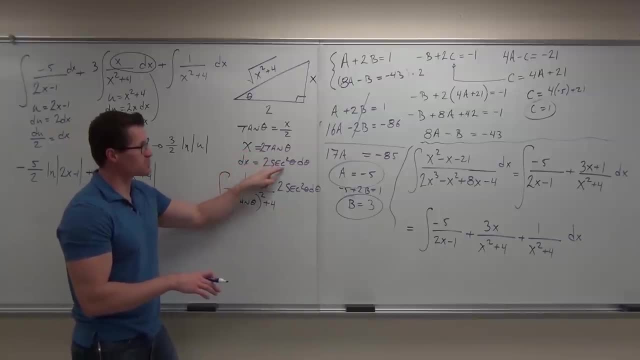 dx equals 2 tan theta. dx equals 2 secant squared theta d theta. Make our substitution. 1 over 2 tan theta squared plus 4. 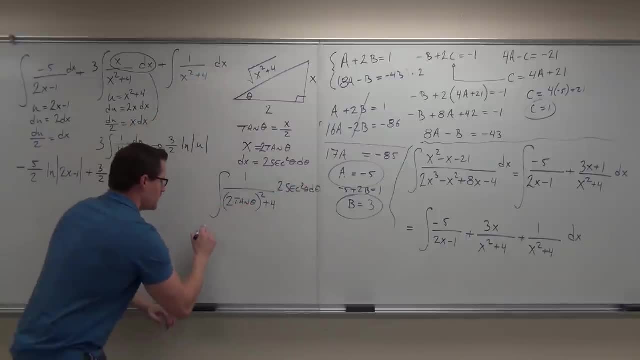 dx is 2 secant squared theta d theta. That means that our integral becomes 4 tan squared theta plus 4. 2 secant squared theta d theta. 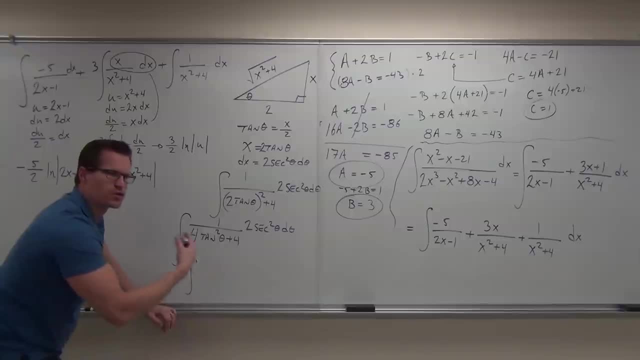 Factor the 4 out. If I factor the 4, notice, it's even easier. There's no square root here. If we factor the 4, we get 2 secant squared theta d theta 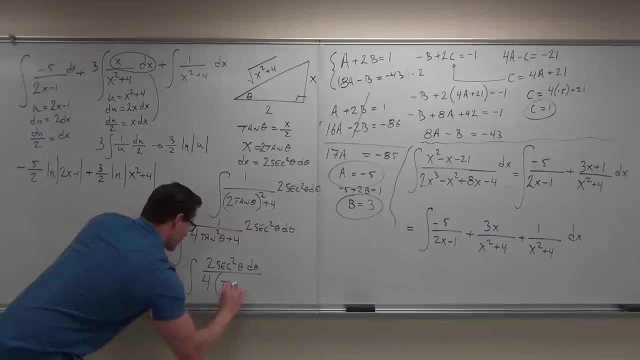 over 4 tan squared theta plus 1. Do we follow that? Yeah. 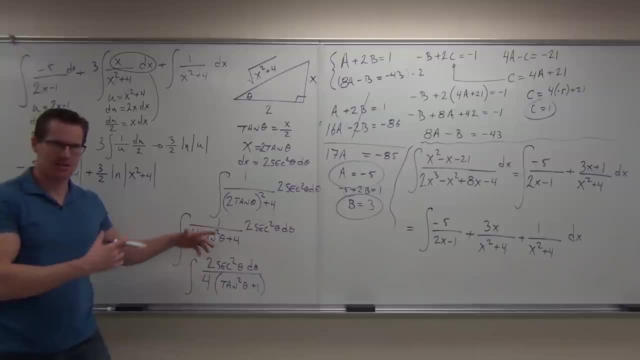 Hey, look at that. Do you see the 1 half? Told you it was a 1 half. That's because of those constants. Hey, 1 half. Integral. Hey, how much is this? 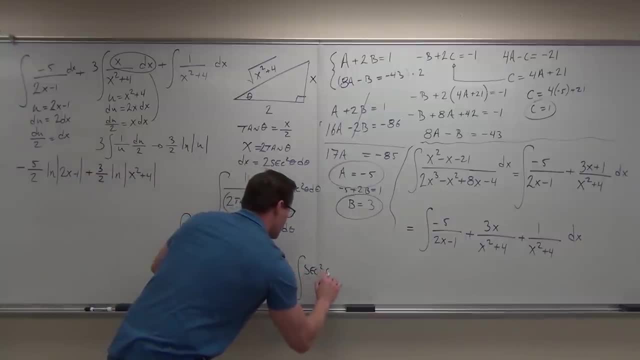 Secant squared theta. So we're going to have secant squared theta over secant squared theta. d theta. That's equal to 1 half integral. Oh, my gosh. This is secant squared theta, right? Uh-huh. This is secant squared theta, right? Uh-huh. This is 1 half. 1 half. 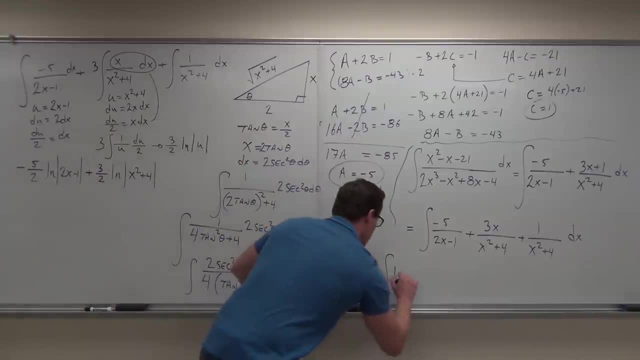 Secant squared theta. Secant squared theta of what? 1 d theta. Can you integrate 1? We can. 1 theta. 1 theta. 1 theta. I don't even want to plug the data. So . So this is 1 half theta. Oh, goodness gracious. 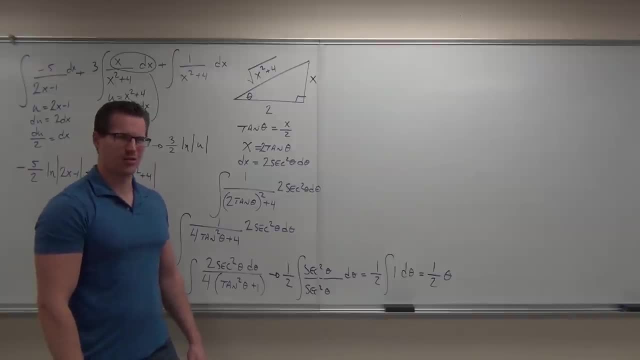 Here's the whole banana. Is that even a term? Is that a thing? We just made it a thing. It's a thing. Whatever. 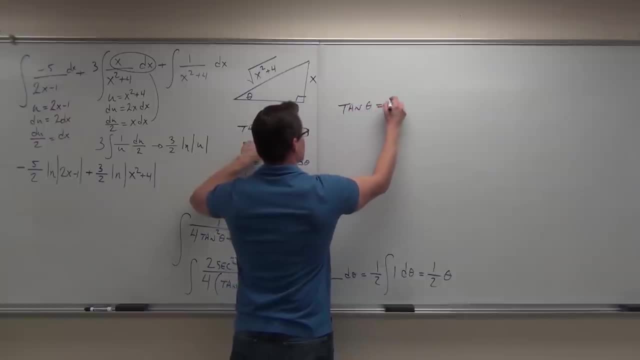 If tan theta. Theta. Equals. X over 2, this is if and only if theta equals tan. 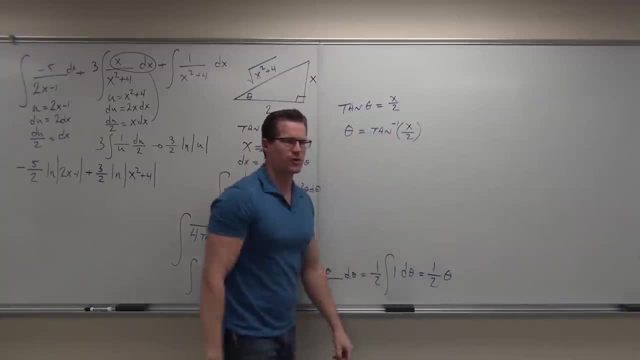 Oh my goodness. This is where all your inverse integrals came from. Booyah. 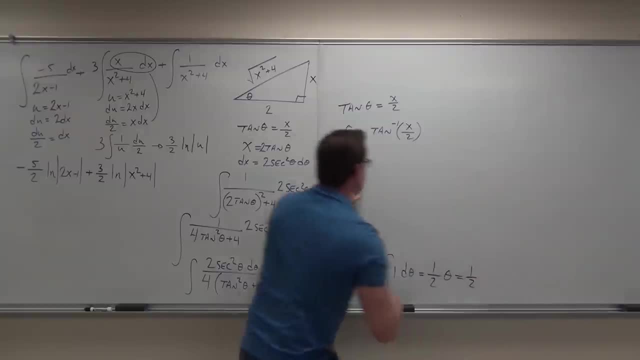 Then this is the same thing as 1 half. Tan theta equals X over 2, correct? Theta equals tan inverse of X over 2. 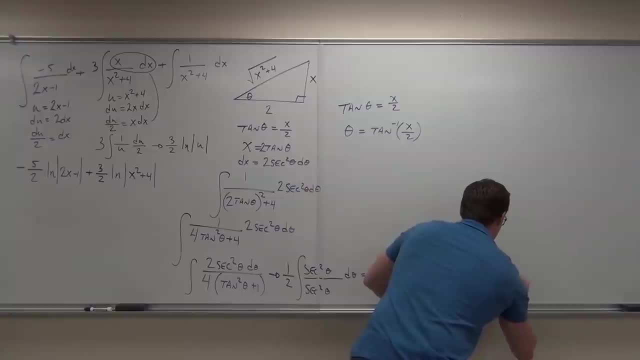 So 1 half tan inverse X over 2. I believe I had that on the board just a little while ago. 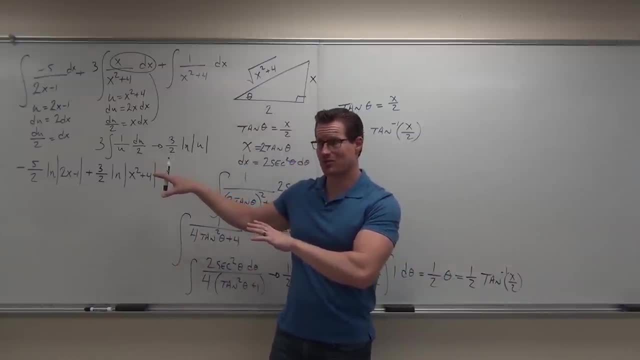 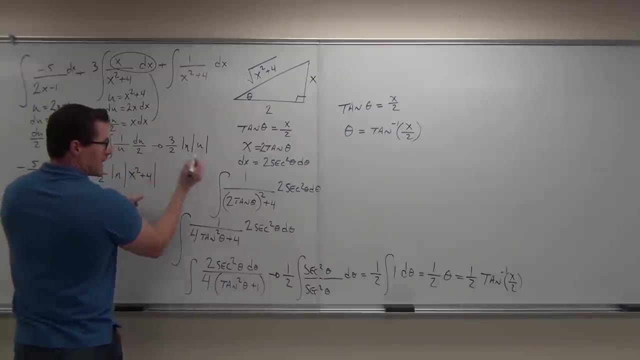 So if you know how to factor that, you could do it with just your inverse trig function as far as your integrals go. So one last little piece. We're gonna add this up here. Don't forget this is our first part. We have plus 1 half tan inverse X over 2 plus C cubed. 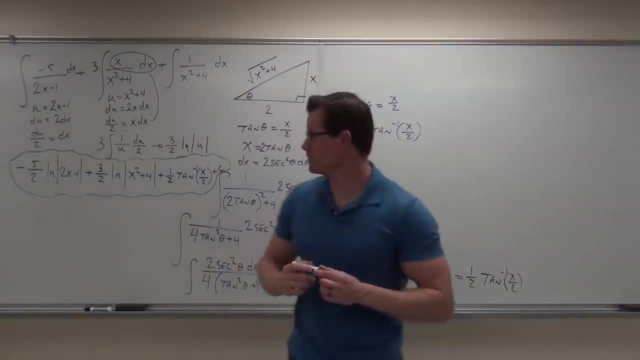 Now my question is, did you understand it? Yes, somewhat. 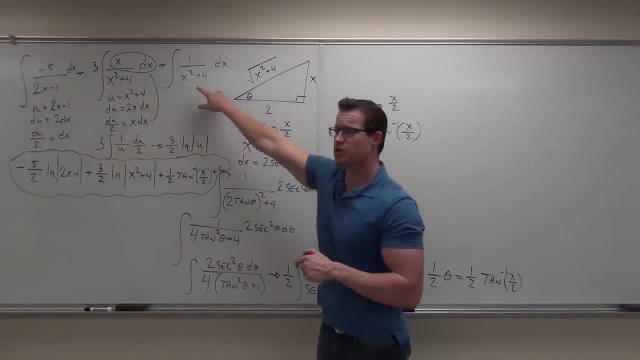 So this one LN, this one's substitution in LN. This one you can do it two ways. You can draw the triangle. This still works. Don't even have to worry about the square root, okay? Just make the triangle accordingly. Or you could have made this factor out the 4. 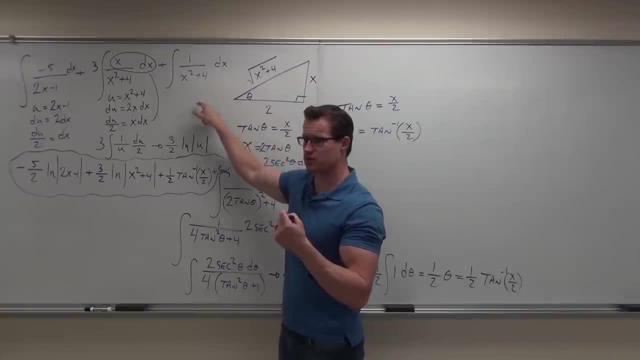 Make it factor the 4. You'd get X over 2 squared plus 1, and then a 1 fourth outside. Do a little substitution for X over 2, and you have an inverse tangent. And that's the idea. So I guess we're okay with this one. All right. 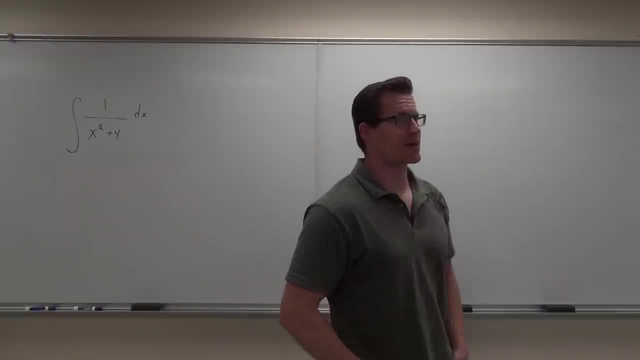 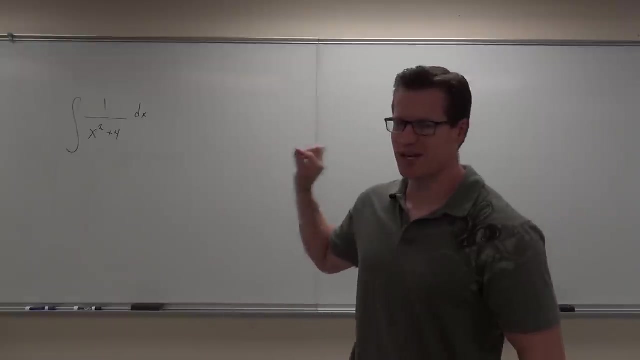 Okay, so before we get on to our last, thankfully our last example of partial fractions, I covered an example that had this little piece in it. 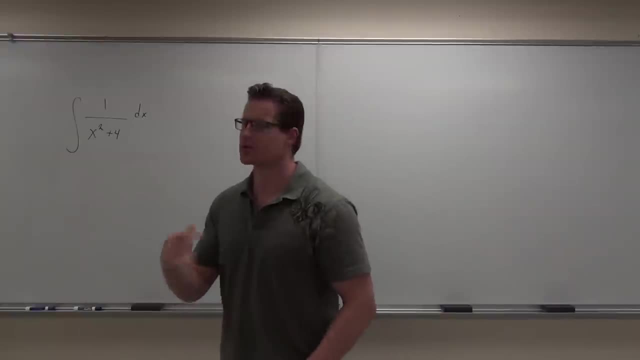 And I want to go over this a little bit more slowly on how you, there's two ways to actually do this, how you can go about doing this problem in one of two different ways. 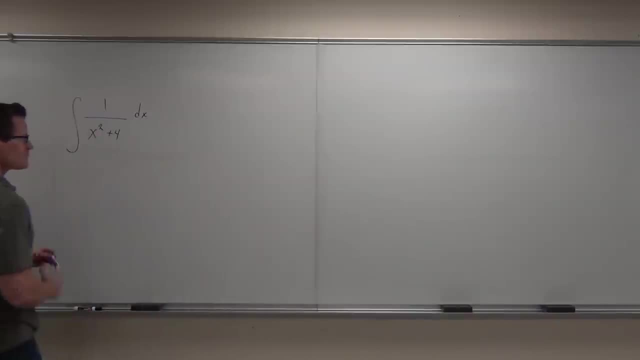 Now the first way. The first way is an idea that we get from trigonometric substitution. It's, well, you know what? That looks almost like a triangle, almost like one hypotenuse of a right triangle. 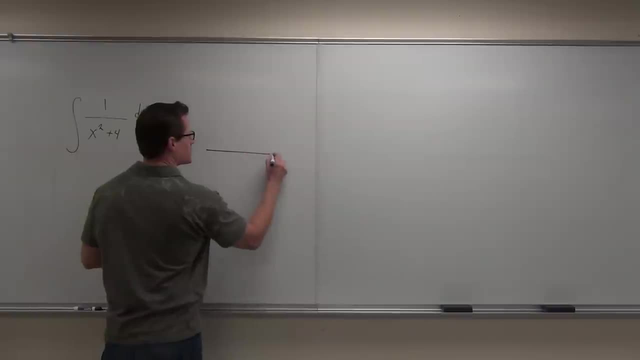 You can actually do that. So you could make a right triangle out of this. 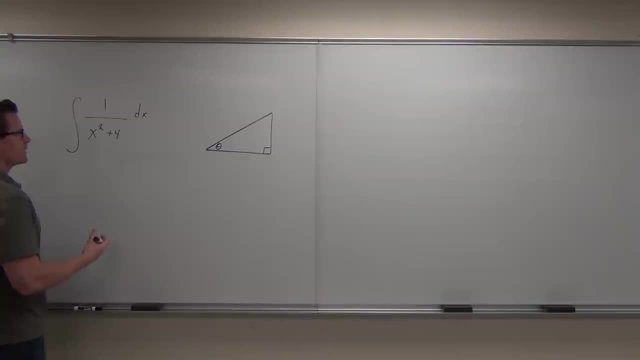 And the way you can think about it is, well, if this were to have a square root around it like that, this would be the hypotenuse. Does that make sense to you? So it would be like this. 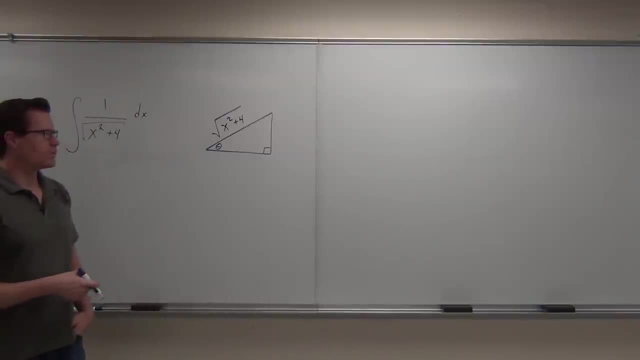 If that were the hypotenuse, well, the other two dimensions here are the sides, are the legs. 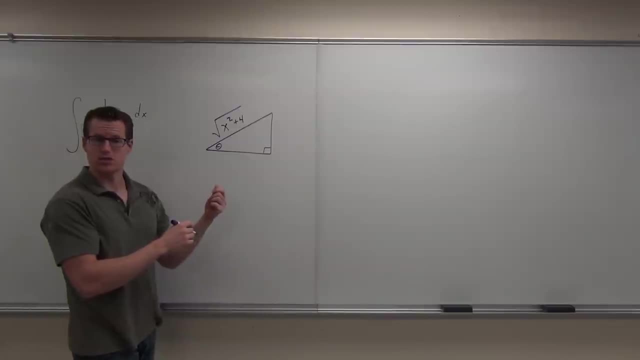 Well, we would have x and what? Two. X and two. Where would the x go? 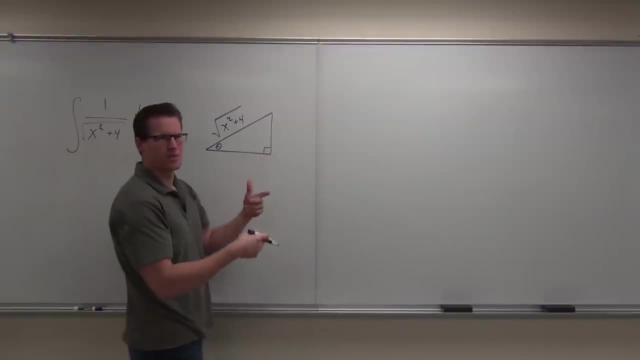 This one. Yeah, because what we'd want to do here is make up our tangent relationship. So we'd have x, we'd have two, and we'd have tan theta equals x over two, or x equals 2 tan theta. 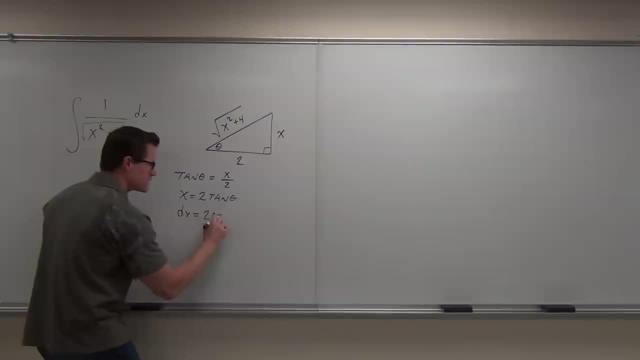 And then, of course, we take our derivative. We have dx equals 2 secant squared theta d theta. You guys OK with that so far? Mm-hmm. 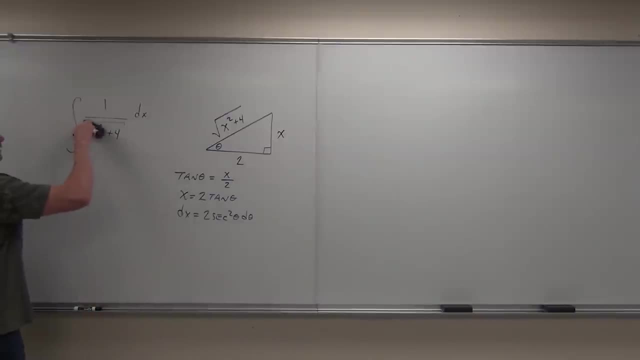 If you really think about it, you can do this lots of times. Let's consider this one more time. If you had just 1 over x squared plus 4, someone made a comment earlier, well, maybe we can manipulate this a little bit so it's easier to see. 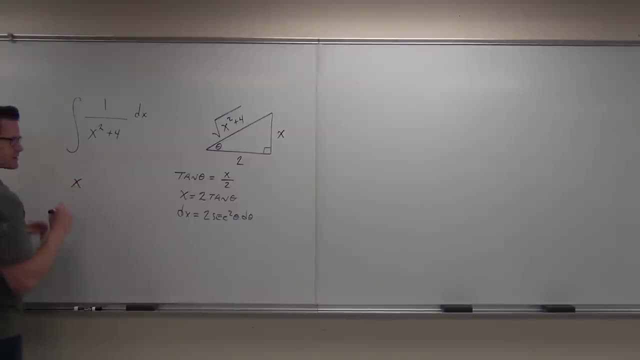 Check it out. If I have x. Do you understand that it's almost the same thing? 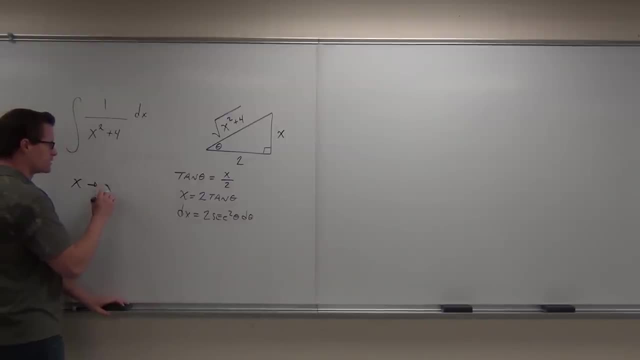 It's not the same thing. It's almost the same thing as the square root of x squared. This is almost true, but it's not true because we'd square it so our negative x's don't really work that way. It's really the, it's really an absolute value type of idea, but we can use it for here, especially since we have both positive. 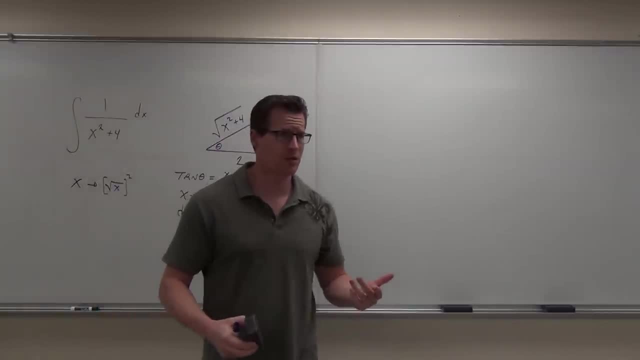 We don't have to worry about that. We can get a negative out of this anyway, so it's going to be positive no matter what. 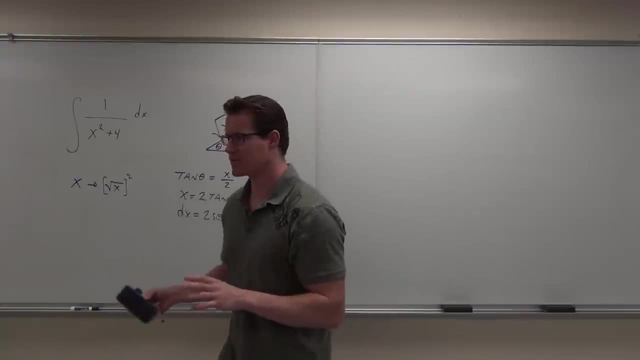 Does that make sense to you? So whether x is positive or negative, we get a positive out of it. 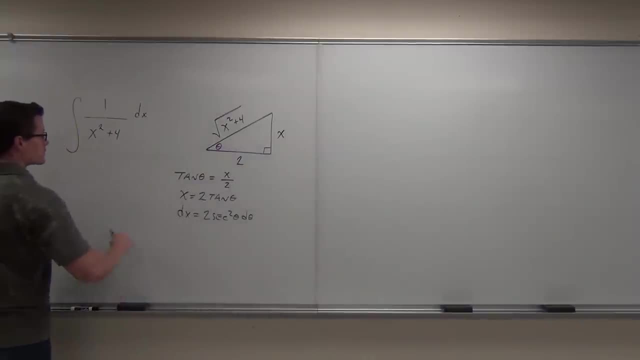 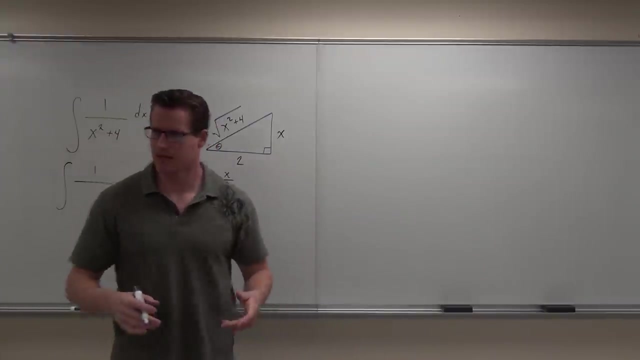 We don't have to worry about that scenario. So in our case, we'd say, all right, well, if you want to make this a little bit more understandable about why this can fit a right triangle, here it is. 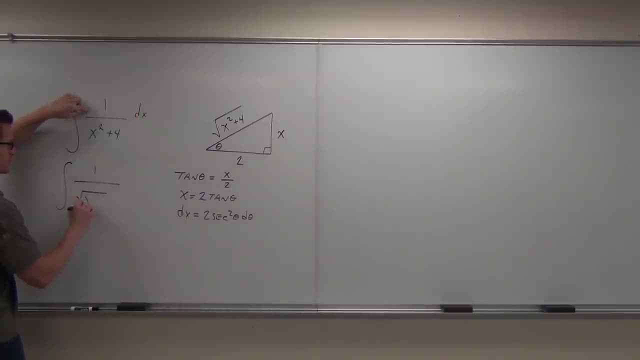 Why this can fit a right triangle is that we can make this the square root of x squared plus 4 squared. Now, for those of you who didn't say it before, you guys see what I'm talking about? 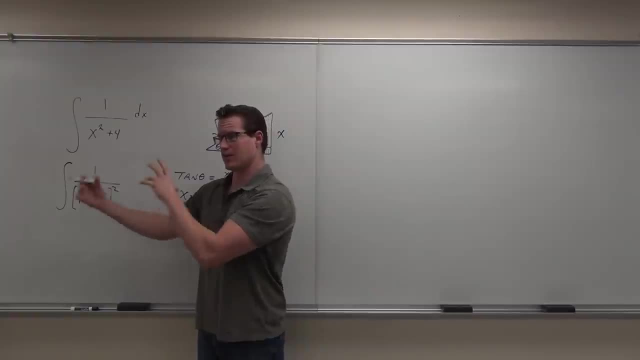 That is, I mean, that, now that, that is a hypotenuse right there. It's just now we have a square. Does, you follow me? You can do that, no problem. 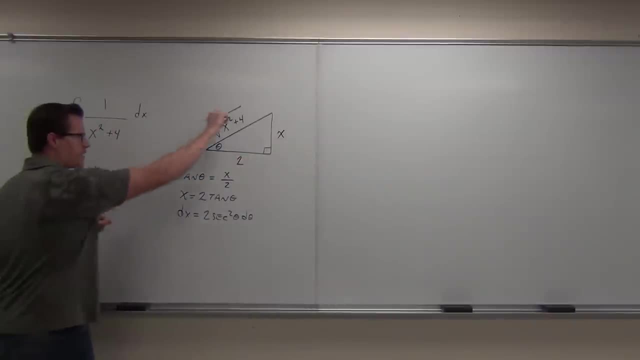 We have our x, we'd have our 2, we'd have, hey, that's my hypotenuse. 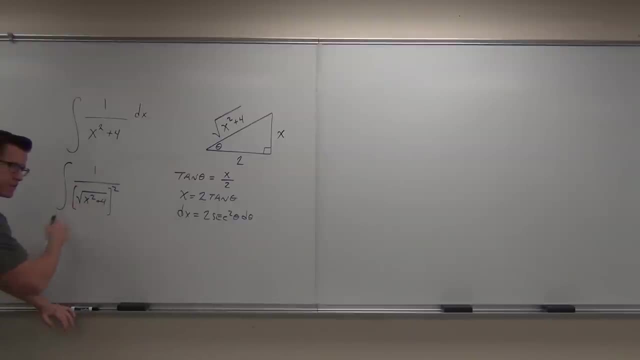 Now, either way you go about doing this, you're going to get the same thing because when we plug this in, when we do our actual substitution, well, we've got 1, I'll leave it this way just so you see what I'm talking about. We'd have 1, we'd have something being squared. You with me? Inside here, we'd have a square root. We would have 2 tan theta squared plus 4, and then we'd have our dx becomes 2 secant squared theta d theta. You guys get me so far? Now, look what happens with a square root and a square. 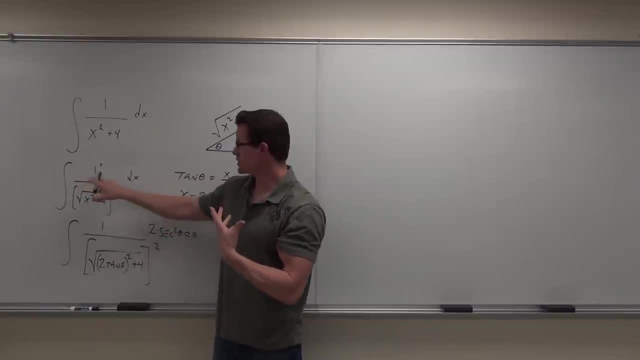 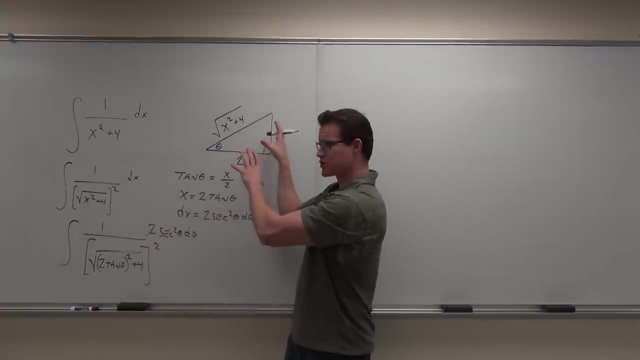 Now, we didn't have to do this. Me, personally, I would have gone straight to my triangle. From right here, I wouldn't have needed that because I'm used to it. But if you need this, you go, okay, well, this is the same thing as something with a square root squared. Yeah, that's true. That will allow you to see the triangle a little bit more easily, let you set up this relationship on our triangle, let you find tan theta equals x over 2, no big deal. But now watch it. What happens when you square a square root? Take it away. It goes right back to what you had. Does that make sense? 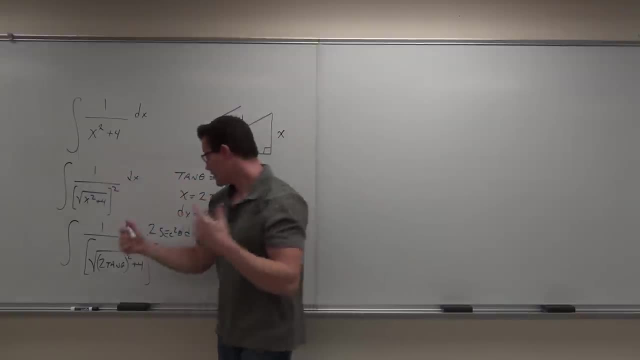 So you really didn't need to do it, but you can do it if it helps you see it. 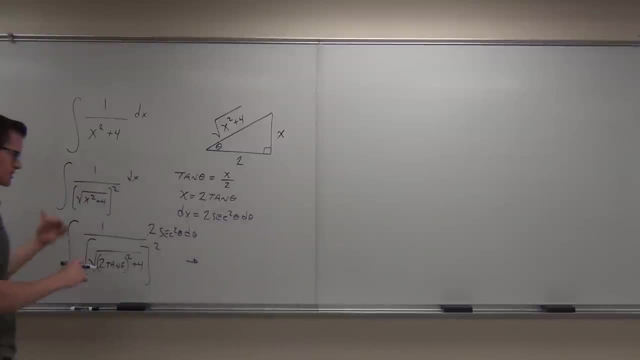 So in either case, what we end up getting, and I know that I did this earlier in class, but we'll do it again. 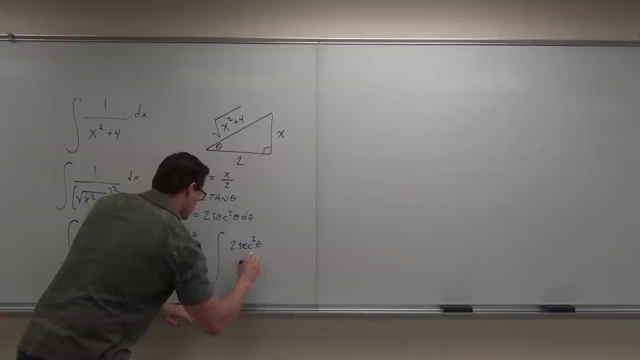 We get 2 secant squared theta d theta over, what happens here is we're going to get, I'm going to do a lot of math in my head right now, just so you, hopefully you're with me here. The square and the square root are gone. You follow? 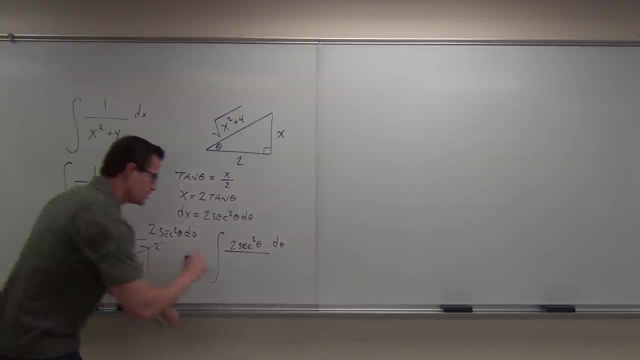 I'd pull out the 4, I'd take a square root of 4, I'm going to get 2. I'd have a square root, I'm sorry, I wouldn't have a square root anymore. The square root's gone. 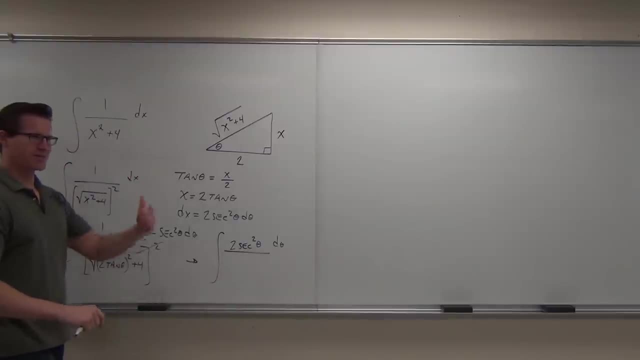 I made a mistake. This is why I don't like to do the square root because it's gone now. 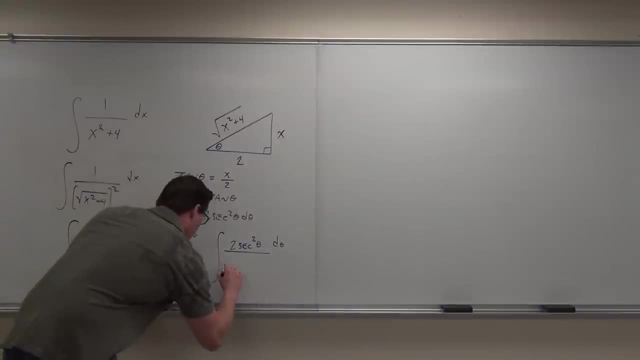 So maybe I can write this and you guys can follow me from here. We'd pull out the 4 and we'd have secant squared theta, shoot. 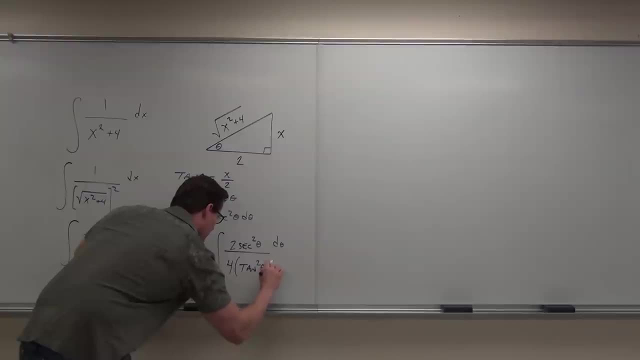 I'm going too fast for my own good, aren't I? There we go. That's gone. We pull the 4 out. 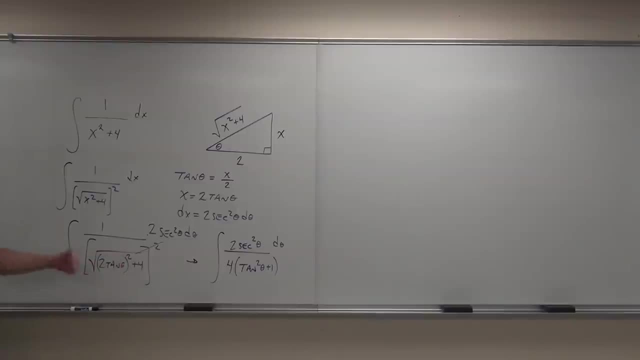 Of course, we square the 2, we square the tangent. Pull the 4 out. After this, we'd have a 1 half. We'd have a secant squared theta. This becomes secant squared theta, d theta. 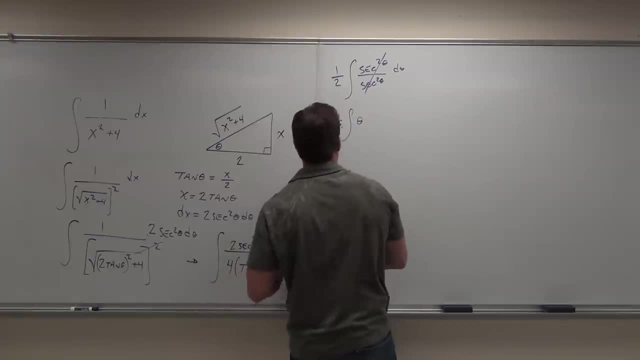 This is 1 half the integral of theta. Again, I'm going too fast. I'm doing the integrals in my head. 1 d theta. We don't even need the 1. What's the integral of what? I. I went fast. 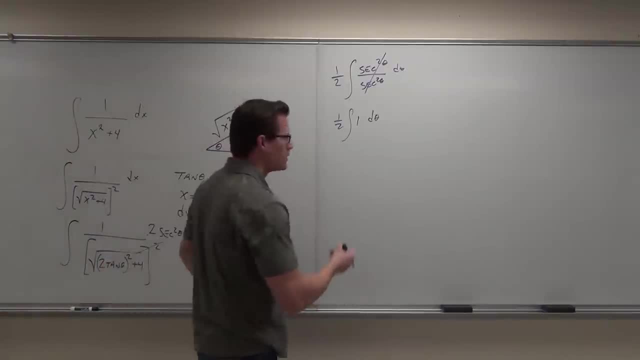 Are you guys OK with getting down that far? What's the integral of 1? Theta theta. Yeah, in this case, it's theta. So 1 half theta. Can I leave it in terms of theta? No. 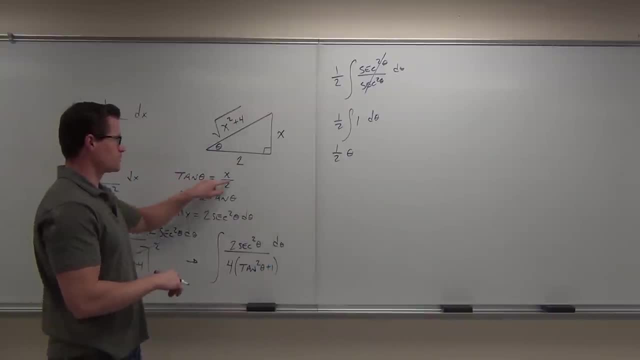 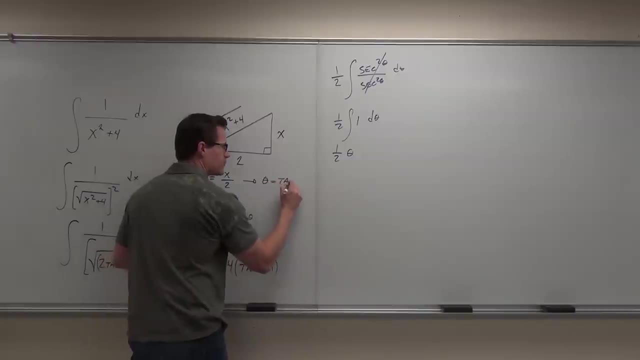 No, but here it is. If tan theta equals x over 2, this happens if and only if theta equals tan inverse of x over 2. Did you guys find that one? Tan theta equals x over 2? Hey, theta equals tan inverse of x over 2. 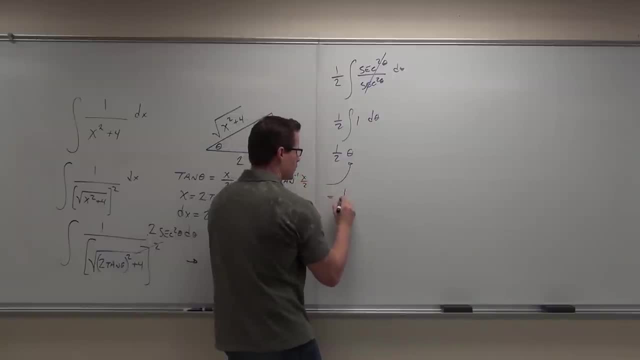 So what we get out of this substitution, we get this. So what we get out of this substitution is that our integral is 1 half tan inverse x over 2 plus c. 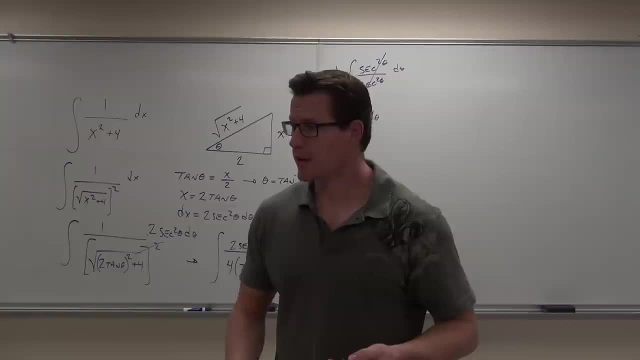 This would be the long way of doing things, but it is a way. Show of hands if you feel OK with the a way of doing it. 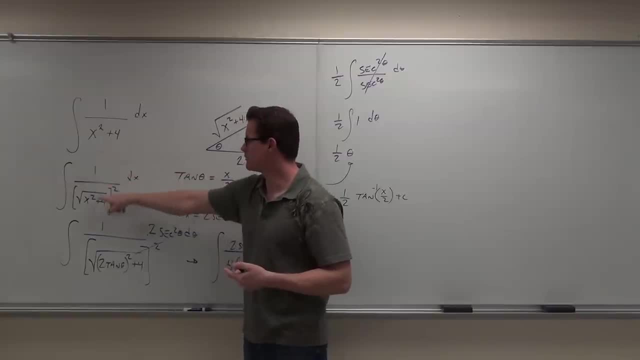 You could do a trig sub just by looking here. You can make it fit more of the trig sub idea. Or you could do this. Here's way number 2. 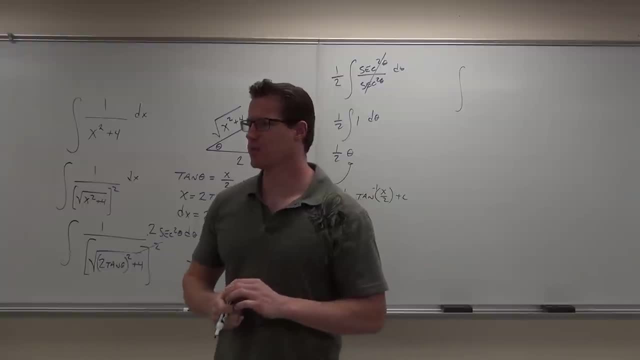 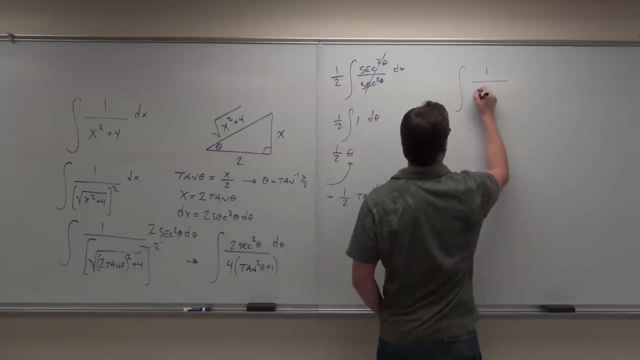 Way number 2 is to try to fit this to an integration table. To try to fit this into an integration table just the way it is. And the way it is would be, well, if I can fit this to u squared plus 1 du. 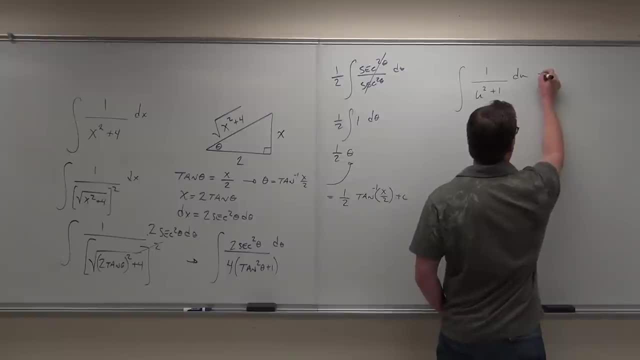 The integral of 1 over u squared plus 1 du is tan inverse of u. Plus c, of course. Well. Here's another idea. 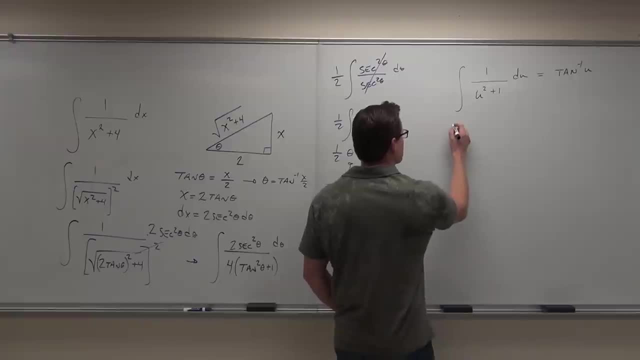 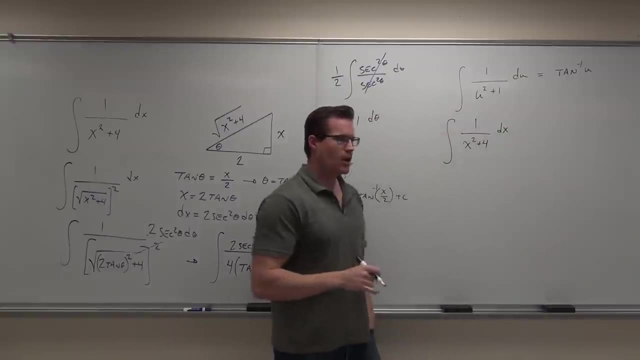 Then instead of going through the whole trig sub idea, well, maybe we just think of instead of 1 over x squared plus 4 dx, we force this thing to factor out a 4 here. 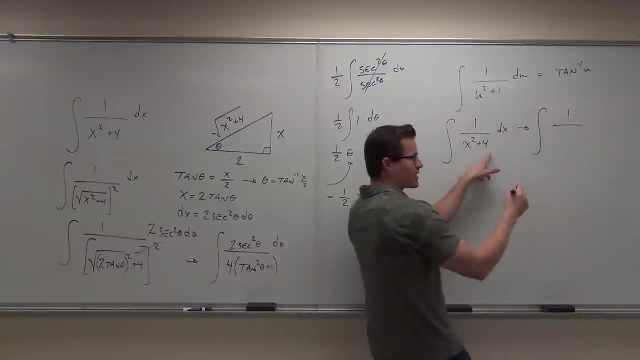 So we could say, OK, well, if I'm trying to make this a 1, I've got to factor out a 4. Are you getting me? 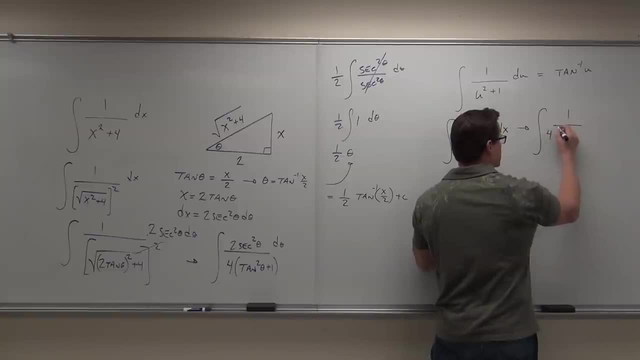 Then I'd have 4. And I'd end up getting inside my bracket x squared over 4. 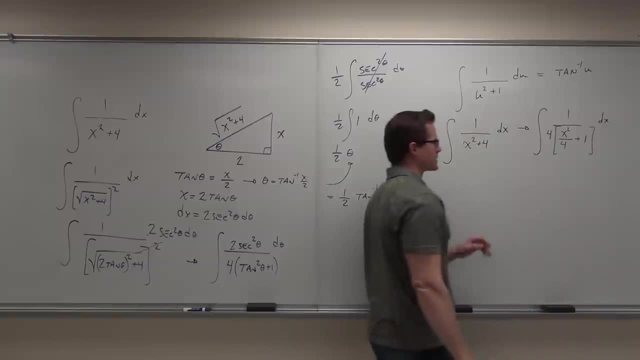 4 plus 1 dx. Do you guys follow the algebra on that? If you don't, just distribute right now. 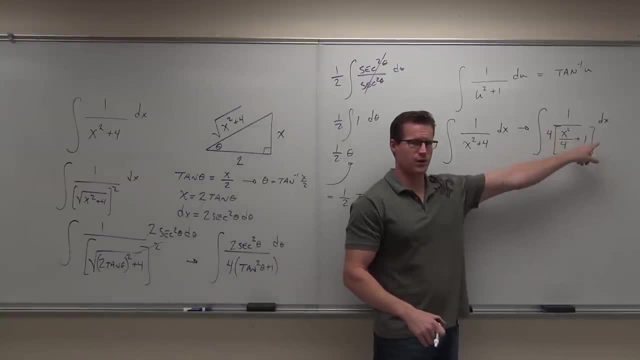 And you'll see that this goes to x squared and this goes to plus 4. Do you follow? Then what I need to do to fit this format, I need to make this as something squared. So x squared over 4. No, no, no. 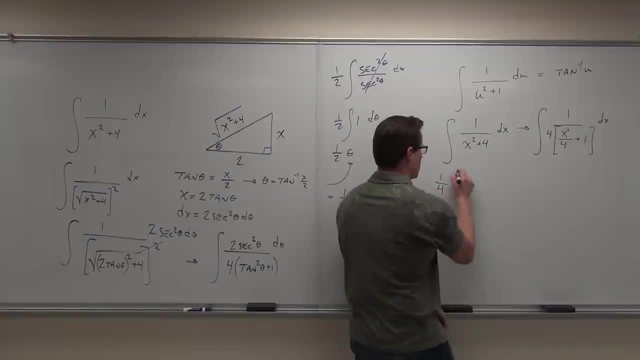 I'm going to pull the 1 fourth out. I would have 1 over x over 2 squared plus 1. OK. 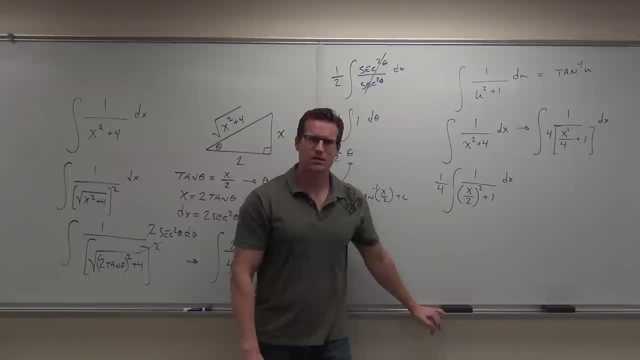 Plus 1. Does that make sense to you? 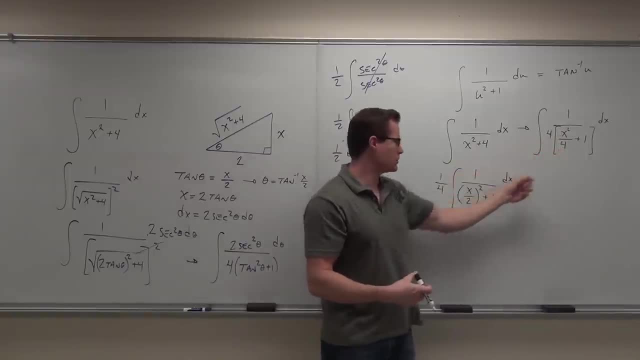 So instead of x squared over 4, no, no, let's think of this as something squared. Let's do x over 2 squared. You'll notice that 1 fourth is outside, out front. 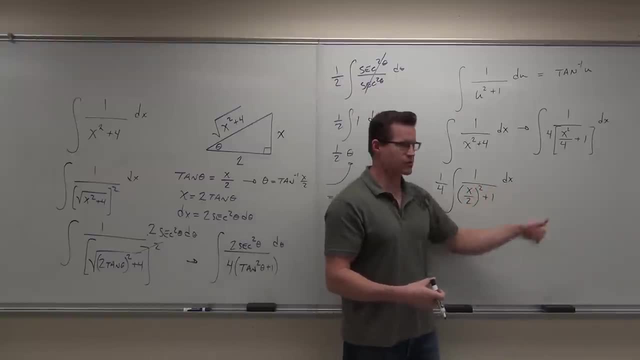 This becomes x over 2 squared. That's still x squared over 4 and then the plus 1. So far so good? 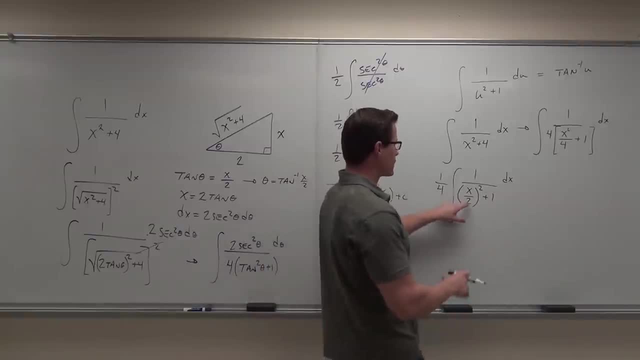 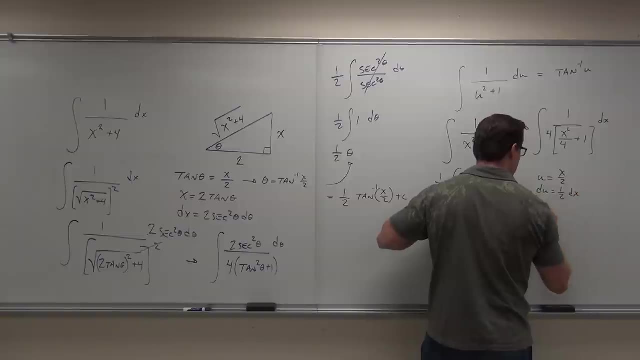 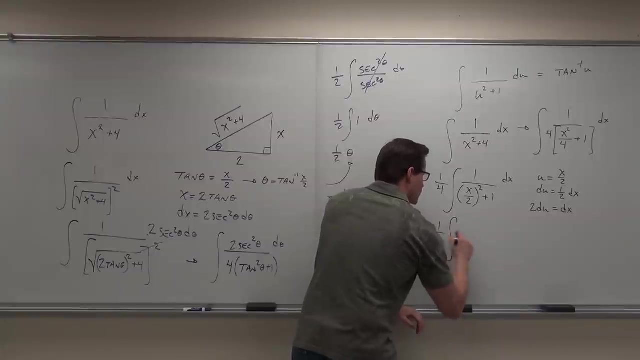 Now you're doing just a basic u substitution, basic. So the u equals x over 2 du equals 1 half dx. 2 du equals dx. And what we end up getting is 1 fourth the integral 1 over, what's the x over 2 become? u. Yeah. 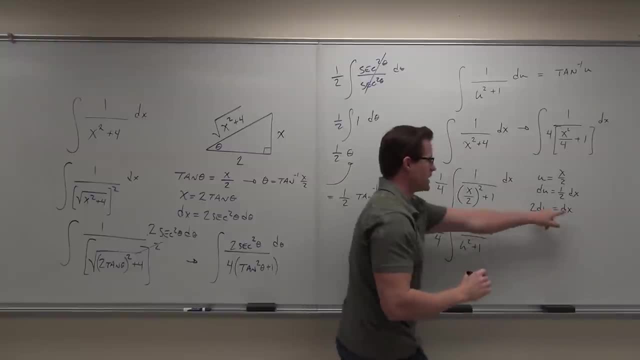 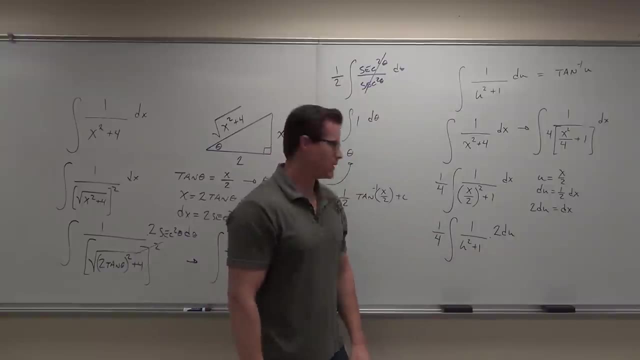 u squared plus 1. And then we have 2 du. So instead of dx, we get our 2 du. Tell me the next thing I'm going to do. Pull out the 2. So I get 1 half, 1 fourth and 2. The integral of 1 over u squared du. 1 over 2. 1 over 2. 1 over x squared plus 1 du. 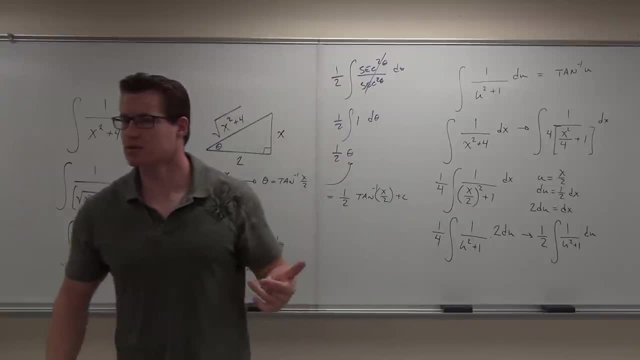 Hey do I know of the integral of u squared, 1 over u squared, plus 1 is? Tan inverse of u. Tan inverse of u. 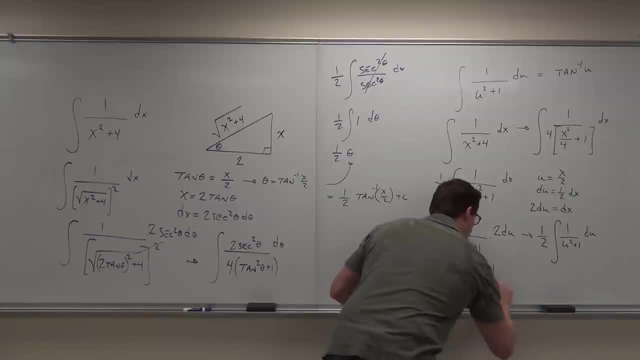 So this becomes 1 half tan inverse of u. How much is u? x over 2. Plus c. It ends up being exactly the same thing. 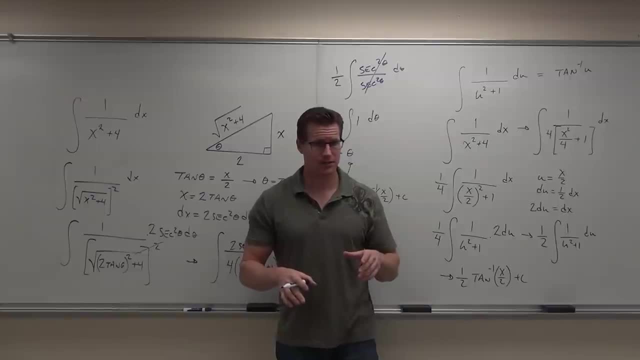 So if you ever see, and you're going to get this a lot. Listen. You're going to get this a lot. One of these things where you have 1 over x squared. 1 over x squared. plus 9 or plus 1, if you see that, how many ways can you go about doing it? And either way is fine. 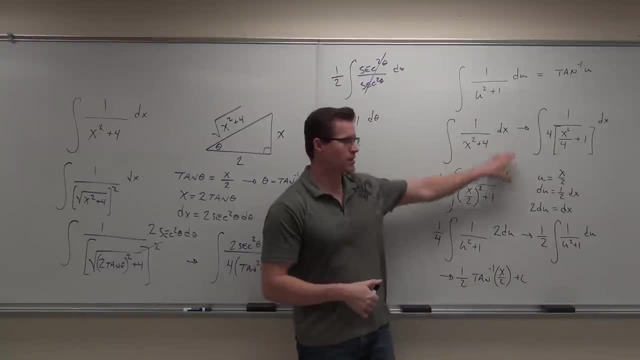 If you want the quick way and you want to do just a little substitution, do this. If you like the triangle method, do this. Do I care? I don't care. So as long as you can do one of these ways, I'd say do both of them. 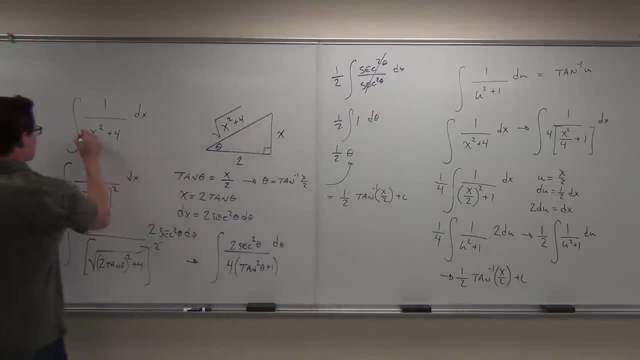 Sometimes this is going to be nicer because if I do this, like that, you can still do it. Here, you can't. 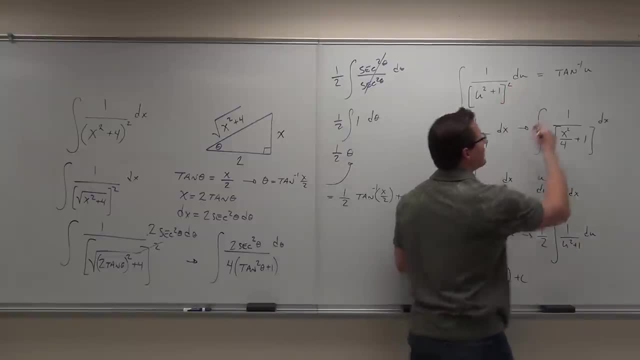 If I do this, this is not this. No. Don't do that. 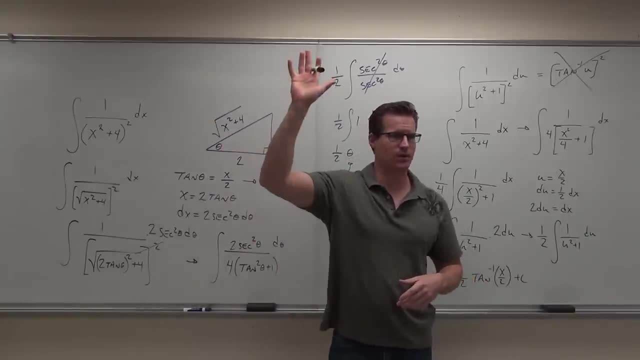 So then you'd have to do something along these lines. So if I just feel OK with this one. Now, that was a little bit slower. But I just want to give you a heads up on what you can and can't do with this problem. Did that explain it well enough for you guys to understand it? OK. 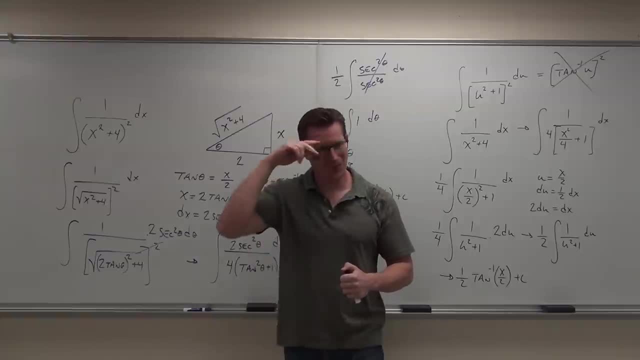 Can we go on to our last example? Yes. Last one. Let's do it. I'm glad you said yes. I was going to anyway. 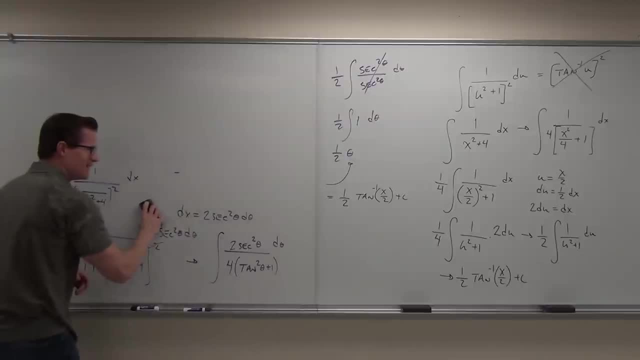 But now that I have your approval, it could much be better. 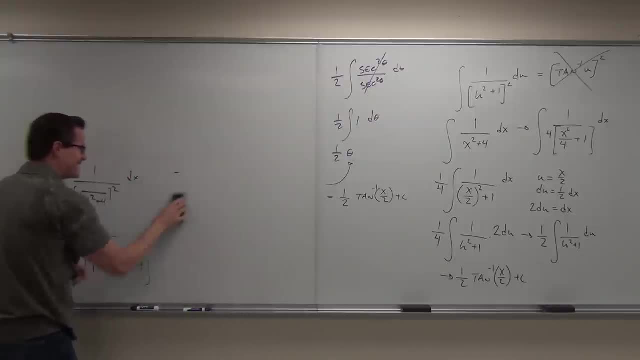 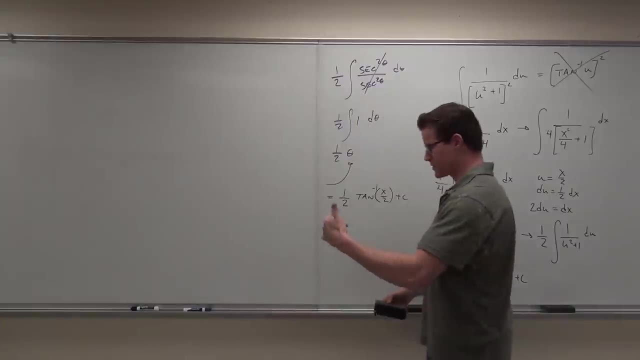 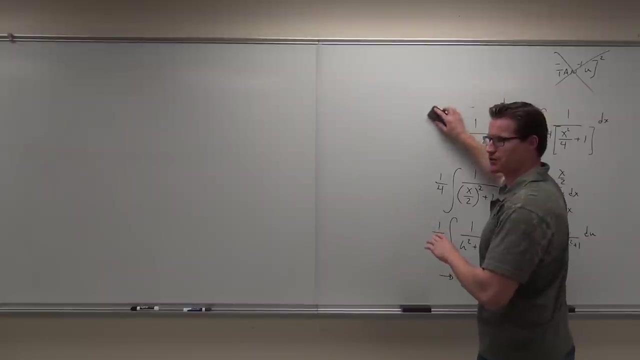 By the way, were there any questions on this? Too late. We did this stuff earlier in chapter 6, right? We did this stuff earlier in chapter 7, as far as the tree sub. We also did all sorts of stuff in chapter 7. 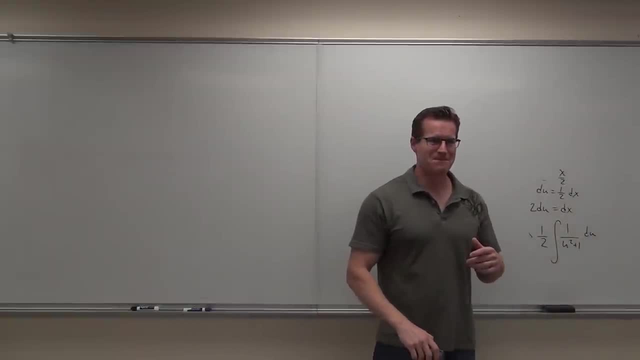 You guys got plenty of paper today, right? What? A notebook full. 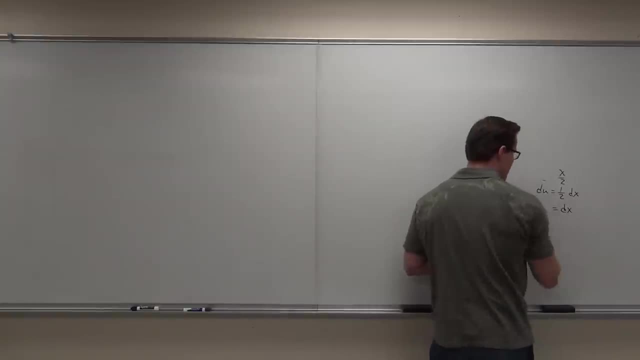 Paper? I hope you have a notebook full. This is going to take a few pages of paper for you. We'll start a new page, then. Maybe start a new page. I'm going to need at least two of these boards for this. So heads up. 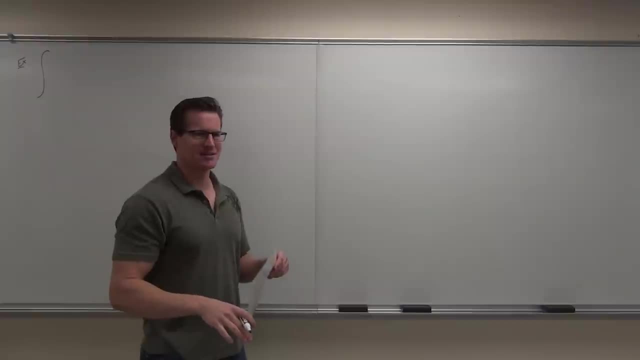 This is going to take at least a gig or two of video, at least. Probably two gigs. What's my next example? What's my next example? This example. Two gigs. Oh, my gosh. It's this. It's this much. See? This and this. 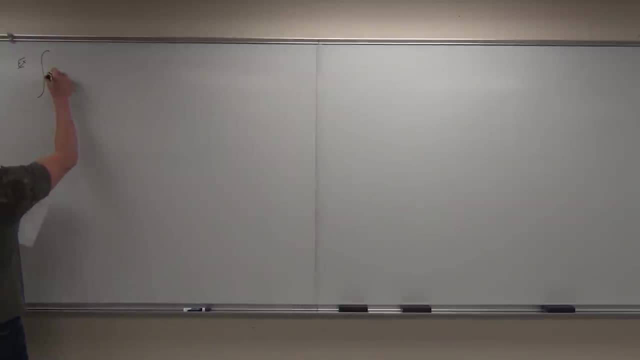 That's one. Yeah. That's not good compared to grad school, so. 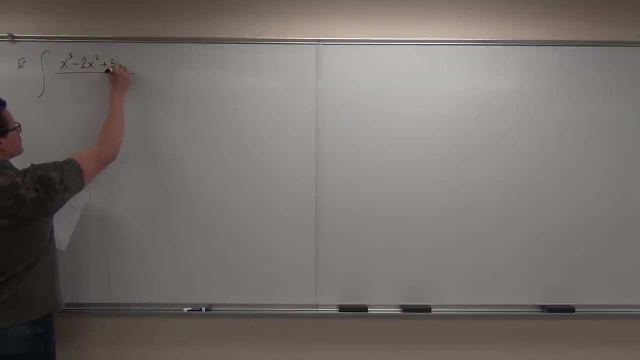 Don't worry. You're going to know how to do all of it. It's not hard. It just takes a lot of steps. Oh, my god. We're going to have a long division. No long division, because I'm a nice guy today. Awesome. Let's see who's the greatest. Long division is not that bad. I like long division. 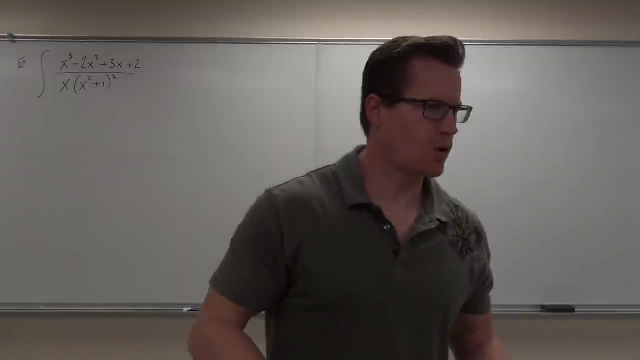 OK, so let's take a look at our example here. Let's see what exactly is going on. Remember that we have had three cases so far, haven't we? Yes. 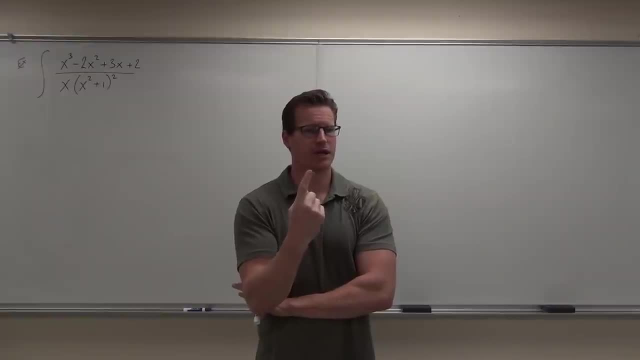 Our first case was the easiest one. You get a lot of LNs. It's just linear factors. 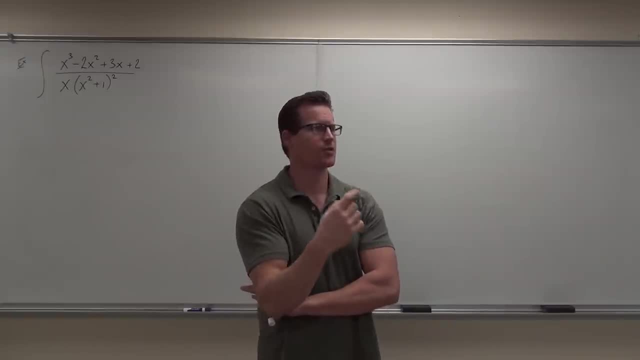 The denominator is all linear factors, like x plus 1, 2x minus 3. Those are linear. And the next case after that, case two, was you have linear, but then you might have repeated linear. And remember building up on the repeated linear? You do for every power until you reach the highest power. 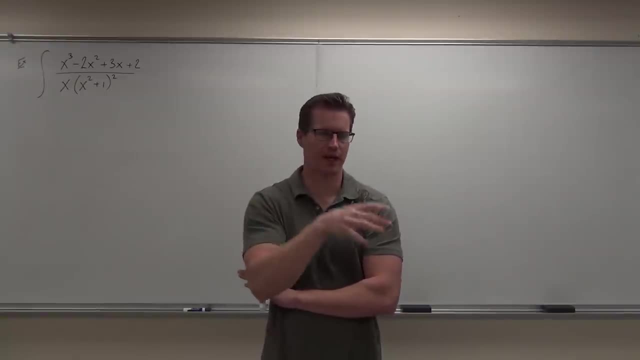 So a over whatever, b over whatever, c over whatever, and you build that up. 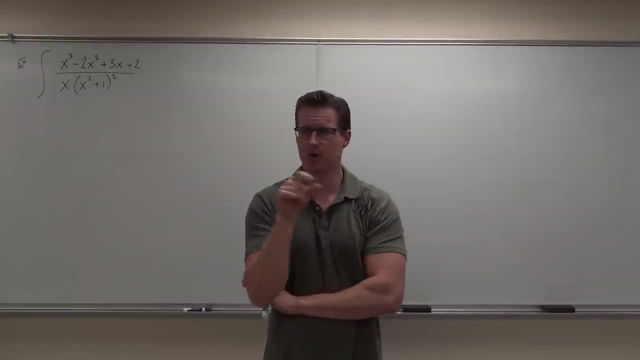 Now, when we got to quadratics, irreducible quadratics, we no longer had just a constant numerator. 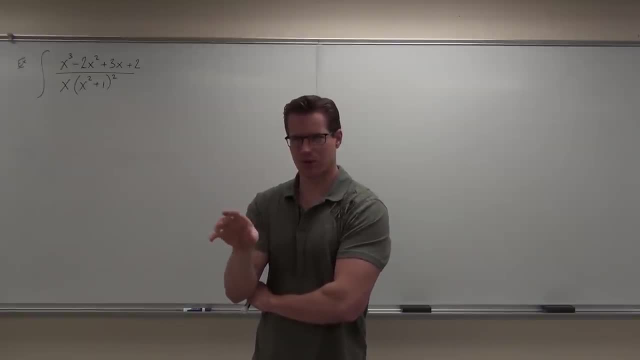 We had one, did I tell you this? It's always one degree lower than what your factor is. So for linear, we have constants. For quadratics, we have linears. That's what our numerators are. 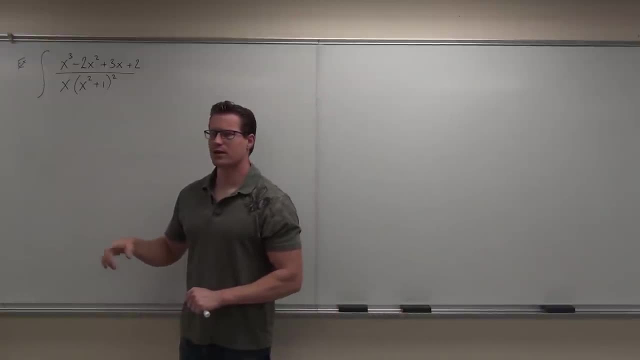 Well, this last case is not just linear. By the way, can you tell me what the linear factor is here? 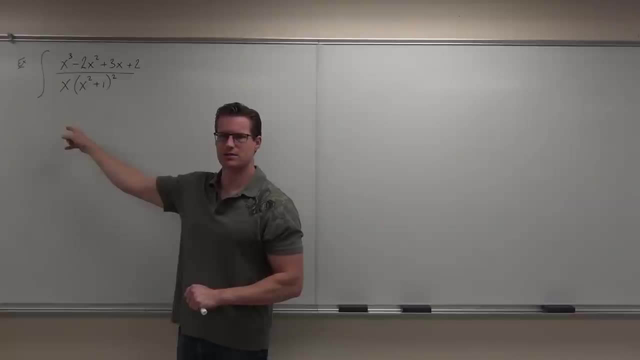 Whatever that is, turn it off now. Can you tell me what the linear factor is? x. Yeah, that's linear. We're going to have a over x right now. You with me? 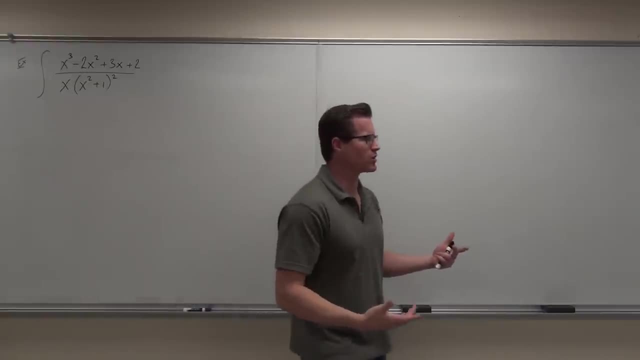 So we don't just neglect our previous knowledge of, hey, what do you do with linear? You're kind of building on them. 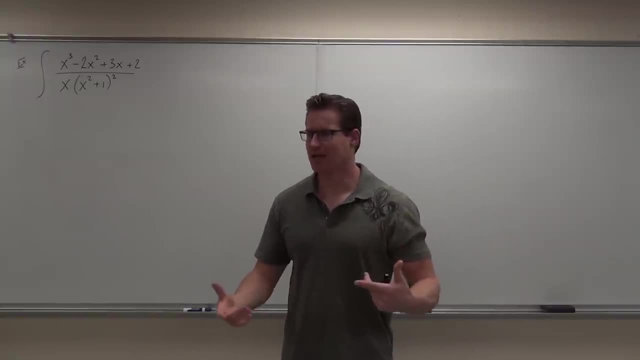 So you can have more than one case in each example. So linear, sure. 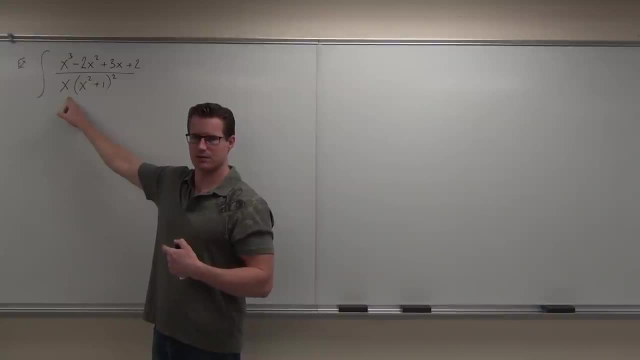 Now, do we have any irreducible quadratics up here? x squared plus 1. x squared plus 1. Yeah, that's an irreducible quadratics. Can you factor that? No. That's irreducible. 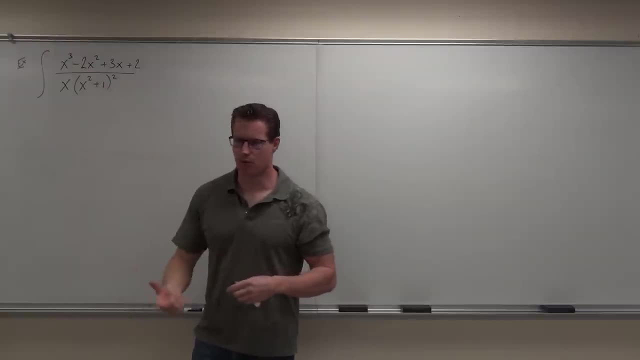 But we also have it repeated. To a power. And this is our case 4. 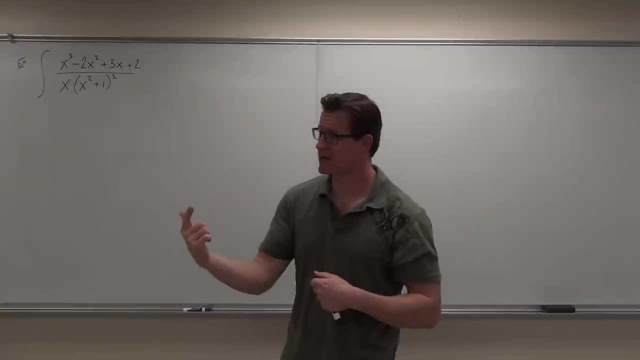 So we had linears. Then we had repeated linears. Then we had irreducible quadratics. Now we have repeated irreducible quadratics. So this is our case 4. 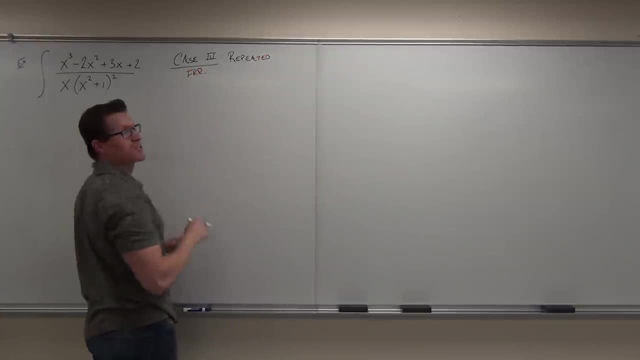 You forgot the dx. I wasn't done yet. 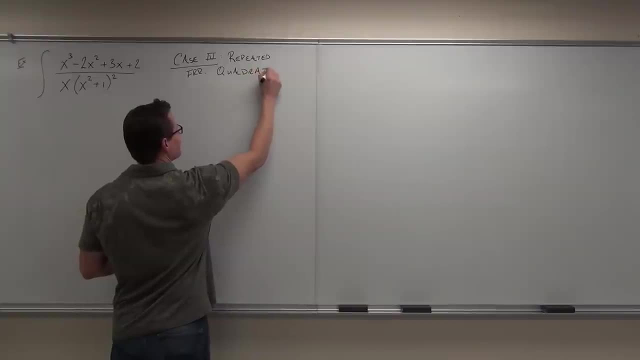 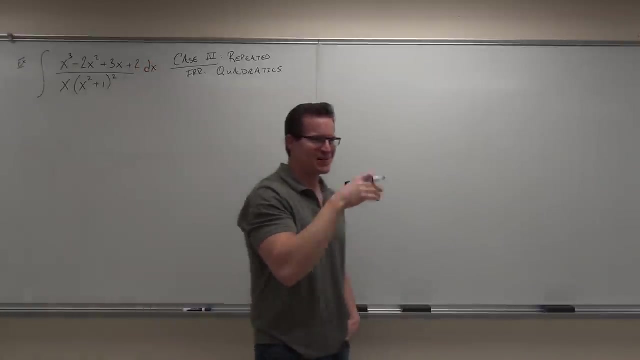 So now that we're ready to go on our example, let's see what happens when we do this. Now, before we go and do this, I want to give you an example that's we're definitely not going to go through this whole thing, all right? I want to see if you understand how to build your partial fractions from this. 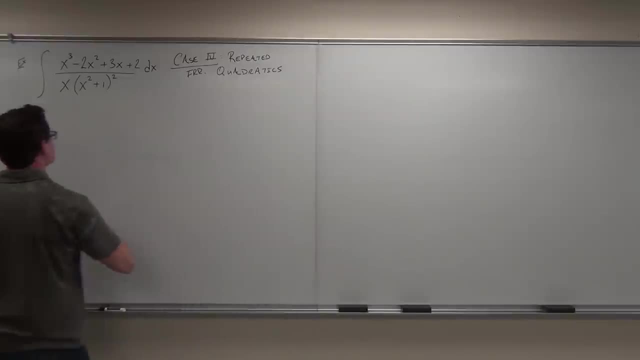 So a little sidestep, OK? Let's say that I had. Not even an integral. Just this thing right here. 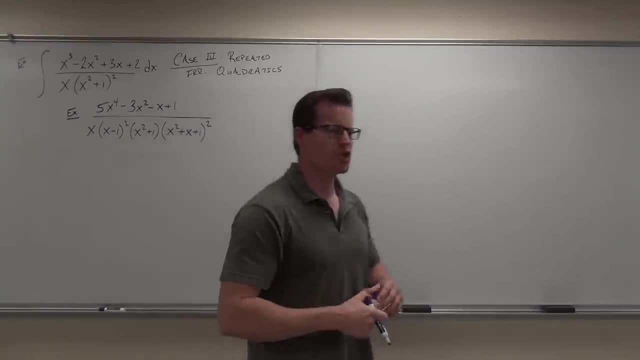 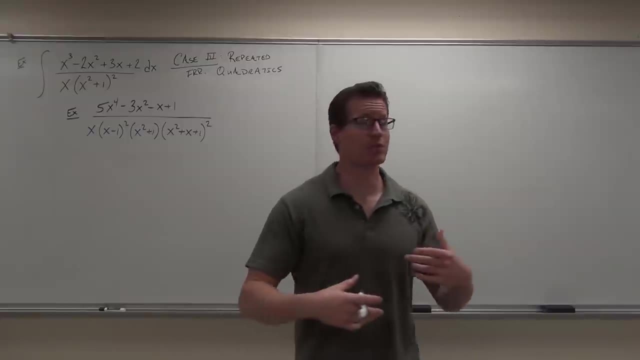 If I gave you that, would you know how to write the partial fractions to it? This has every case that I can imagine here. So I think it's kind of nice for us to go through this just so you see what's actually going on. Are you guys with me on that one? Yeah. 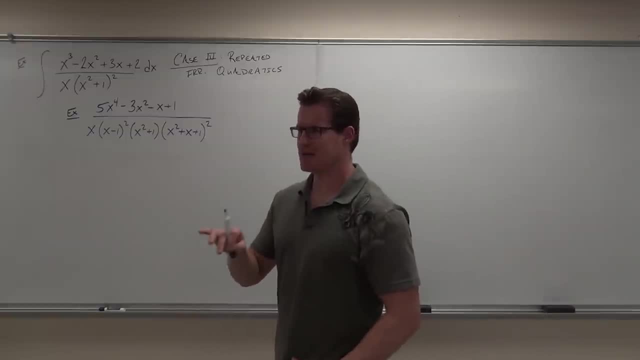 First thing you check for is can you factor your denominators any more? 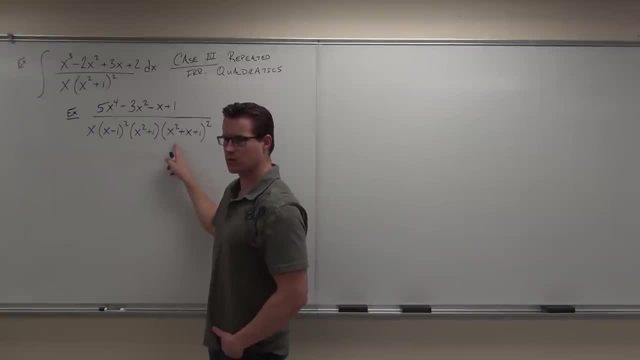 No. No. Factor. No. No. No. No. No. So these are all non-factorable. Do you believe me? Yes. OK. 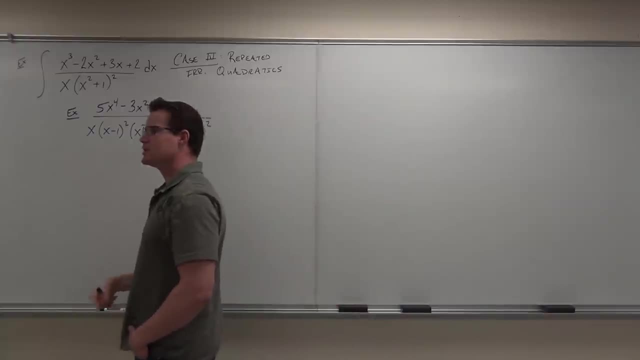 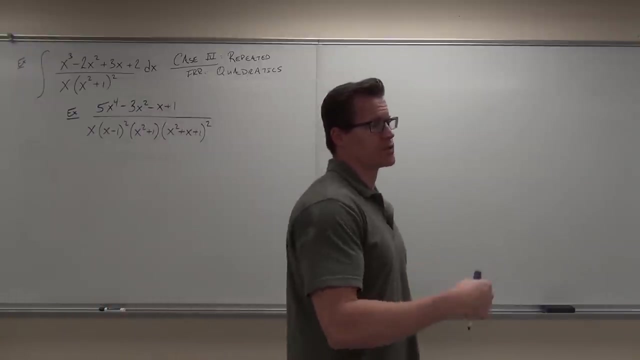 So they're completely factored. Now, when we go through this, you need to be good at identifying what linear factors are, what repeated linear factors are, what irreducible quadratics are, and what repeated irreducible quadratics are. 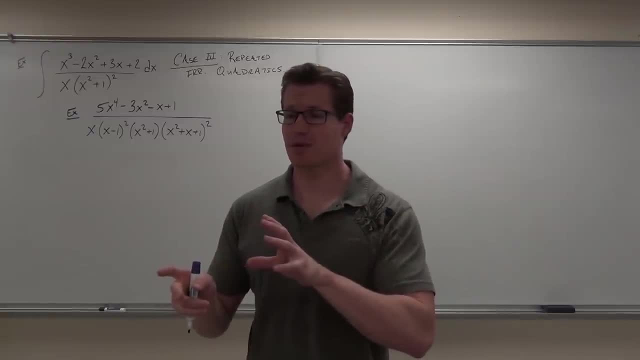 The same method we use for repeated linear is the same thing we're going to do for repeated irreducible quadratics. Same basic idea. 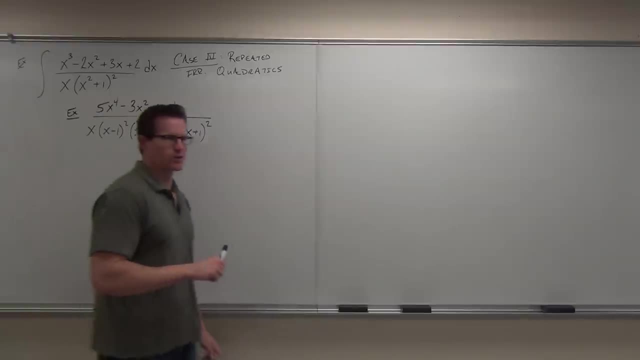 So when we go through this, oh yeah, you know what the next thing we talked about? You've got to check the degree. So how in the world do you check the degree here? What's the degree of the numerator? Four. Four. What's the degree of the denominator? Three. A lot more than that. A lot more than that. A lot more. 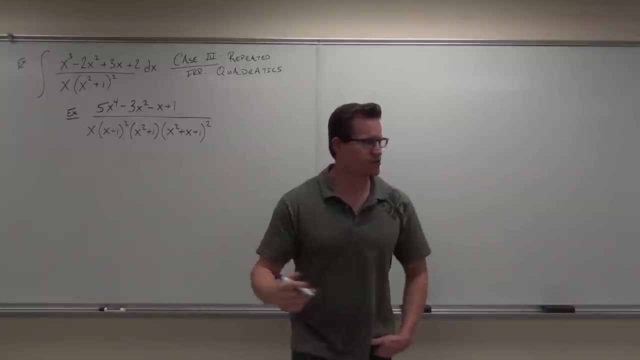 Because degree is after you've distributed everything, right? So let's start here. You'd get an x to the fourth somewhere here, would you? And you'd get an x to the sixth. 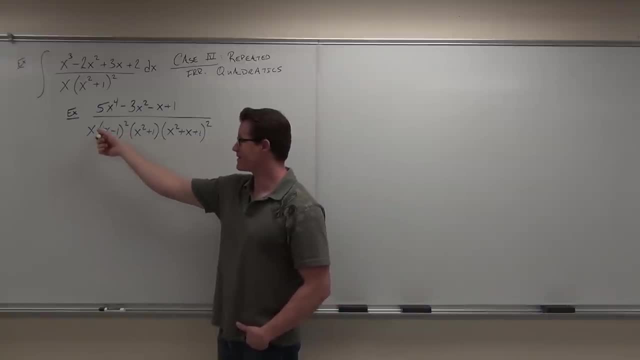 Then you'd get another x squared. So you'd have x to the eighth. x to the ninth. Basically, you'd have an x to the ninth somewhere up here. 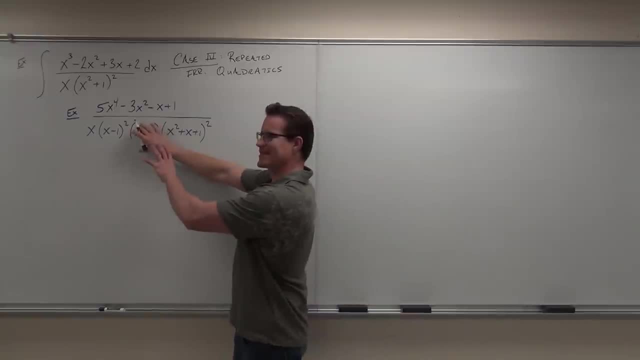 Do you follow? So naturally, our degree here is less than the degree on a numerator. So degree of denominator is less than degree of denominator. And that's what we're looking for. 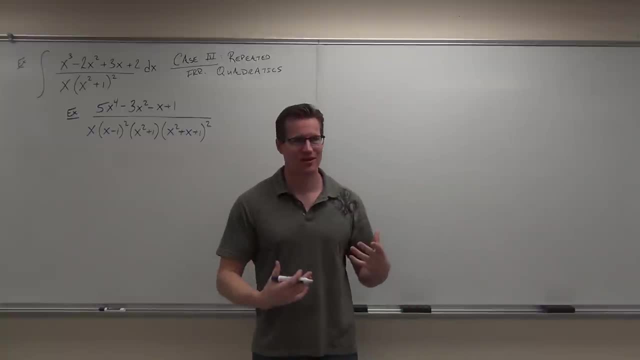 Thank goodness, because if it wasn't, what would we have to do here? You'd have to distribute it and then do long division with it and then refactor it would be crazy again after that. But anyway, this would be the idea. Should we be OK with the idea? No. 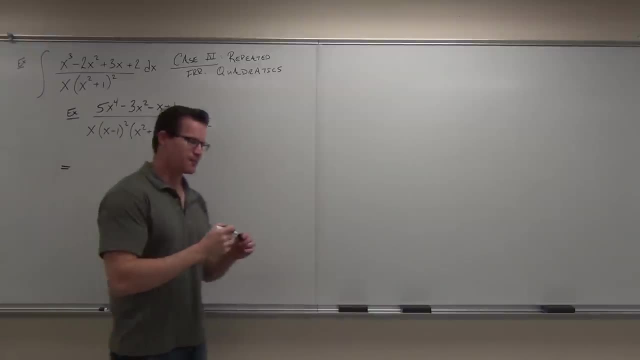 Let's see if you're good at telling me how many fractions we're going to get. Don't say it out loud. 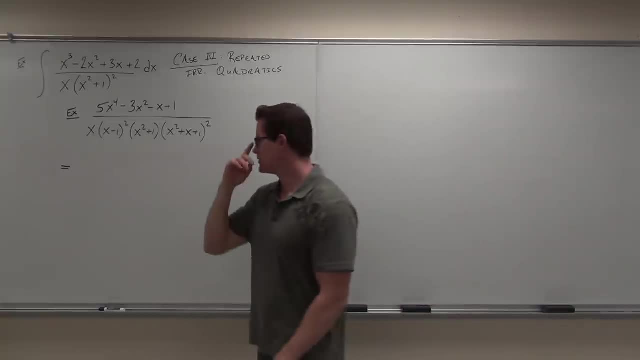 I want you to count them up, how many fractions you're going to get, OK? Don't say it out loud. 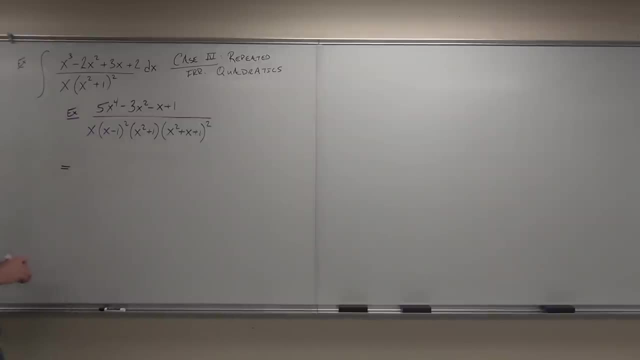 Everyone do this. How many fractions we're going to get? Have you counted? Letters or fractions? Fractions. How many fractions we're going to get? Four, six, seven, eight. 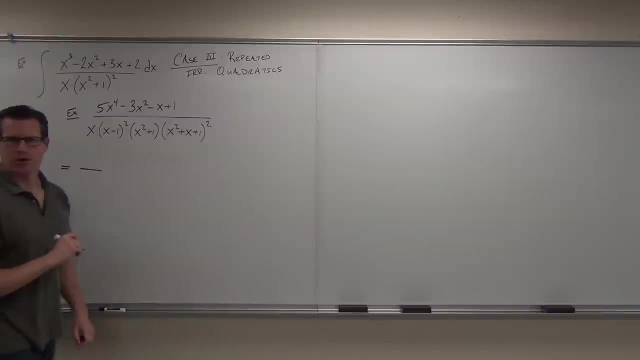 Let's see. Do you remember what to do with our factors here? Let's see. 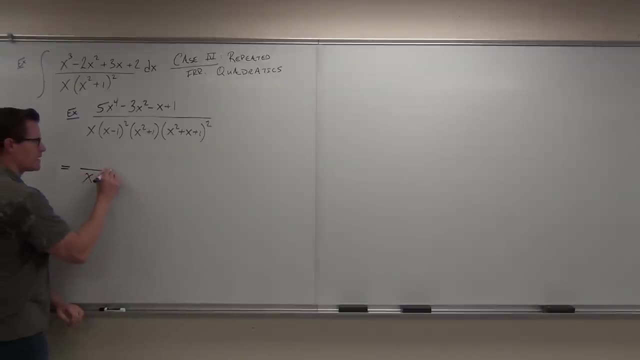 What's the first one going to be? X. And then I'm going to have another one with? X minus 1. Oh, so with repeated, remember this? When they're by themselves, no problem. 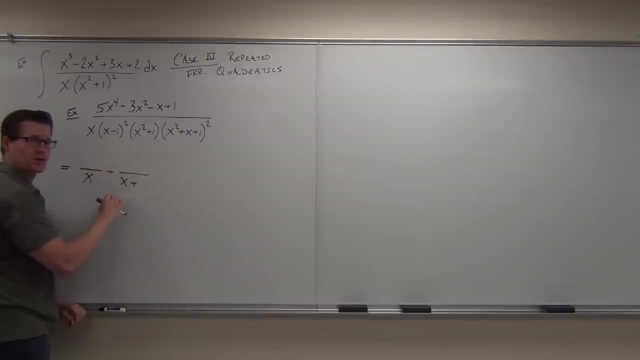 When they're repeated, you put the first power. You put the first power correctly. Then you put? X minus 1 squared. 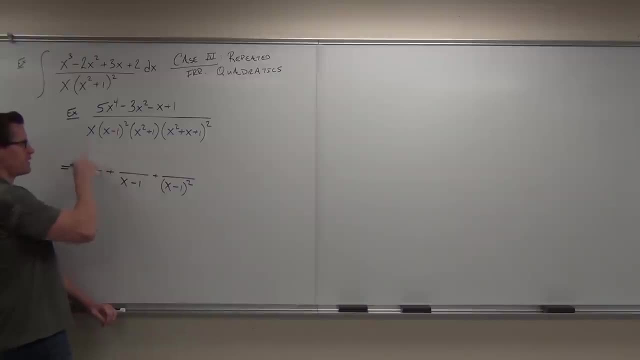 Until you build up to the greatest power here. So here we have x, we have x minus 1, we have x minus 1 squared. That's what repeated linear was. 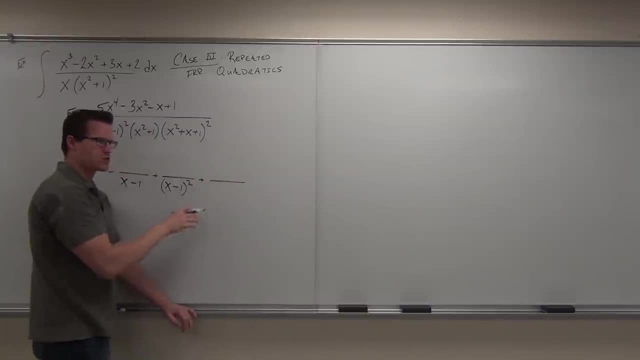 Remember that? Let's just work on all the fractions right now. Then we'll fill out the numerators. What's next? X squared plus 1. You go to your next one. 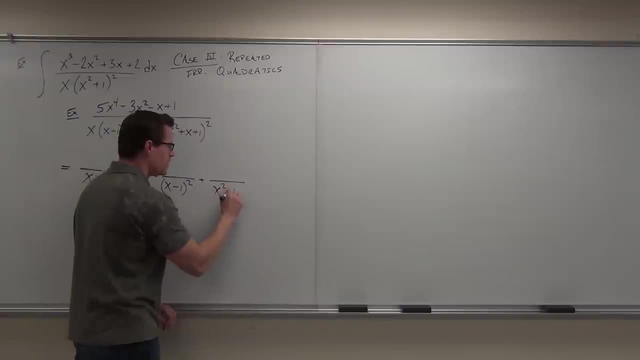 So our repeated, our quadratics. So x squared plus 1. That one's not repeated, so I'm good to go. 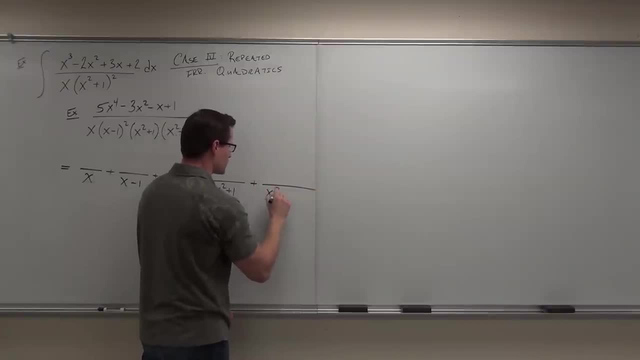 After that, what? X squared plus x plus 1. 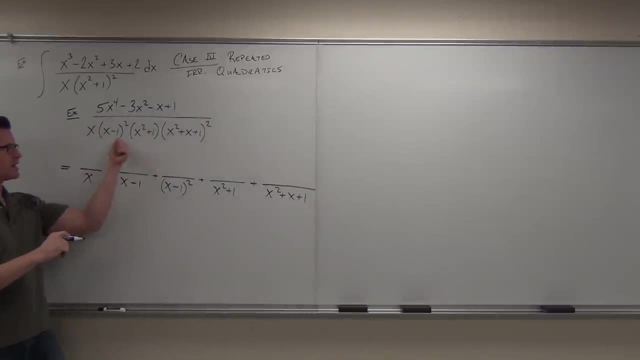 The same thing we did with our repeated linear. So here we had x minus 1. Then we had x minus 1 squared. You take every power up to the largest power. So here, x, no problem. X minus 1 squared, well, you've got to have an x minus 1. Then you've got to have an x minus 1 squared. X squared plus 1, no problem. That's not to a power. 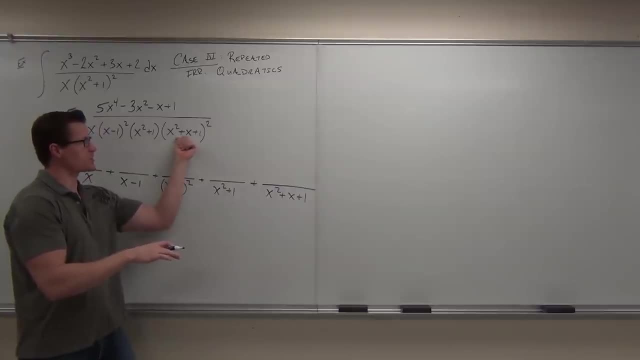 So we just have one of those factors. Here, this is repeated. So I have x squared plus x plus 1. But then I'm going to have another one because it's repeated. 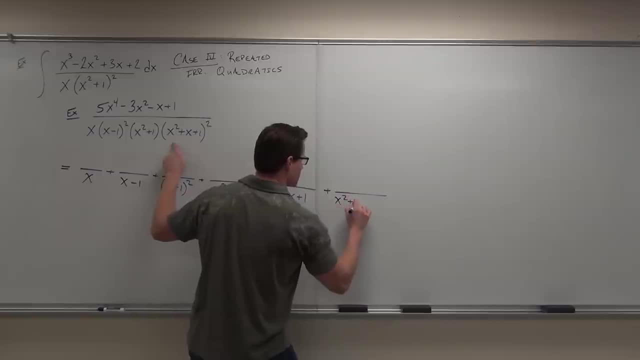 You have to go to the largest power that you have. And x squared plus x plus 1 squared. 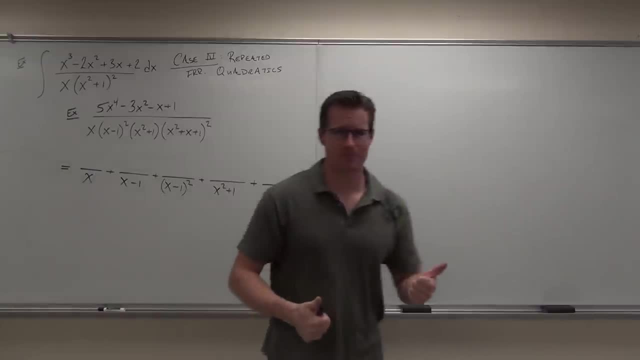 1, 2, 3, 4, 5, 6. If those people said 6, you're right on the money. If you didn't say 6, do you understand why not? Why don't we get 6 now? You sure? OK. 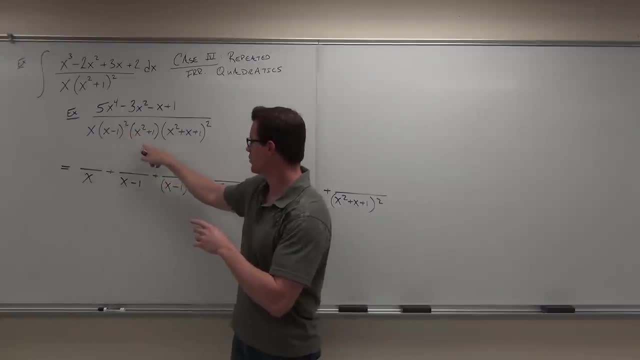 So we got this. Hey, repeated. You're going to have two of these. That's what it says, 2. 1, 2 of these. 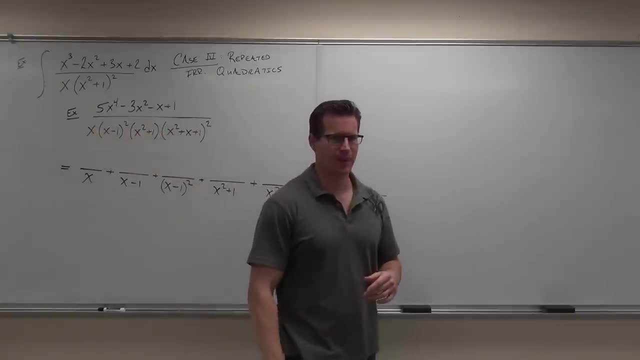 So 1, 2, 3, 4, 5, 6. Just count the powers up. That should be how many fractions you actually get here. So far so good? OK. Especially if I would have something like this. A lot of people screw this up. 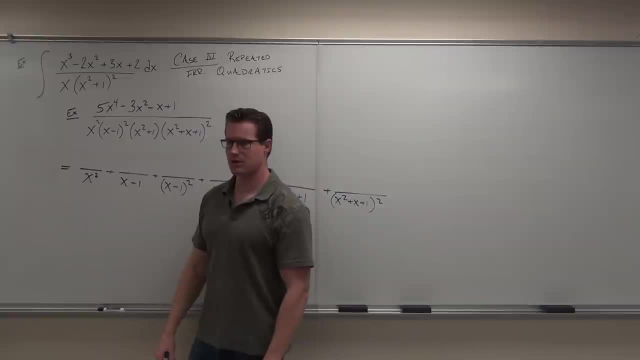 A lot of people do this and they do that. Is that the appropriate thing to do? No. You'd have an x. And then you'd have an x squared. 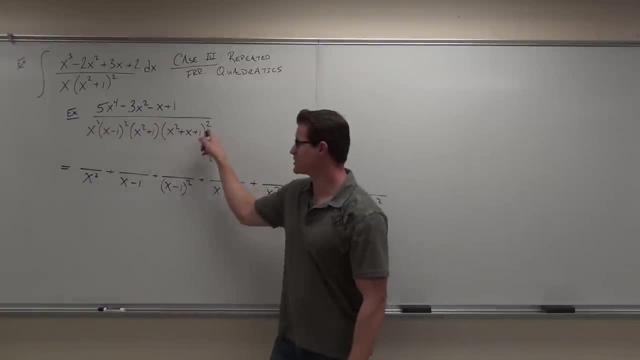 So if you count the powers, 1, 2, 3, 4, 5, 6, 7. This would give you those 7 fractions that you should have on this example. You OK with that one? Now, let's go ahead. 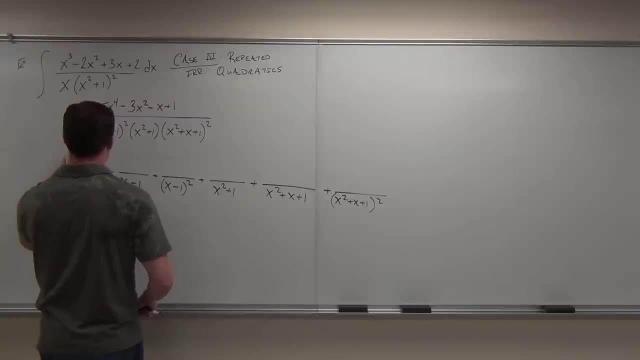 I'm going to erase that again. Let's figure out what we should have. 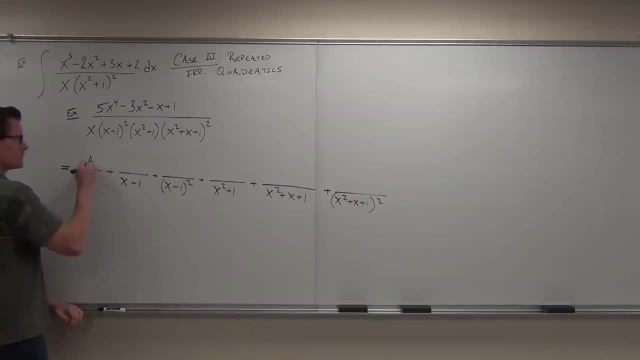 What's the first letter we would start with? A. It's linear. Next one. B. Good. How about? C. This would be C. Yes. 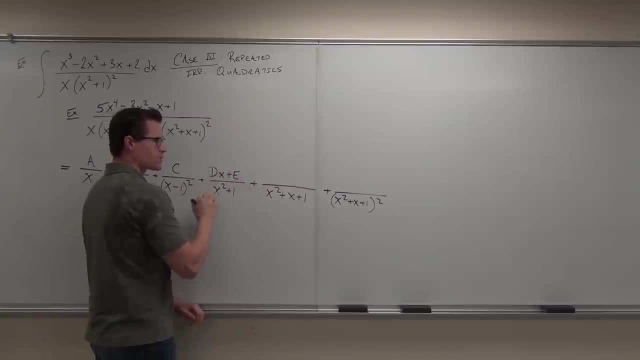 That's still C because it's repeated linear. Every time we get a quadratic, we have a degree left. So power 1, power 1. This is repeated linear. 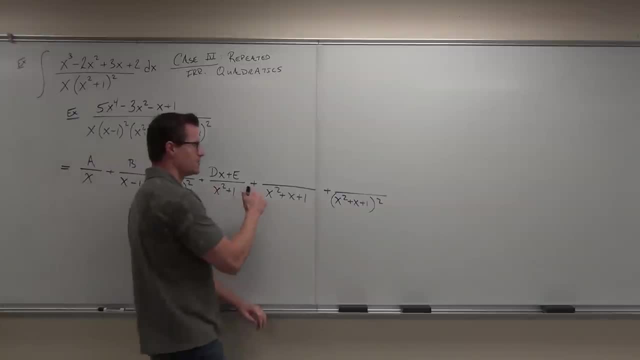 It counts towards linear. So we have a C. We have dx plus E. We have? 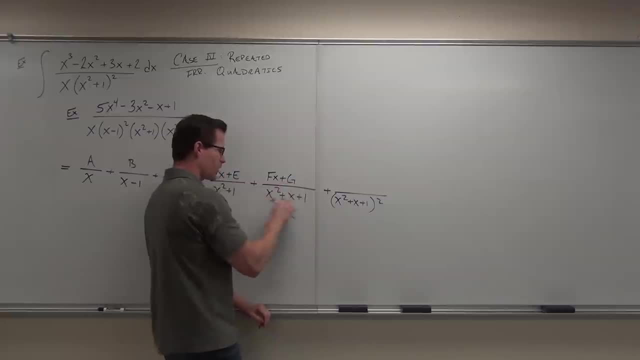 fx plus g. Quadratic? hx plus g. A, b, c, d, e, f, g. 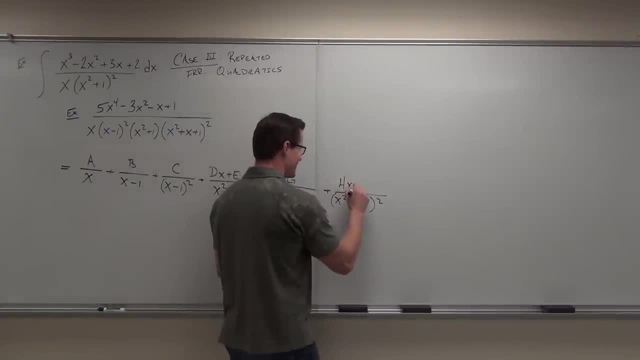 hx plus i. hx plus i. Fantastic. That would be the idea. Why? I just put it over the floor. This is the idea. Chopin should be OK with this one. This is why we're not doing this because this is crazy. 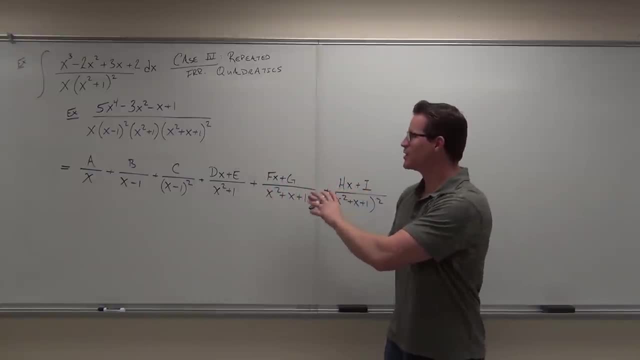 But you could. You really wanted to. You could find your problem. You could find your common denominator. 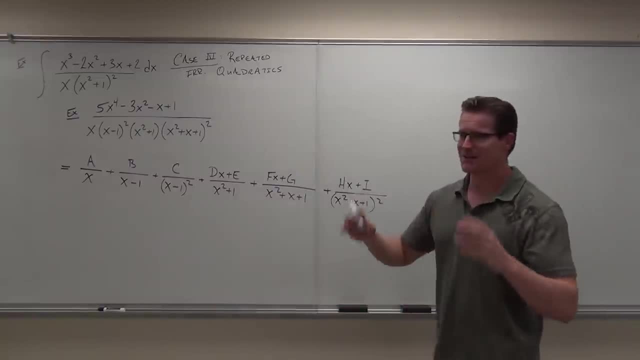 And you could figure out your a, b, c, d, e, f, g, h, i, l, m, n, o, p, whatever you get out of there. And you could do your partial fractions. 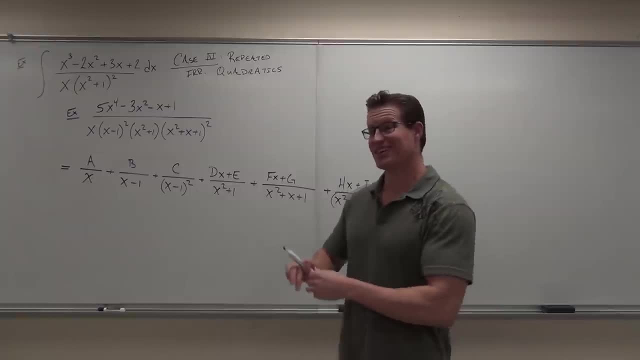 There's an easier way? There's no easier way. This is it. 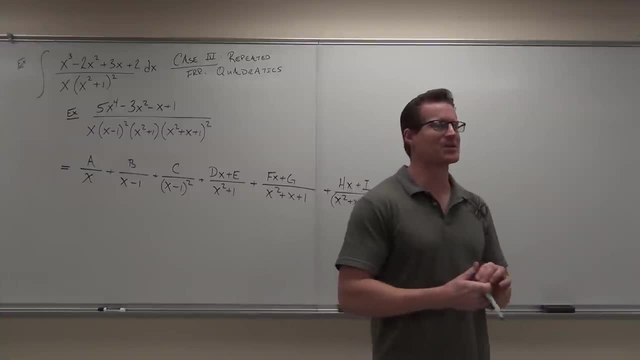 This is the partial fraction reduction for this. Our decomposition, as we say. 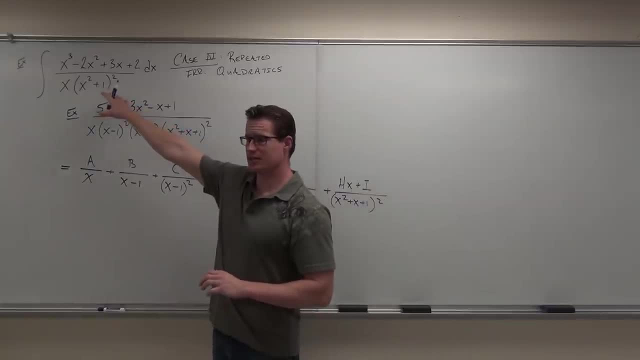 Now, fortunately for us, this one should be substantially easier than this one. We have a lot less fractions to deal with. What I want to know is, does this actually make sense to you guys? Yes. So we count our powers. 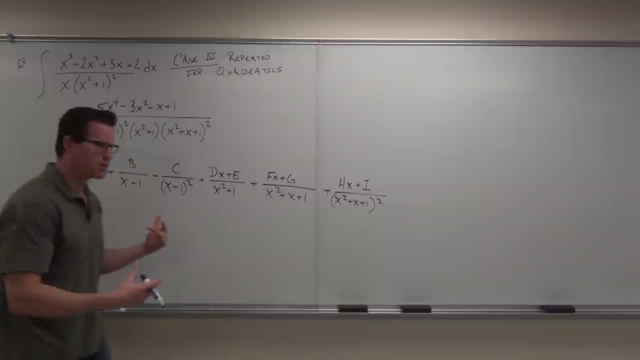 Make sure you have that appropriate number of fractions. Make sure that you don't do silly things like put a bx plus c here. Don't do silly things like forget to do the x plus e. Don't forget the x's. 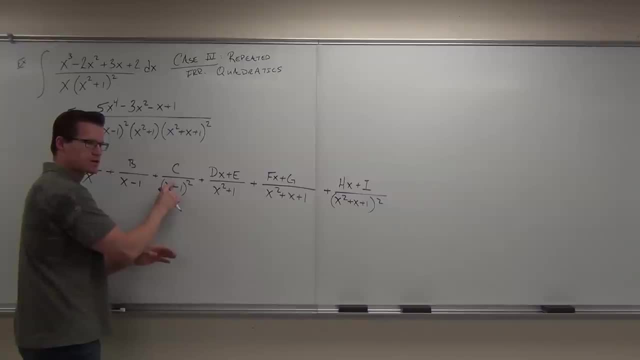 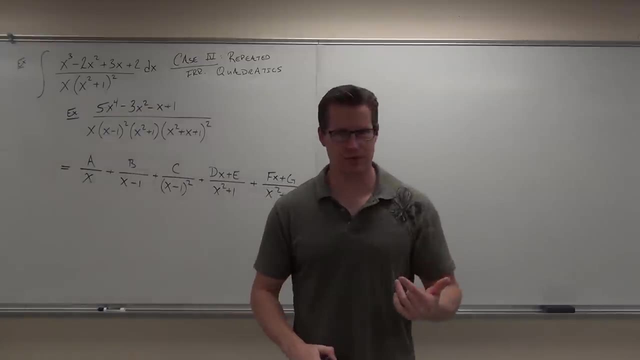 It's always going to be one less degree than whatever power that is. This count is linear. You don't need a cx plus d here. But for every subsequent one where we have our original quadratics, you definitely do need that. 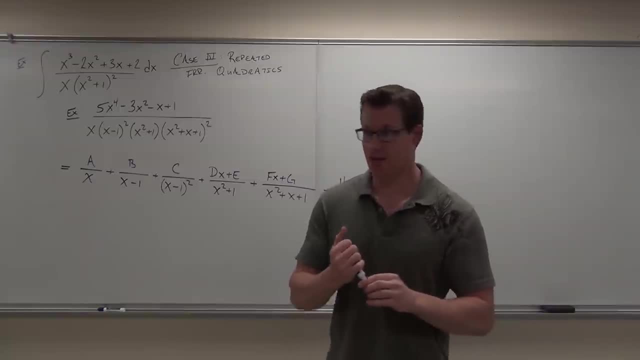 Any last minute questions before we get on to our actual example? OK. 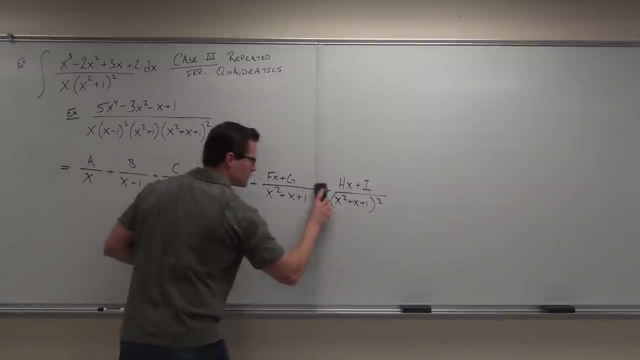 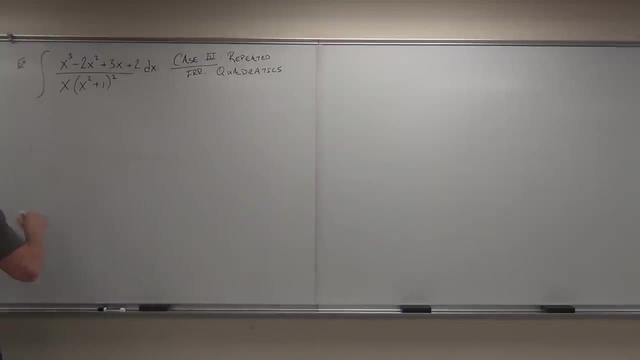 The rest of this thing is going to take us a while. I'm going to erase this because I need the room. Let's go back to this one. 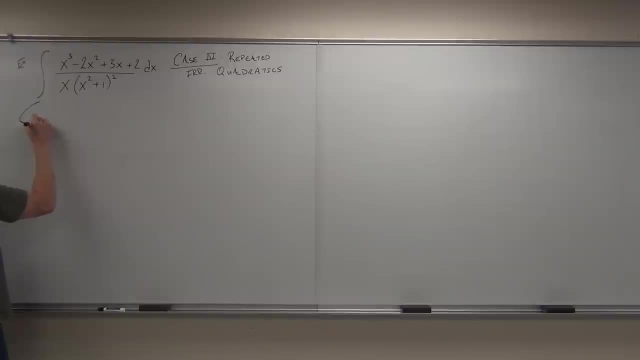 If we're looking at this, then what we know is that x cubed minus 2x squared plus 3x plus 2 over x times x squared plus 1 squared can be reduced into some partial fractions. Question. 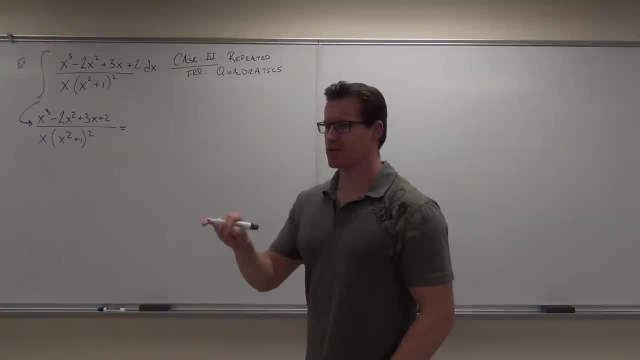 Is the degree of the numerator less than the degree of the denominator? Yes. Yeah. This counts as x to the fourth. Here's x to the fifth. That's more than x to the third. That's great. 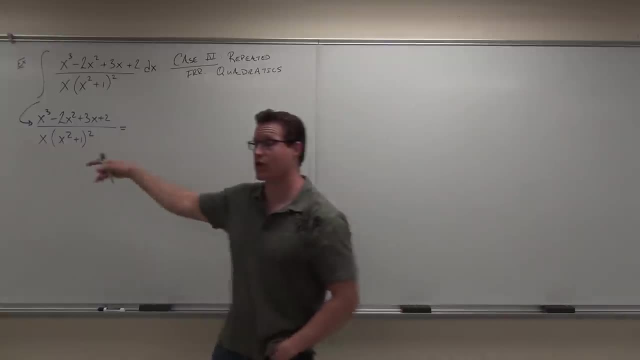 So we don't need to do long division or anything like that. This is nice because that would be very hard to do with this problem. We don't want to do that. We don't have to redistribute and then refactor. OK. 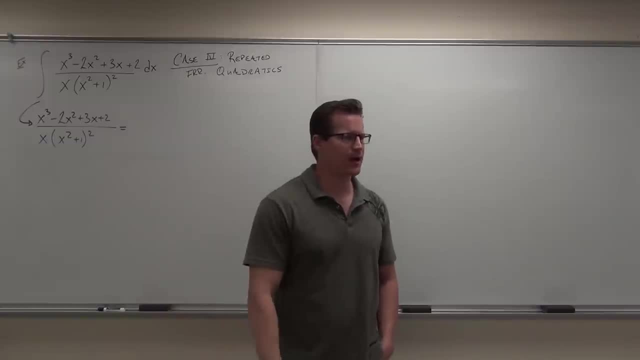 Can you tell me? Actually, you know what? Why don't you do it? Why don't you write out the fraction that you're supposed to have here? I think you guys are all at that level. OK. Go for it. 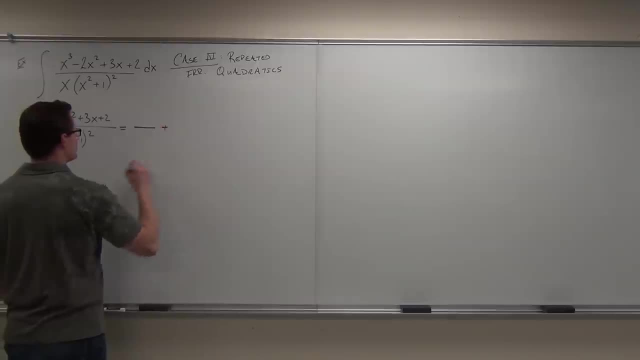 I know there's at least one. How many in total are we going to have? 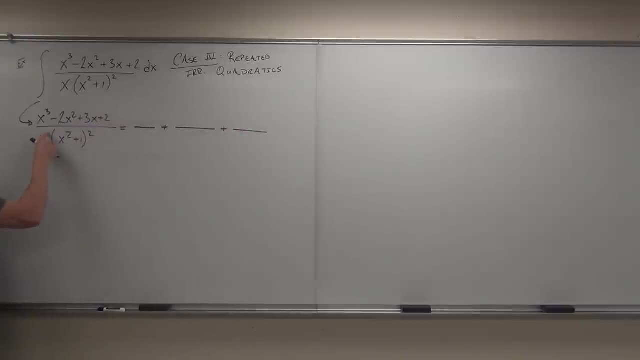 Three. Three. Power one. One, two, three. Yep. You're right. 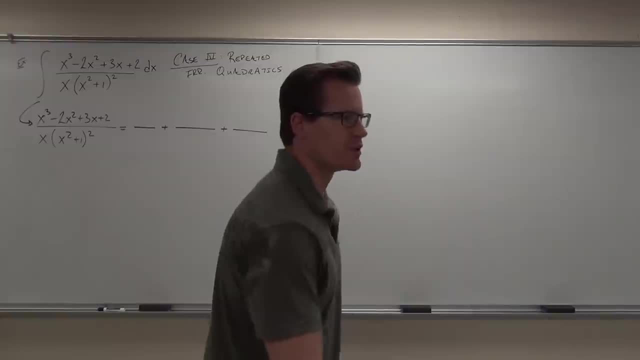 Can you tell me what the denominators will be? Tell me what the denominators will be. First denominator. What is it? x. Second denominator. x squared plus 1. Perfect. Perfect. Perfect. Last one. x squared plus 1 squared. Fantastic. That's exactly right. Show of hands if you've got the denominators. Perfect. Good. So repeated quadratics work just like repeated linears. You just put the factors until you reach the largest power. So here we have x to the first. No big deal. 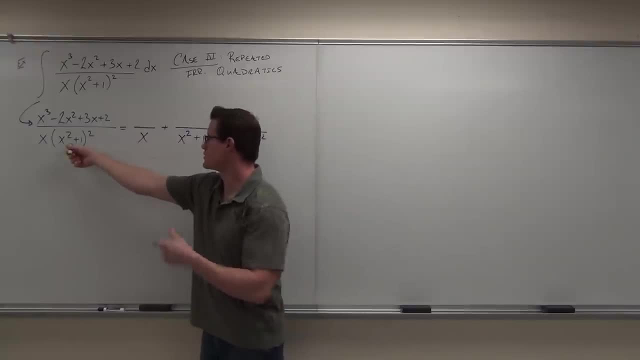 We have x squared plus 1 to the second. Well, we need our first power. We need our second power. Now let's fill the numerators out and make sure we get those right. What's the first thing we're going to write here? K. Is this going to have x's up here? Yes. It's a quadratic. It's going to be bx plus c. This one, it's also quadratic. bx plus c. All right. So what's the first thing we're going to write here? K. Is this going to be bx plus c. This one, it's also quadratic. bx plus c. All right. Did you get that? Yes. All right. Does it make sense to get that? We have linear. 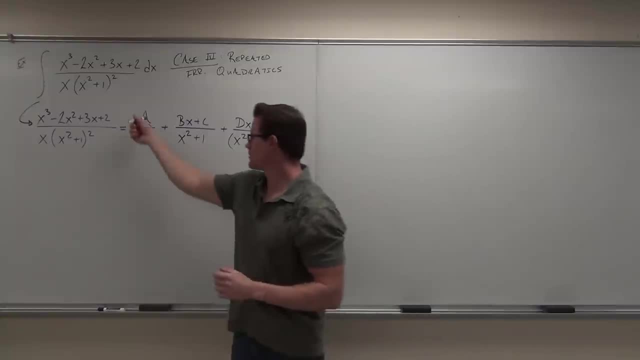 It should just be an a. One power less. So one degree less. Quadratic should be one degree less x's. Quadratic should be one degree less still have an x. 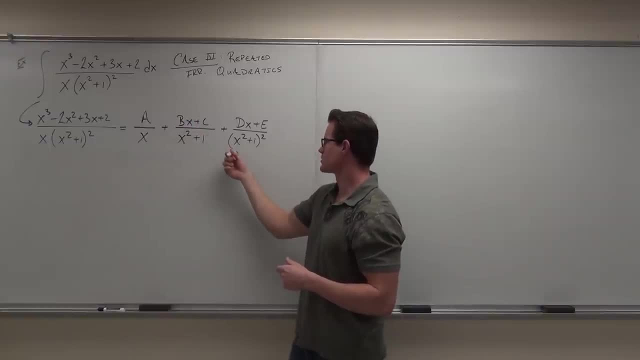 Show of hands if you feel okay with this one. Are you sure? You positive? This is big time, right? If you don't get this, are you going to get your problem right? No. That's an issue. 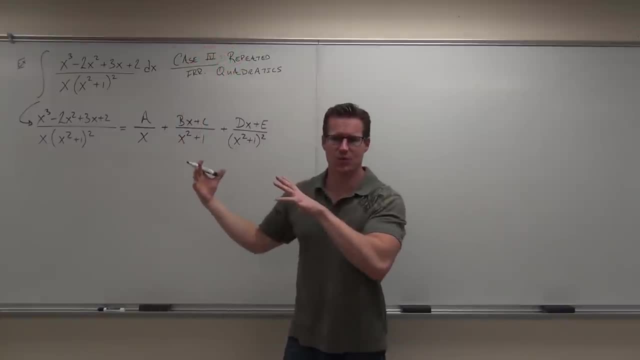 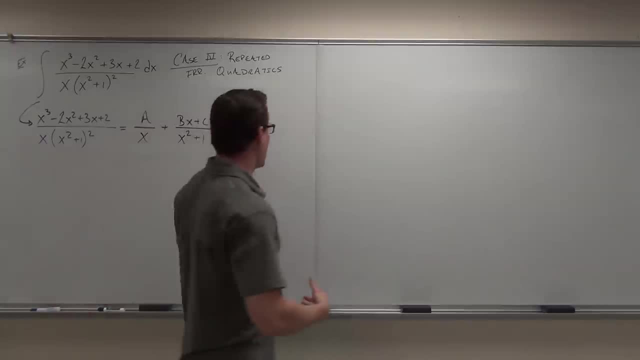 Now, moving on. What's the next thing we do after we figure out how our rational expression is going to be decomposed into partial fractions? What are we going to do? Find a common denominator. Let's find a common denominator. Why don't you go ahead and do it. See if you can do it. 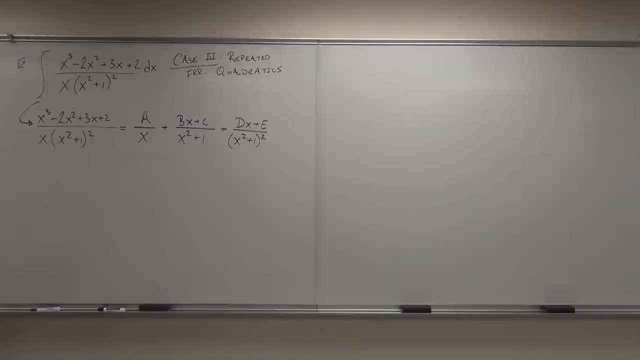 I'll do it up here in just a second so I'm only going to give you a little bit of time. 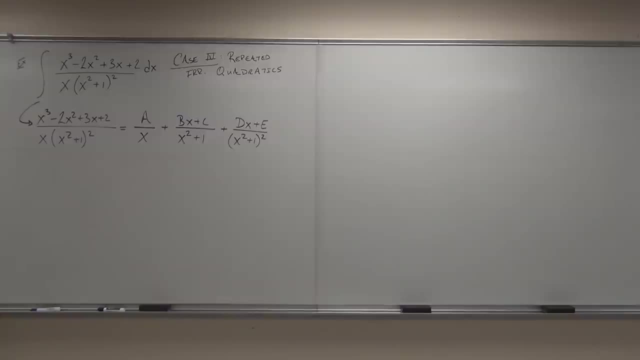 Did you get it back there? So remember what we do, we look here, we look here, we multiply by the missing factors just like any other time in the world you would ever find a common denominator. Just like in algebra. It is algebra. This is all algebra. 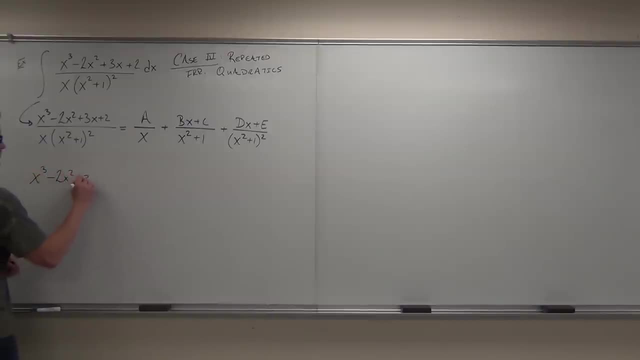 Okay, I know I've said it about 50 times so far, but your idea is to find a common denominator between here and here. 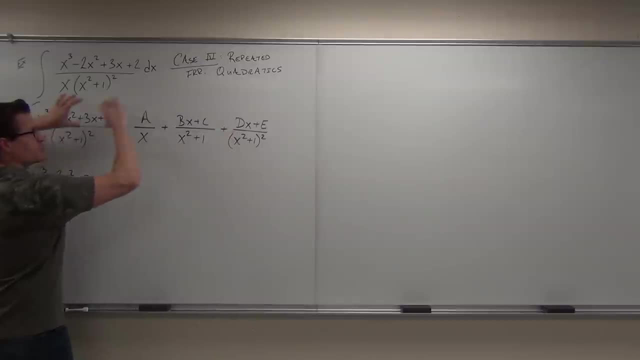 If you can do that, then if the denominators are the same, your numerators must also be equal. 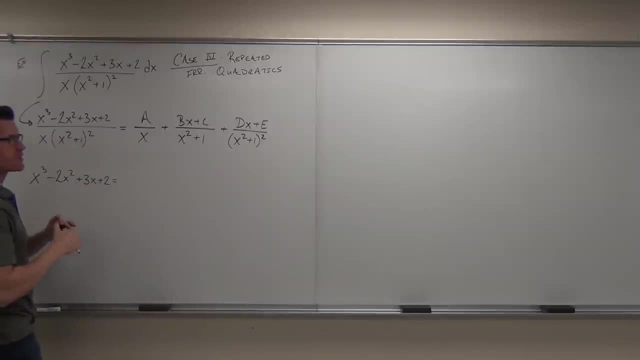 Therefore, when we multiply by the missing factors, we get that common denominator automatically. That's why we don't write these denominators here. 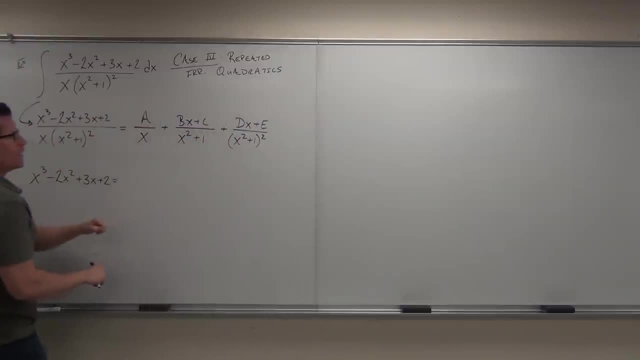 So we're going to have numerator equal to our new numerator. What I do, I look here and I look here at each individual fraction. I just multiply by what's missing. 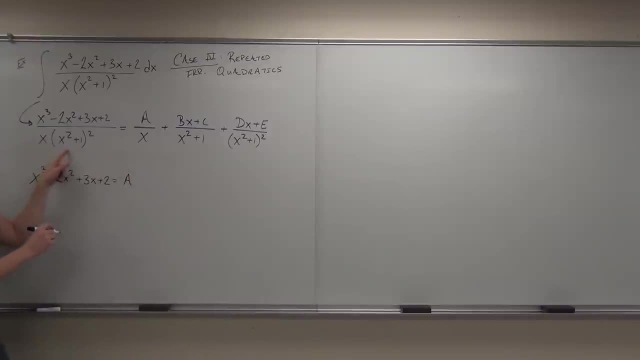 So I know I'm going to have a, and the thing that's missing between here and here is my x squared plus 1. You guys follow me on that one? 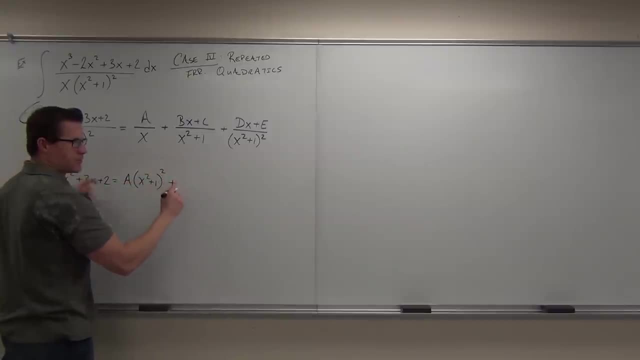 Between here and here, well, be careful, I know some of you guys hate parentheses. I don't know why you hate them, they're friendly. When you have bx plus c, you've got to have parentheses there. You will be distributing. 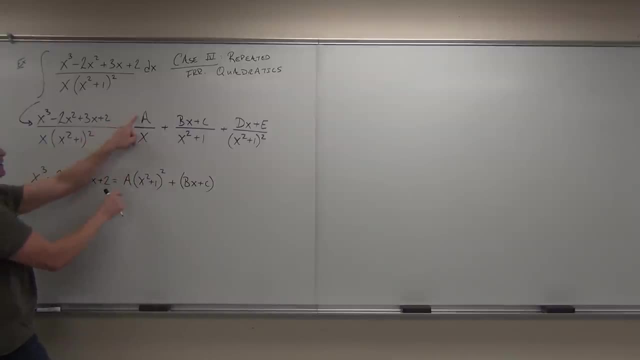 So a times, well, I'm missing this whole x squared plus 1 squared, got it. Bx plus c, okay, I'm missing, what am I missing between here and here? What's missing? An x and 1 factor after x squared plus 1. Good. I'm missing x for sure. 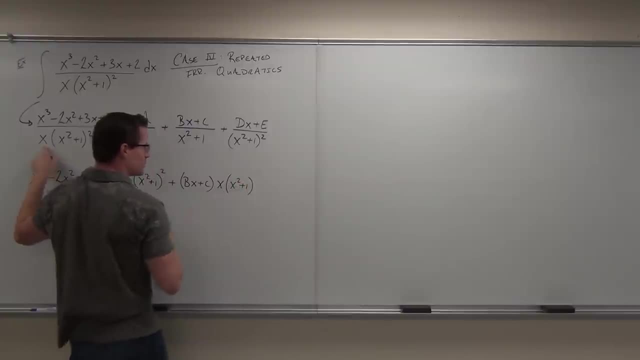 And then one, I like how you said that, one factor of x squared plus 1. Let's make sure. I don't have the x, so I got that now. I'm missing, oh, I'm missing the square. So I need one more factor than x squared plus 1. 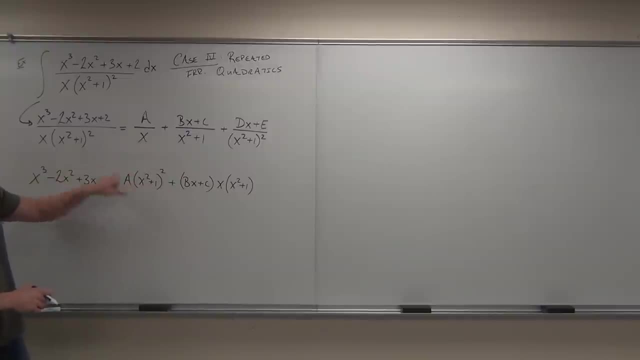 If you multiply this times this, it should give you this. If you multiply this times this, it should give you this. That's how this stuff works. So you're multiplying by the missing factors. You guys okay with that so far? 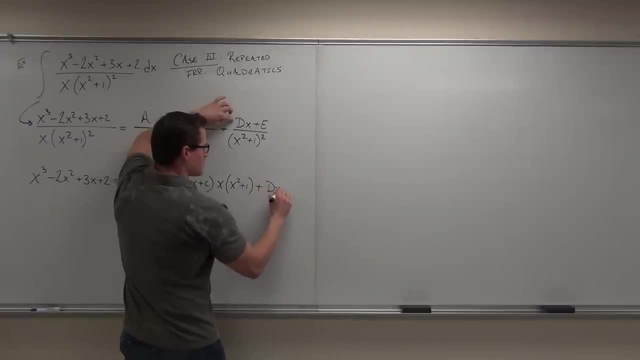 And lastly, we've got a, well, we have a dx. We've got a dx plus e, again in parentheses. So here we were missing this guy. Here we were missing x and one factor of this guy. Here we're missing what? So it's just got to be dx plus e times x. Okay. Chopin should be okay with that. Perfect. 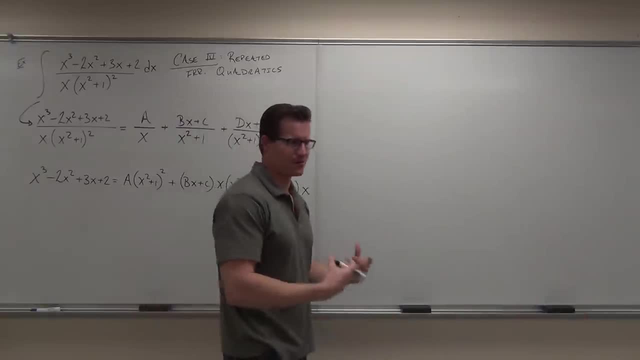 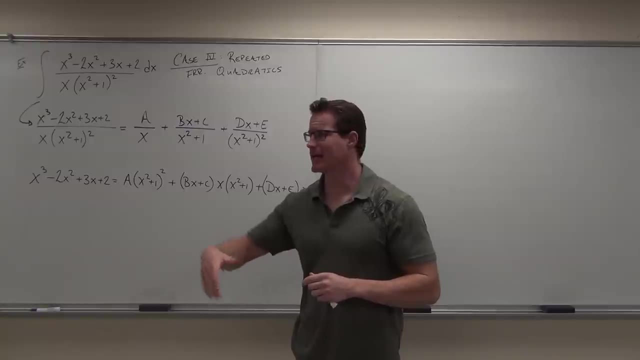 Now, I think I mentioned this earlier. When you have these quadratic factors, it's not as easy as when you have the linears. The linears was real nice because you could plug in numbers a lot of the times and eliminate entire terms. Like entire sections of this. You can't really do that all that well here. 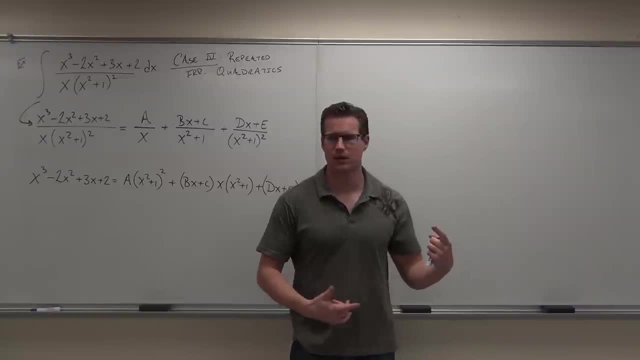 There's one number I'd probably plug in if I wanted to just really quickly. I'd plug in probably zero. If you plug in zero, this whole thing's gone. This whole thing's gone because x's would be zero here. This would be one. One squared is a. If I plug in zero, I get two. Right off the bat, I know that a is two. Does that make sense to you? 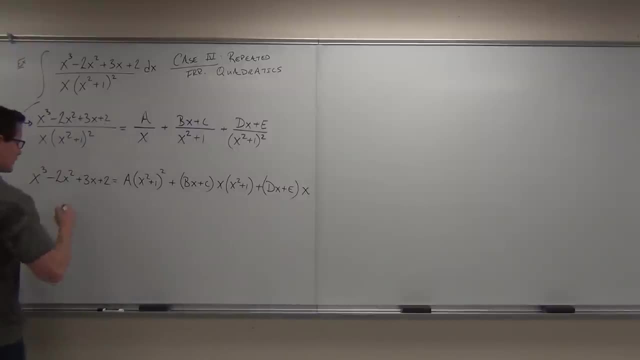 So I'd probably do that first. 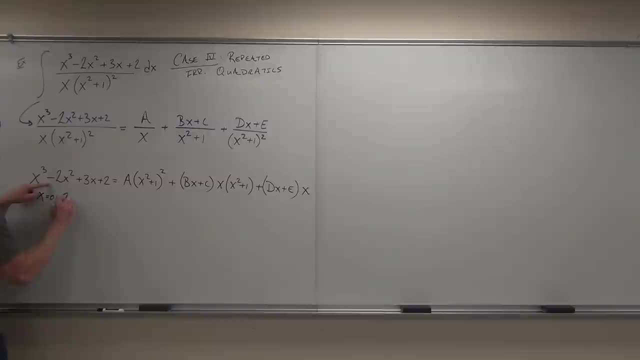 So if I do x equals zero. Okay. I know that two, so zero, zero, zero, here's two. Here's zero plus one is one. One squared is one. A times one is a. A equals two. All this stuff would go to zero. Zero times everything would be zero. 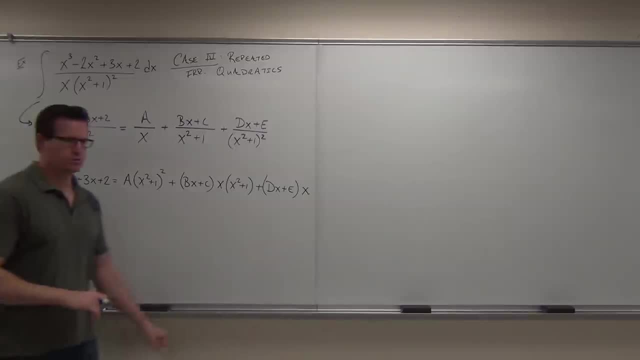 Zero times everything would be zero. So right now I know a is two. So if that's really okay with that logic. 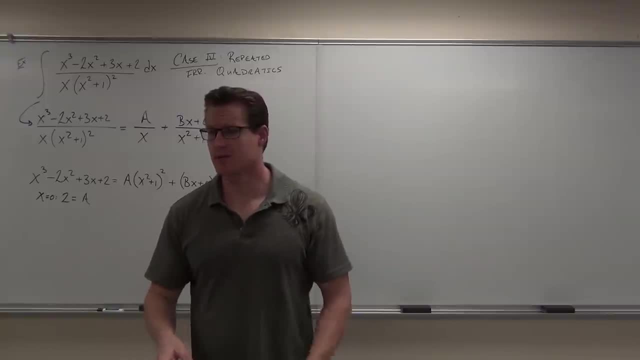 If you didn't do that right away, it's going to be very apparent to you later anyway. So it's really not that big of a deal. What do we do with the rest of this junk? 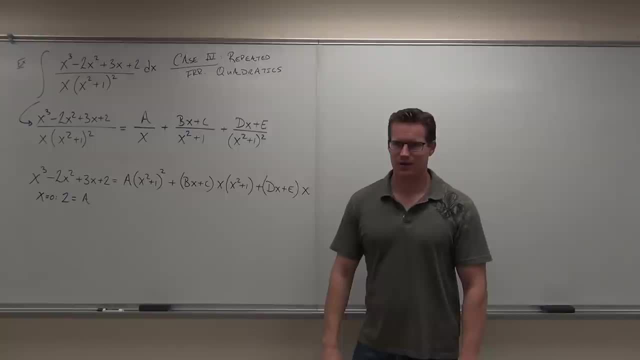 You distribute all of it. No, here's the problem. If you're like, well, wait a minute. Why can't we just plug in? Okay. Tell you what. 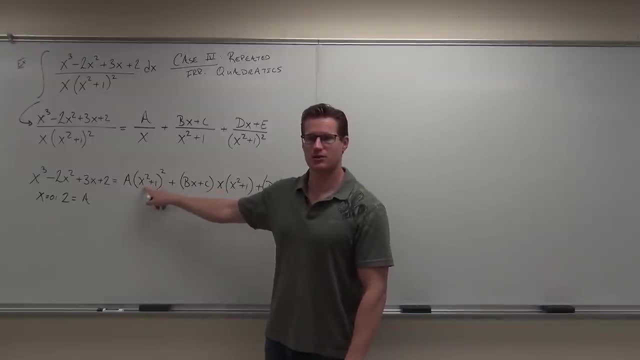 Give me a number here that you can plug in that makes it zero. I'll give you a million dollars if you don't use complex. 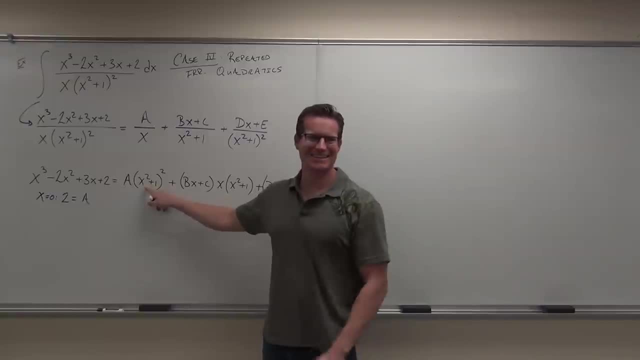 Dang it. I. Yay, I win. Yeah, we're not talking about complex analysis, are we? Class is horrible. Yeah. Yeah. That's it. Upper, that's later. Okay. 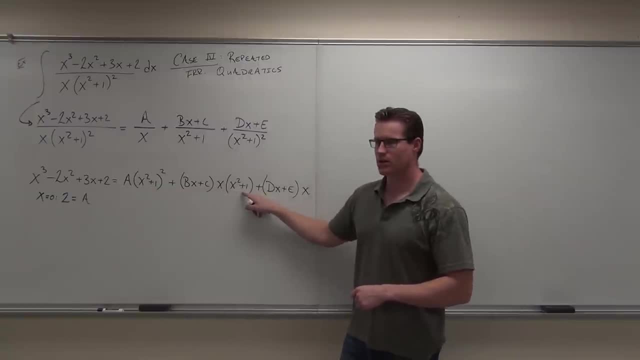 So no. Can you plug anything to make this zero? No. No. Can you plug anything to make this? I don't know because you don't even know what d and e are. 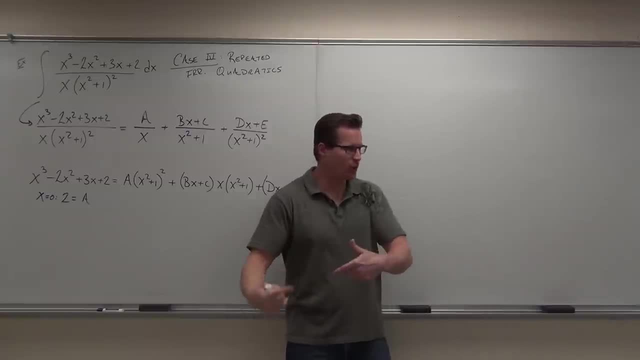 So no. The only thing we can plug in to help us here was zero. We're done with that. 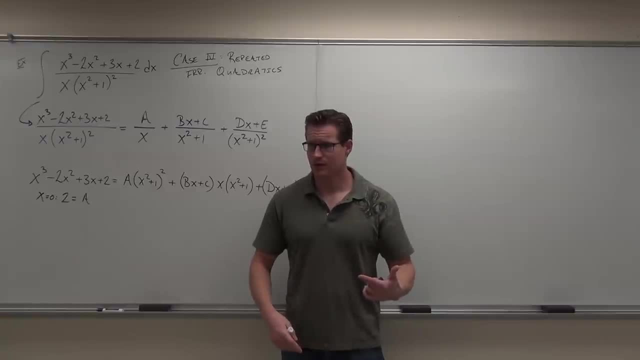 So you're left with? Distribute. You can distribute it. Distribute it. 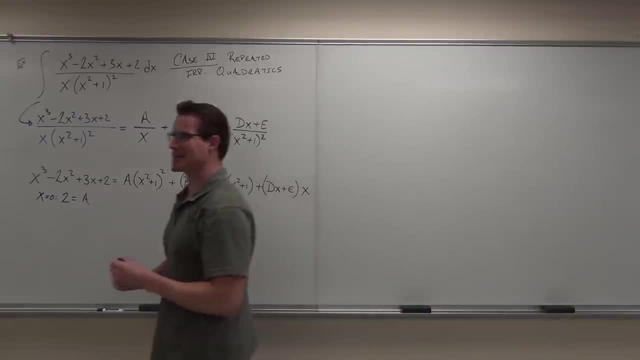